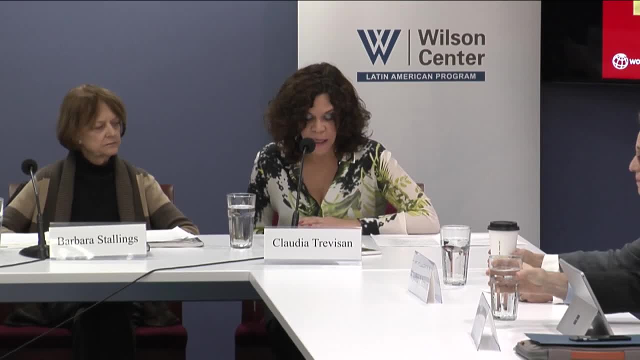 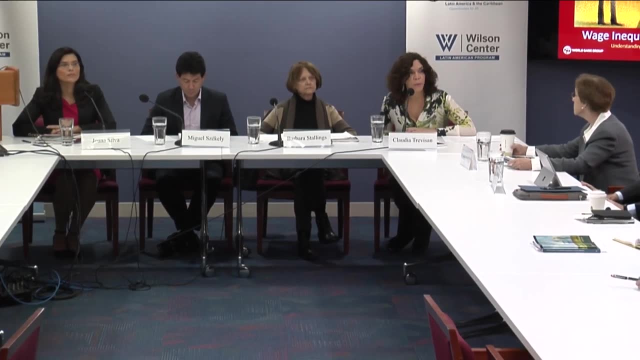 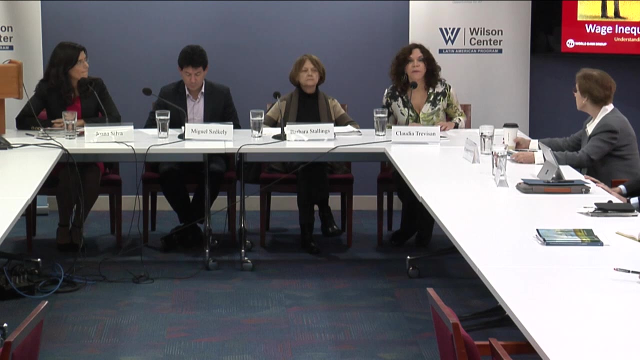 University and Miguel Zekla, director at the Center for Education and Social Studies in Mexico. I'd like to thank our partners: the Wilson Center, the World Economic Forum and the Estado de São Paulo. I would also like to greet our viewers who are following us on our Facebook page on the. 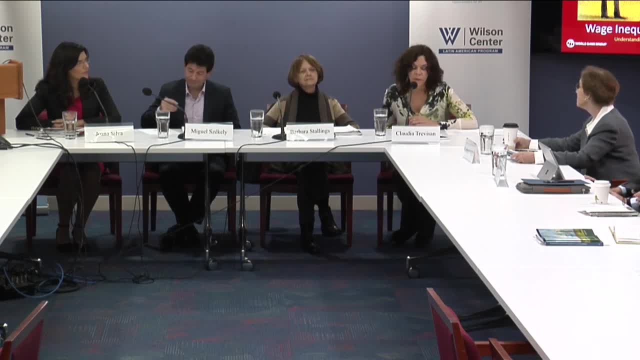 Estadão website. If you'd like to ask a question or leave a comment on social media, please use the hashtagcom and tag the page. Thank you, hashtag desigualdade salarial. This event is being broadcast live in English and in Portuguese. 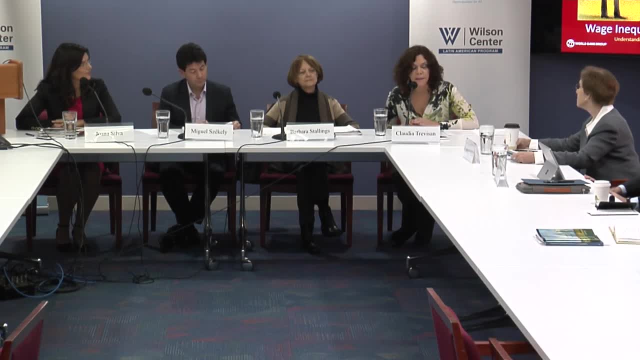 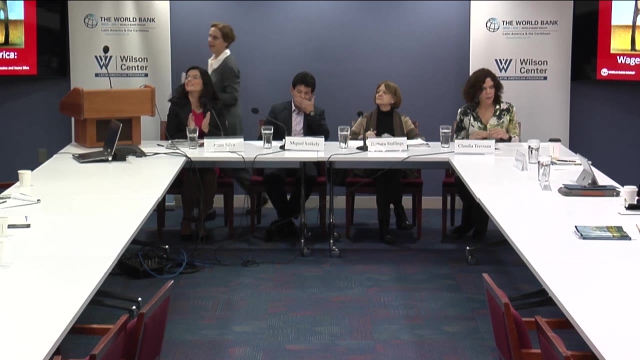 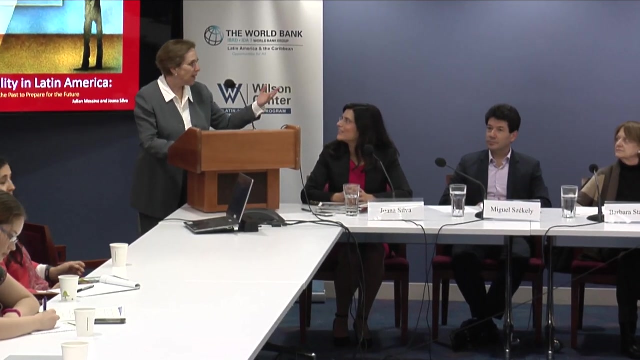 Please join the conversation, asking questions or commenting on the live stream with the hashtag wage inequality. Now please help me welcome Cynthia Arnson, Claudia. thank you so much, Gwen Gia. I'm delighted to join with the World Bank and our distinguished panelists. 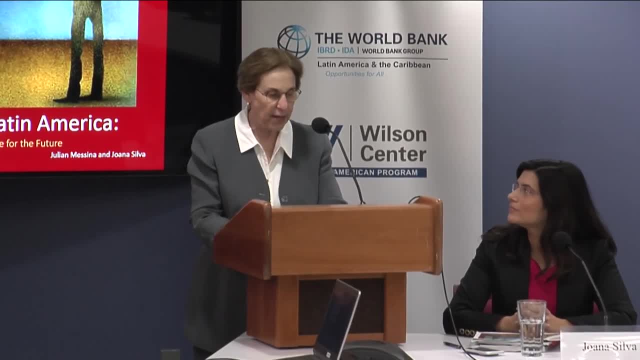 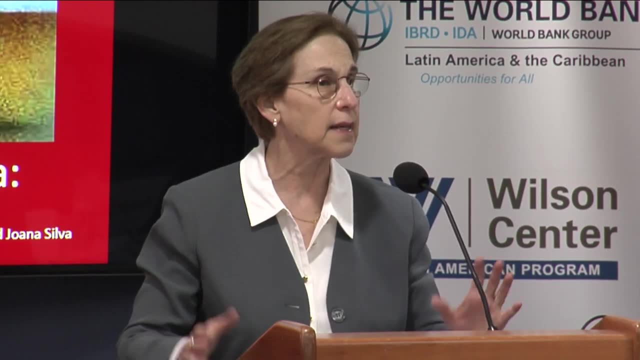 for a discussion of the trends and inequality in Latin America and the Caribbean, but, more importantly, the policies that are needed to sustain these trends into the future, And so I'd like to make a few brief observations to help frame the discussion, especially for 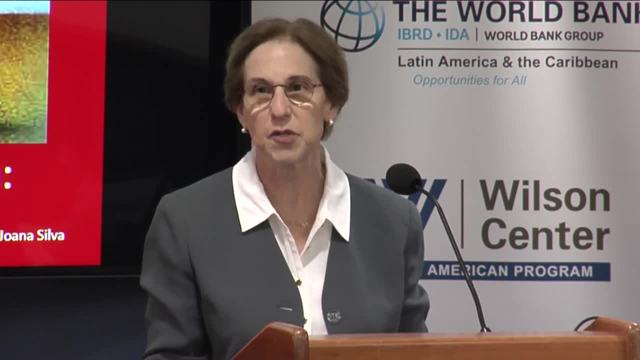 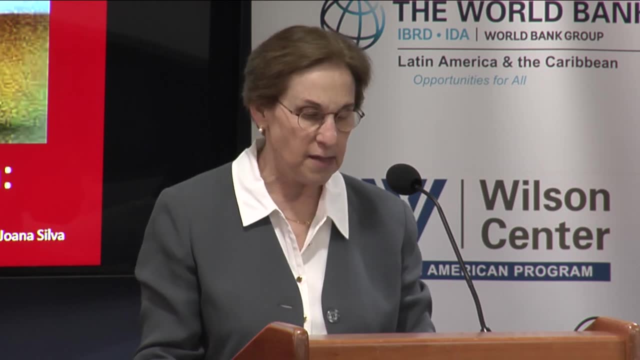 those who were babies or toddlers in the 1980s, when many of us were first reading about these issues in Latin America. A lot of people are probably too young to remember the debt crisis in Latin America in the 1980s, the so-called lost decade. 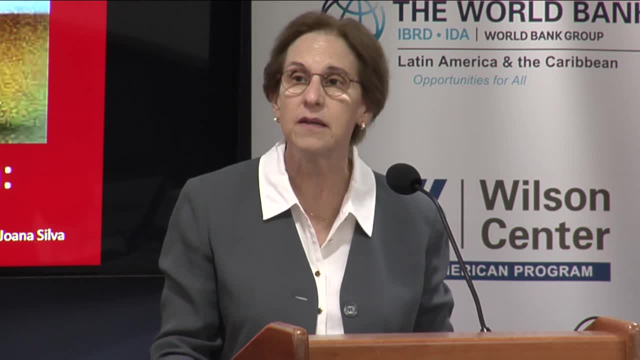 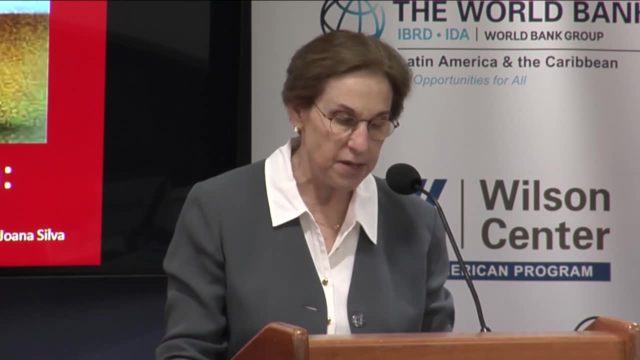 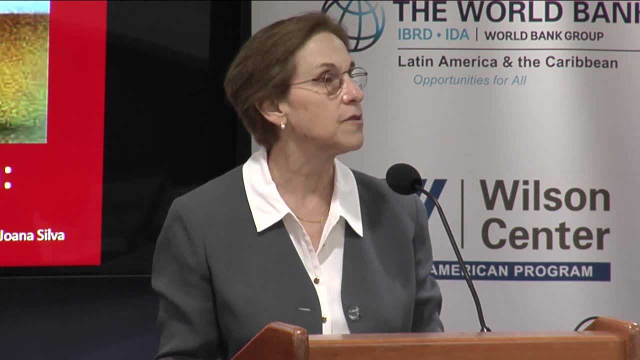 This was followed by policies in the 1990s of structural adjustment that centered on the privatization of state enterprises, the economic liberalization and reforms that dramatically reduced the role of the state in the economy and cut social spending, With perhaps only one exception. 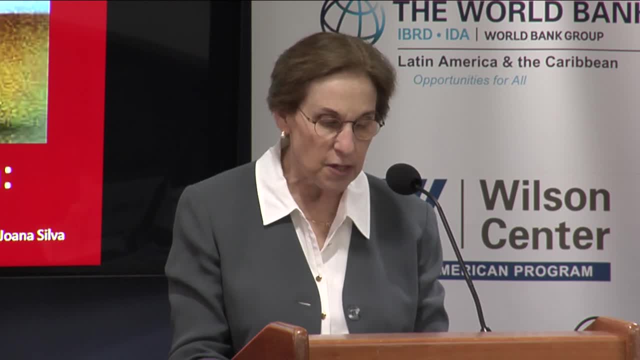 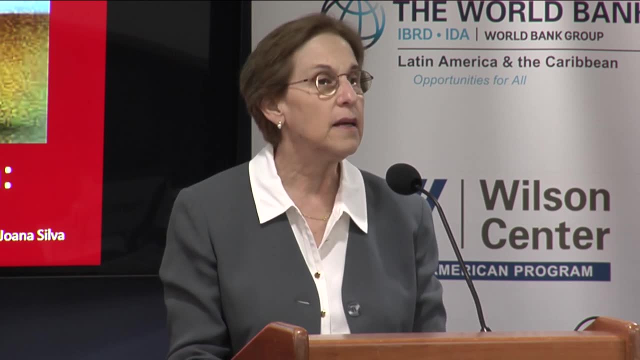 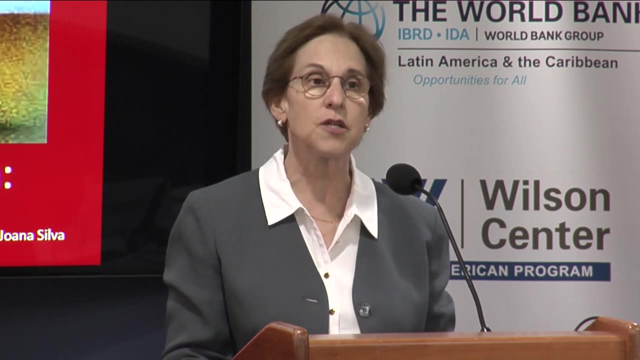 Uruguay, always exceptional. The policies of structural adjustment, which were dubbed, probably unfairly, the Washington Consensus, resulted in vast increases in inequality throughout the region, So much so that one of the explanations for the rise of the left in the 1990s and the 2000s- 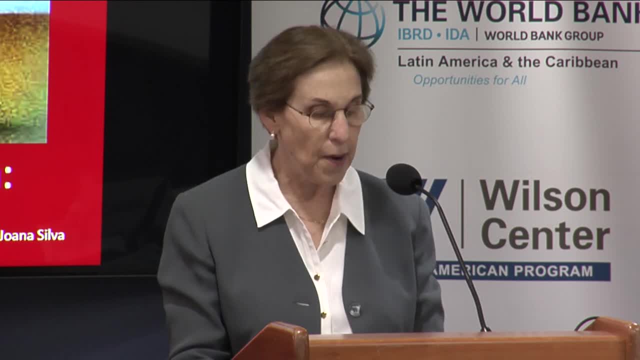 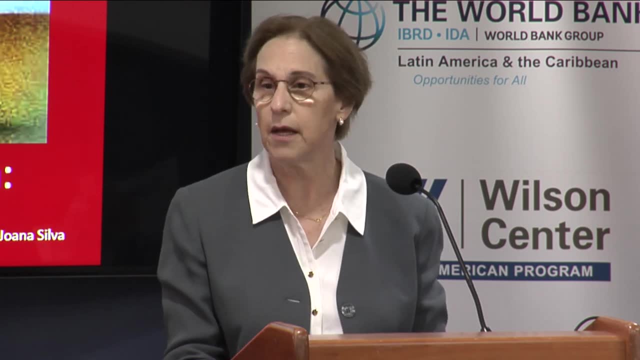 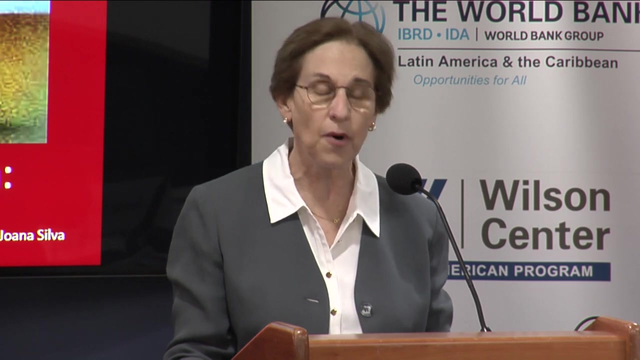 the so-called pink tide could be attributed to a popular backlash against the policies that had caused so much unemployment, dislocation and reduction in services. Then came the golden decade of the 2000s, with high commodity prices, the surging demand. 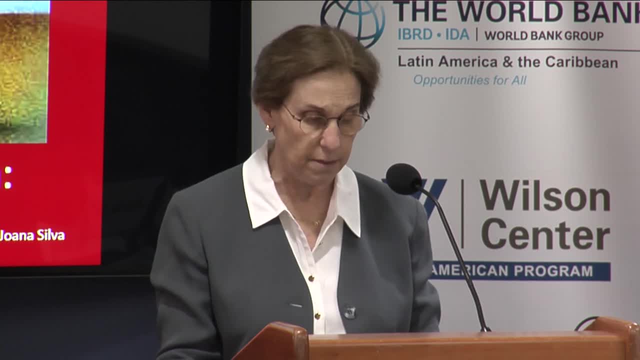 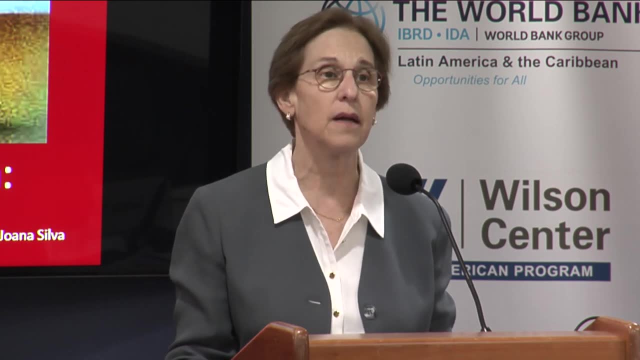 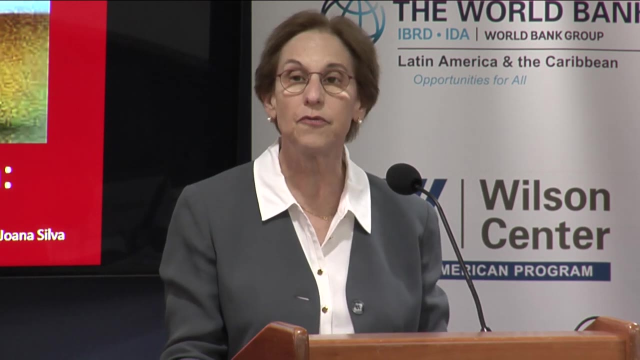 in China, with growth rates of something like 11%, demand for Latin American exports of primary materials and a determination of both center-left and populist governments in the region to bring the state back. As the world bank and others have documented so thoroughly, this decade saw historic reductions. 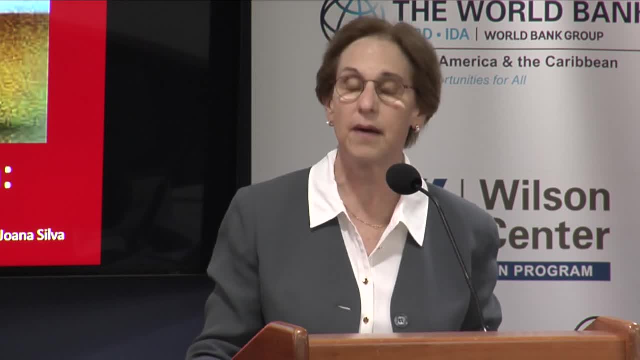 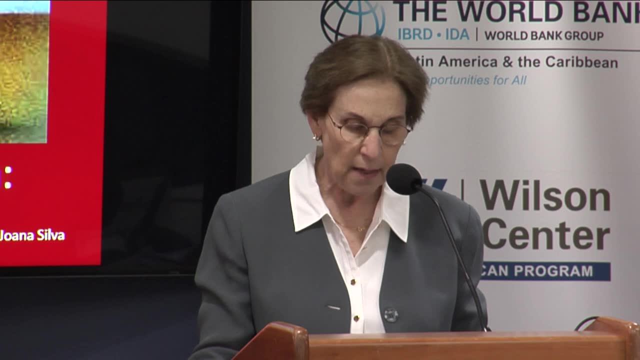 in poverty, the growth of the middle class and also important reductions in inequality. Of course, this is a vast oversimplification, but I hope these brief comments help to frame today's discussion about how and why inequality fell in Latin America and what spellbinding 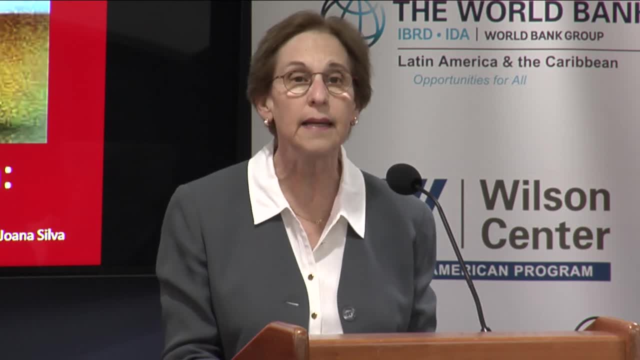 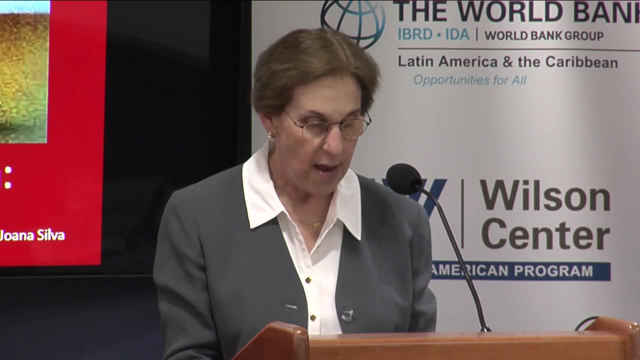 measures had been taken to make it so that the state as a whole could take full control of its own wealth. Thank you, Thank you. What specific policies can maintain or restore those trends, as Claudia was saying, at a time of weak growth overall? 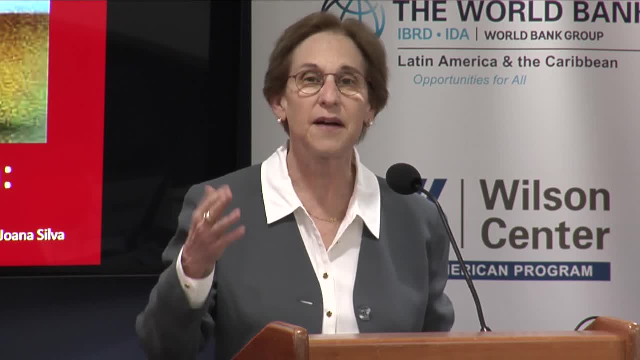 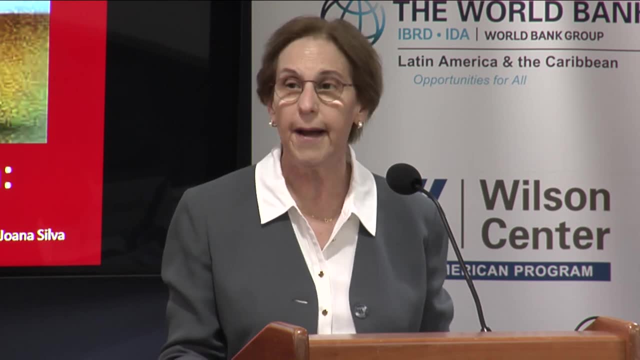 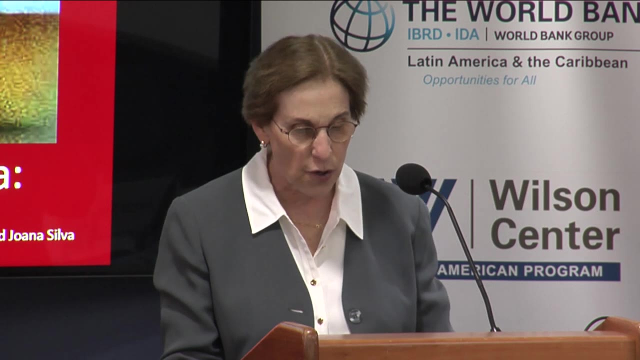 I'd like to say a special word of thanks to Jacqueline Doles, all of our staff there behind the lens of a camera, our interns Jamie Shank and Stephanie Arrella, Anders Biel of our staff, and also Candice – I'm sorry for mispronouncing that – de Cruz. 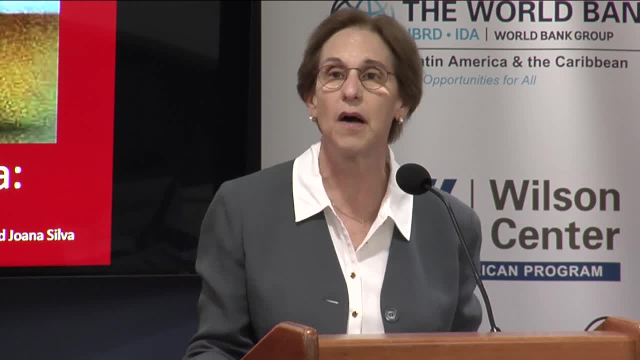 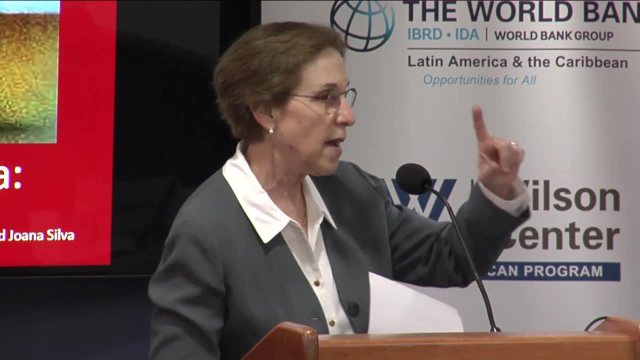 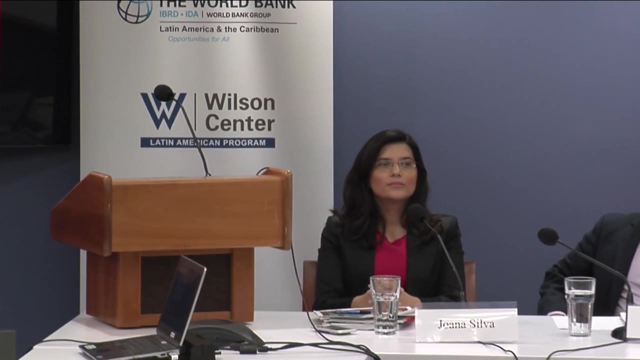 Rocha, Alejandra Viveros, Marcela Sanchez of the World Bank. It's a pleasure once again to join with you. Our next speaker, Daniel Leatherman – I forgot my notes here, excuse me – has joined us due to the illness of his boss. 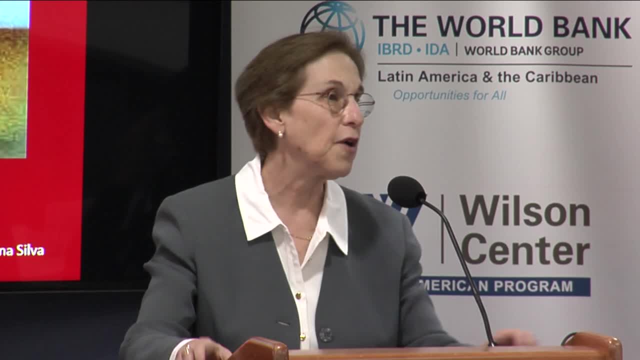 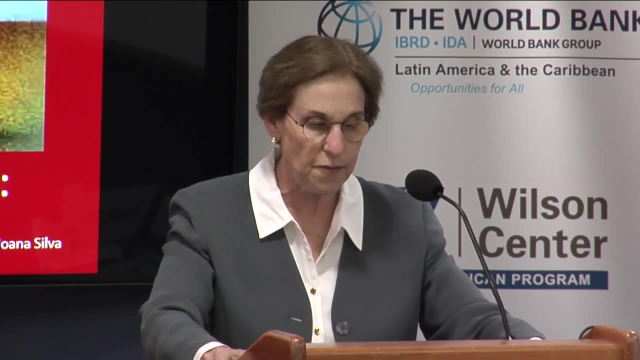 We wish Carlos Vey a speedy recovery, but we're very pleased to have Daniel with us. Daniel Leatherman is an engineer. He's a native of Chile. He is the lead economist and deputy chief economist for Latin America and the Caribbean at the World Bank, positions that he has held since May of 2013.. 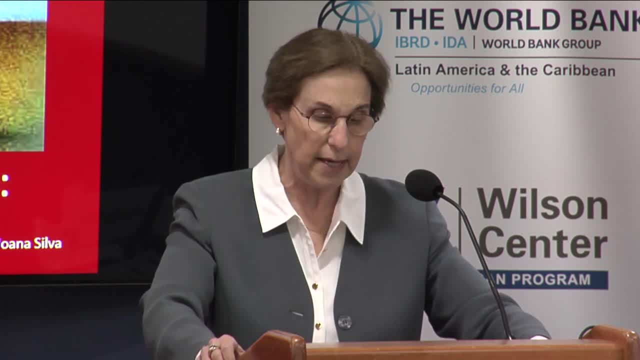 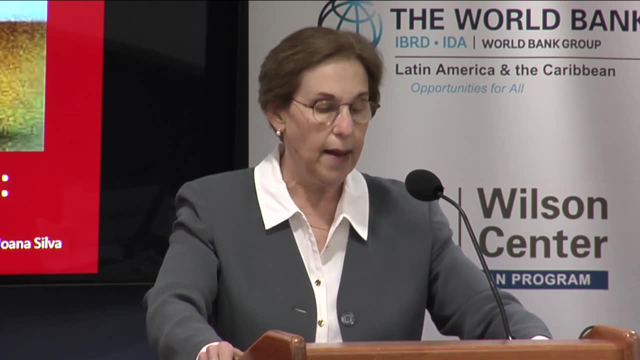 He's had a number of positions of leadership within the bank – the lead trade economist in the International Trade Department, senior economist in the Development Research Group and, prior to joining the World Bank in 1995,, he worked for the United Nations Economic Commission for Latin America. 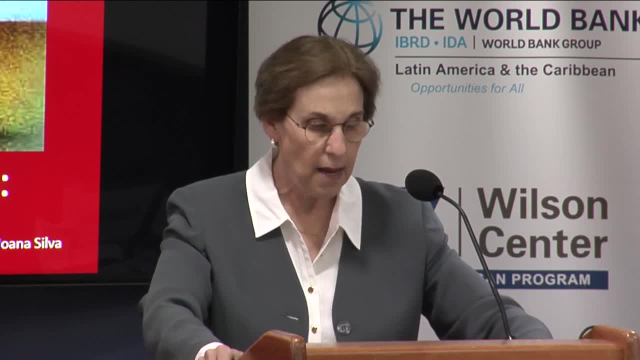 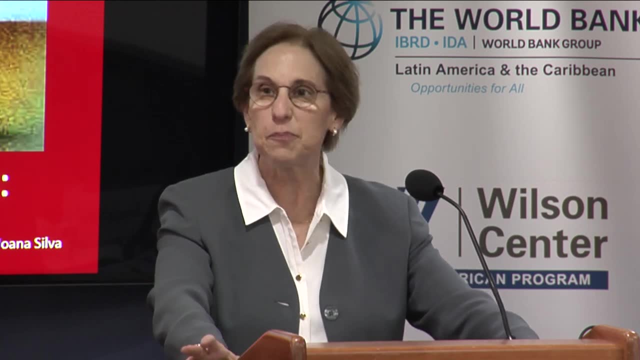 He's also an associate professor at the University of New York and the Caribbean, Barbara Ewan. he probably know many people in common. There you go, There you go, There you go. Daniel has published widely on issues related to economic development, financial crises. 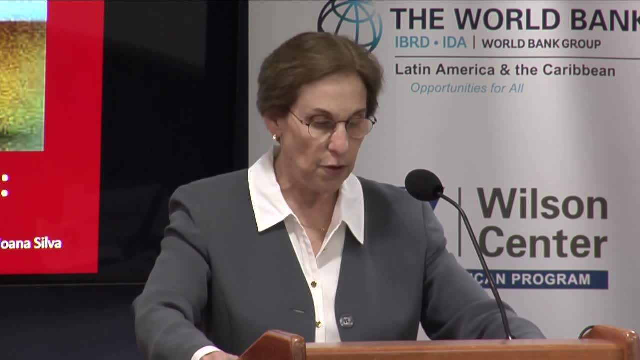 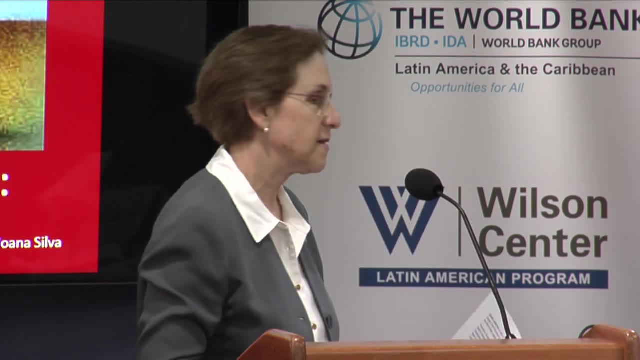 crime, political economy of economic reforms, innovation, international trade, labor markets. He has a BA in political science from Yale and an MA and PhD from my alma mater, Johns Hopkins University School of Advanced International Studies. Daniel, thank you for joining us. 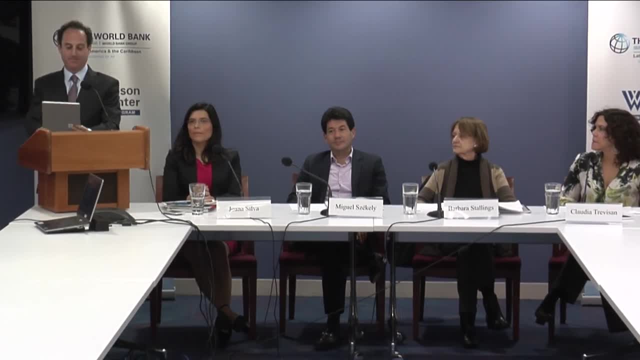 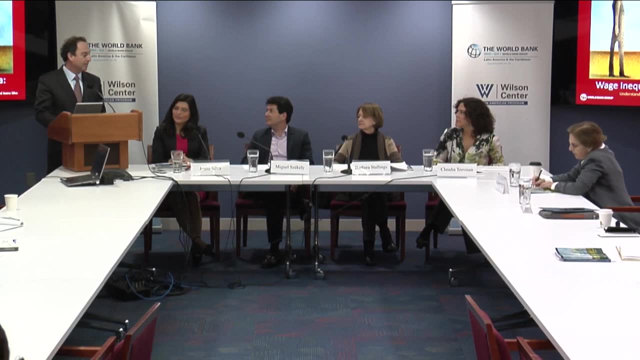 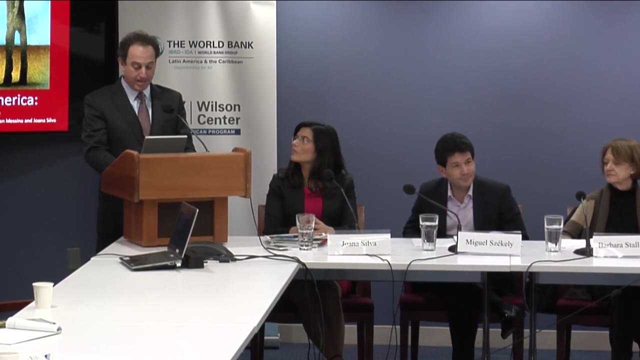 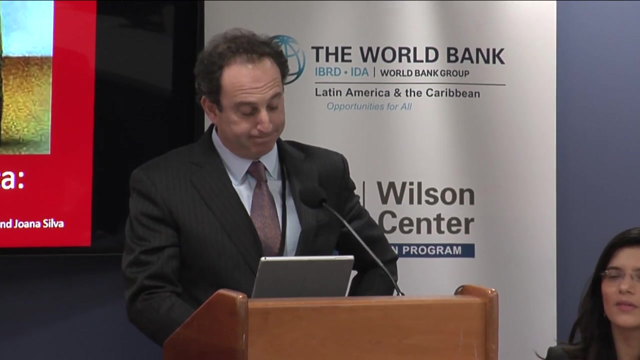 Good morning everybody. It's an honor and a pleasure to be here. We have a nice program here with Cindy's team, and I would like to start by thanking everybody for all of those attending in person, as well as those who are watching us online. 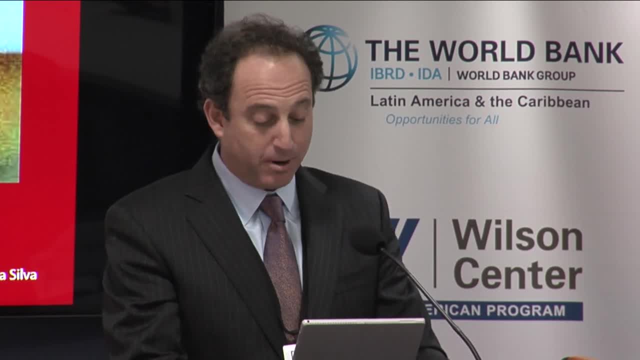 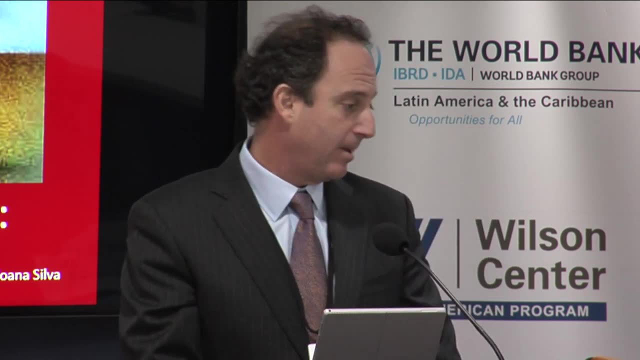 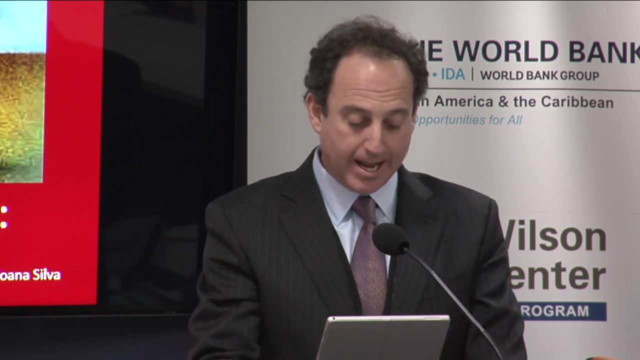 Thank you so much for joining us. We're delighted to partner yet again with the Latin American program of the Wilson Center. This time, we're gathered here to discuss a new book by Joanna Silva and Julian Messina titled Wage Inequality in Latin America: Understanding the Past to Prepare for the Future. 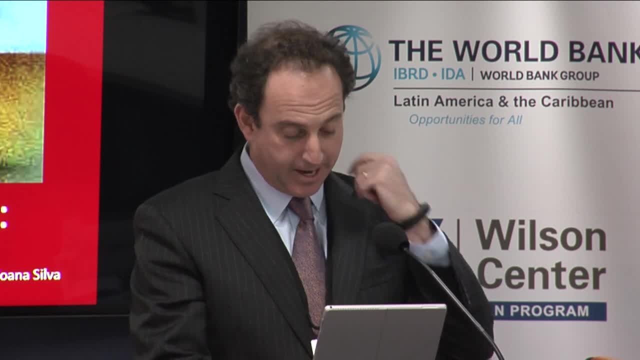 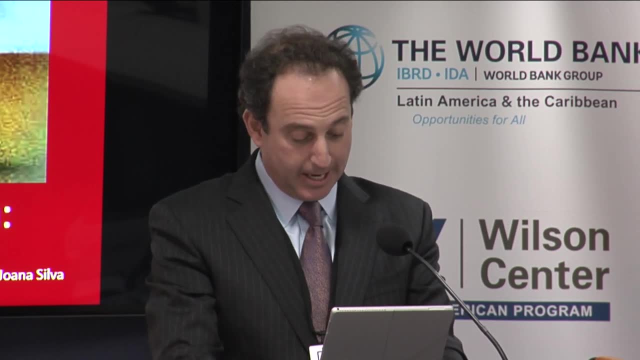 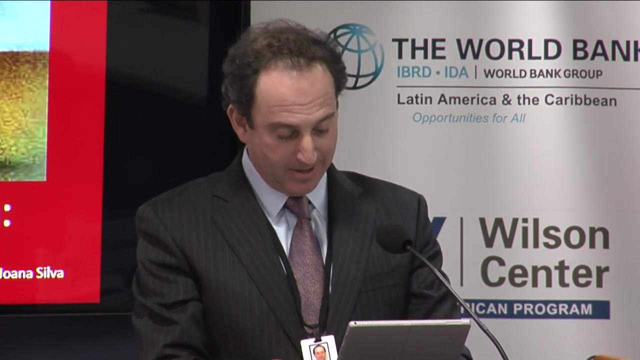 And again I would like to thank you for joining us. Thank you, I would like to thank the Wilson Center and Cindy's team. We have an awesome panel: Dr Barbara Stallings from the Watson Institute for International and Public Affairs at Brown and Miguel Seque, Director of the Center for Education and Social. 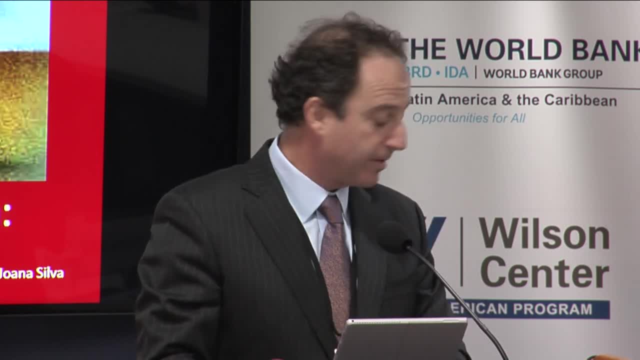 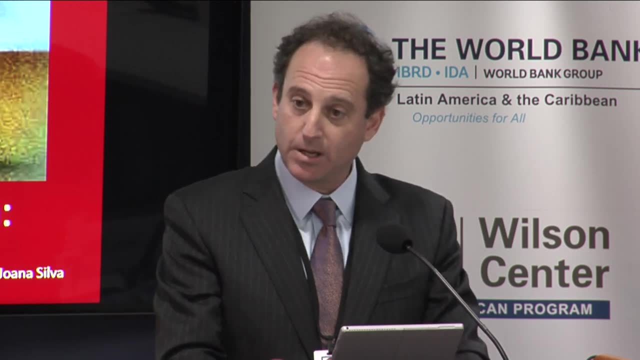 Studies in Mexico. We're very much looking forward to hearing your insights on this important topic. Indeed, inequality has been a historically important subject. Thank you, Thank you. I would like to begin with the lecture on the role of equal society in Latin America. 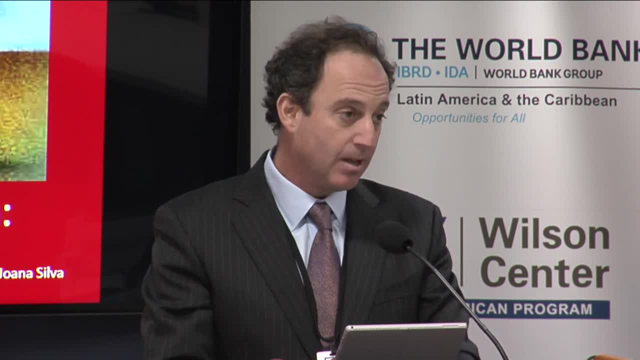 and the Caribbean. I do not think that the first decade of the 21st century has understood what the power of equal society means, because, as a expansionist or a power builder, it is important for academics but more importantly for our societies in Latin America and the Caribbean. 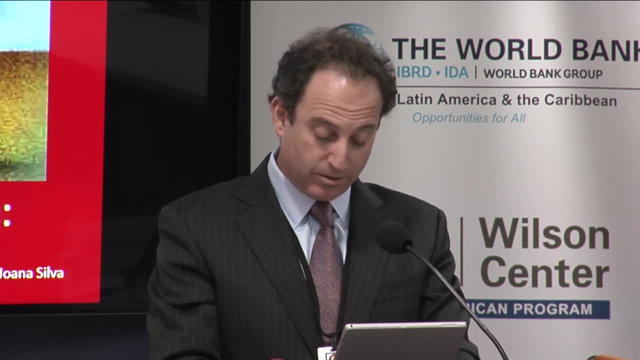 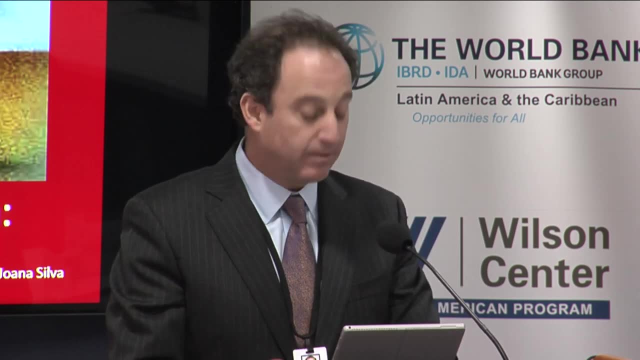 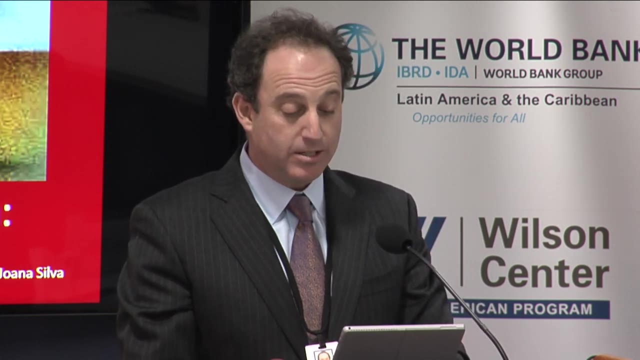 At a time that our countries are finally resuming growth after six years of slowdown. it is worth stressing that the region achieved something that's truly remarkable during the first decade of the 21st century. It sustained vigorous economic growth with declining inequality. This was in sharp contrast with the rest of the world, where the issue of inequality 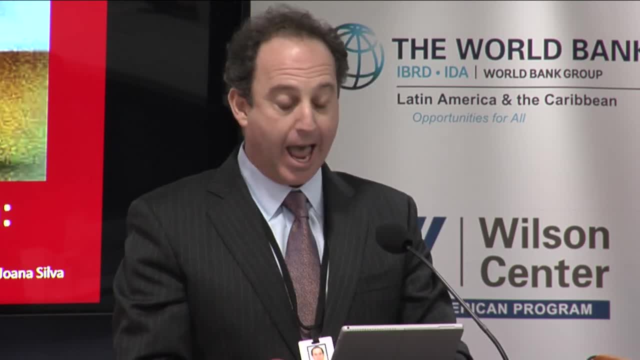 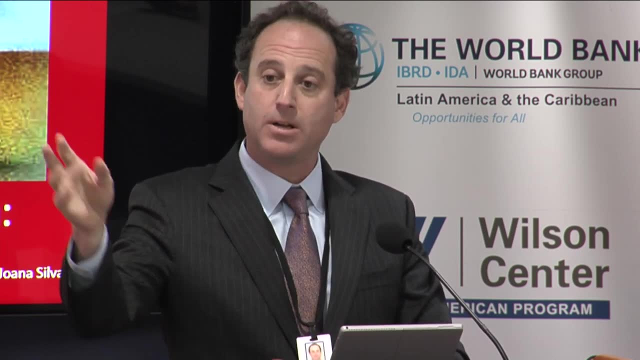 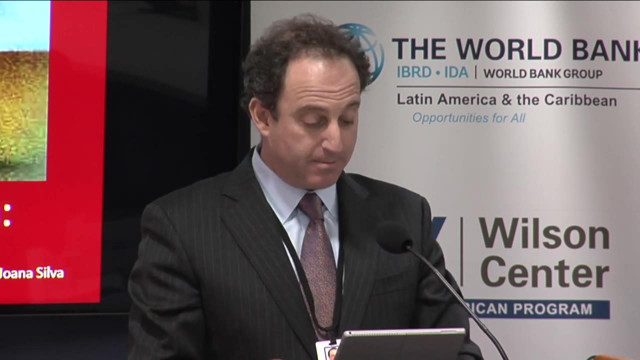 has surfaced to the top of the scope of the policy discussions and where most countries have struggled with rising inequality: in the United States, in Europe, in China and almost in every other corner of the emerging developing countries, Latin America and the Caribbean, in fact. 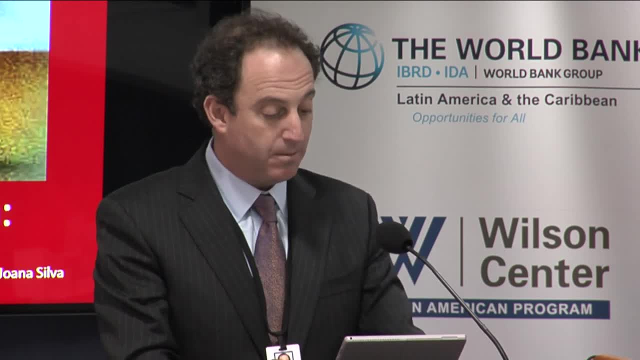 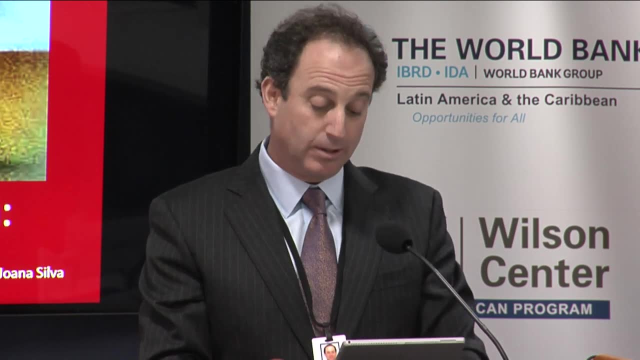 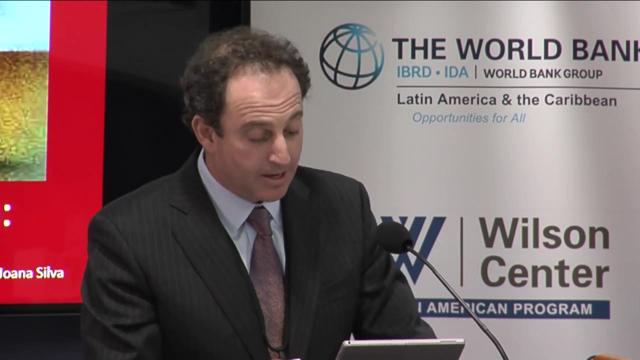 has demonstrated that inclusive growth is attainable. So what caused this unique reduction in wage inequality- in fact of household income inequality- in the region? Does this remarkable development for Latin America and the Caribbean bring important insights that we can share with the rest of the world? 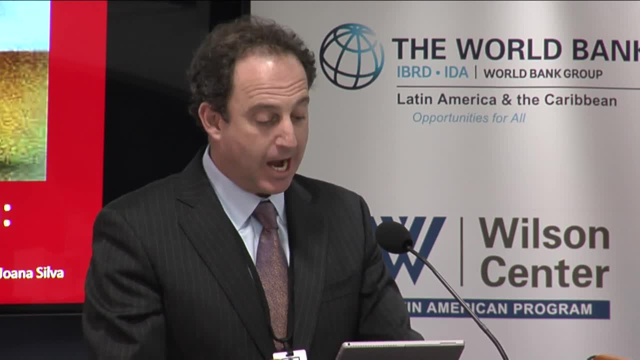 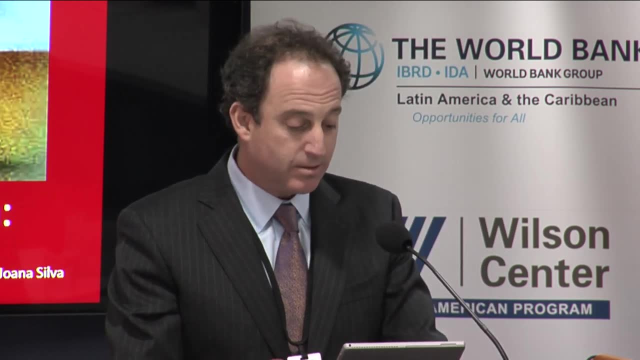 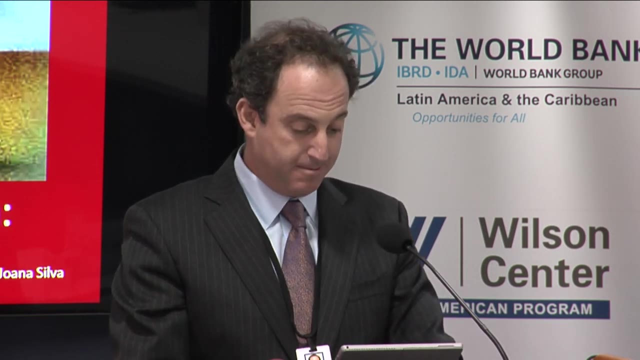 What happens now that growth is lower? How can we better prepare for the future of a potentially new normal of slower growth? Those are the main questions that this book seeks to answer, And there are valuable answers there for promoting growth with equity In this low-growth environment. it 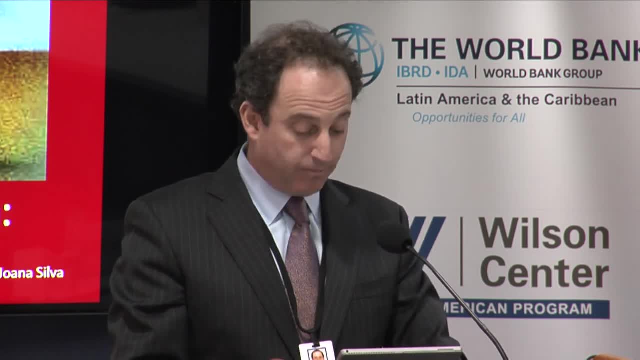 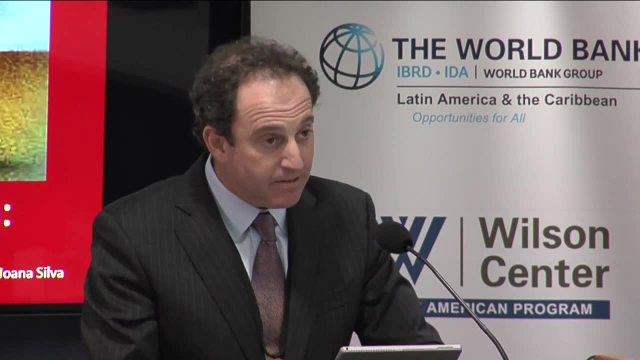 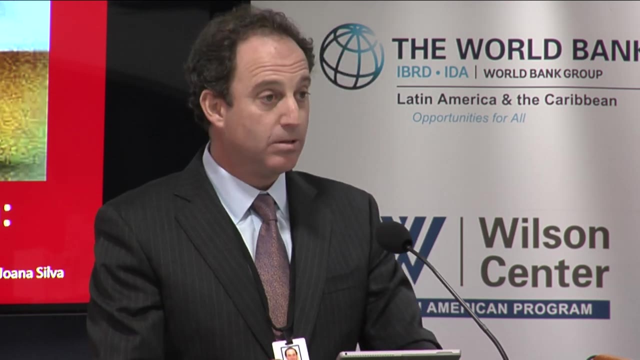 is important to assess how to move forward with policy reforms. We have to ask whether the social gains that Latin America and the Caribbean has achieved in the dawn of the 21st century, whether or not these gains are sustainable well into the future, and whether lower wage growth is occurring. 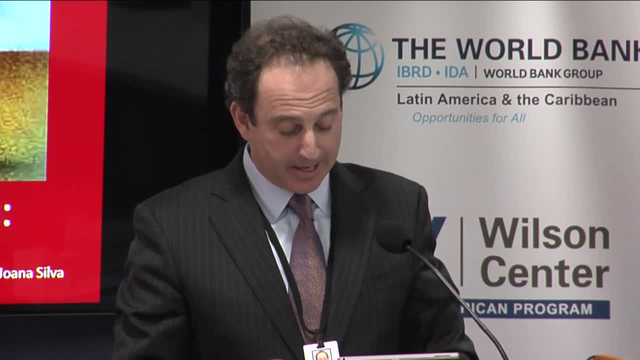 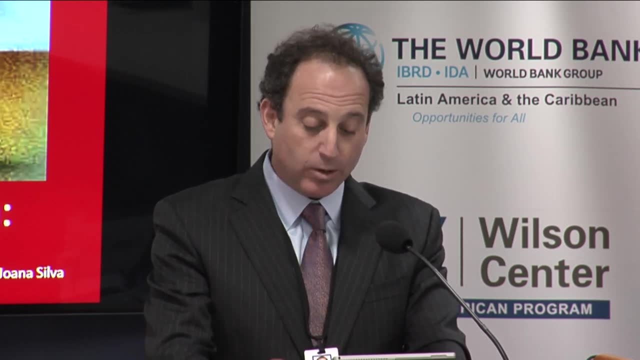 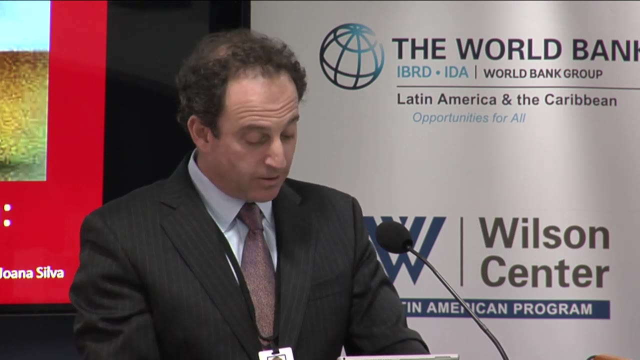 across all segments of the distribution in Latin America. Thank you. In Latin America and the Caribbean? or is this slow and disproportionately hurting those who have less? How can further progress be achieved? To answer these questions, it is essential to understand the successes of the past. 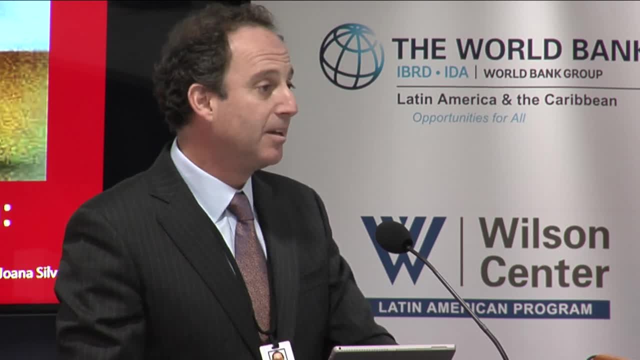 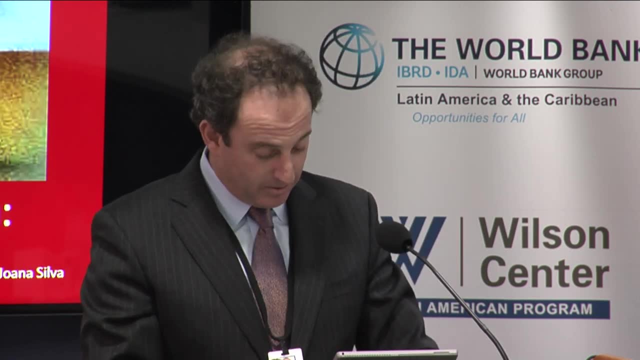 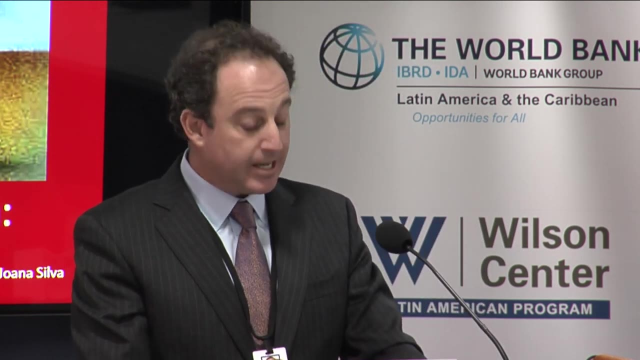 And a key contribution of this report is precisely to teach us about the past in order to prepare for the future. The discussion of wage inequality is especially important, given the enormous inequality which is still prevalent in our region. Investing in our people should definitely be a priority. 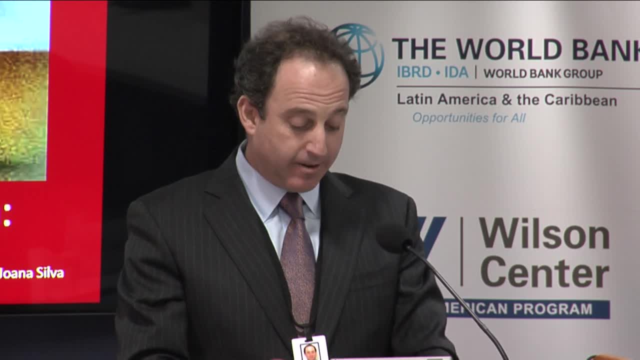 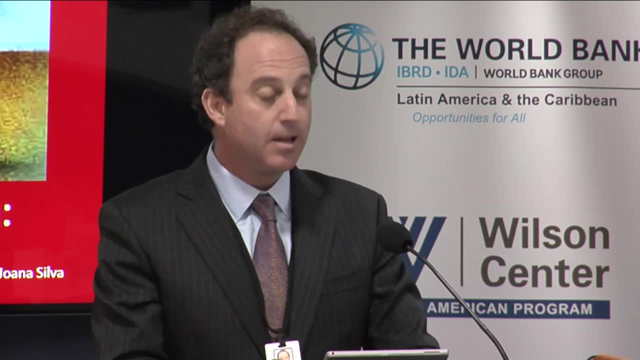 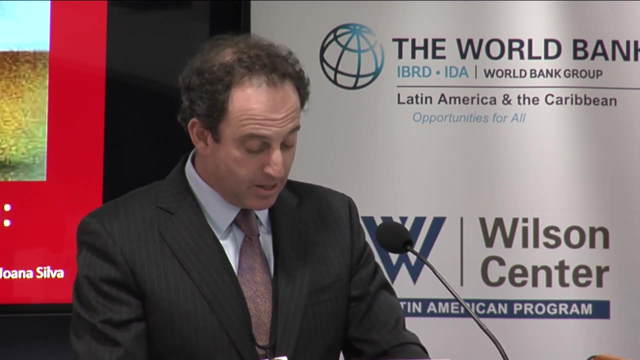 We need to work to create equal opportunities for all. One of these areas is the quality of education, which plays a fundamental role in generating the skills the labor market will demand of our citizens well into the future. Again, it is truly an honor to have this book and topic. 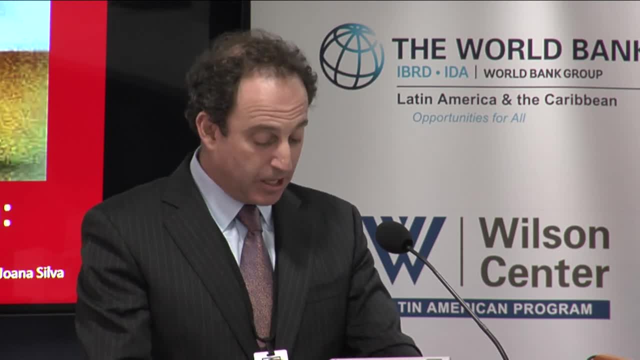 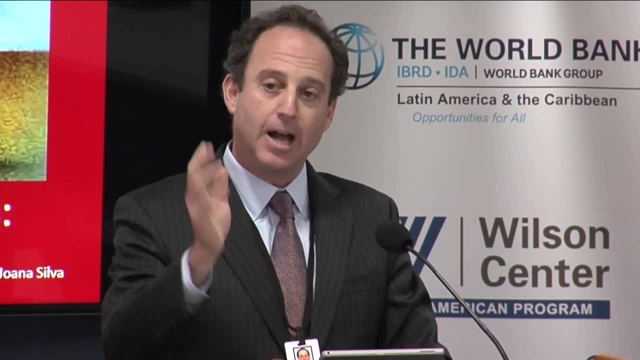 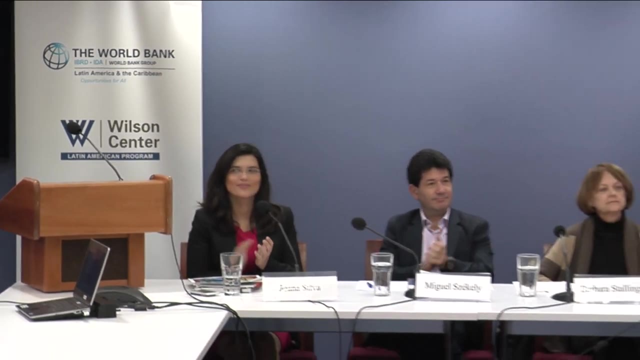 discussed here today at the Wilson Center by such a distinguished group of speakers. Thank you so much for the opportunity to share these insights with all of you in person and online. Thank you very much. I'd like now to invite Joana to present the report. 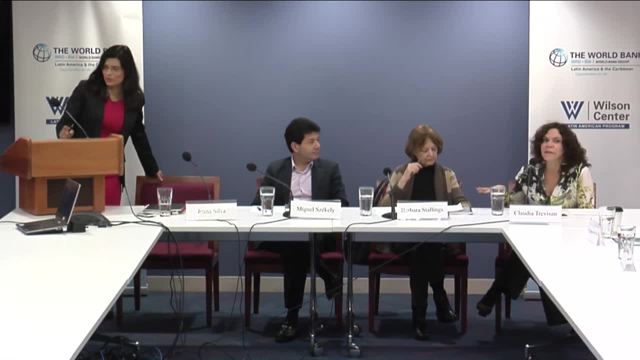 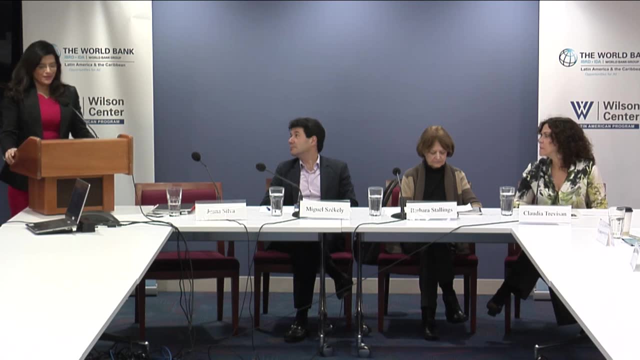 After that we are going to have a half an hour discussion with the panelists And after that 20 minutes for your questions. Thank you, OK. Thank you very much for the opportunity to present this new World Bank report here at the Wilson Center. 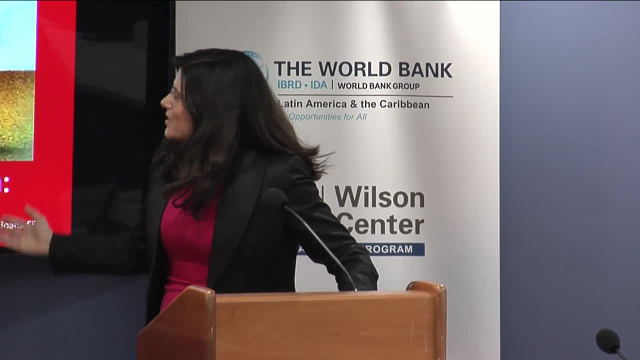 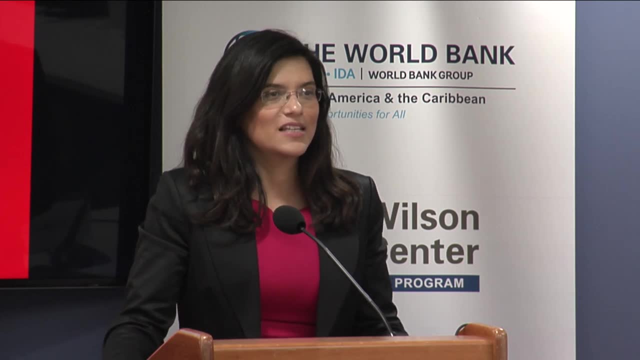 This is truly a pleasure We are going to. this book is about wage inequality in Latin America: understanding the past to prepare for the future, And this was research led by myself, along with Julian Messina, there in the audience from the IDB. 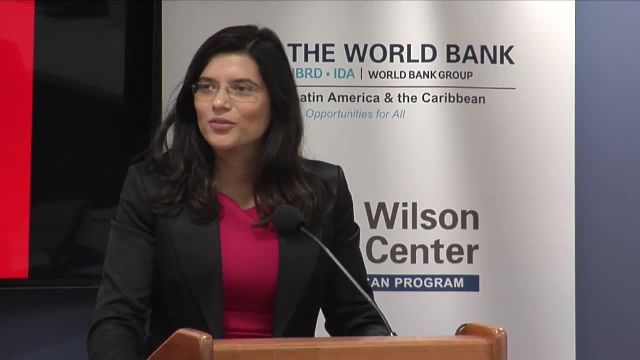 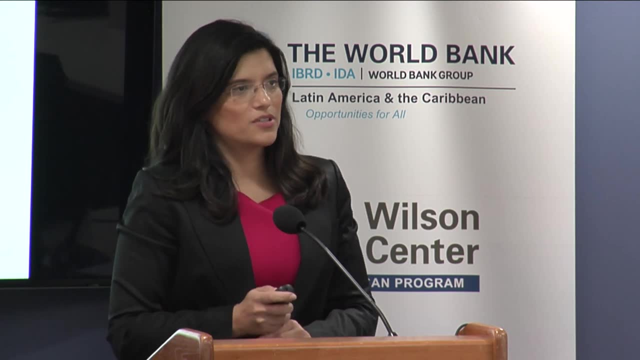 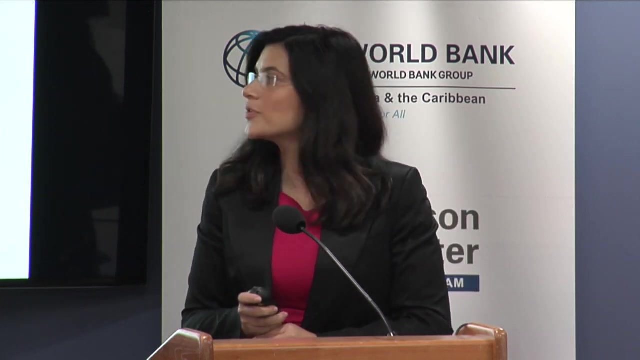 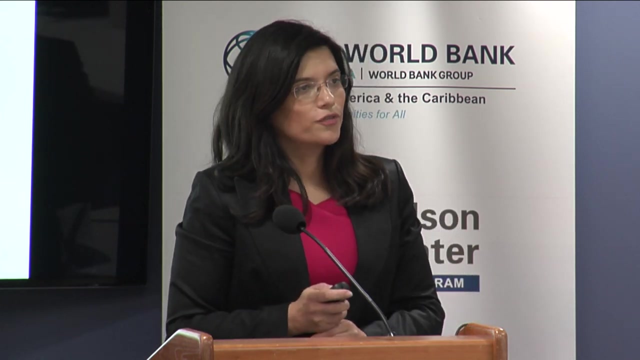 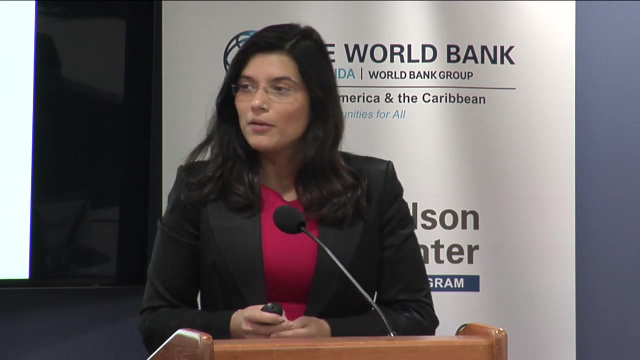 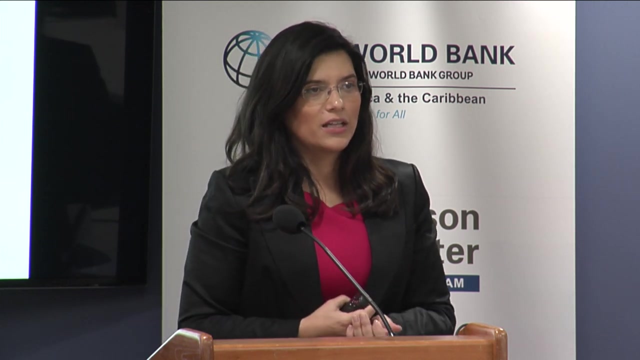 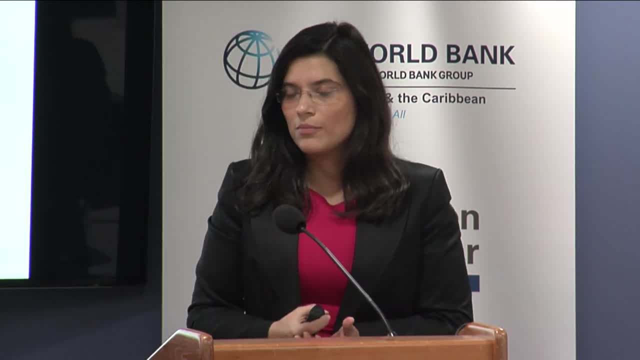 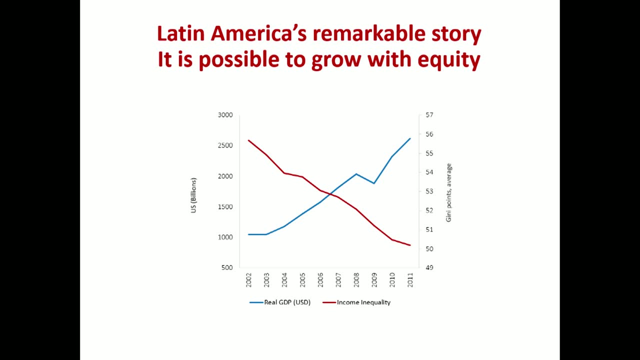 we are going to focus today. Not all income are wages. Wages are a part of the income And really this remarkable trend in income inequality was driven by what happened in the labor markets. what happened to wages? Wage differences across workers became more. 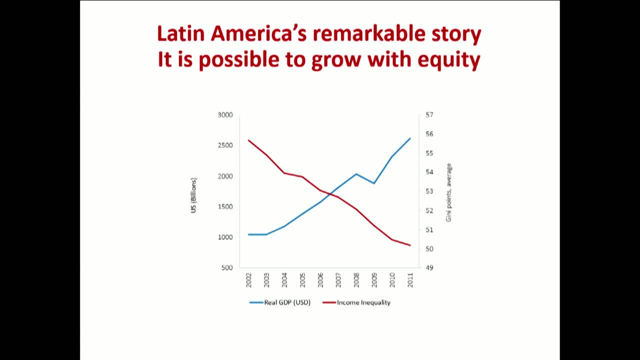 similar, and this was what drove the remarkable reduction in income inequality in Latin America. Let's now focus on three questions that this book tries to address: How did this happen, Why did this happen And what to expect now in this new context of lower growth? 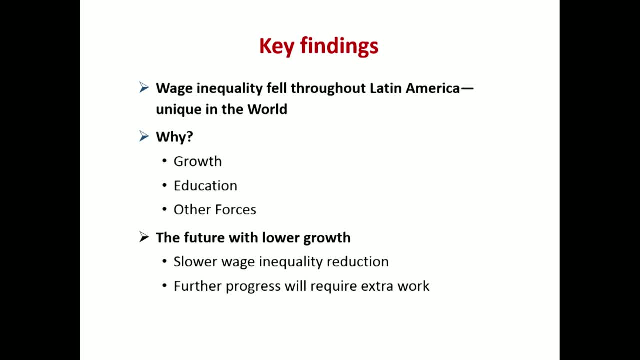 So let me give you a brief overview of the main findings of our book. First, we are going to show you that wage inequality fell significantly throughout the region, And this was in sharp contrast to what happened in the rest of the world where, in fact, most 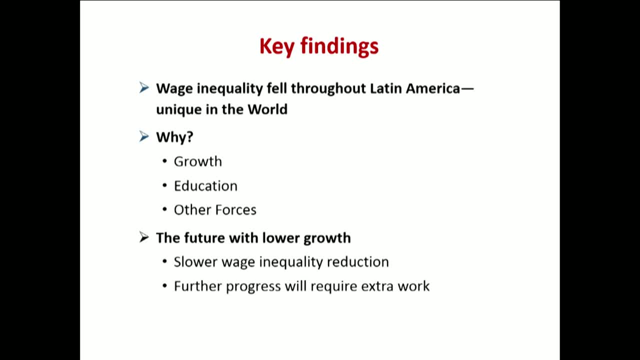 countries were struggling with rising wage inequality. This happened mainly for two key reasons: the expansion of education and economic growth- its pattern. There were also other factors that contributed to such a remarkable development, such as the minimum wage and the reduction in informality, And we are going to speak about those as well. but arguing, 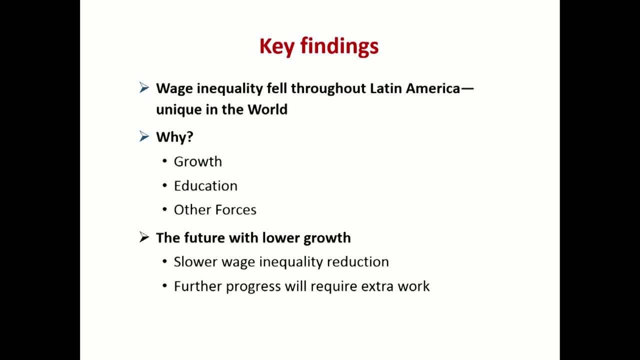 that they had a secondary role compared to gross and income. Thank you very much. Today, economic growth is in a new pattern, is in a new level. Since the mid-2011, growth has slowed down and this has slowed the reduction in wage inequality, but has not reversed it. 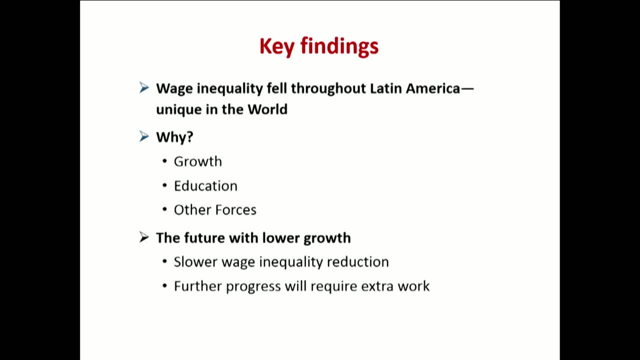 However, looking towards the future, this slower reduction now calls for action, and further progress will require extra work, And this book is going to talk about this, and I'm going to talk a bit about which type of policy actions could lead to continuing. 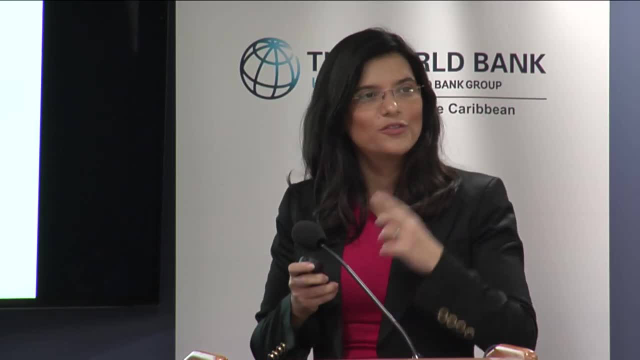 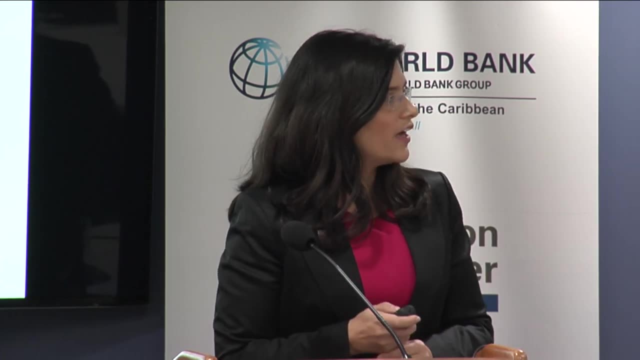 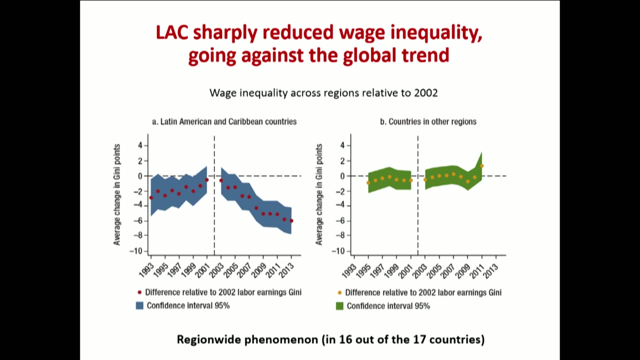 the large fall in wage inequality. So now let's dig into each of these aspects. So first let's look at the facts, at how wage inequality fell in Latin America. Here in this graph we have wage inequality in Latin America on the right since the 90s. 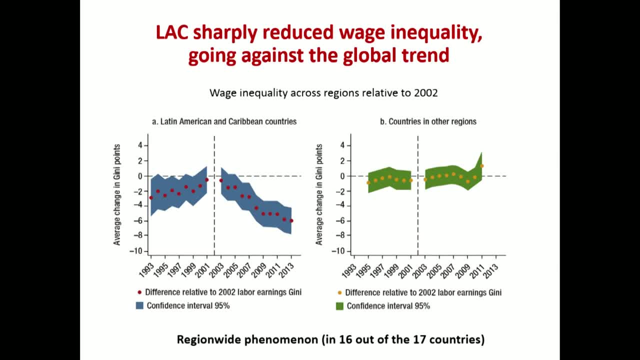 until today, and we are always comparing it with 2002,. this was the year where the trend changed. During the 90s, wage inequality was stagnant in increasing in Latin America, But then, after the early years of the new millennium, something changed and wage inequality 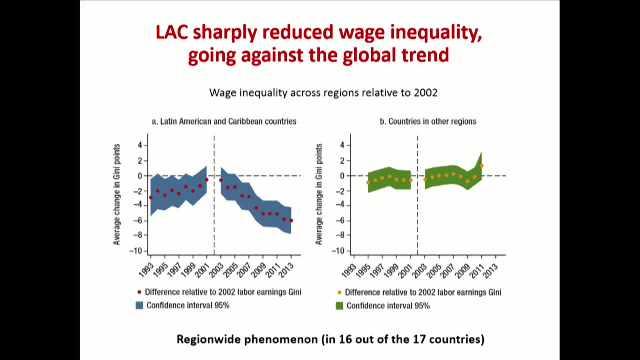 fell dramatically in the region. It fell by about 6 points. These are, for example, the difference today between countries in the cellOnline Splitoty, which although is the OECD, such as Germany, and countries in Latin America, such as Argentina. This was 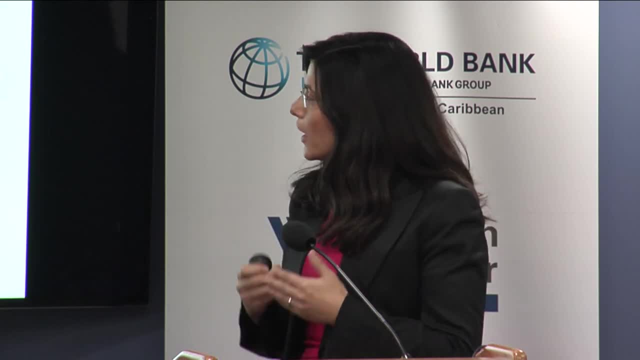 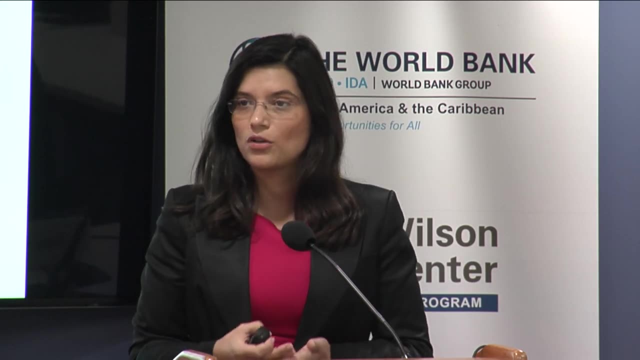 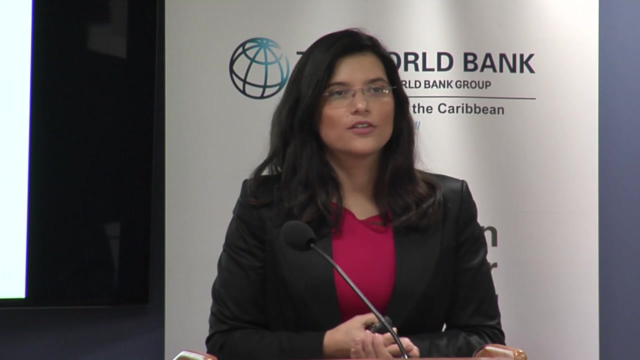 a large fall in wage inequality. This happened in 16 out of the 17 countries in Latin America. The only exception was really Costa Rica, so it was really a region-wide phenomenon. Moreover, it's in sharp contrast, as I told you, with the 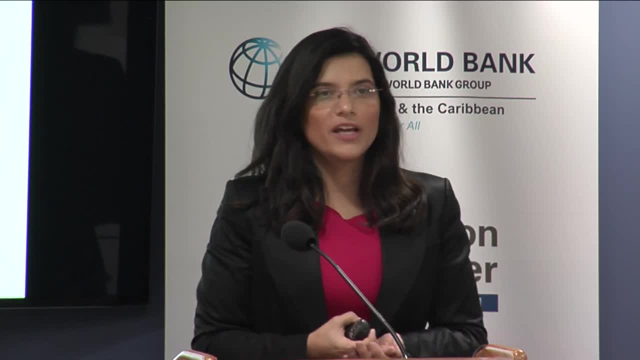 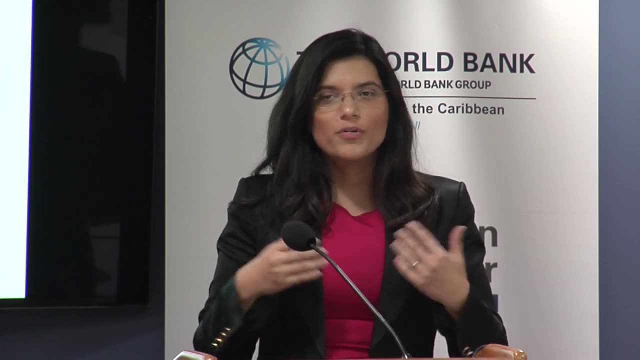 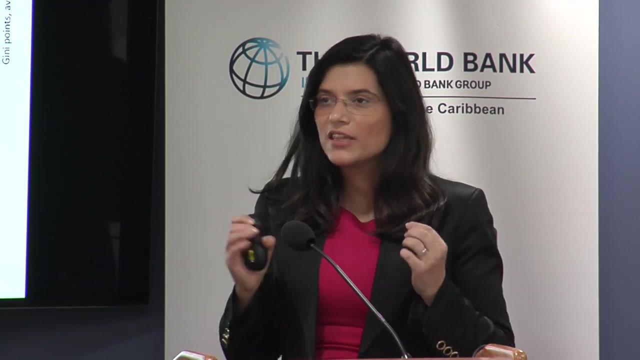 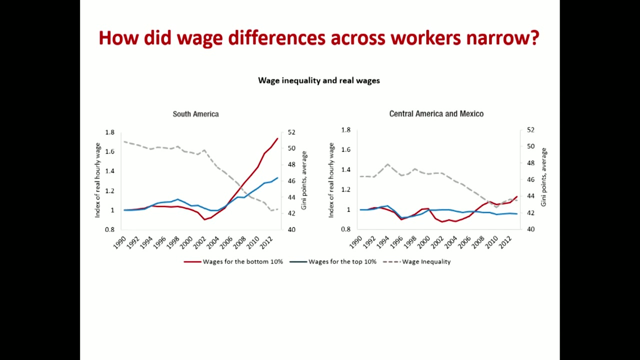 rest of the world, here in the graph on the left, where wage inequality was increasing. This was really something unprecedented and something very large. This phenomenon is what we study. So how did this reduction in differences in wages across workers in Latin America occur? Two important aspects: 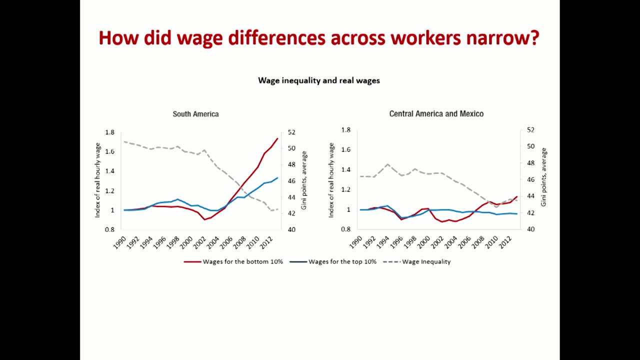 here depicted in these two graphs, of course, thank you. The first one is that in South America, where growth was stronger, the unemployment rate was much higher. The unemployment rate in Latin America was: the reduction in wage inequality was larger than in Mexico and Central America. 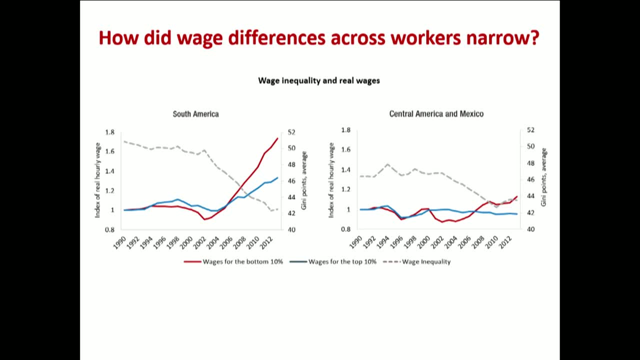 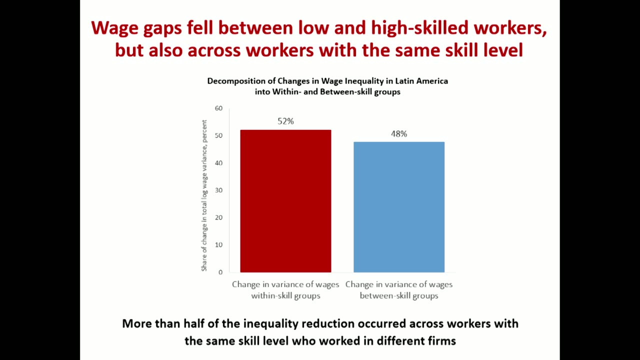 The second aspect was that wage difference fell because wages of the unskilled workers increased more than wages of the skilled workers. was a push from the bottom in both sub-regions, and this is very important. Another very important fact that this book analyzes. 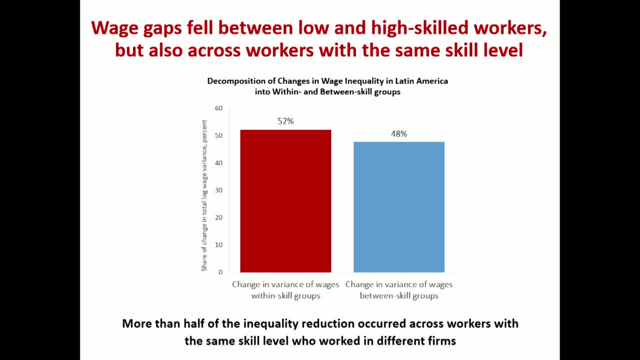 is that wage differences in economies can fall because skilled workers and unskilled workers get more equal pay, but also because workers of similar skills working at different firms get more equal pay. So we went ahead and did a decomposition of the change in wage inequality in the 2000s. 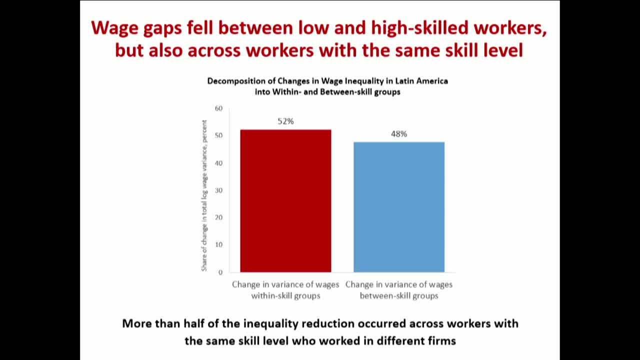 between these two components: the part that is due to differences in skills, in education, in experience, and the part that is due to workers with similar skills making now more similar wages. Here I'm speaking about the difference in wage between a manager at McKinsey and a manager at McDonald's. 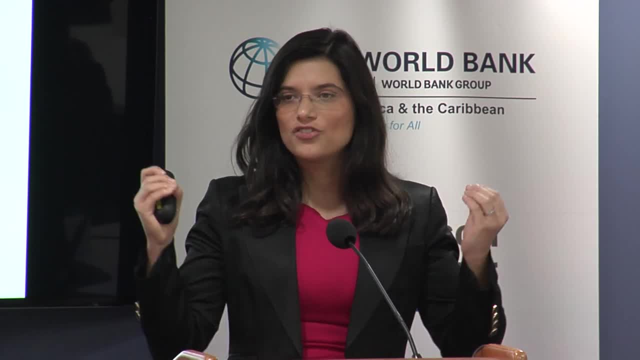 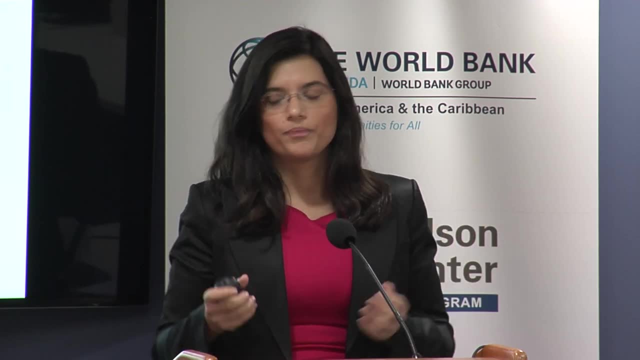 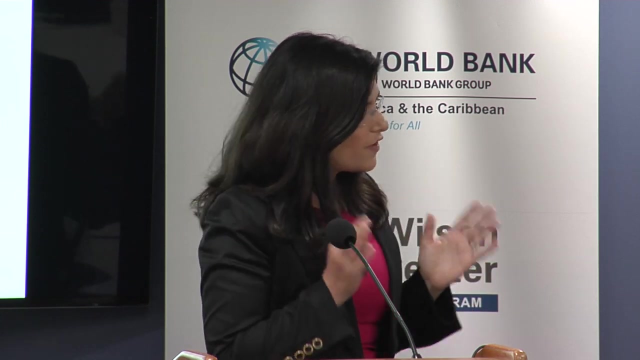 This difference also shrank in Latin America Wages and this happened mostly because wages across firms became more similar, less unequal, And this is a very important aspect for our study. So just to summarize in terms of facts the important reduction that occurred: 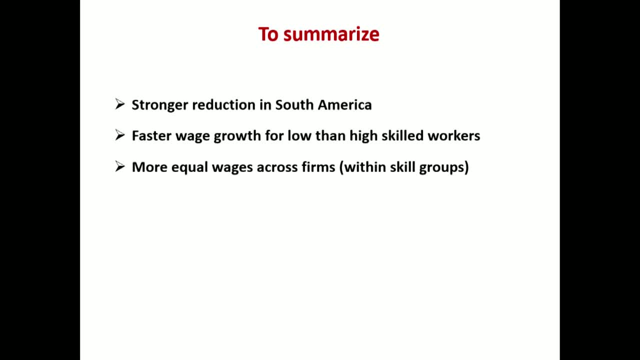 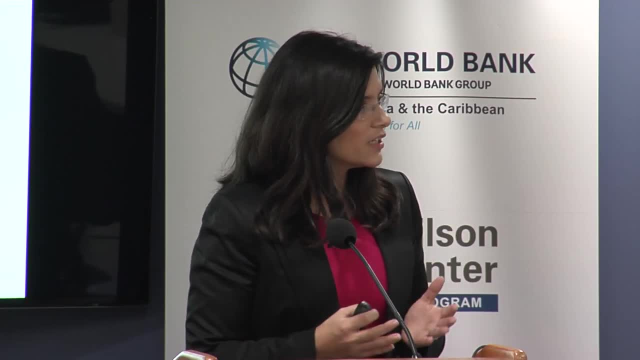 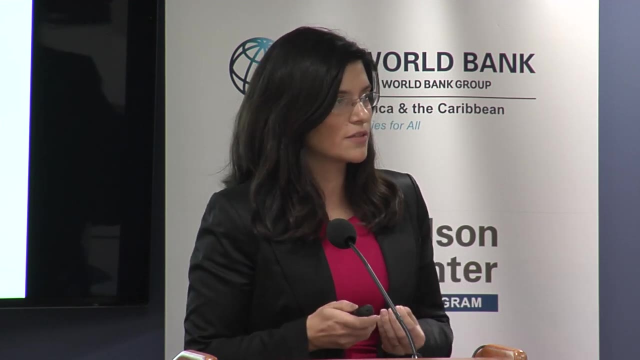 throughout the region, was stronger in South America than in Mexico and Central America, was pushed by the bottom wages of unskilled workers, increased more than wages of skilled workers, and was pushed by more equal wages across firms for similar workers. Let's now, with this in mind, 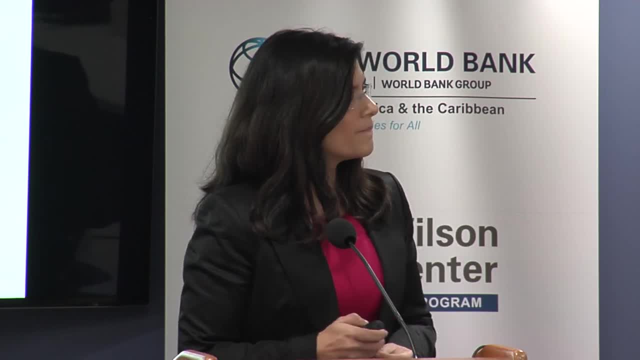 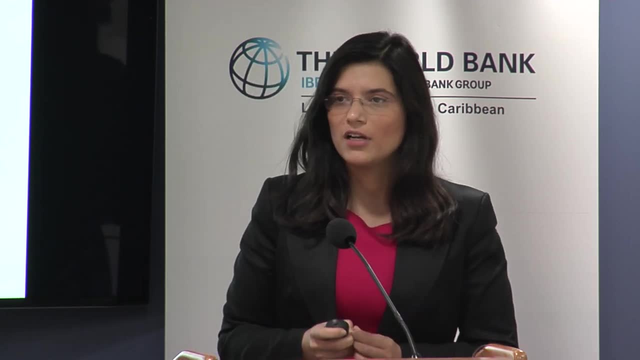 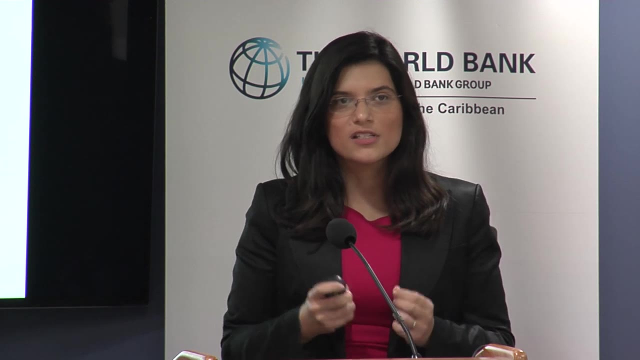 try to understand what drove this remarkable phenomenon. So what caused the reduction in wage inequality In Latin America in the 2000s? The first big driver was growth, And it wasn't just the level of growth. Inequality fell because the pattern of growth. 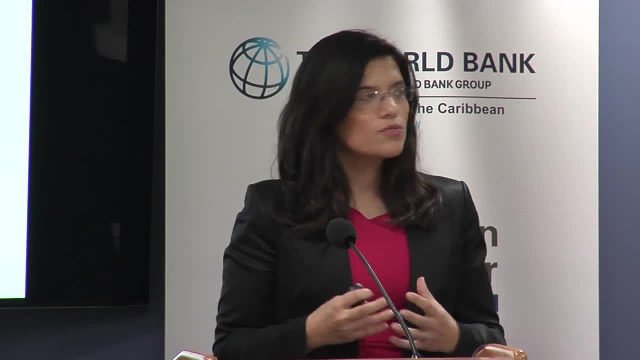 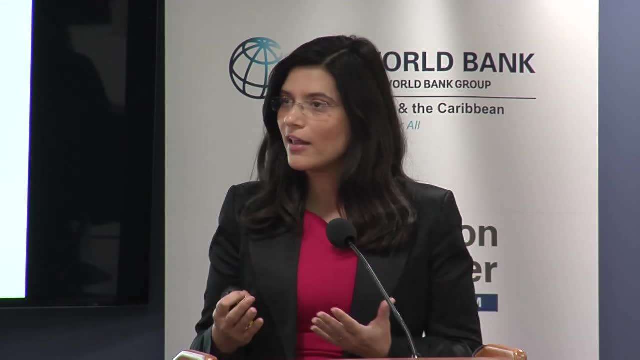 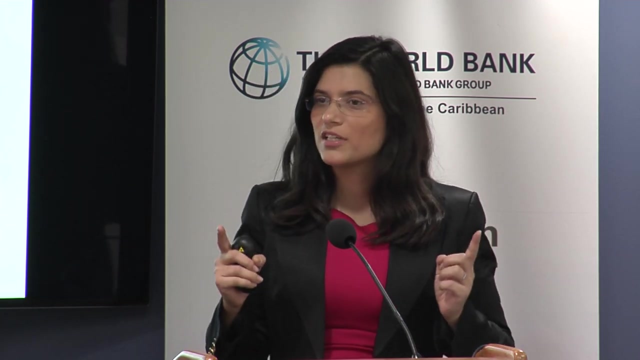 was different and was very important. Growth was associated with a real exchange rate appreciation. This was pushed by the commodity boom but also other factors, And these had a key role in one particular aspect: in wages of similar workers, in difference in wages across similar workers. 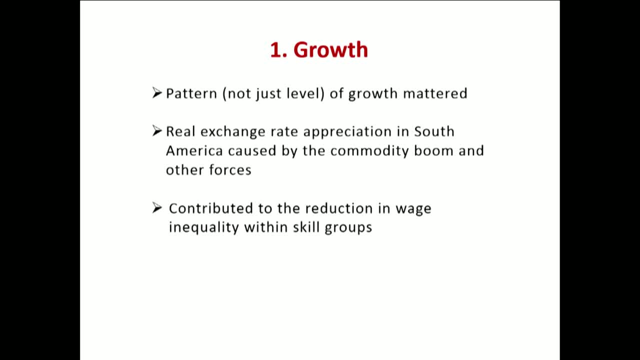 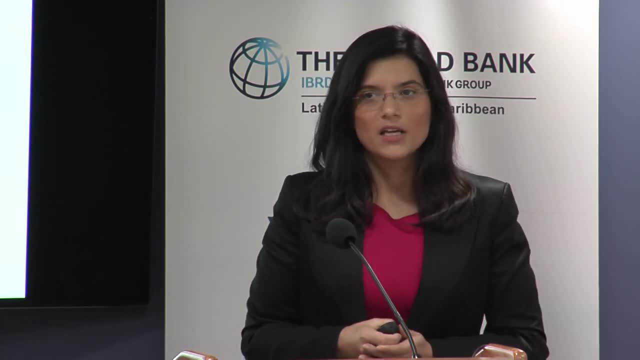 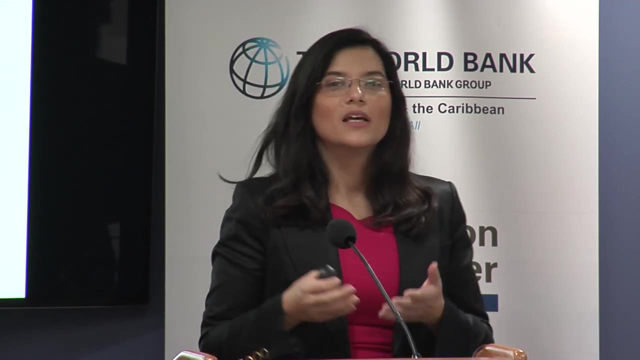 It reduced wage inequality because it reduced wage inequality within skilled groups across firms. So let me now dig into this. South America and Mexico and Central America had very different trends in terms of growth during the 2000s. In South America, labor market demand was more dynamic. 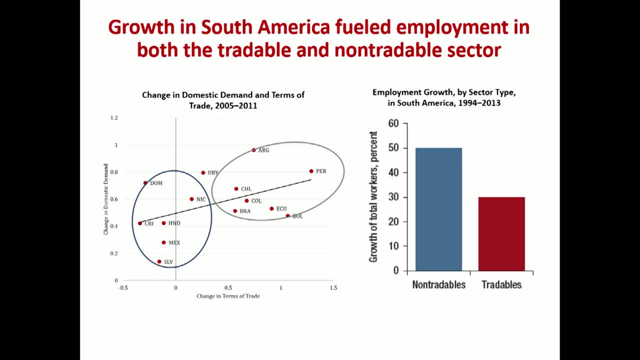 The region- the sub-region- grew at about 4.8%, Whereas Mexico and Central America grew at about 3.3%. The growth in demand was also accompanied by an improvement in terms of trade, fueled by the commodity boom, but also by capital inflows into the region. 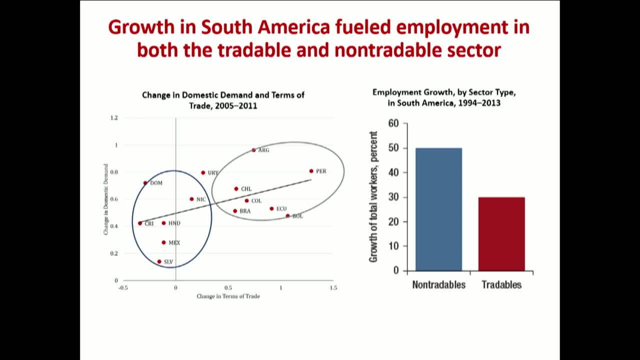 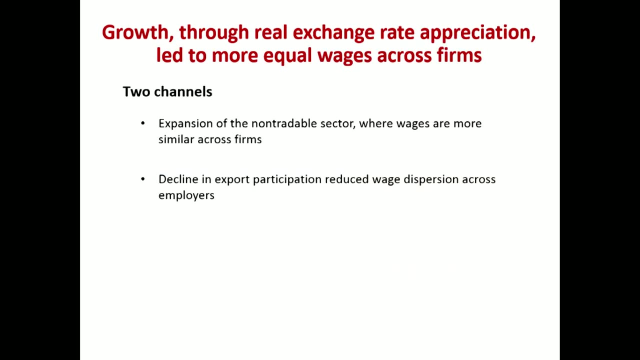 Through spending effects as money poured into the countries. no tradable sector employment expanded more than the tradable sector employment. So employment in sectors such as services expanded more than in manufacturing in the tradable sector And growth acted through the exchange rate appreciation on inequality. 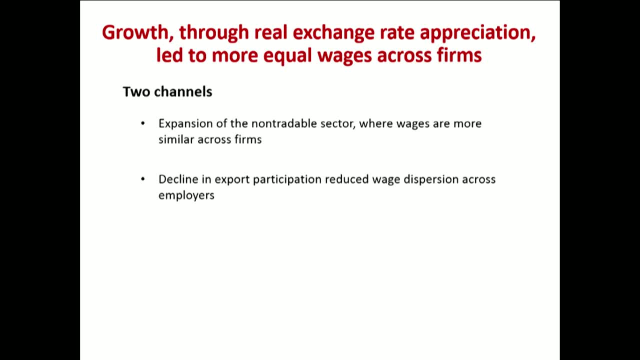 Let me tell you how, through its effect on the real exchange rate, appreciation growth led to more equal wages across firms. This occurred through two main channels. The first one, this expansion- the expansion that I just told you of the non-tradable sector, led to more equal wages. 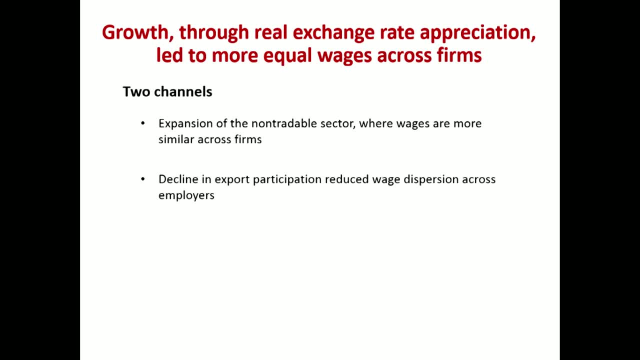 because wages across firms in the non-tradable sector are more similar than wages across firms in the tradable sector. Second, it reduced wages across firms- wage differences across firms- because it led to a decline in export participation Within the tradable sector and within an economy. the more productive firms, the higher the price, the more The high-paying firms are the exporting firms and by hurting labor demand for these firms and therefore employment, it makes wages within the tradable sector more similar. But there was a second factor. It wasn't just growth. The second factor was the remarkable expansion in access to education. 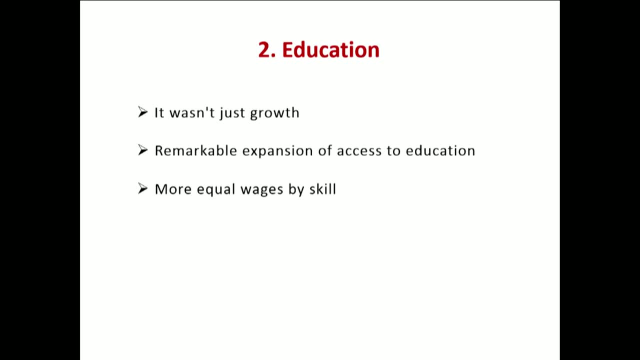 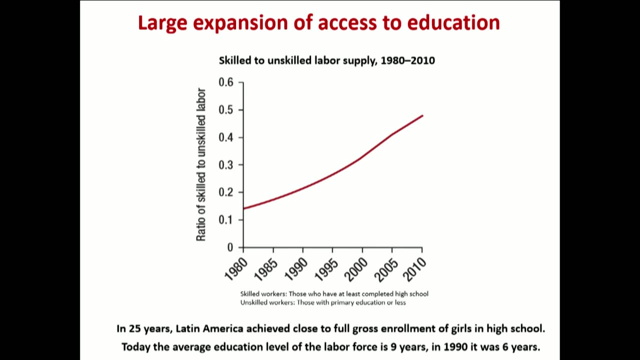 These reduced wages across skills made more equal wages across skills. The relative supply of skilled workers to unskilled workers, depicted in this graph, increased steadily and in a large scale since 1980.. This graph might not seem that striking, but let me tell you some facts. 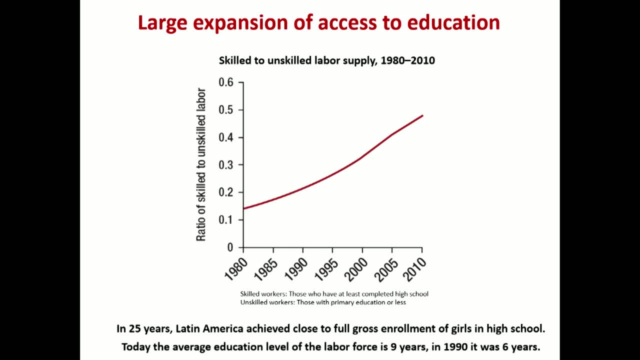 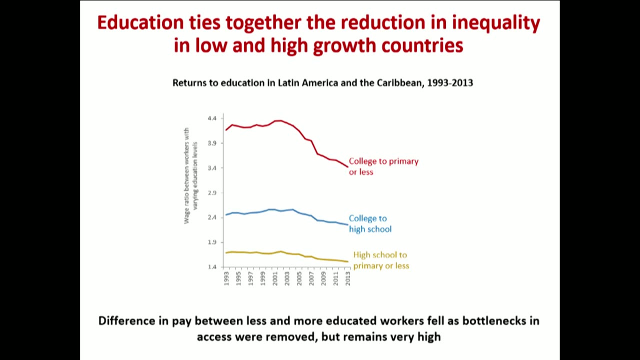 Today in Latin America most young girls are enrolled in high school. Today, The average level of education is nine years of education. In 1990, it was six years of education. This is a big improvement. Through this trend, unskilled workers became a relatively scarce resource as more skilled workers entered the labor market. 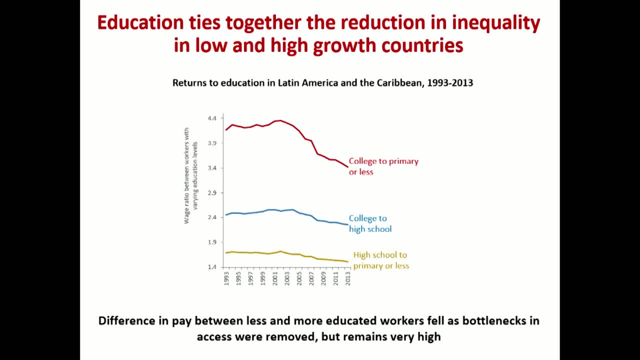 And this throughout the region, affects the gap in wages between skilled and unskilled workers. The college premium, The difference in wage between college-educated workers and primary-educated workers, fell, but fell from a high level. It remains very high And it fell as bottlenecks were removed in access. 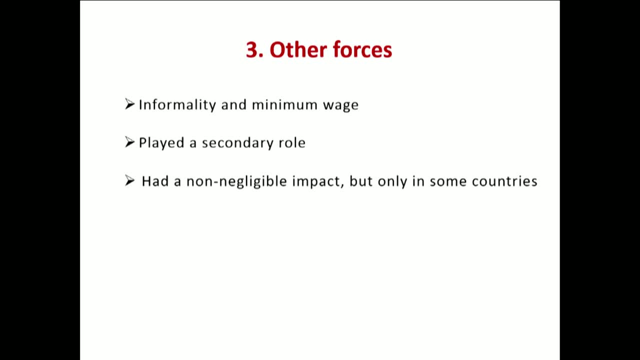 So, now that we have a complete picture, one factor that reduces wage differences across firms- growth- And one factor that reduces wage difference across skills: education. Let's now look at this. Let's now look at other factors, other forces that happen at the same time in the region. 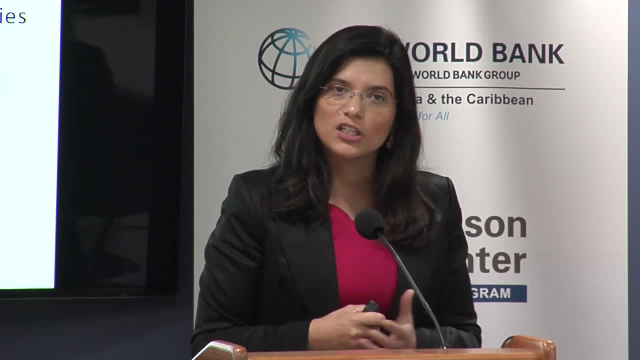 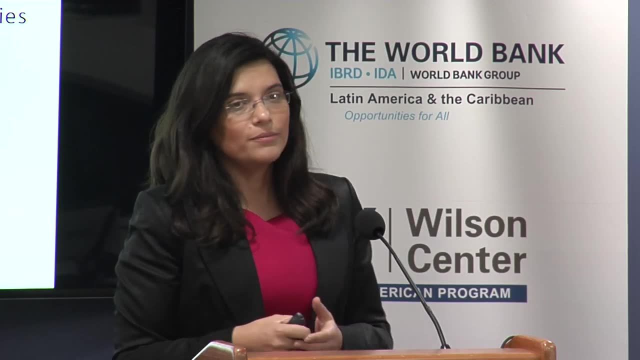 At the same time, in some countries in the region, there was a big reduction in informality and big hikes of the minimum wage. This played a secondary role And they had some impact, but not in every country. Let me give you more details. 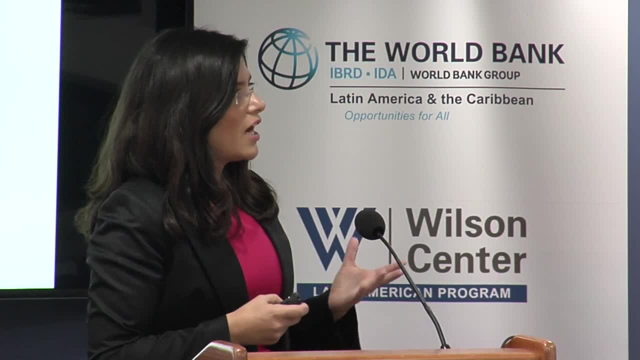 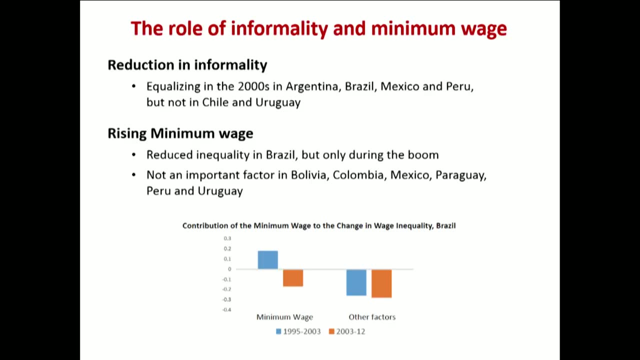 In several countries in the 2000s, for example, in Argentina, Brazil, Mexico and Peru. the reduction of informality reduced wage inequality because those who entered the formal markets, the formal employment, were the low-skilled workers. However, the reduction on informality did not have a strong impact on inequality in countries like Chile or Uruguay. 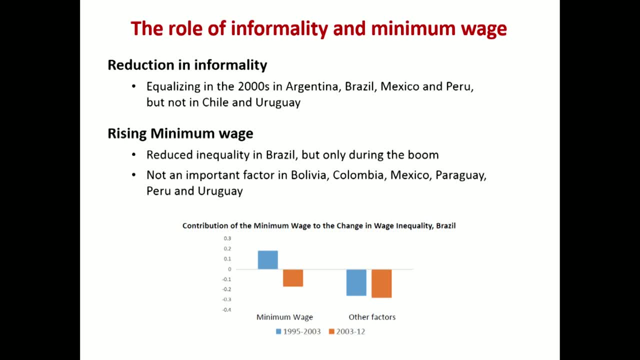 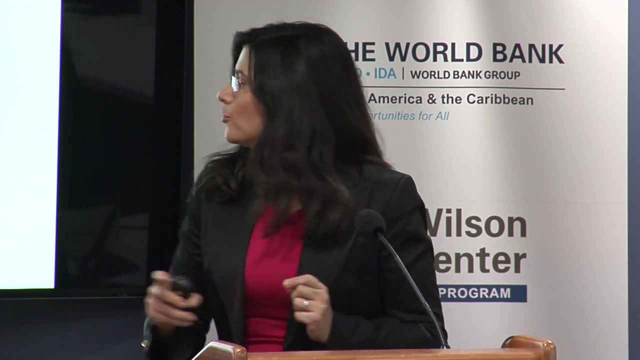 Let's now turn to the minimum wage. The minimum wage increased significantly in many countries. Brazil was certainly a case where this happened And in the 2000s, when minimum wage increased in Brazil, it reduced inequality by about 20%. However, during the previous period, during the period 1995 to 2003,, where growth was lower, 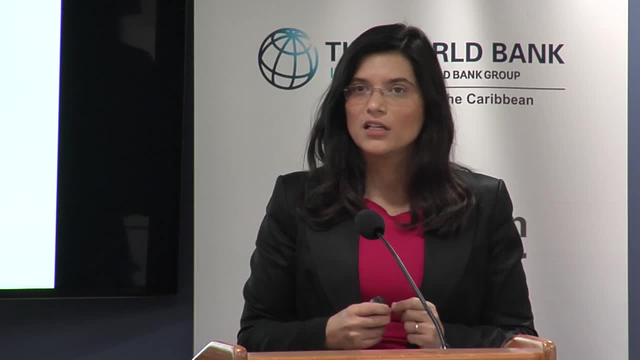 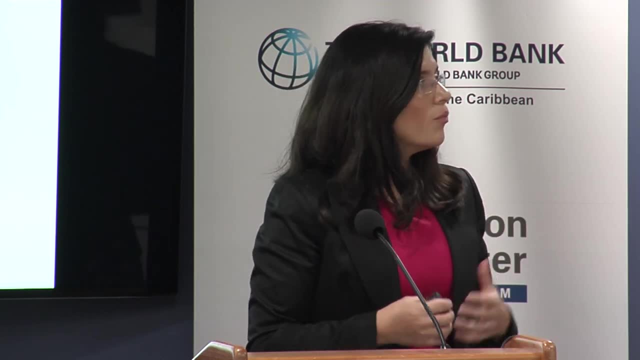 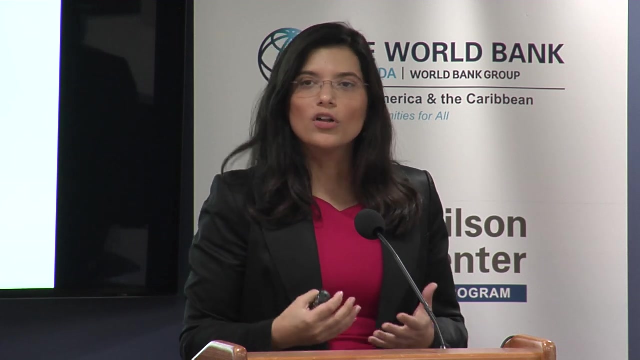 in fact, minimum wage hikes in Brazil increased wage inequality, So, really, when it happened, it was very important. Moreover, in other countries, such as Peru, such as Uruguay, such as Mexico, the role of the minimum wage is not as important. 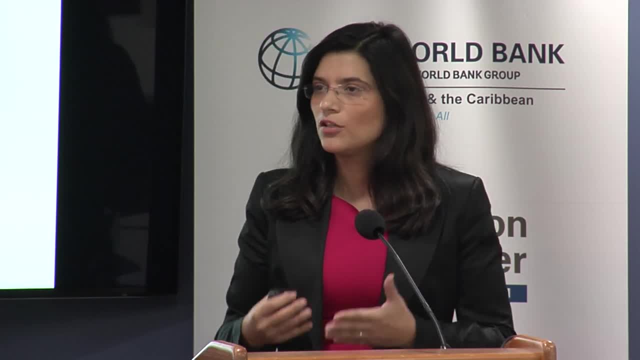 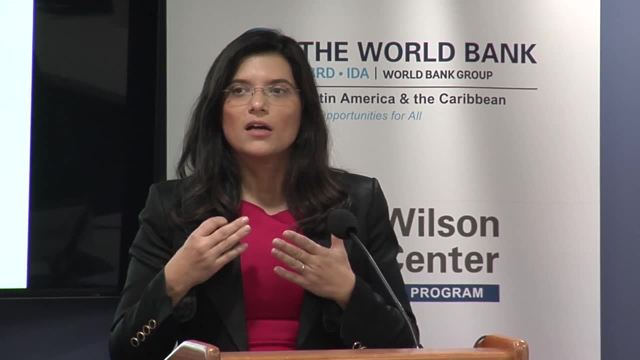 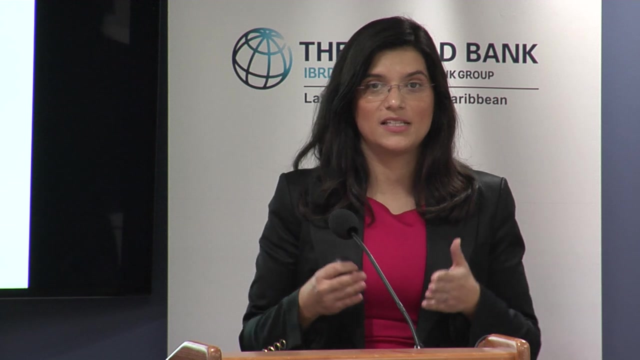 Either because it is too low to matter or because it didn't increase during this decade. So just to summarize, the key drivers of the wage inequality reduction in Latin America were, economically: economic growth, not just level but its pattern- better education. 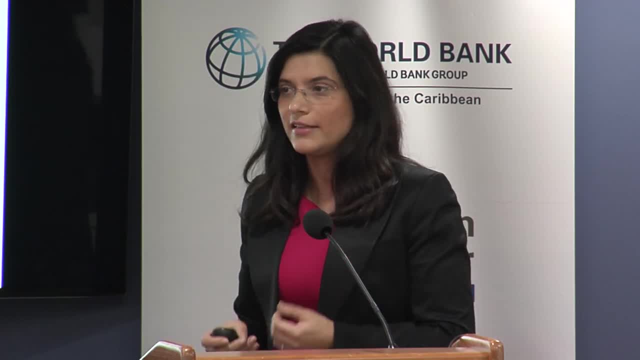 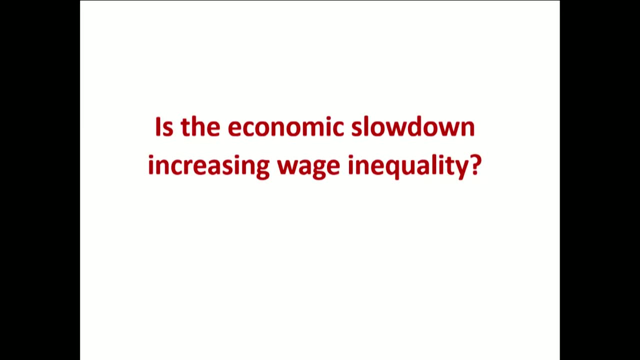 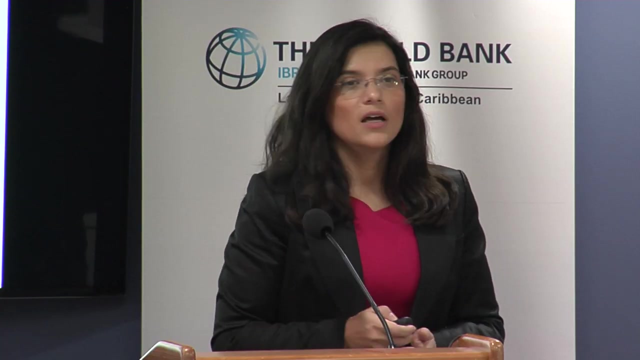 and then there were other factors, such as the minimum wage and the reduction on informality. that helped, but just in some countries. Now, a quick question today is whether the economic slowdown since the mid-2011 is indeed rising wage inequality. 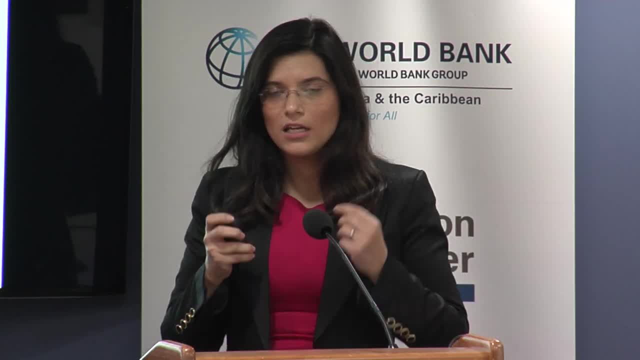 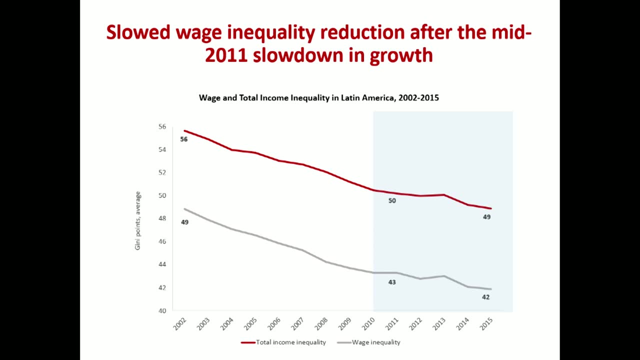 This is not the case. Economic slowdown: inequality continues to fall since 2011,, but it falls at a slower pace. So the slower growth came with a slower pace of reduction of wage inequality in Latin America, as we can see here in this graph. 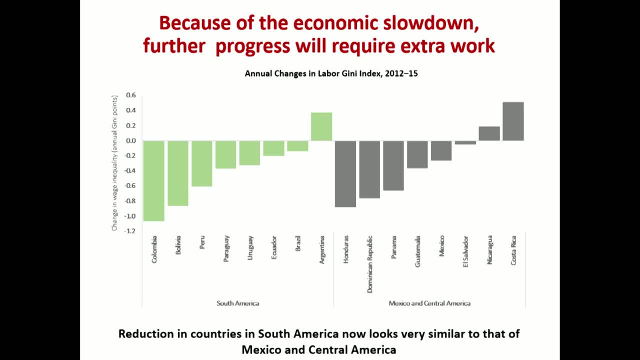 And this happened as countries in South America became more similar to countries in Mexico and Central America in terms of their reduction in wage inequality. Here in this graph, we depict the pattern of change of wage inequality in South American countries and in Mexico and Central America within the region. 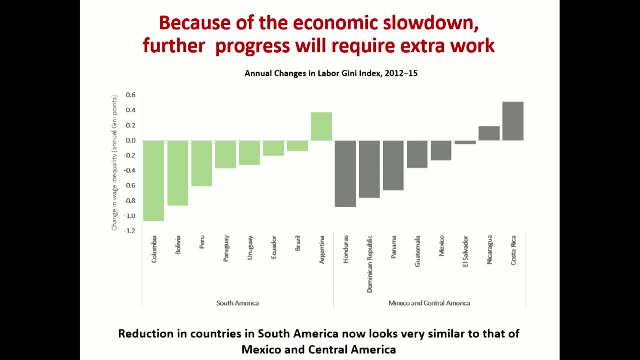 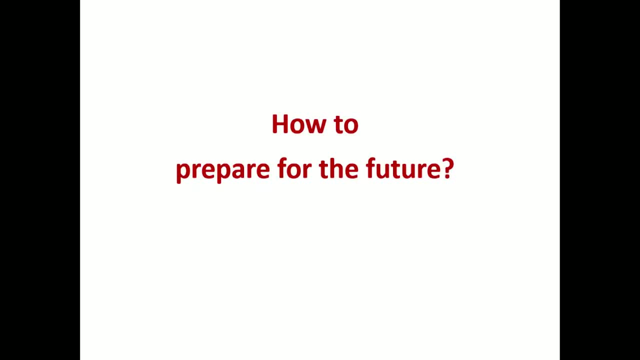 and you see that now they look very much alike. This wasn't the case of the 2000s, when in South America, wage inequality fell much more. So how to prepare for the future? Let's pause for a moment and think about. 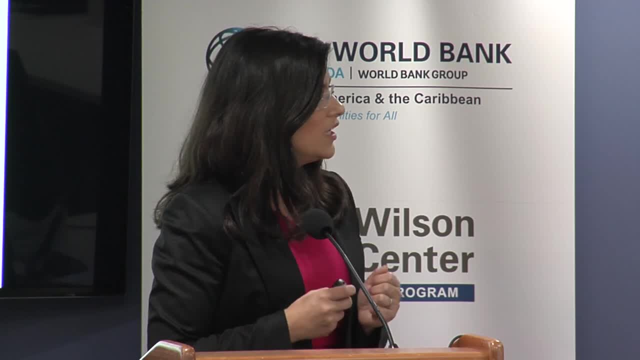 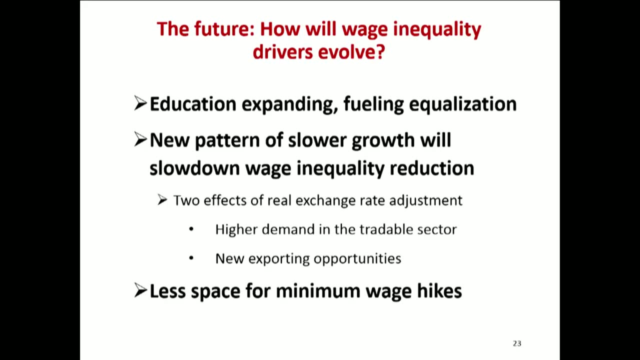 what is happening to the key drivers of this phenomenon today? On the one hand, education is continuing to expand, The levels of education remain below those that the region would desire and education is likely to continue to fall through lower returns to education, more wage inequality. 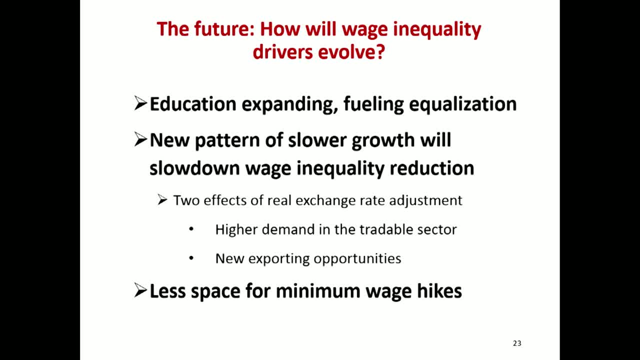 However, growth has slowed down and there is a new pattern of growth And this might affect wage inequality reduction. It might, in fact, slow this wage inequality reduction And this happens mainly through two channels in this framework of our book. The first one: 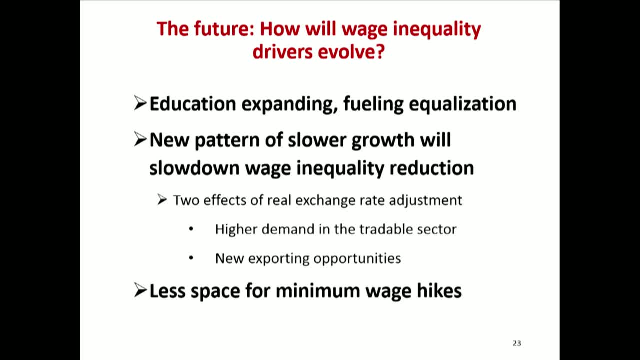 because it fuels the demand in the tradable sector that is more heterogeneous. The second one because it will promote exporting and by a higher concentration in high growth, in high productivity, high paying firms, the wage dispersion in the economy is likely to increase. 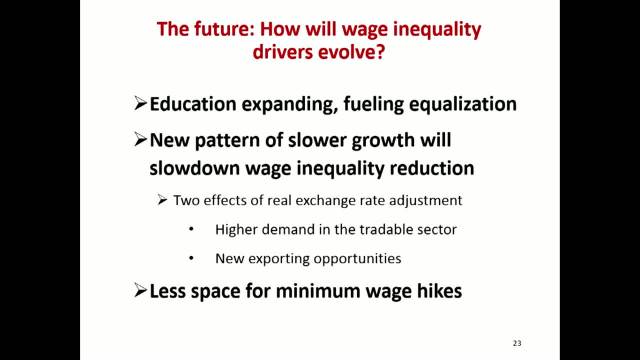 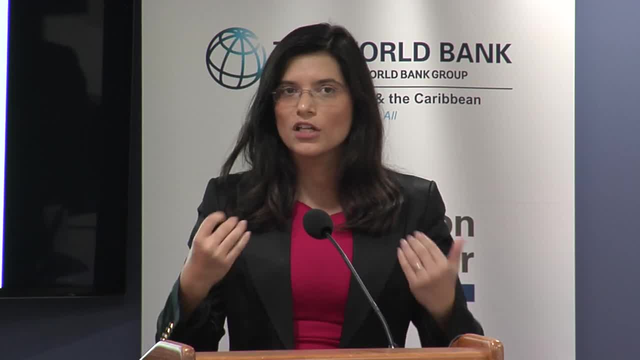 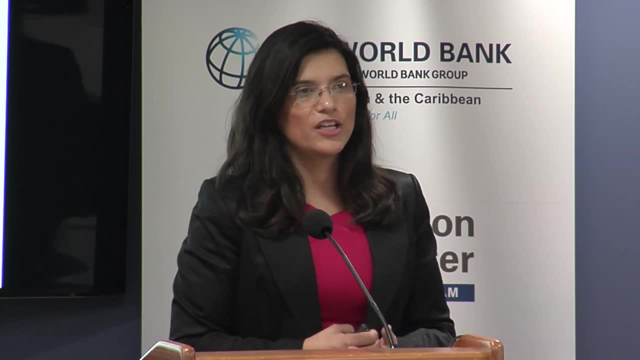 And also because just the act of exporting in a firm increases the skill utilization of that firm. Workers for marketing, workers with knowledge of foreign languages, are important for exporting, and the demand for this type of workers and the respective wage premium is likely to increase as a consequence. 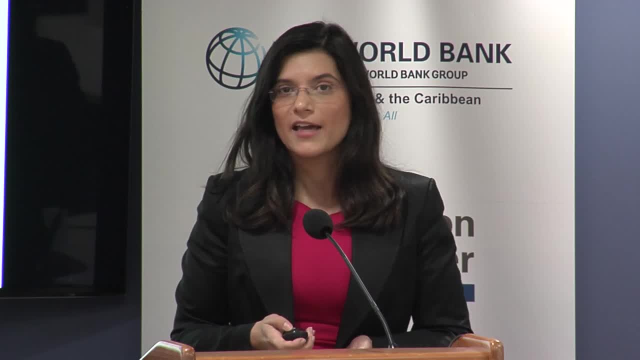 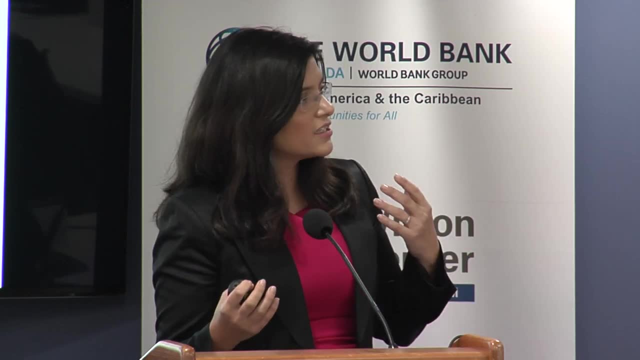 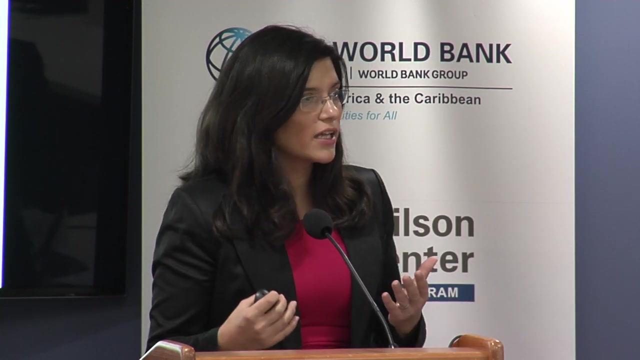 Today there is less space for minimum wage hikes, Whereas, as I just told you, minimum wage changes have different effects in good and bad times, And in fact, in bad times they can have unintended consequences, increasing wage inequality, as firms might not be able to hire workers. 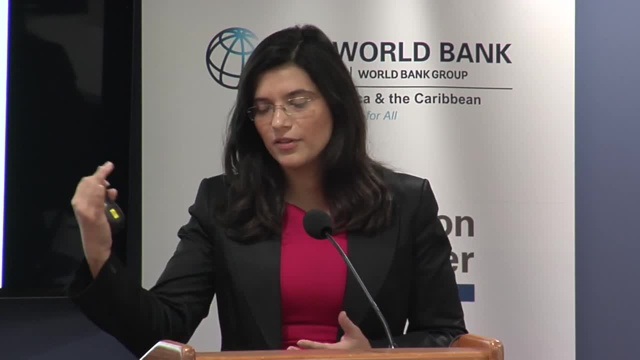 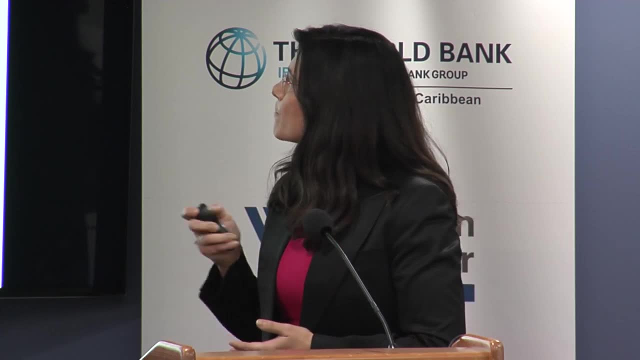 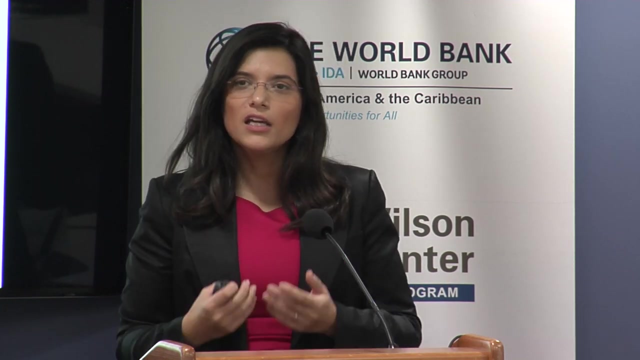 at a higher wage and many might have to be driven to informality or not getting the job. So how to move towards continuing growth with equity? Here in this book we argue for a two-pillar approach, and both are very important. 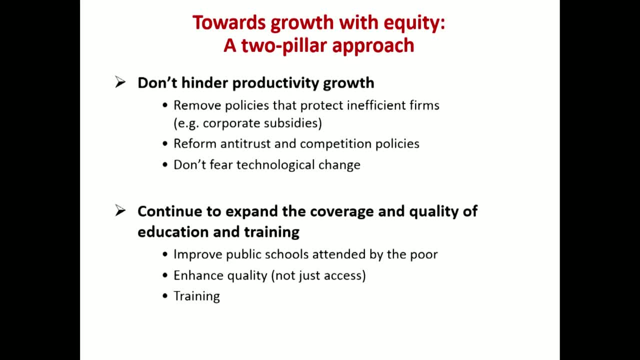 First we say: don't hinder productivity growth. This reallocation that we just told you from less productive to more productive firms improves productivity and has long-lasting effects. So let's embrace it. The first step is to increase productivity. 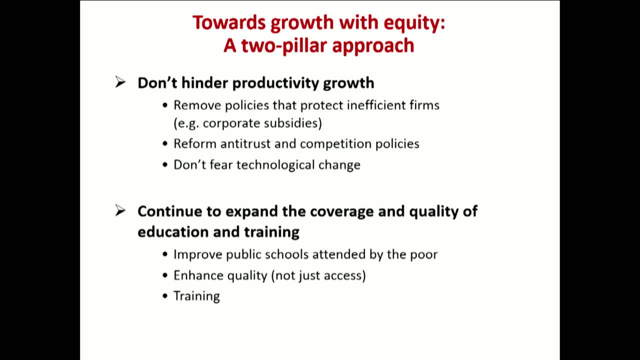 The second step is to increase productivity. This can be achieved by removing policies, for example, that protect inefficient firms. This is the case, for example, of considering reforms of corporate subsidies. It's also important to let more productive firms flourish through better antitrust and competition policies. 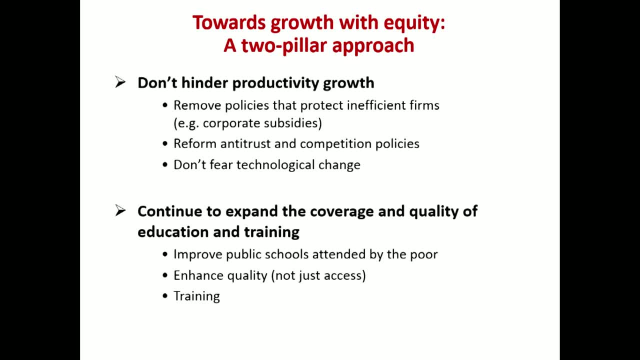 And don't fear technological change. This can have very good effects on productivity and growth, But be aware this can increase wage inequality. So don't do just that. Do more than that. Continue to expand education, But not just access to education. 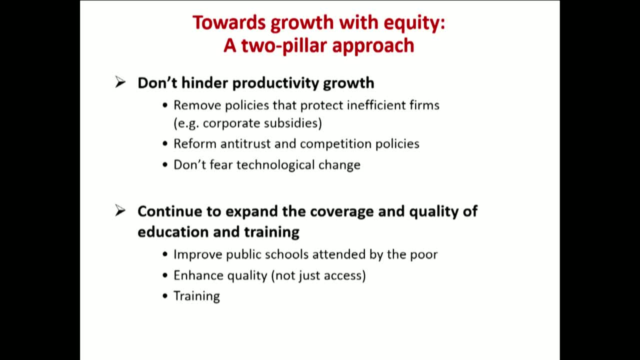 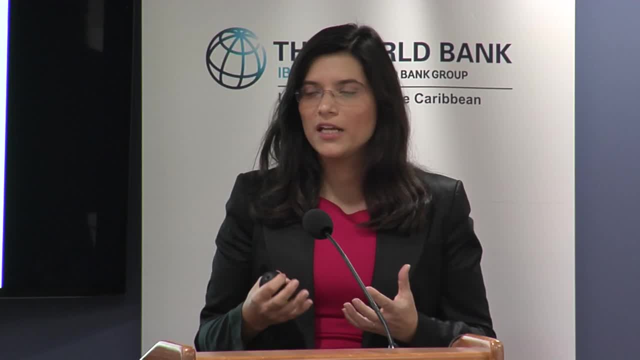 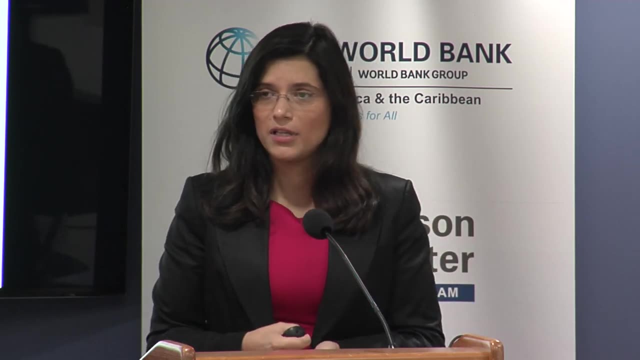 also the quality Focus on the public schools attended by the poor, Focus on training for disadvantaged youth. All these will bring skills up for the population and will lead to more inclusive growth. So, yes, growth is slowing down, But we don't need to be passive observers. 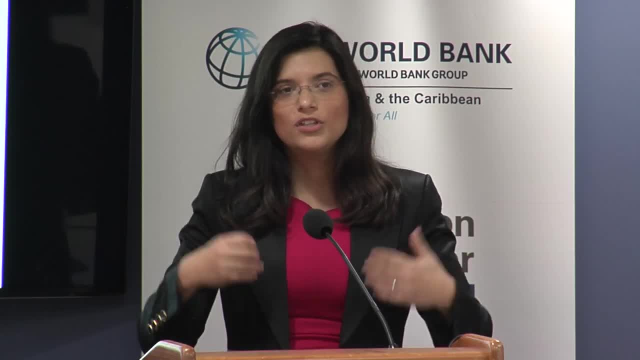 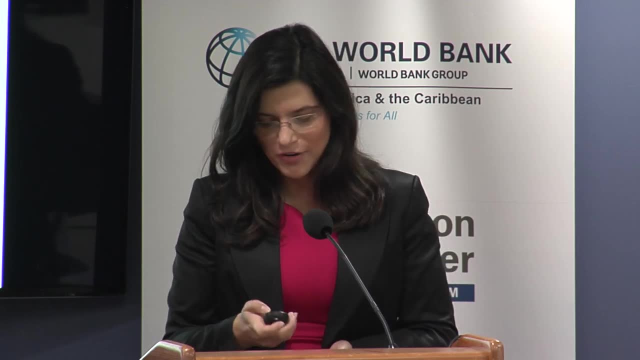 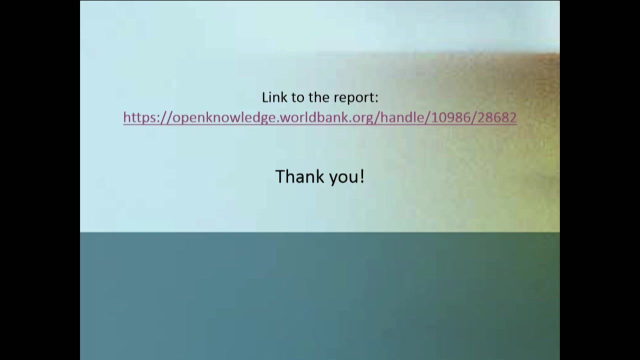 We can do concrete action and, through this, continue the progress of the 2000s with lower wage inequality and higher welfare in the region. Thank you very much And here is the link to our report, Thank you. Thank you, Joana. 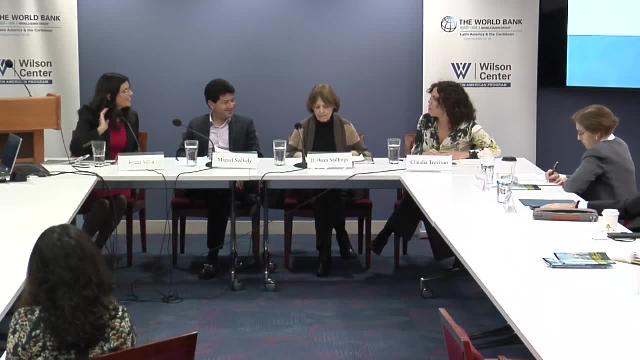 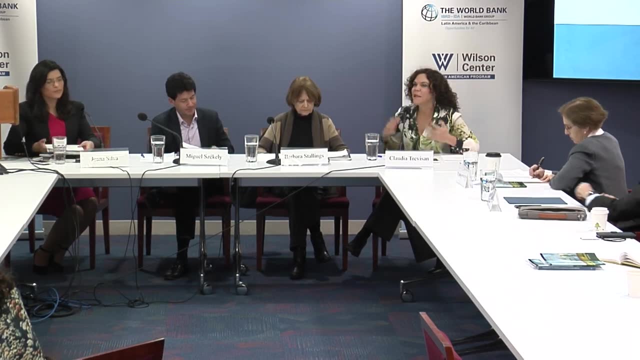 Well, we are going to start our discussion here, And I think we can do it in the more informal way possible. I think we can have kind of a conversation And start with education. That seems to be one of the keys, or the key issue. 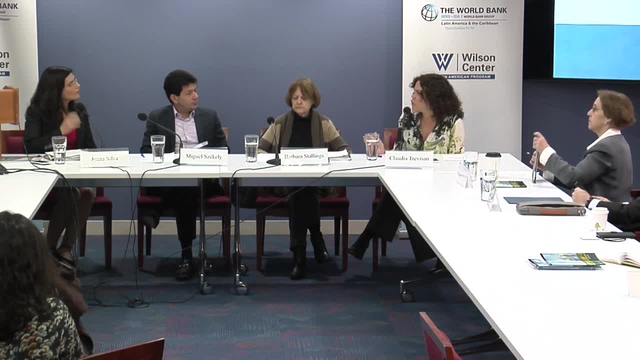 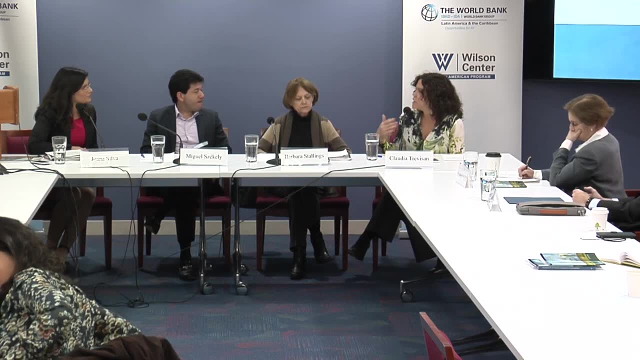 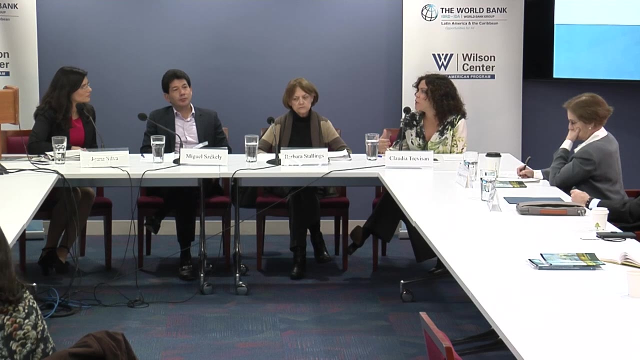 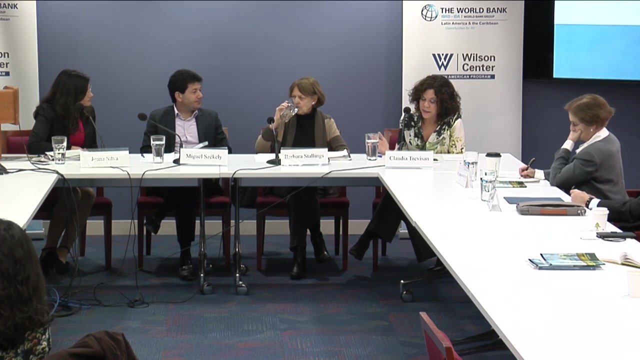 the key driver for reduction in wage inequality And, according to OECD data, countries like Mexico, Brazil, Argentina, Costa Rica already use a significant share of their public expenditure in education. In the case of Mexico, where Miguel comes from, the share is, according to OECD: 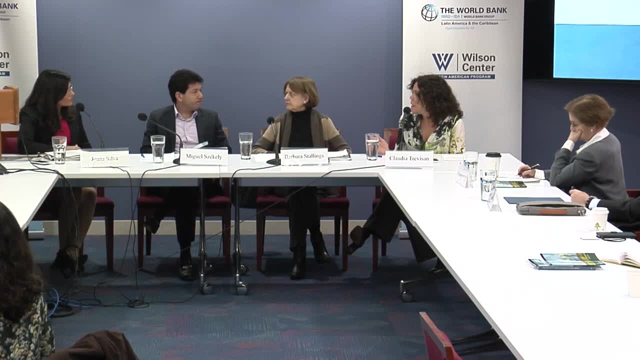 the share is of 17.3%- Roughly the double of France and Japan, And in spite of that, our students have one of the worst performances at PISA tests. So what are we doing wrong? I think you could start. 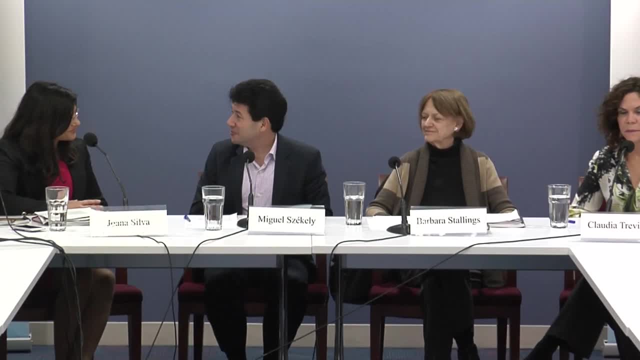 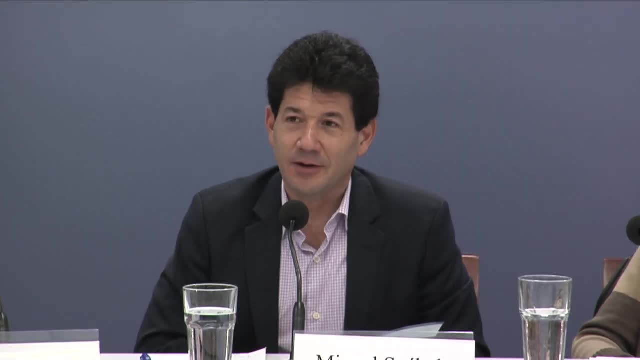 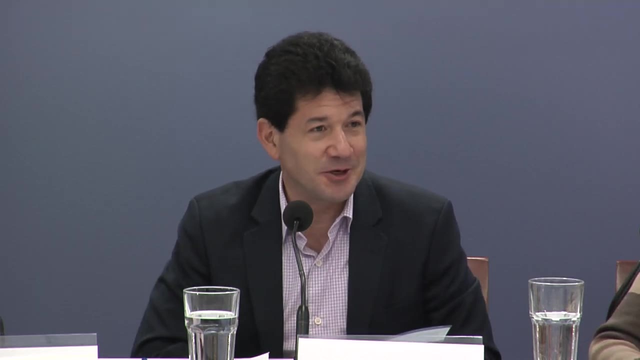 Well, thank you very much. Good morning to all And congratulations to the authors of the book. I recently participated in another event presenting another book by Julian, So congratulations for being so productive. That one was on education, actually, And I think this is certainly an important question. 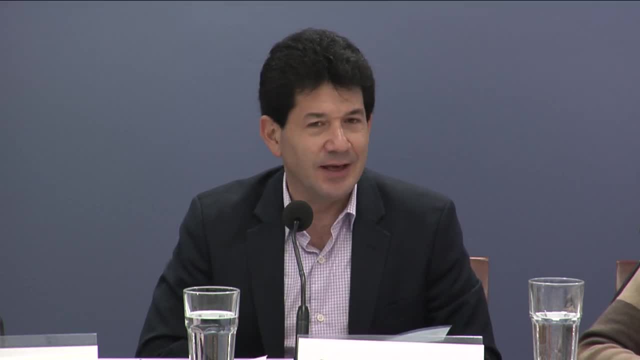 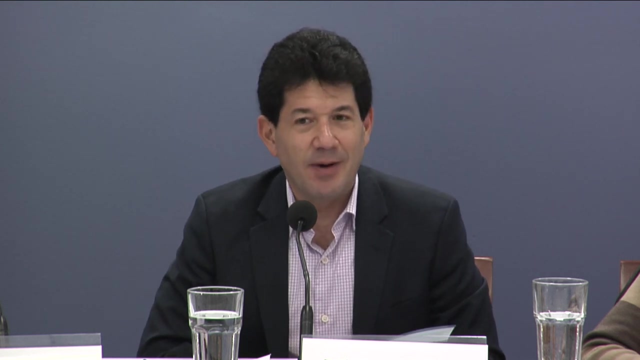 but before answering directly, I think it is important to take a step back And before just saying everything is all of this is about education. I think that there is still some discussion about the relative weight of education in the story. I have no doubt that it's certainly important. 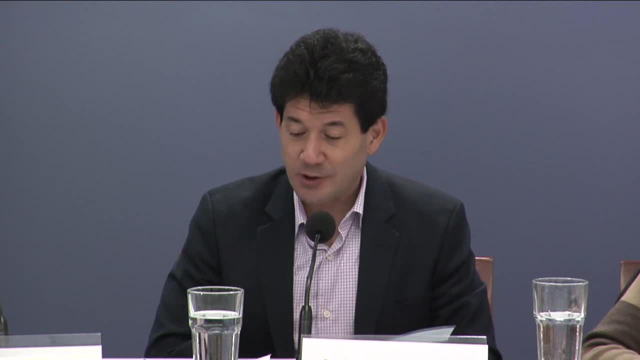 But many of us, but many of the facts- and the book actually talks about this- and many of the facts can also be explained with a hypothesis where more weight is given to the external sector factor and, in particular, to the role played by the prices of primary goods. 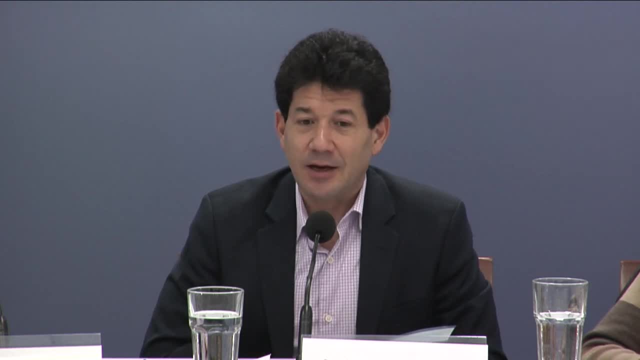 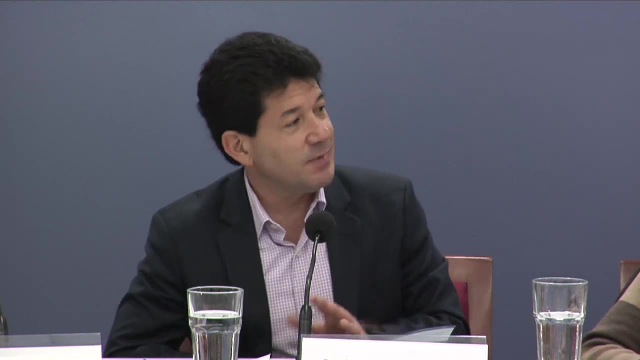 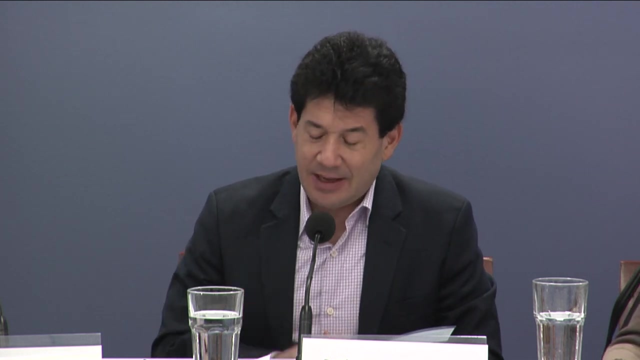 which are basically determined in world markets and which, again, the book definitely acknowledges. But I think we should not dismiss that side of the story. It's that side of the story from the outset. And well, actually, when I worked in the IDB several years ago, 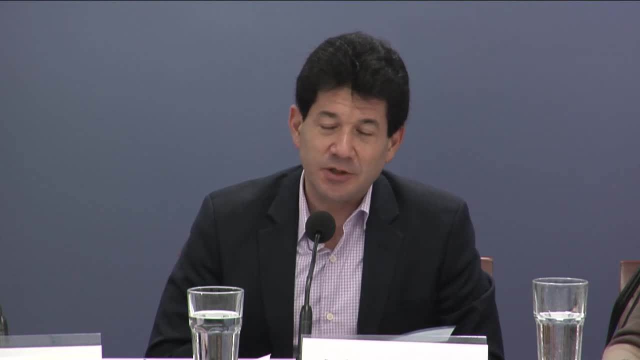 I started there in 1997.. And the reason I was invited to go to the IDB was actually because for the first time, the bank was doing a report on inequality. It was basically the Latin America discussion was much more of macro. macro issues were very, very relevant at the moment. 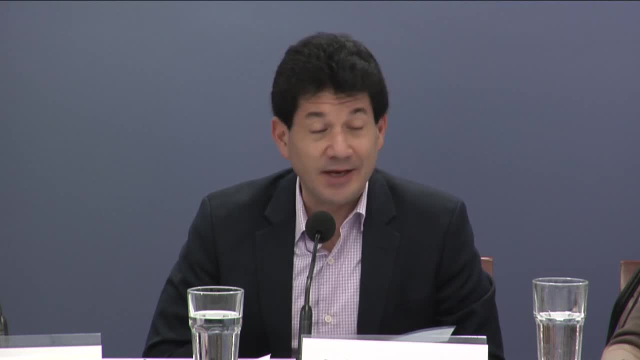 And when we started analyzing inequality around 1997, 20 years ago- 20 years ago, Yeah, The main issue was that Latin America was the most unequal region in the world and that inequality seemed like a fatal destiny for the region. 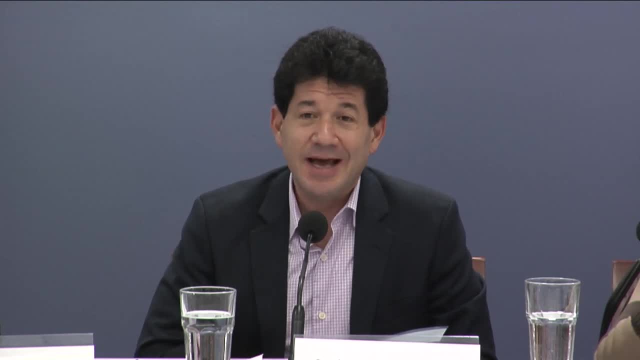 There was nothing to do about it. That's the way it was, And looking at the story today is very surprising. starting from that point, Of course also, I think we should calibrate this reduction. It's more or less a 10% reduction in the Gini coefficient. 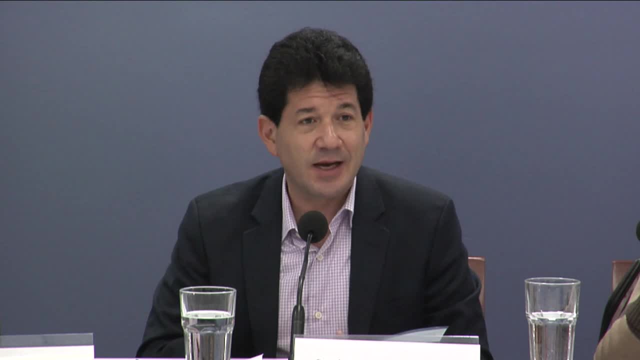 which is very significant, but it doesn't mean that inequality in Latin America doesn't exist anymore, that now we can compare to OECD countries or things like that, But it is a significant reduction. So the main question here in terms of policy is: 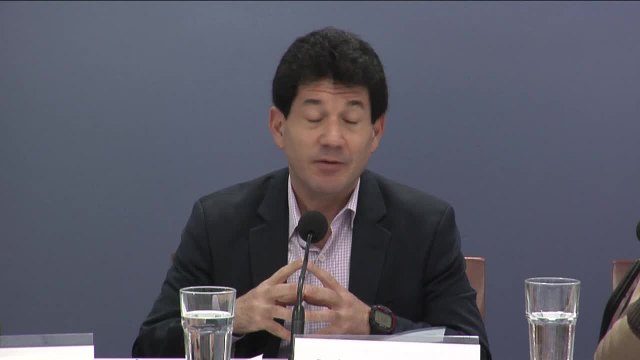 if it is a structural change, for example through education, that led to this improvement, okay, let's just keep on doing what we've been doing right and perhaps the inequality reduction might slow down, but it will continue. That would be the hypothesis under the structural explanation. 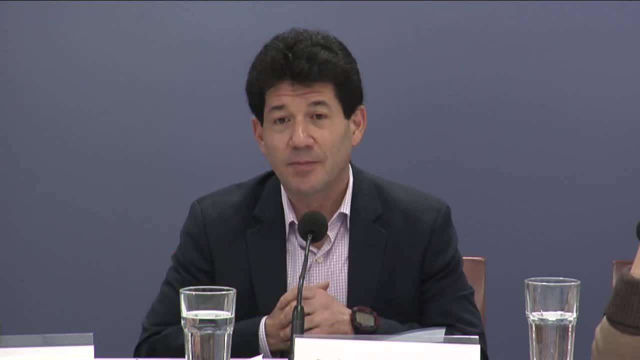 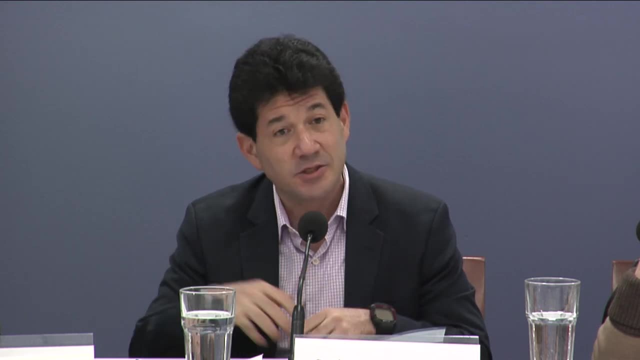 But if it is more of a temporary phenomenon, for example because of the role of the external sector and, in particular, the prices of some goods that are produced in Latin America, and suddenly had a boom, but that boom which does not depend on the policies in the region. 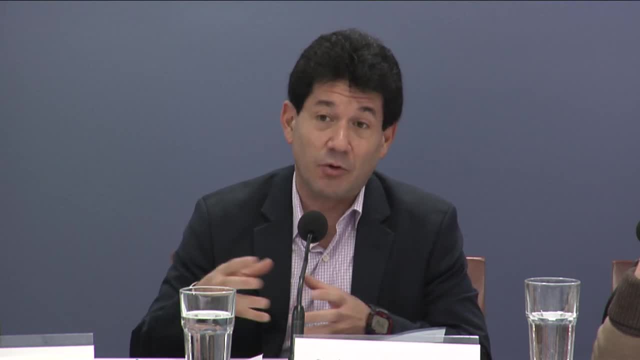 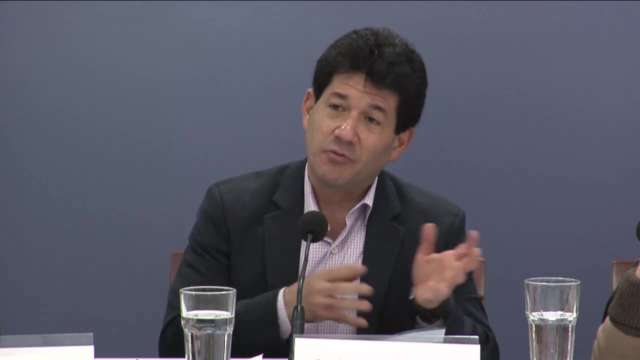 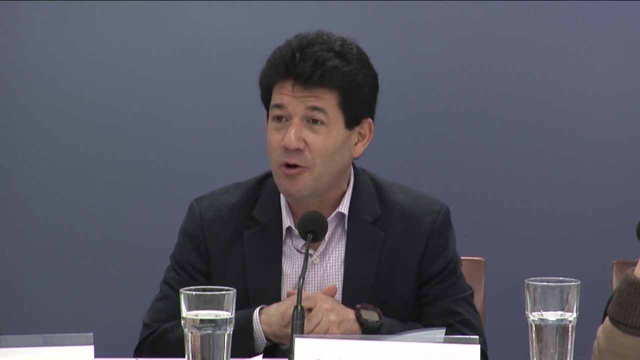 is no longer there, then this could be interpreted more as a temporary phenomenon and the policy response should be totally different. The response under the first would be: let's keep on doing what we've been doing, but under the second the page would still be more of a blank page. 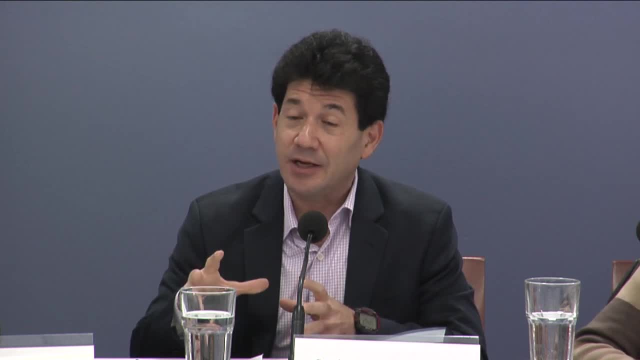 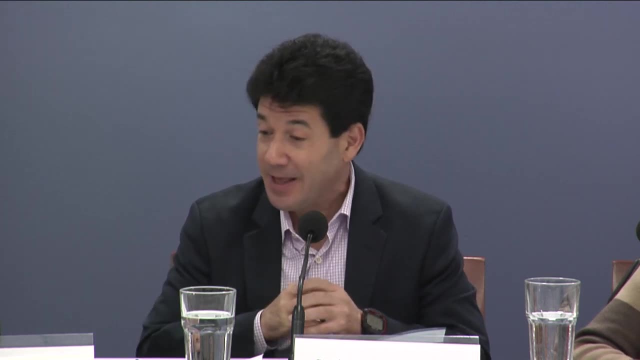 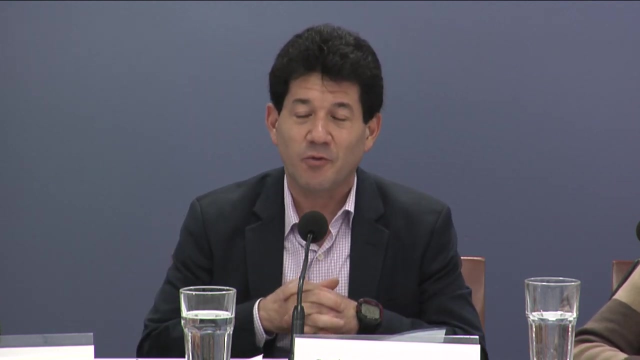 and of course, the book is very helpful in guiding the discussion on where policies should go to change the structure of the economy. So that's why I don't think just going to education as such would finish the discussion. I think we should still look at the external side very seriously. 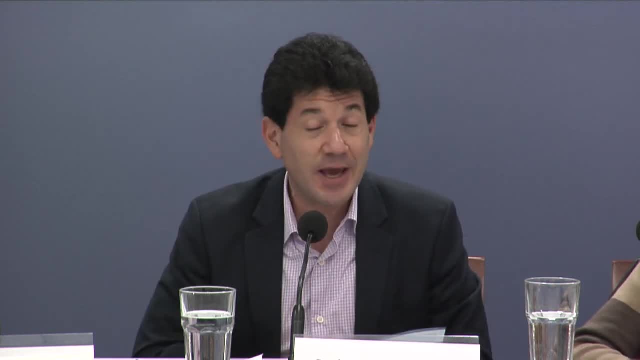 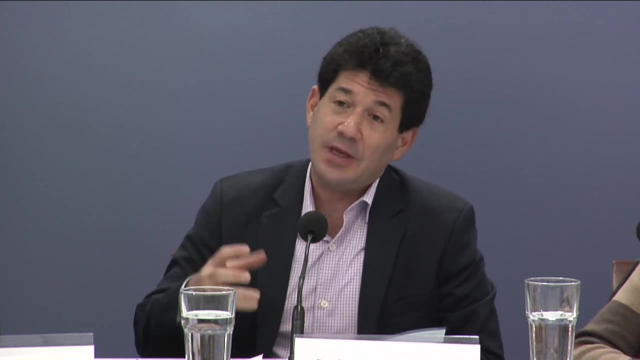 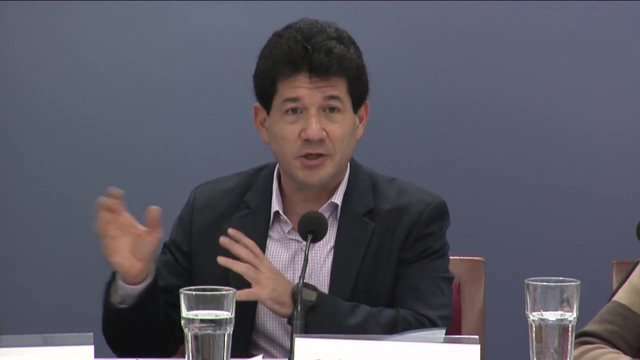 and I'm glad that Barbara is going to do that. Then, on education, it's not that easy either, because one story could be simple: that more people getting more educated, then that would tend to reduce the wage premium, and then we could explain the story quite straightforwardly. 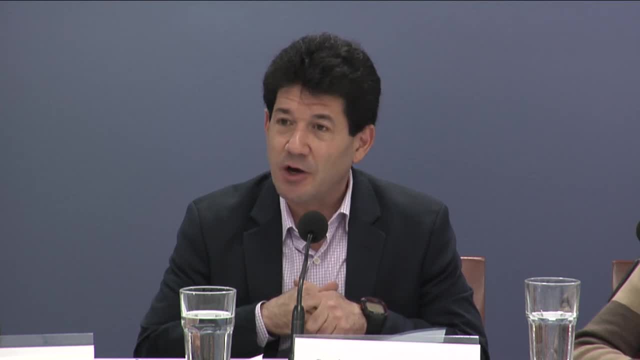 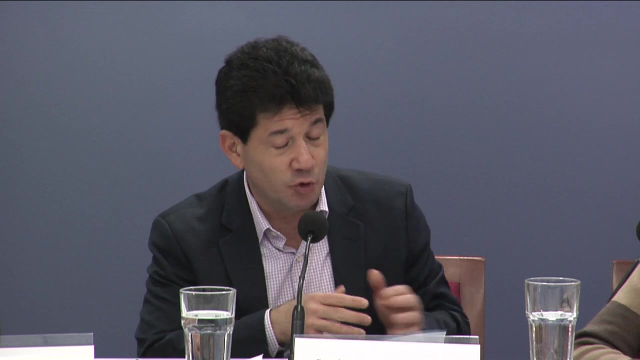 but it doesn't seem that that is the case in many of the countries in Latin America. Actually, an alternative explanation for the decline in the returns to education could be that the economies of the region are not absorbing the human quality, which there is a huge challenge in quality. 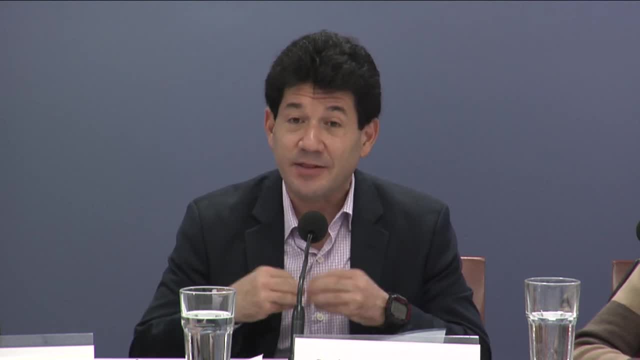 of course, but that they're not absorbing the human capital that is being made available. So if there are more people competing for exactly the same number of jobs, that could have as consequence a reduction in equality, which is not the same as a story. 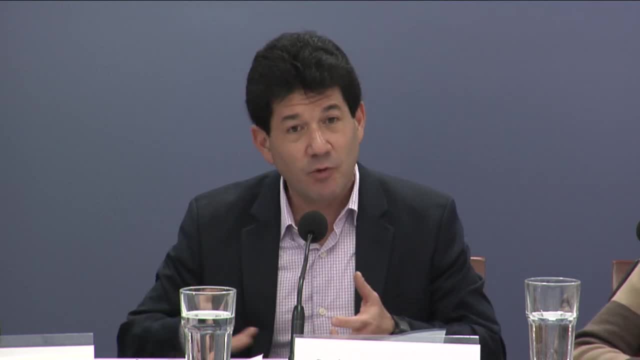 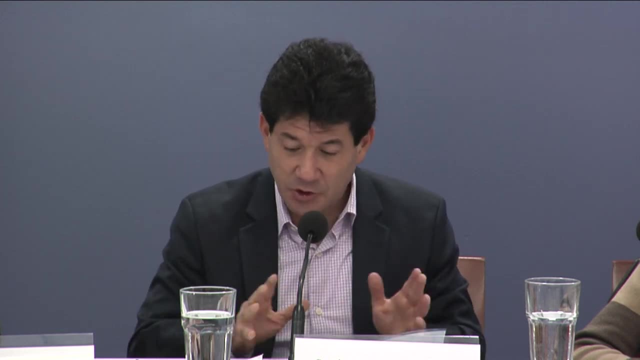 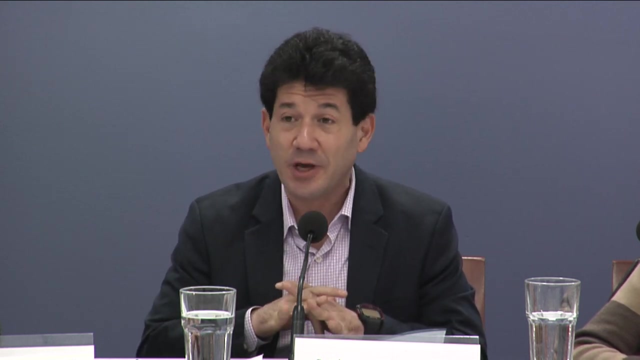 where there are many more jobs for well-educated people. now we have more educated people and then inequality declines. It's a very different story And I think, again, being education central, we shouldn't dismiss the other part of the economies not being able to absorb whatever education is out there. 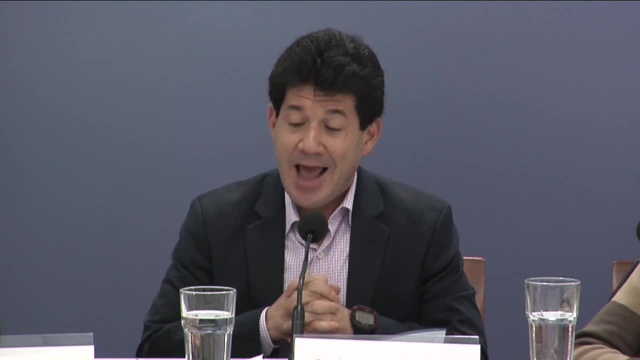 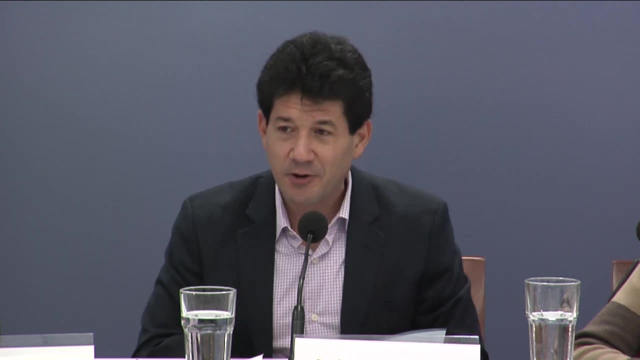 which has certainly been increasing. also, And finally on the. So I do think it's an issue. We could talk about equality in education, and I would there direct you to Julian's other book, which is excellent about that and really discusses in detail. 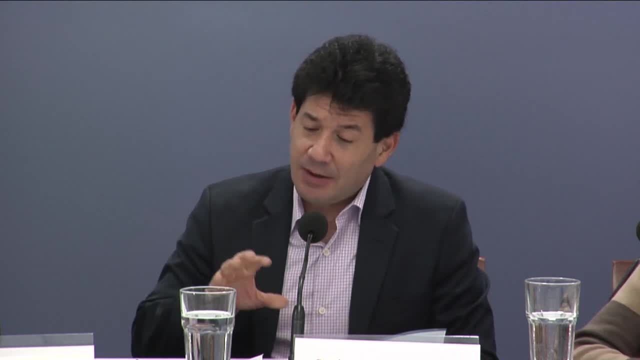 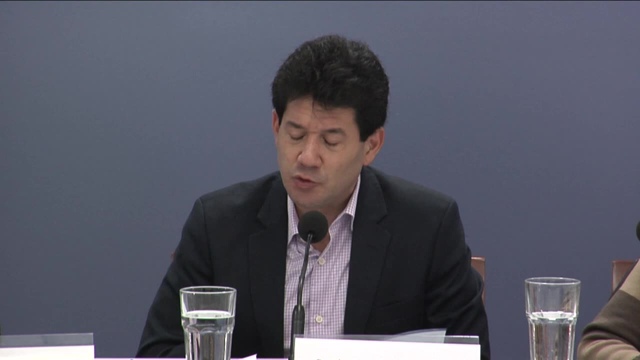 the policies for improving education. But in terms of the future, I think there's another issue that I don't recall seeing in the book, which has to do with the returns to education, which could be crucial, which is that if the returns to education are declining, 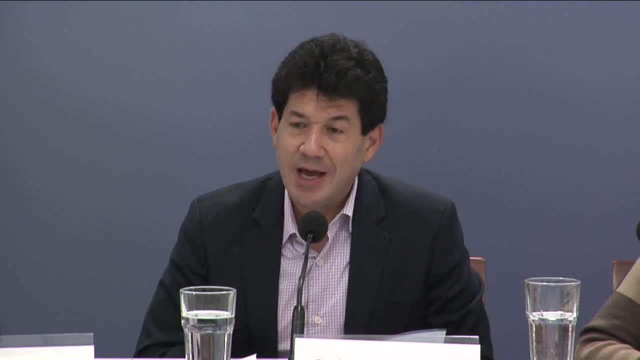 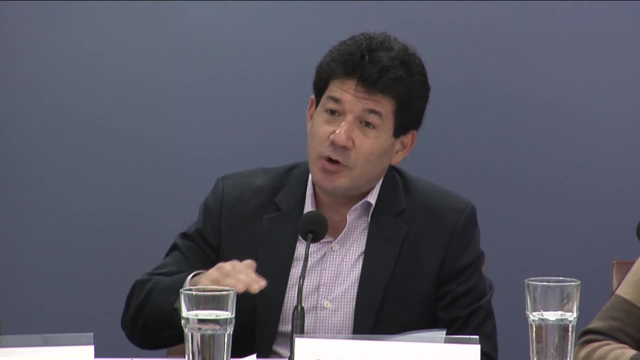 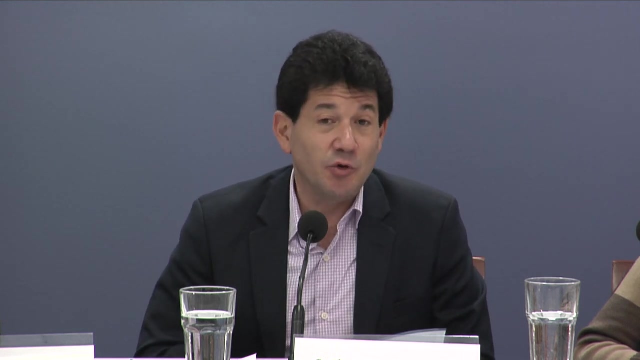 again, it could be for different factors. one consequence to the future is that people might have fewer incentives for investing in education. So this downward trend that we're seeing now, and following the line of argument of the book, would not necessarily continue if the returns themselves 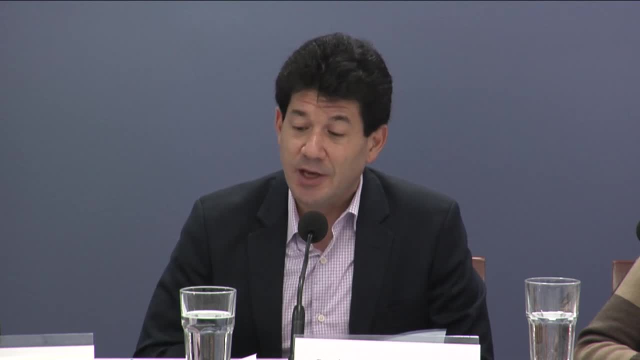 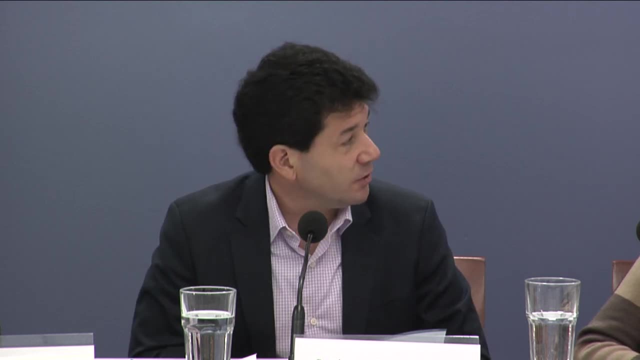 the returns themselves determine the demand for education in the future, And that would be a red light. definitely that in the education policy area should be looked at. Do you want to make a comment, or? Sure, We seem to be sort of making opening statements. 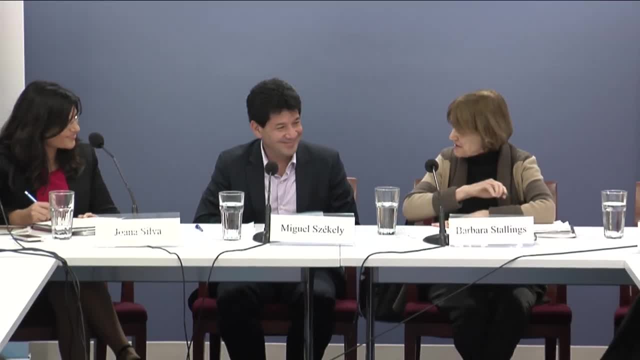 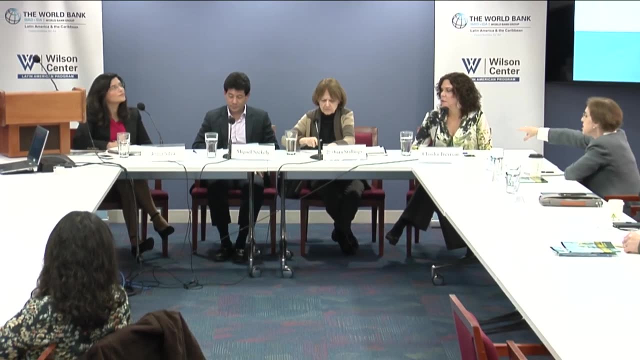 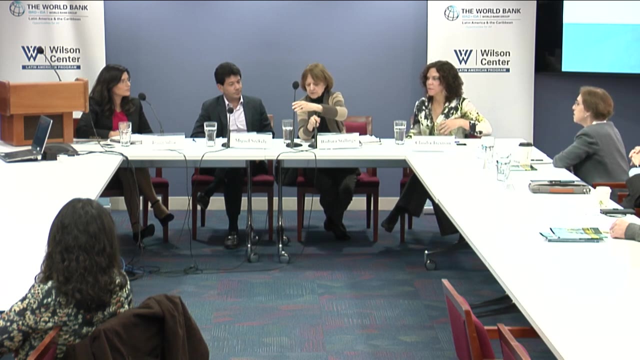 so I'll make my opening statement. First of all, thank you very much to Cindy and the No, Take this. There's no button to question. Is it supposed to be red? if it's on, No, no, It's. 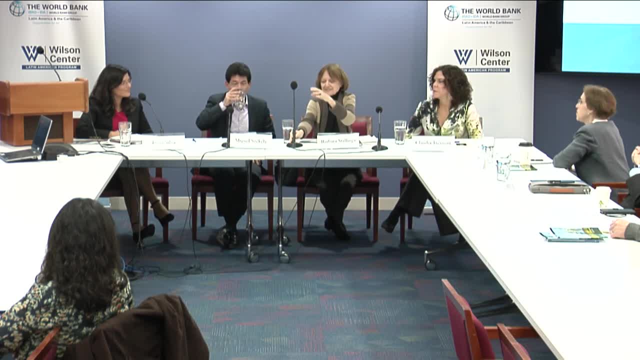 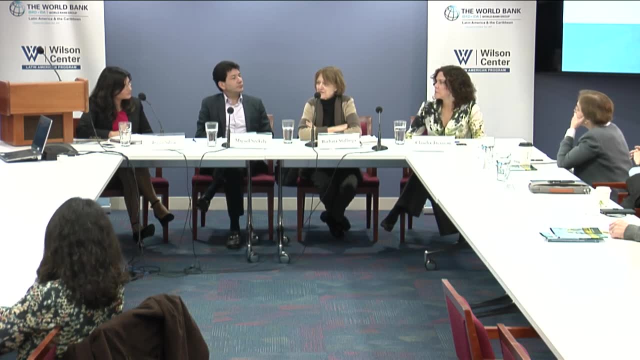 No, It's not on, That's right. yeah, Yes, okay, There we go. Okay, so first of all, thank you to World Bank and the Wilson Center for the invitation to be here. I was not paid to say the following sentences. 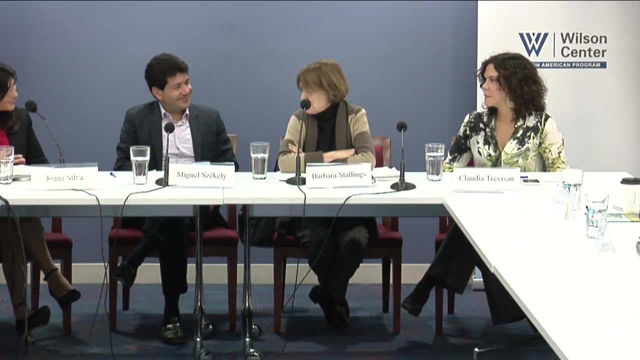 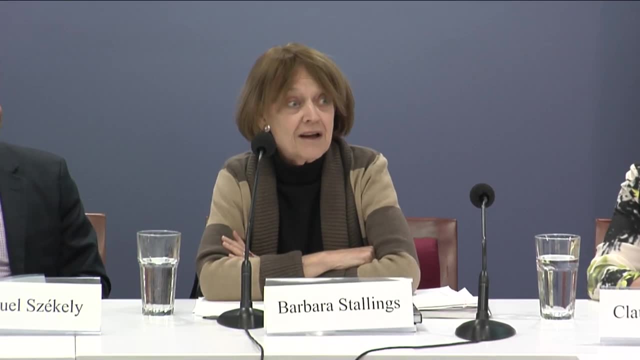 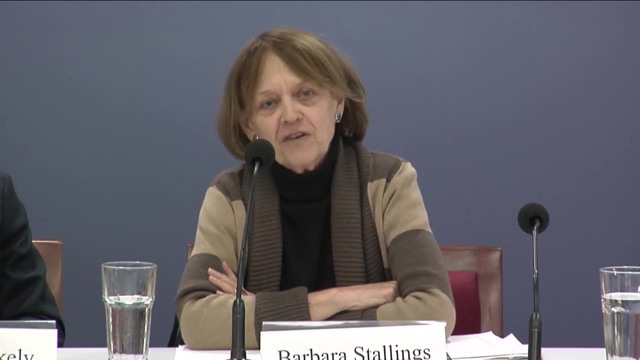 I want to. This is really a treasure trove of data and smart analysis For anybody who's interested in inequality, not just in Latin America, but other places as well. I cannot recommend this book too strongly For other places. it's got some very interesting methodological ideas. 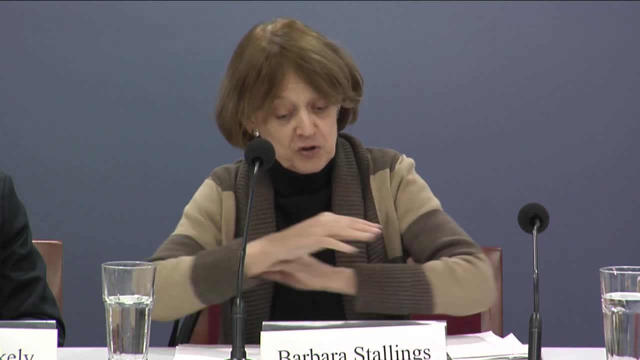 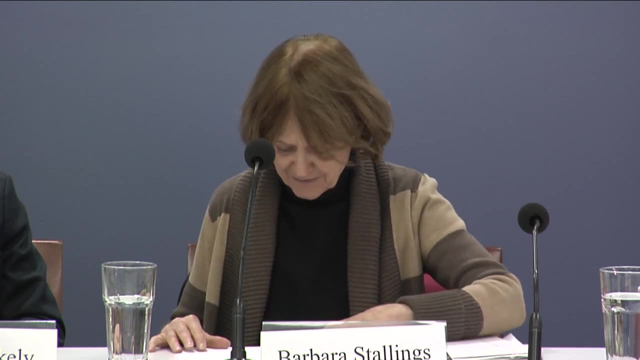 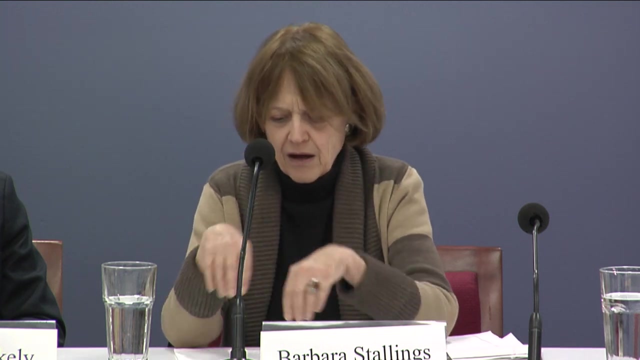 and it would be terrific to have some comparative analysis to put alongside the information in this book. So you did a great job and I was most happy that I had a reason to read it carefully. I want to, as I said to Joanna yesterday afternoon, 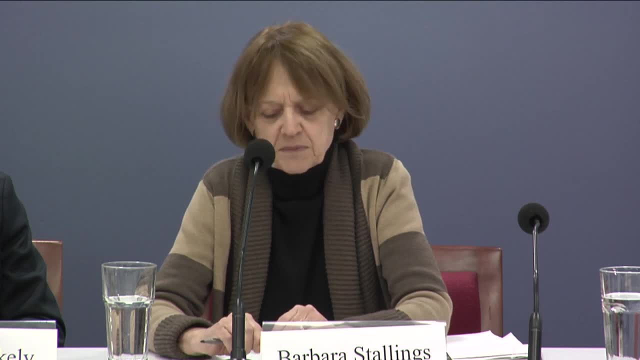 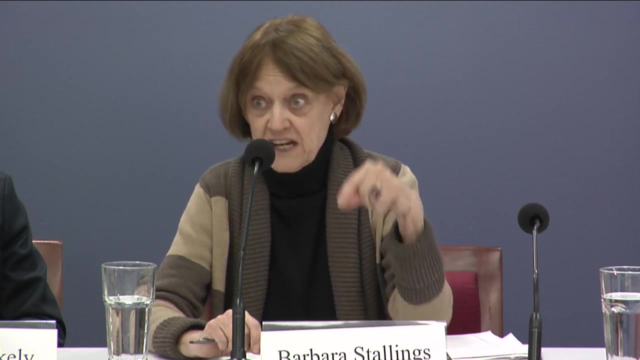 when we talked briefly, just express a little skepticism about one aspect of the methodology, and that has to do with the problems of using survey data to measure inequality. It's especially a problem with household inequality, less of a problem with wage inequality, which is the subject of this book. 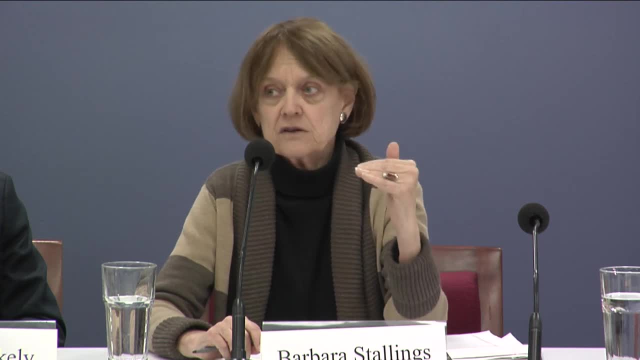 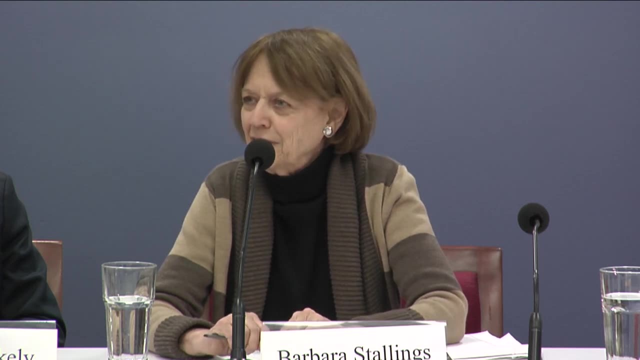 Nonetheless, they make the argument that the two go hand in hand. I think it's more complicated than that. When I was at ECLAC, we did a very large multi-year, multi-million dollar project on the impact of the economic reforms on growth, employment and equity. 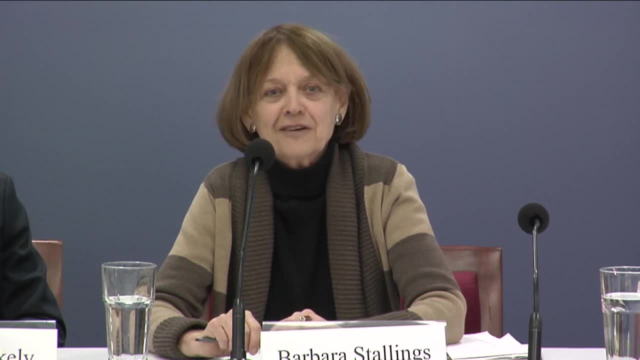 Sam Morley, who might hope to see here today, but he's unfortunately not here. ran, a very well-known expert on income distribution, ran the module on distribution. We talked a lot, a lot, a lot about the use of surveys. 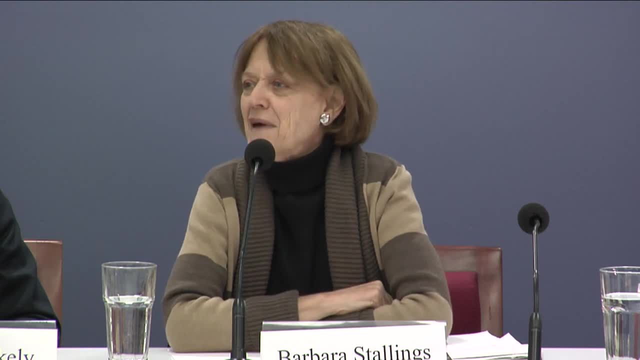 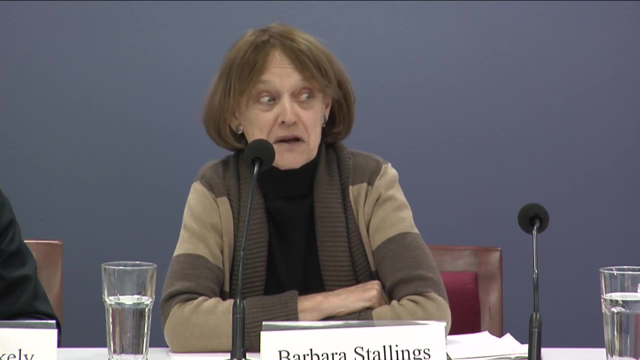 Now, because they're chalkboards, they're topped off at the top. Just imagine a surveyor going and knocking on the door of a very large mansion in any city in Latin America. If the door opens at all, it's opened by a gardener or a guard. 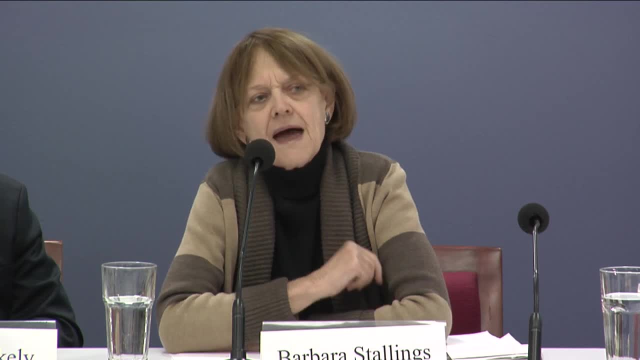 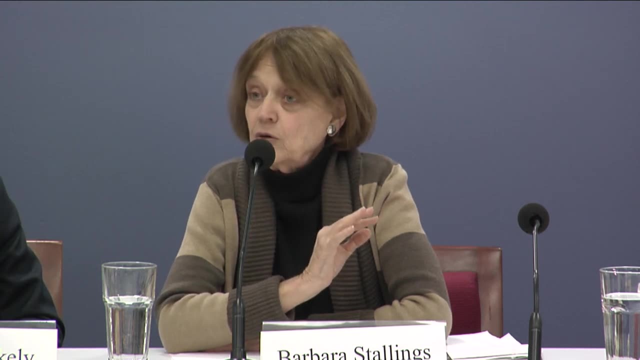 who sends the person away. You can't get that information, And it may well be that at the household level, we're missing something very important. There's an example: right now, The Piketty people just did a study on inequality in Brazil. 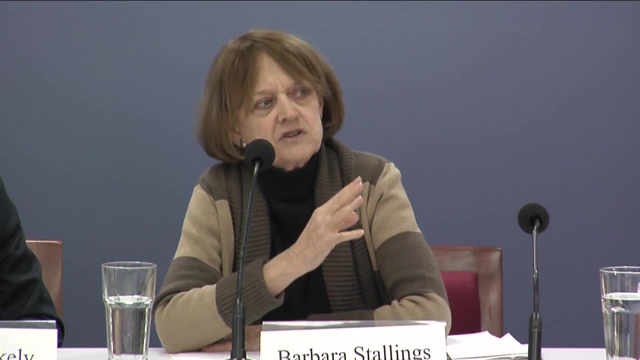 and they say it didn't go down at all. So there are different things going on. and it's not that we shouldn't use surveys. That's the main tool we have. We just need to be a little cautious and see to what extent we can find. 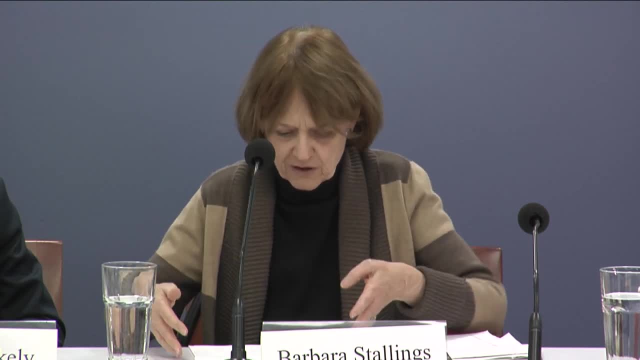 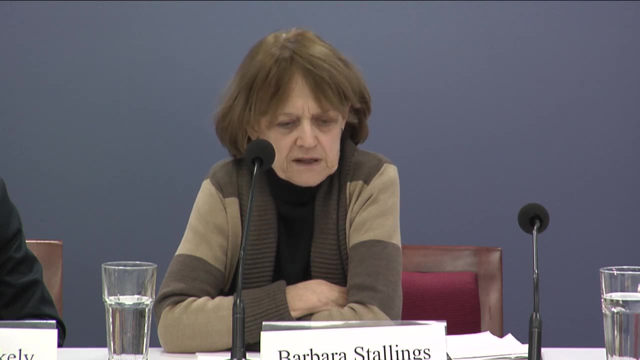 other sorts of complementary data. Now let's get back to the issue of education and growth. In reading this book over the last few days, I've come to think of it about in the following way, and I'm interested to see how you react to this. 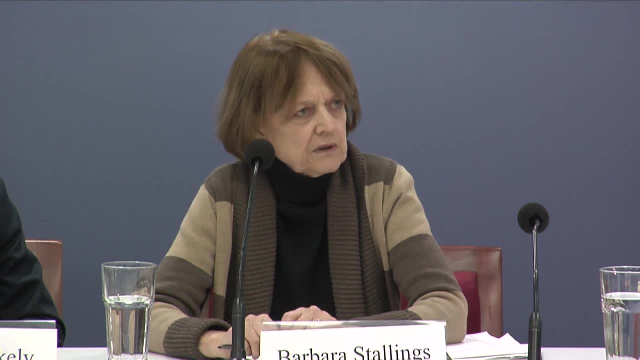 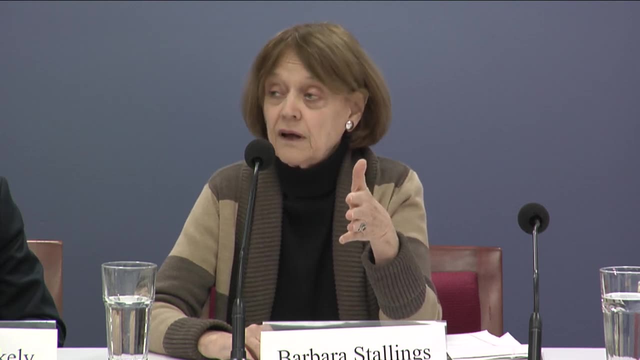 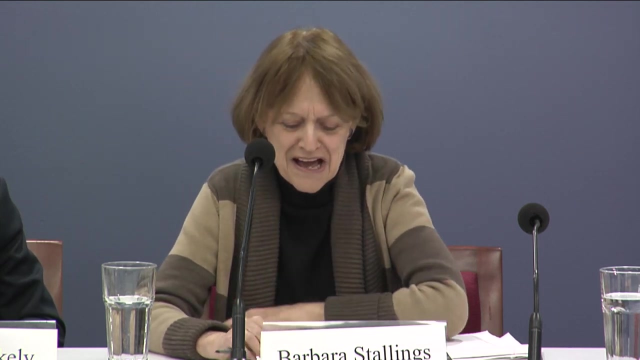 That we have a situation of necessary and sufficient conditions, That education, the increase in education since 1980, that's quite a long time ago, That's over 35 years- None of us can count That that is really a necessary condition. 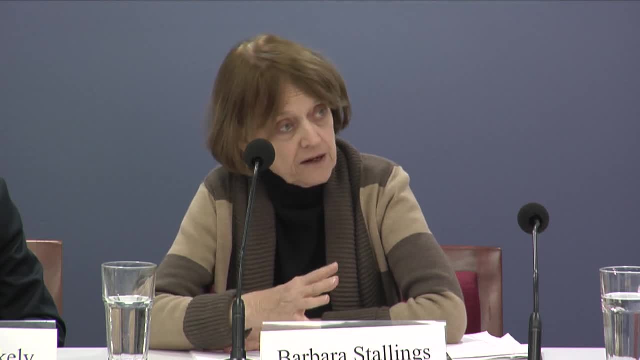 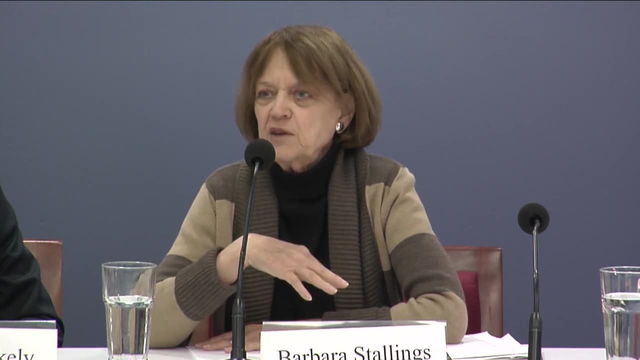 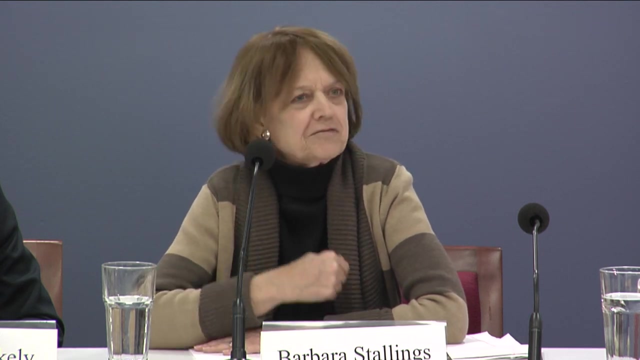 for inequality to have finally begun to go down in the Latin American community, But it is not a sufficient condition. We can just keep on. I think that some of the people at Augusto de la Torre, former chief economist for Latin America at the bank, 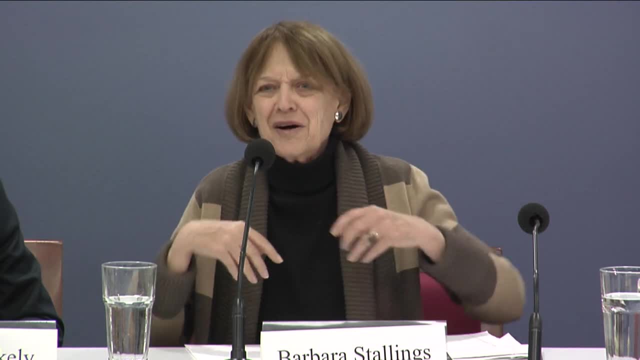 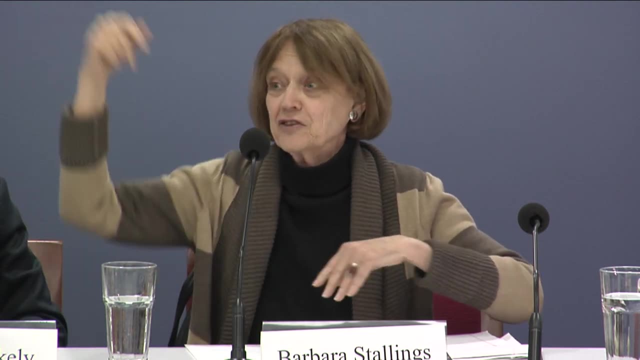 did some work on this and he gave a presentation, I think in this very room a couple of years ago, showing that you can't explain something that goes like this with something that goes like this. But this would not have happened if we didn't have the increase in education. 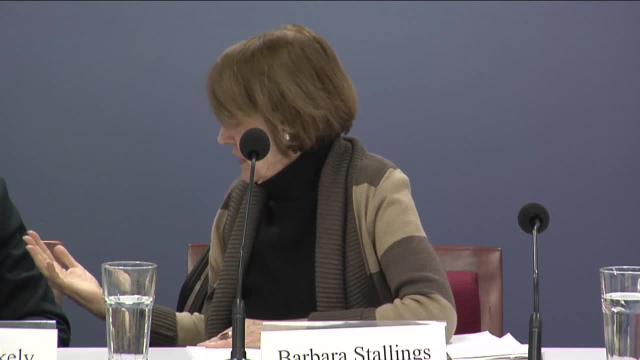 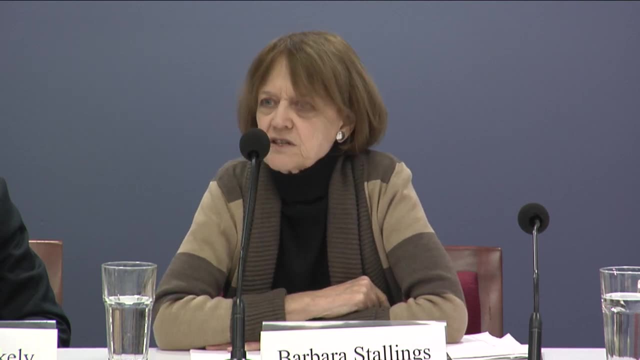 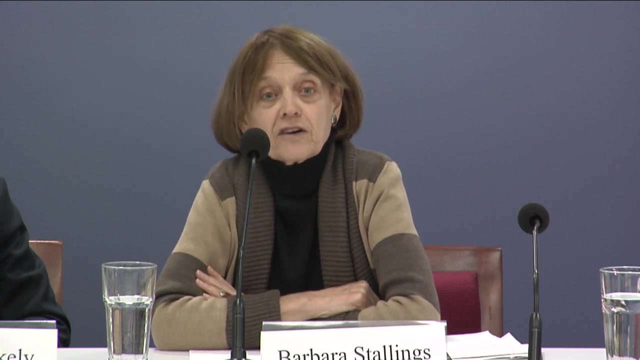 and the decline in the skill premium, for whatever reason, I found convincing your reason, but there may be some others as well. But so that's a necessary condition. The sufficient condition, as far as I'm concerned, is what Miguel called the external factor. 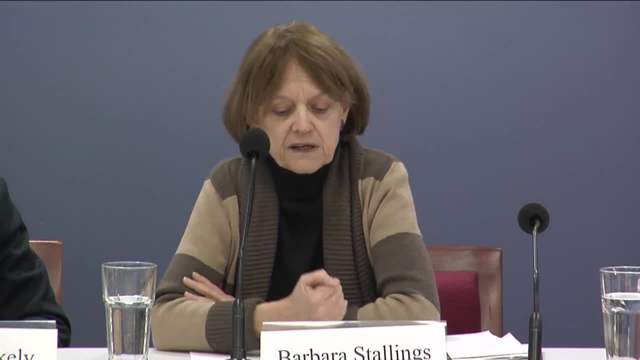 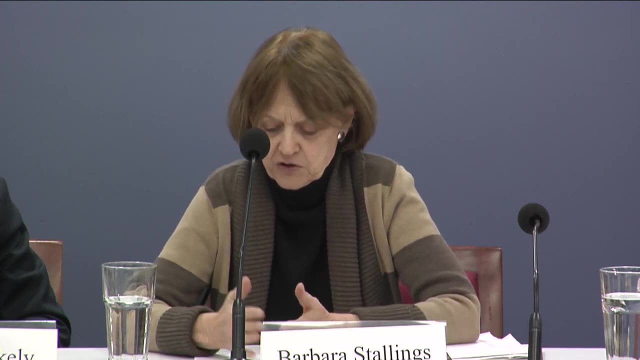 Let's just call it economic growth- And clearly, insofar as that was more important in what they're calling the decade of the 2000s- actually they're using 2002 to 2010-11,. clearly that was more important in South America. Why was it more important in South America? Because of the opportunity to export, especially to China, but not only to China, And that really spurred a decade-long period of growth, the likes of which we have not seen for a very long time in Latin America. 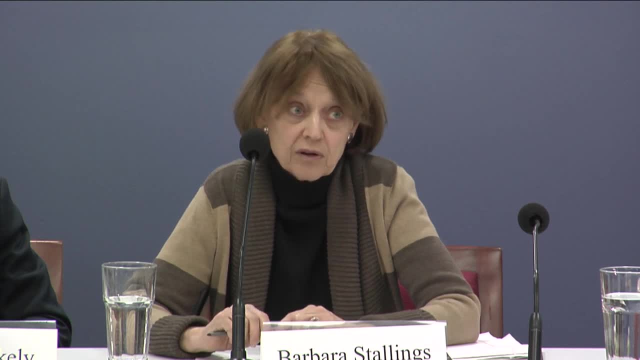 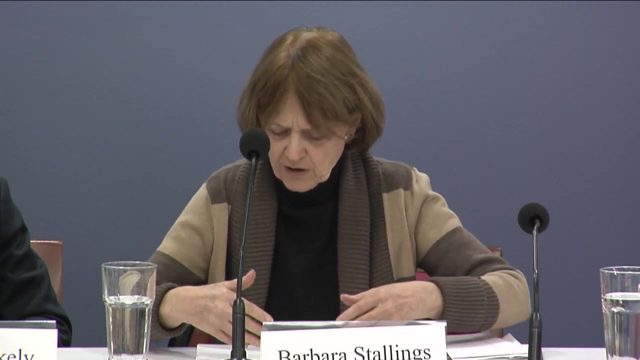 Unfortunately, it turned out not to be very sustainable, And as soon as China starts trying to change their growth model, then Latin America's growth has slowed down. Let me just say there are lots of things that I think go together here. I think that formalization and high growth 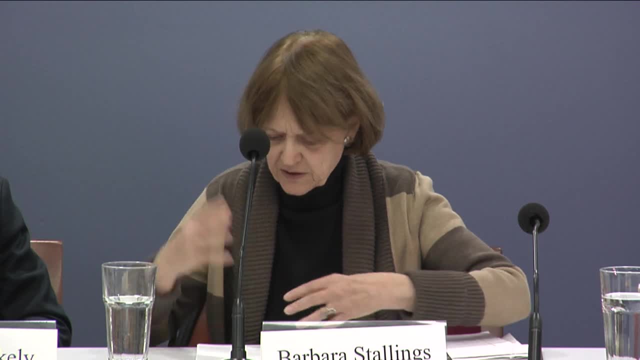 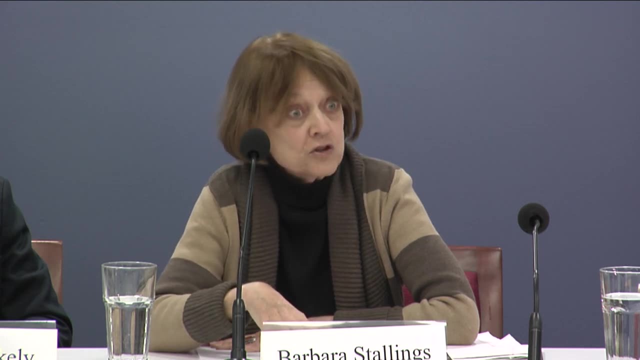 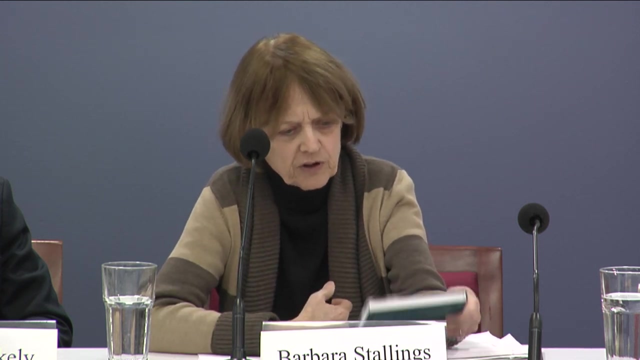 probably tend to go together. Sectoral aspects, your very nice analysis of tradables, non-tradables. So it's a constellation of factors around growth that are the sufficient factors in the current conditions and the way I see things. I just co-edited a book with Alejandro Foxley. 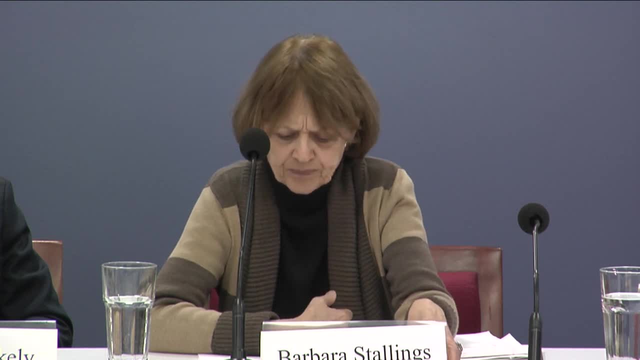 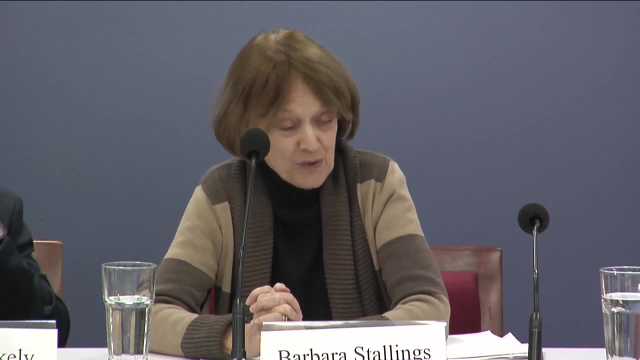 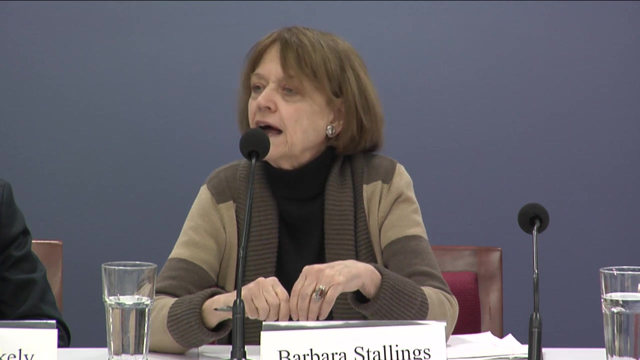 that came out last year called Innovation and Inclusion in Latin America, And there's a very interesting chapter in there- more interesting than my chapter in there- by a Korean economist who works on Korea and China. His name is Kan Lee, from Seoul National University. 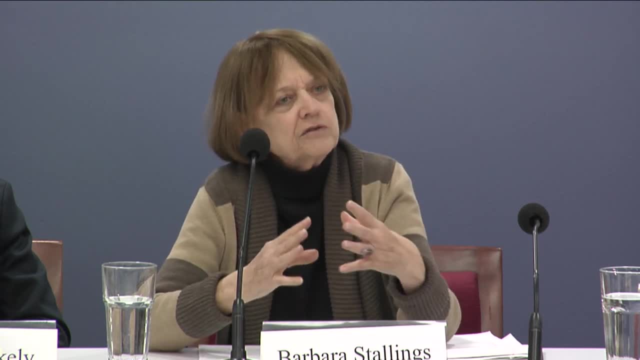 And he's trying to see if there are any lessons that can be drawn for Latin America from the Asian experience. In a couple of sentences here's what he says, which I think is very interesting and very telling: That in order to get inclusive growth. 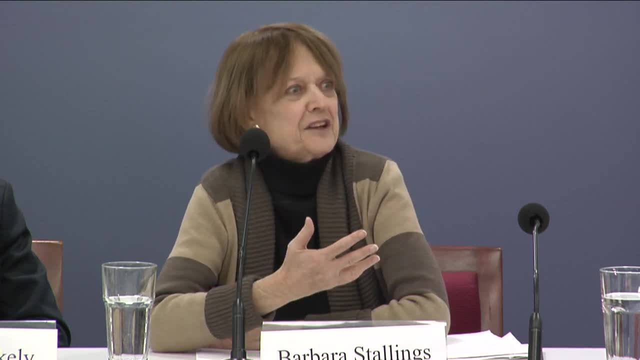 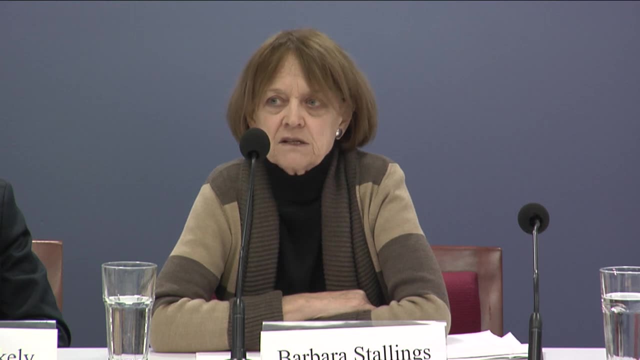 you need to have not just education, which is in abundance in the Asian case. you need to have a long period of sustained growth. He says at least two decades, if not more. It's not until you have a long period of sustained growth. 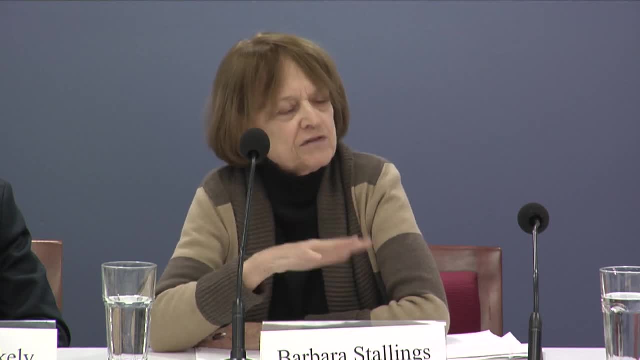 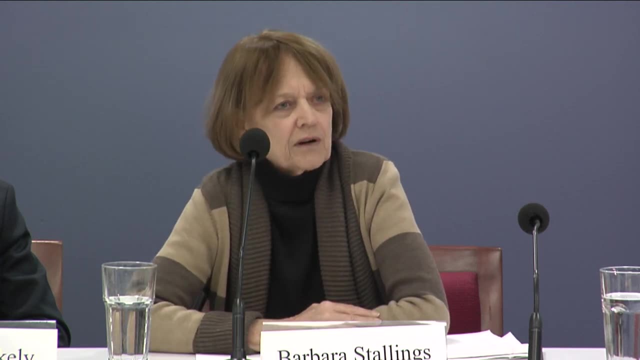 that wages will begin to be driven up. Now how does that compare to Latin America? Lots of high growth, we've seen it, but it doesn't last too long. Why doesn't it last too long? Dependence on commodities. We all know this story. 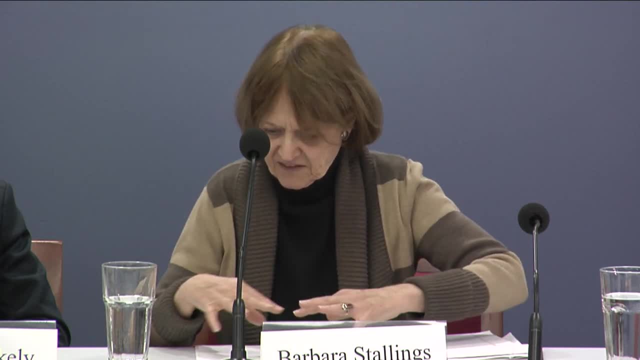 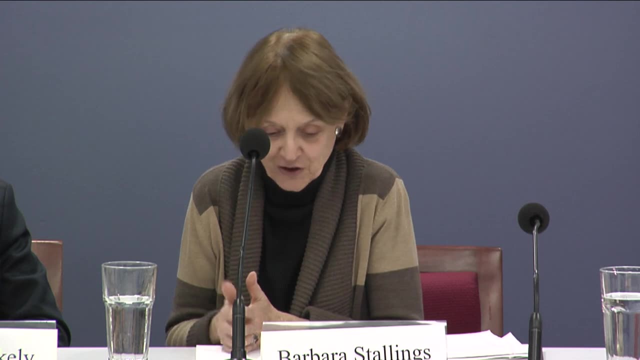 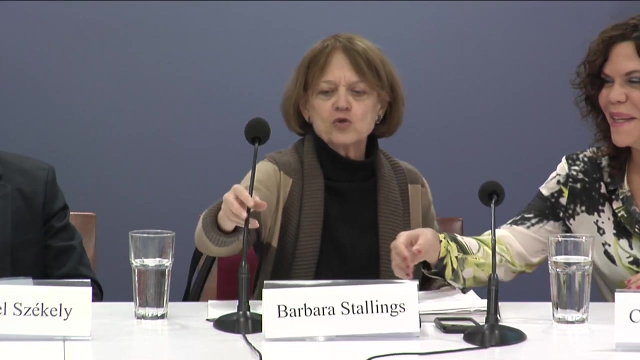 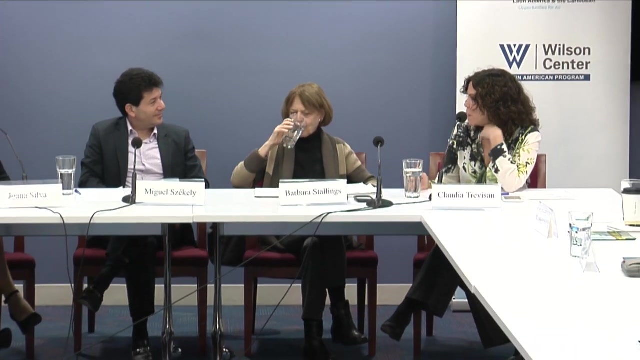 This is not a new story at all, So I think that this is an interesting thing to add in here in terms of my idea of necessary and a constellation of sufficient conditions centered around growth. So let me stop here and we can go on. Yeah, and there is this question that Miguel raised. 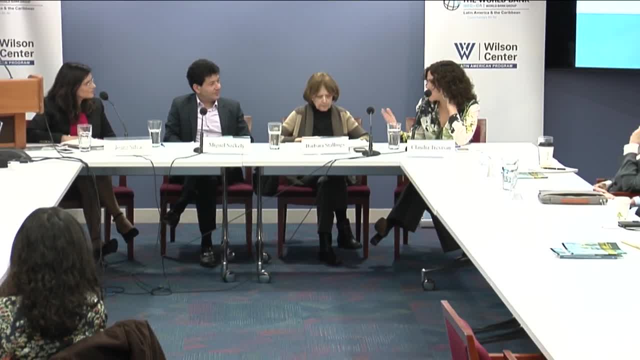 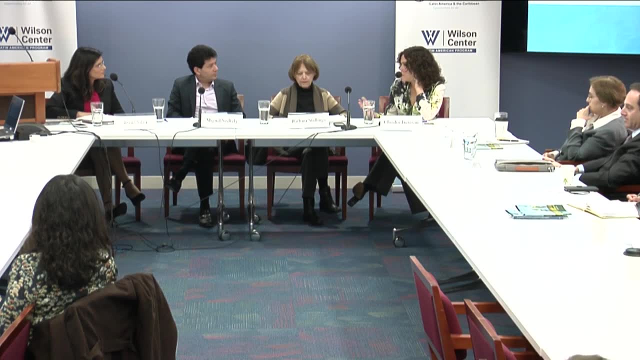 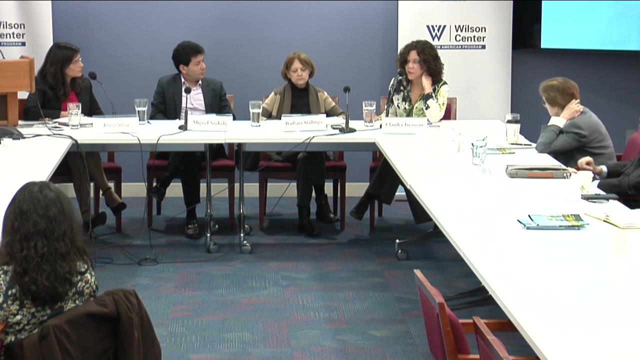 the commodity boom that we saw, this spectacular commodity boom last decade, And with this low down in China, there is no indication that we are going to see another commodity super cycle anytime soon. And growth if you look, if you look at the numbers of the projections of the IMF. well. last year, the region contract GDP of the region contracted after two consecutive years of sluggish growth. In 2017, the expansion will be of 1.2% Next year. no 1.2% this year. Next year, 1.9%, followed by 2.4%. 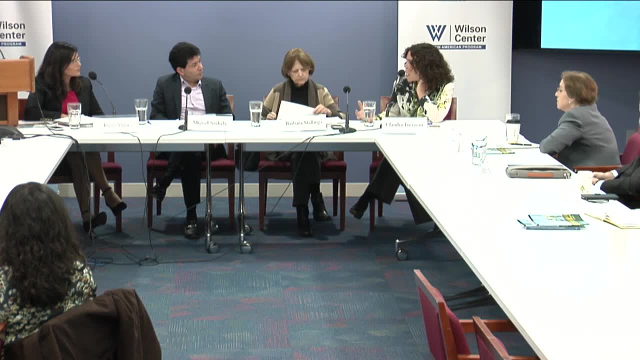 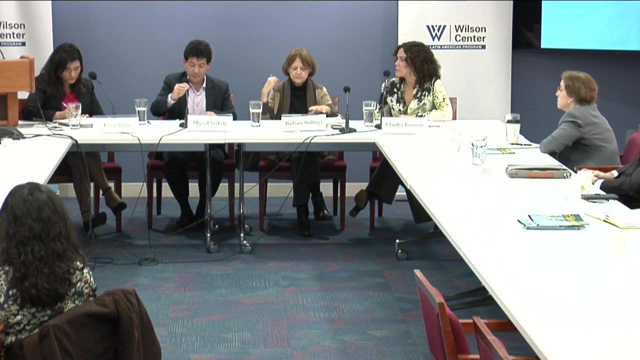 far from strong growth. So how is it possible to change this scenario without expecting for another commodity boom? Yeah well, I think that the book is very good there at pointing this: the final part of the future, and especially these elements that have to do 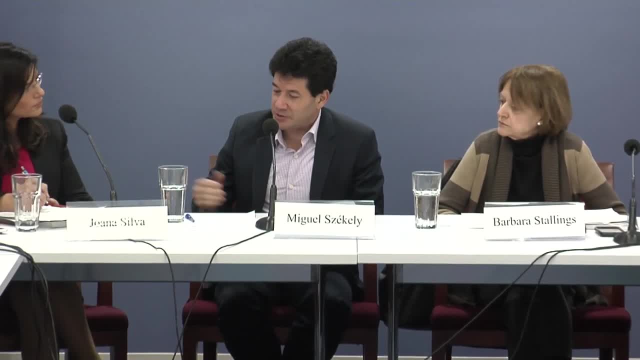 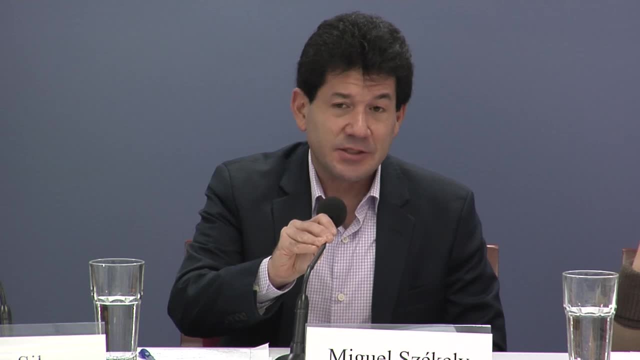 not only with education, but more broadly with the economy, for example, competition, labor markets. I think the answer is really really clear. I think the answer is really really there Because, if I mean again, if we 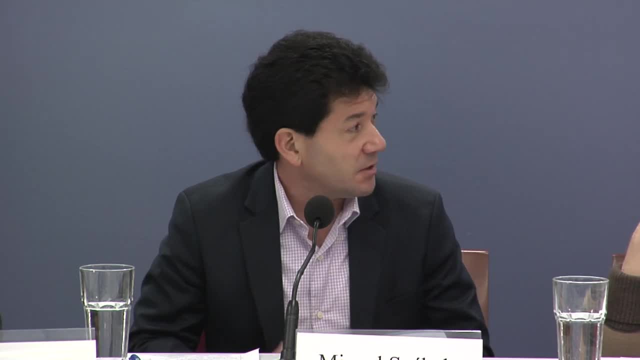 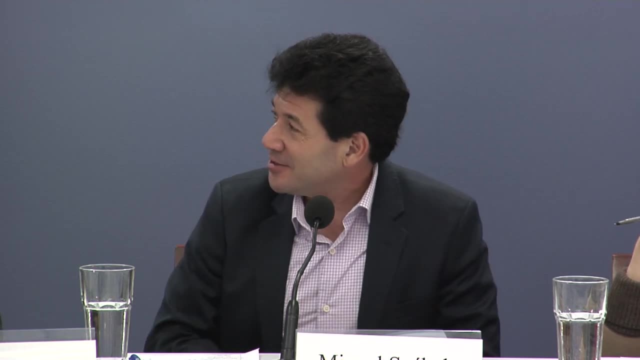 if the explanation is only education, well, let's just. even if it's a lousy education, let's keep on doing it. if it's having this much effect, I would rather go to that other agenda. And if you think of it as a system, 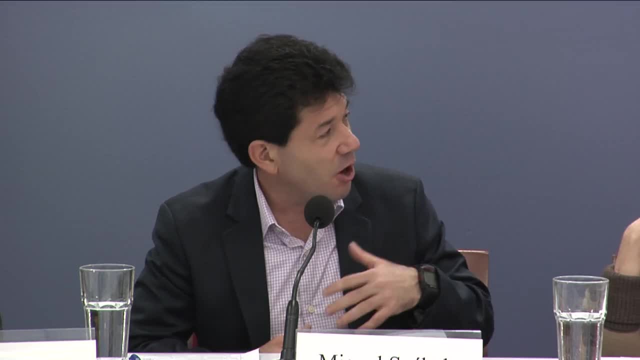 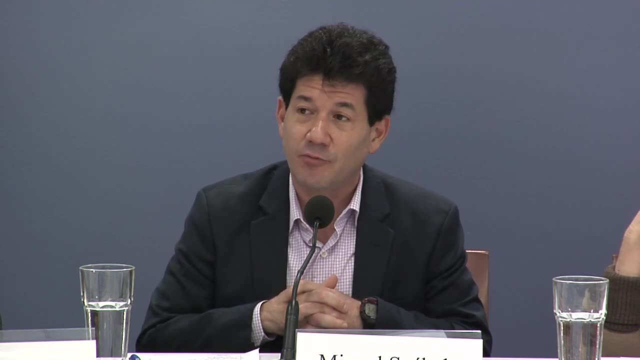 it makes sense, of course, to continue with education regardless of the other factors. But if you don't do something about the capacity of the economy to absorb that improved education, then the effect, if at all, will be very, very small. 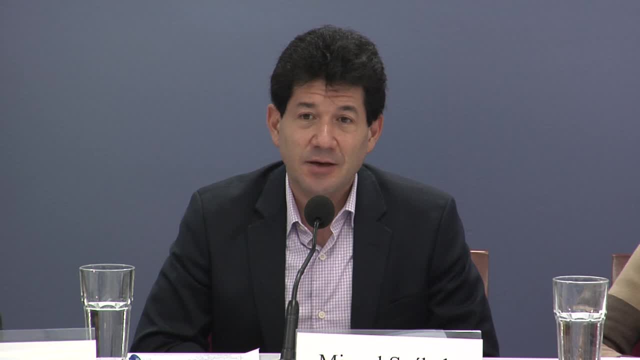 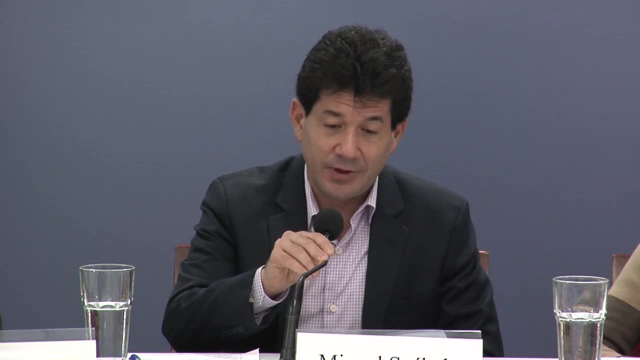 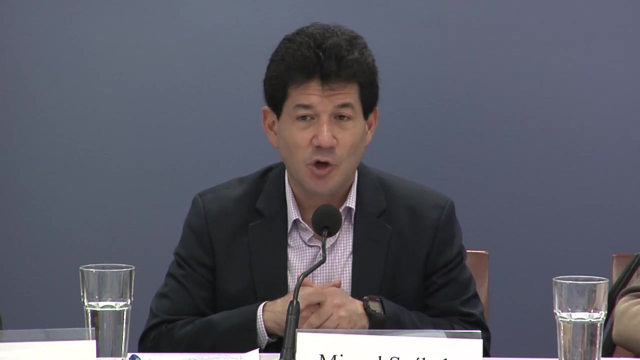 And I think there are many illustrative cases in Latin America of how this is actually happening, For example, with data for Mexico for the last two decades- if you look at the number of people that have higher education, for example, that has been increasing no doubt. 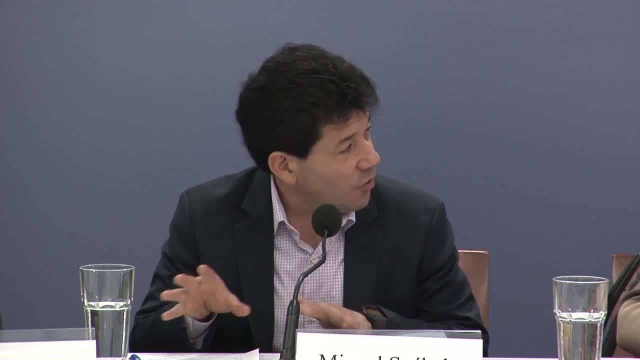 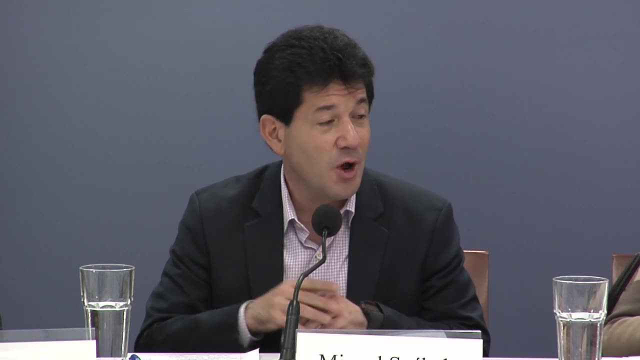 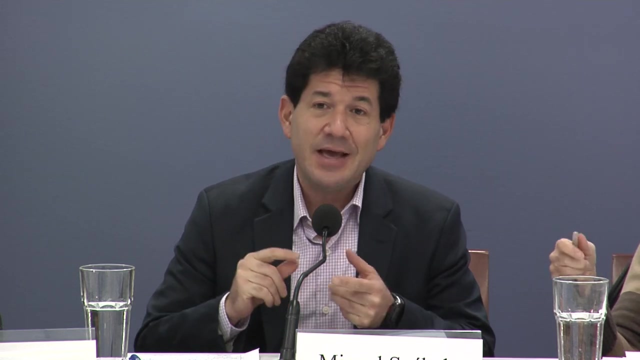 And if you look at any quality indicator, although of course, it's very low quality in general, the indicators show that that low quality has been increasing. It's better quality now, although it should be much, much better, of course, But if you have better, more people being educated. 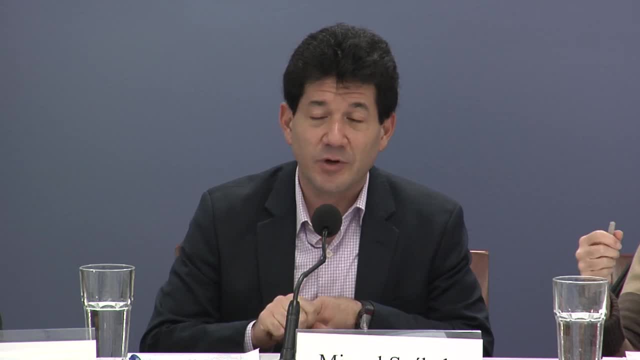 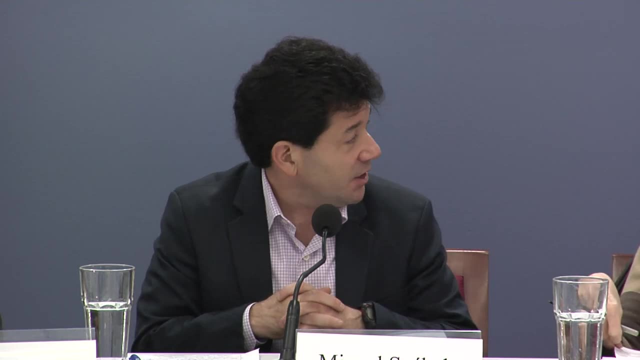 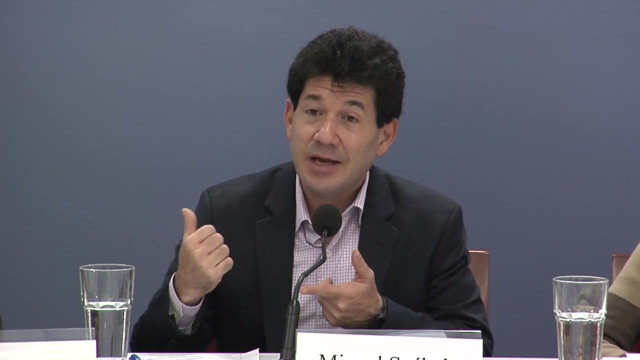 with better education, even if the increase is slow. you would expect then to see the consequences in the labor market, such as in the Asian economies, as the example that Barbara gave, And we're not seeing that. In Mexico you still have very high informality. 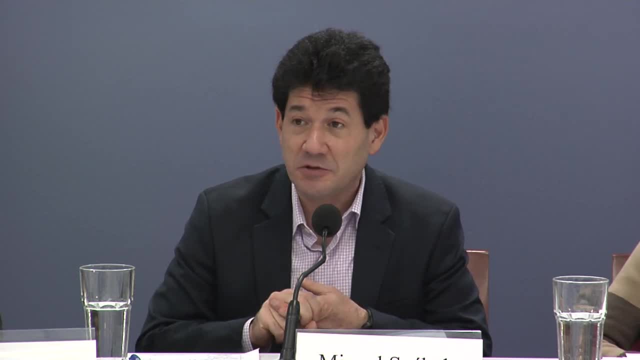 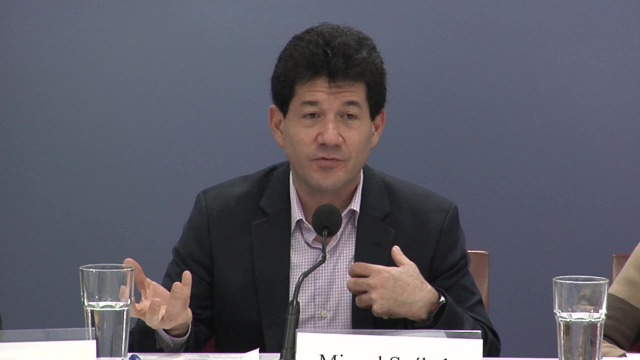 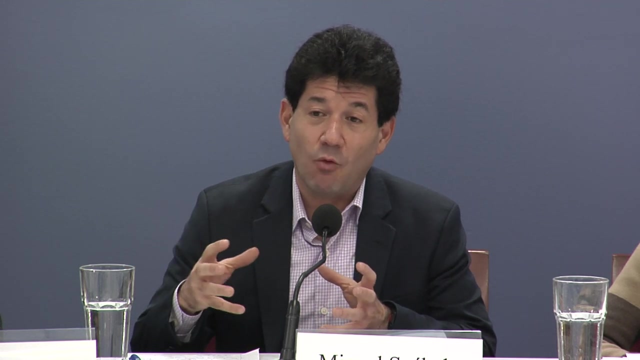 Inequality has declined very, very slightly. Growth is very under expectations. So the promise of investing in education only as a way of solving all the development problems is definitely not there. So when you look at what is the consequence of having more education in Mexico today, 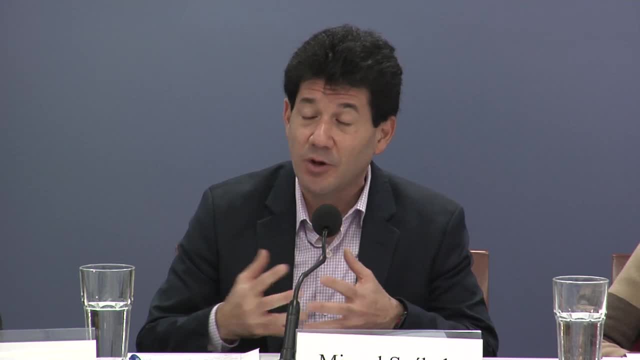 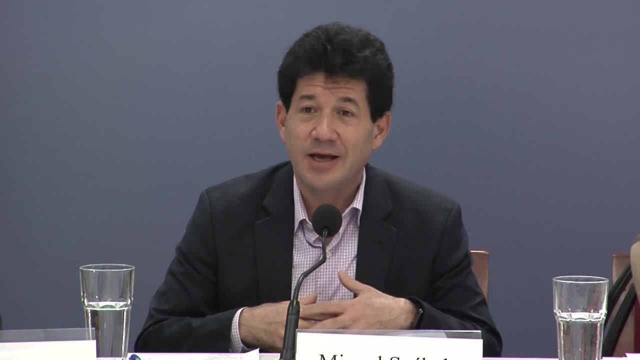 it's not necessarily a better job or a higher wage. There are many people with university degrees that are now performing jobs that they performed when they had only high school education. It's not that education opened the access to a new world, And that again has to do with the structural elements. 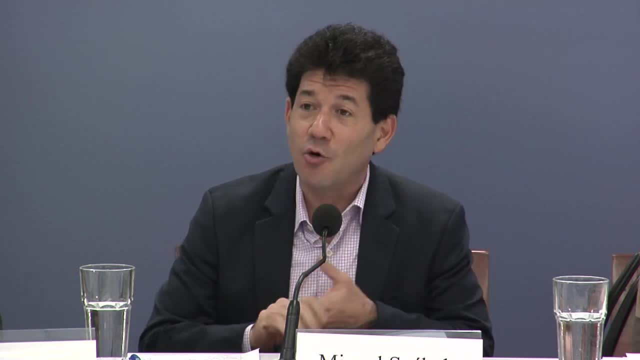 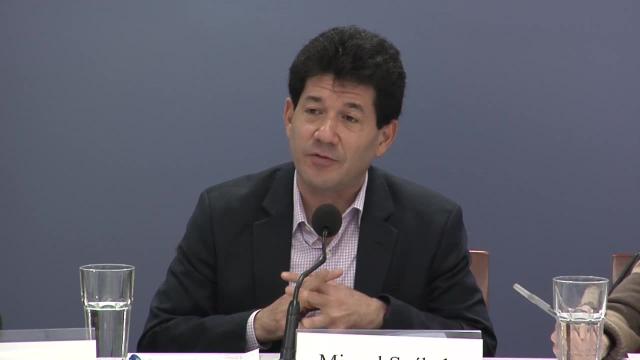 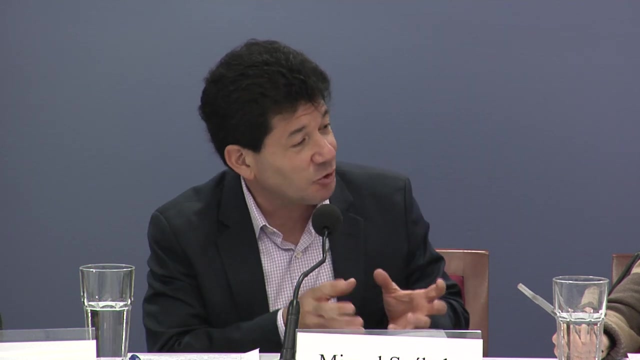 of the economy, competition, how the labor market works, how investment, where investment is directed, which sectors are more the focus of government interventions and promotion. So I would point out that I think there's a lot more to that agenda that is outside really what we conceive as a social sector. 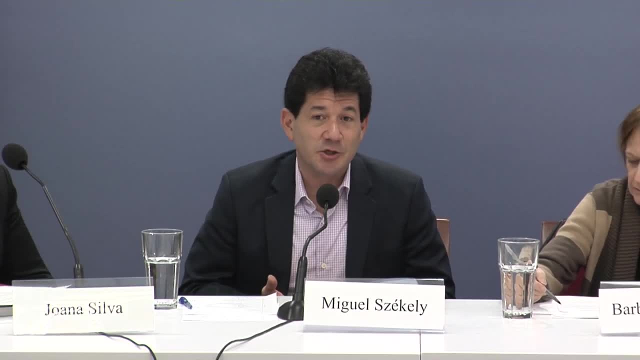 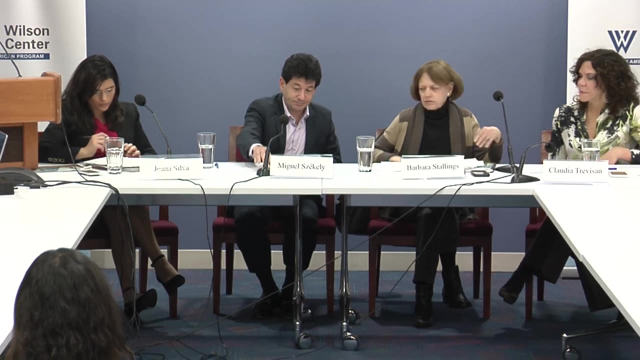 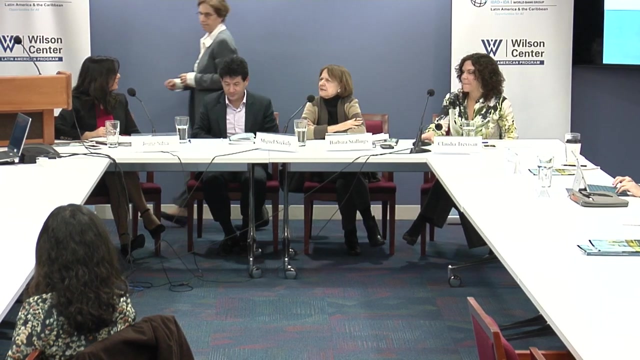 But I think that that is really the That would really lead us to a discussion where the policies to make a big change are really So one of the things that sort of- I wouldn't say confused me but led me to ask some questions. 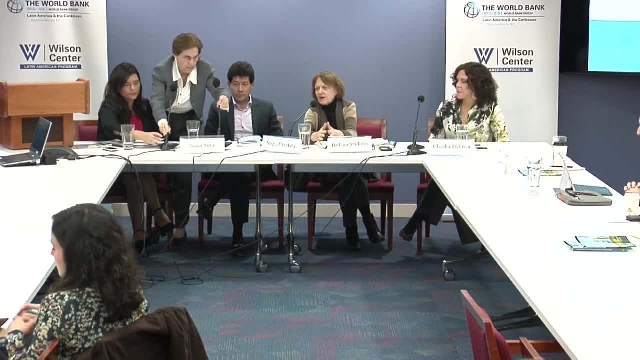 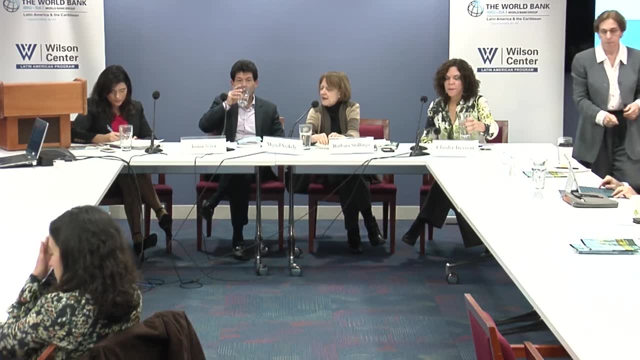 is this distinction between? To me, it's pretty clear what was going on in South America in this decade of the 2002, 2012,. let's call it Less clear to me what was going on in Mexico and Central America. 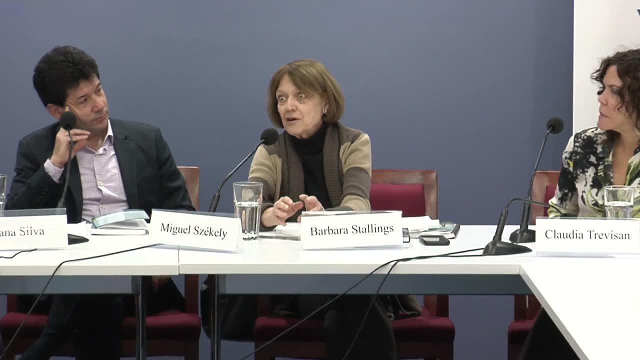 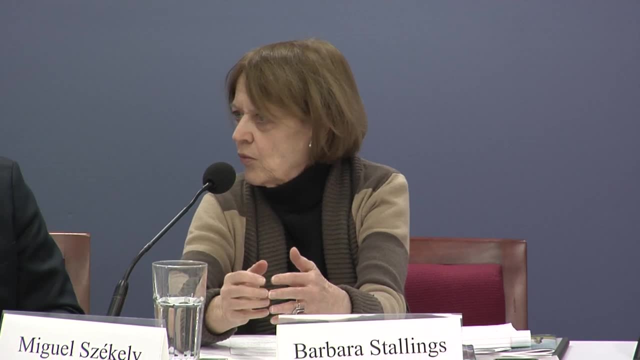 And when you now say that what's going on in South America is more like what was going on in Mexico and Central America, I think we need to study those cases to know what was going right and what was going wrong and if there are things. 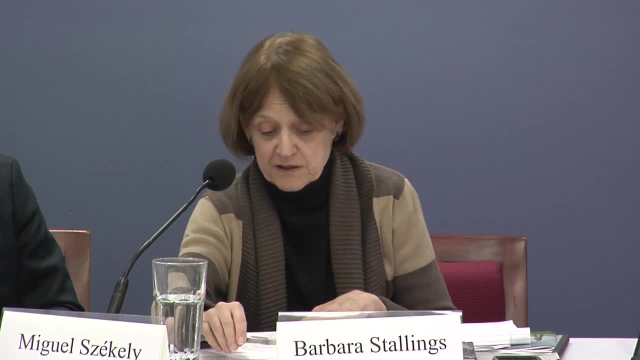 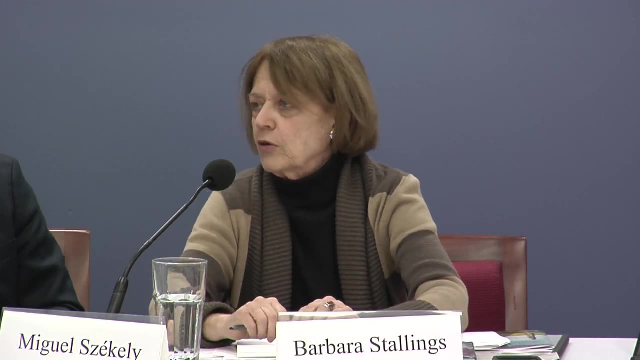 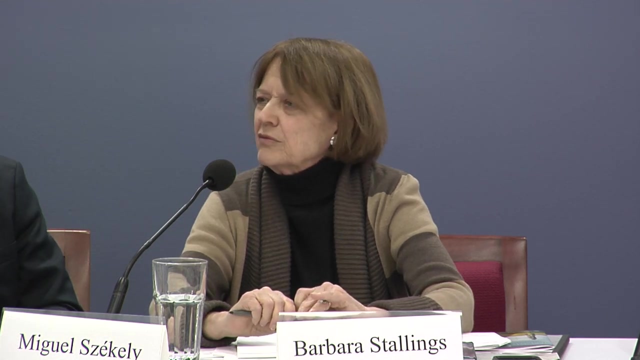 that could be done. Miguel's comment about Mexico doesn't sound very encouraging. The whole idea of pro-poor growth, which is a term that's been around for decades, in some ways, is what we're talking about here, And one of the really interesting things about the period. 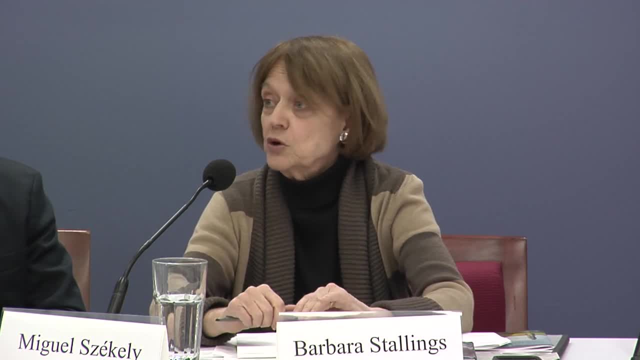 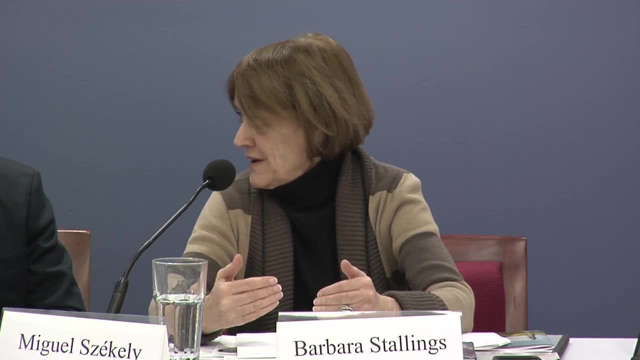 this high-growth period, at least in South America, was that it really reduced the number of unskilled workers, And so when there was a demand for those workers, wages had to go up, more for the poor workers than for the richer, better-educated workers. 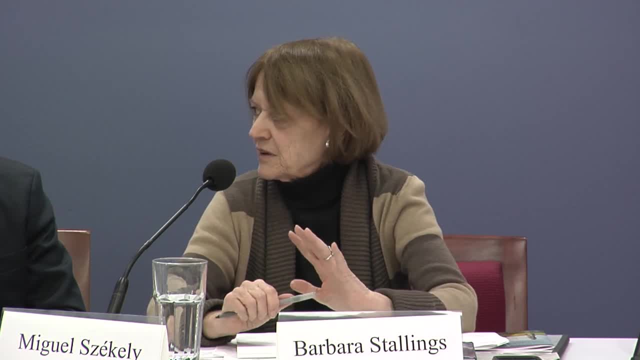 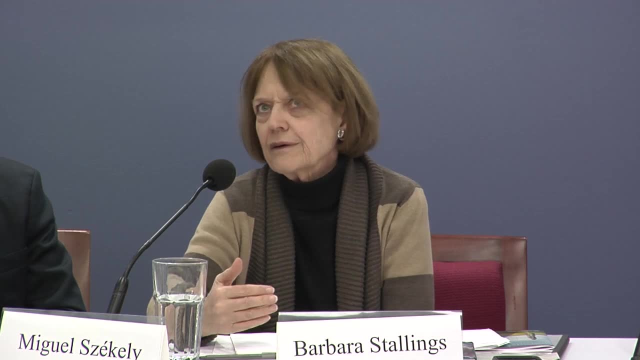 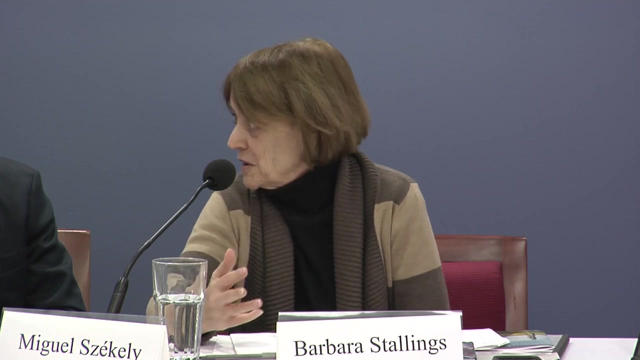 because there were fewer of them. So that's an interesting piece of this story. I have no idea how much that happened in the case of Mexico, But I want to put another kind of policy on the table, to perhaps be provocative and perhaps see what anybody thinks about this. 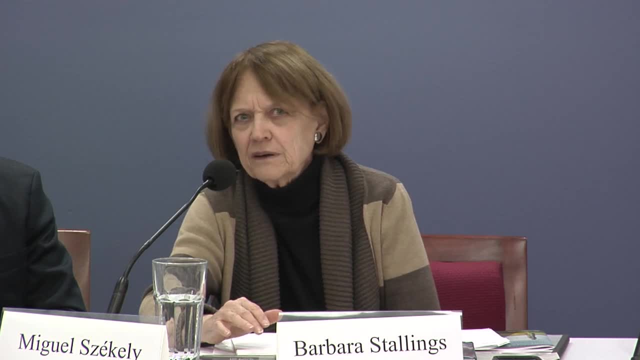 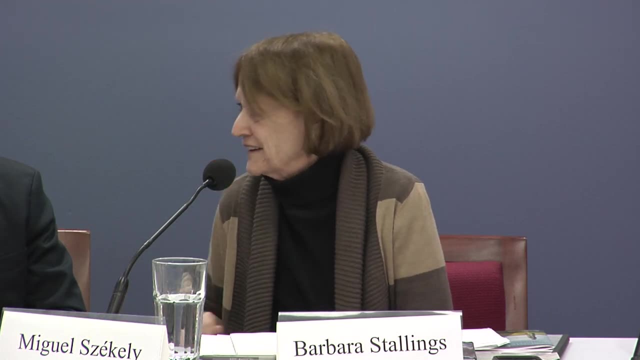 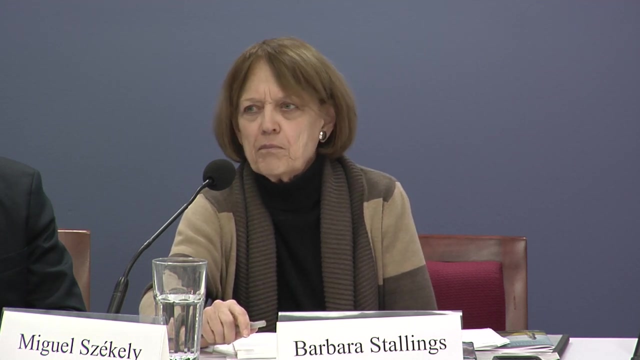 One of the reasons that inequality has been a bit of a taboo subject, despite the IDB report that I got out this morning that you were involved in- is because inequality sort of implies redistribution, so that poverty is a much safer topic. Everybody agrees that reducing poverty is good. 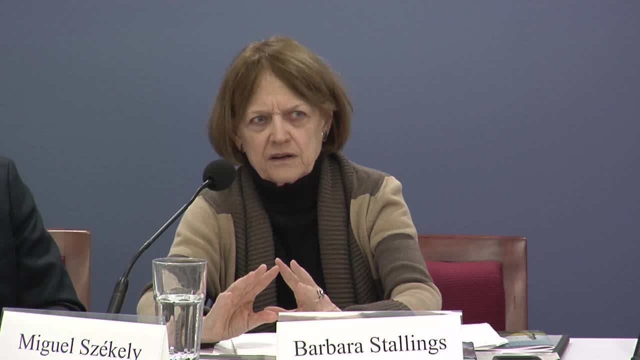 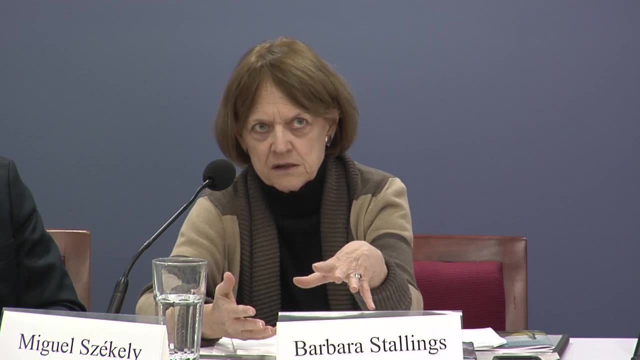 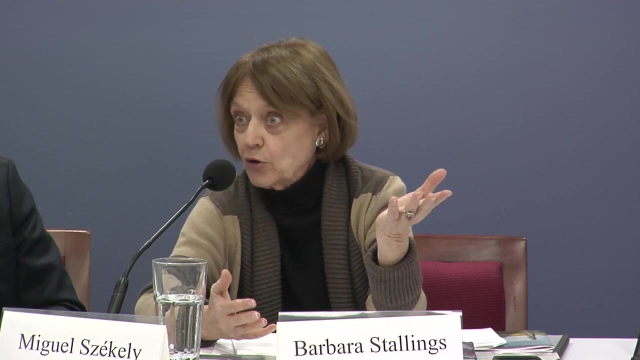 Reducing inequality is more complicated. First of all, the question is of incentives. Some people think that too much equality is a bad thing. There was a day back in the 60s- 70s when it was thought the only way that you could grow 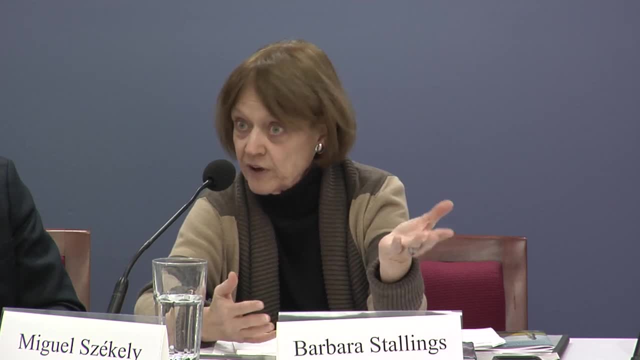 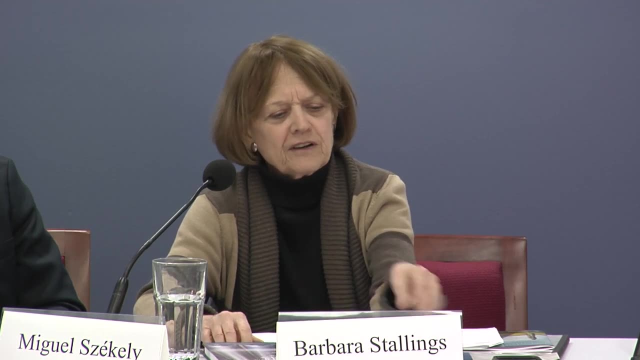 was with inequality, because it was only the rich that saved the Kaldorian view of economic growth. But one of the things- and there's a, very Fortunately we have a book out on the table. We're talking about other books that have been done. 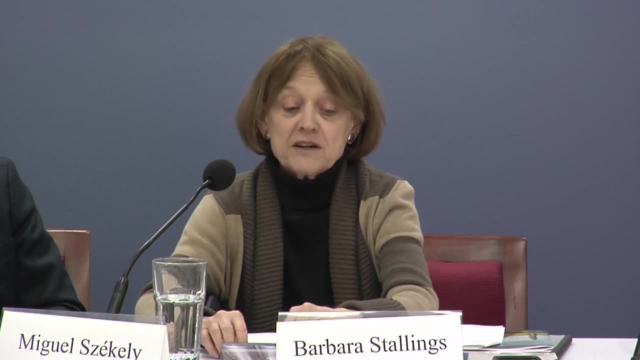 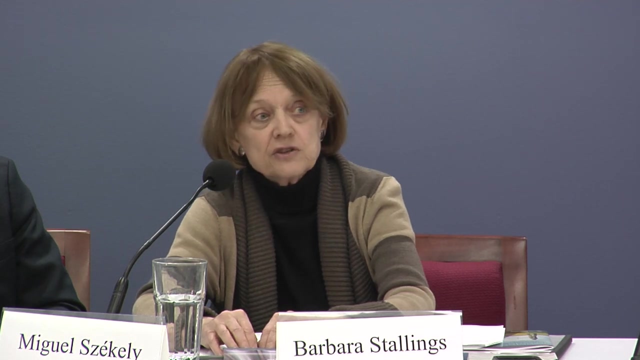 that Cindy was one of the co-editors of about progressive taxation. In the case of Brazil, we have a very high tax rate. Whether it's efficiently spent or not is a different question, But many of the countries in the region have very low tax rates. 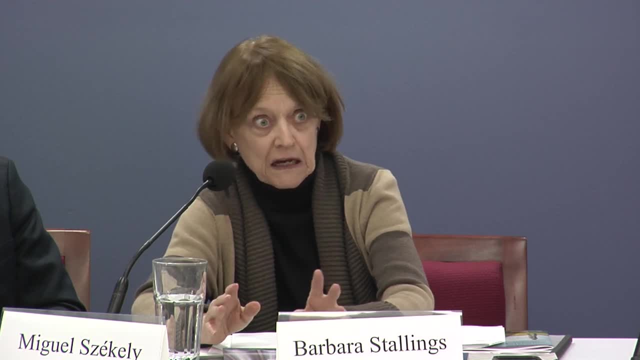 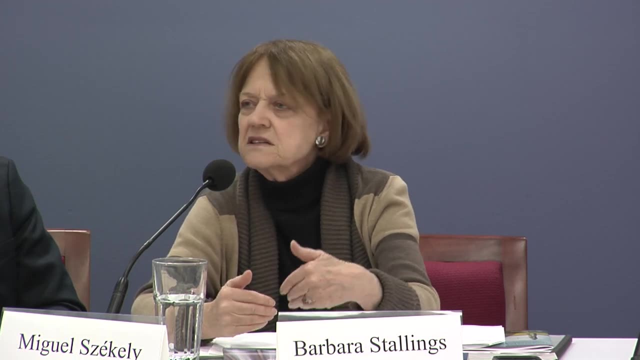 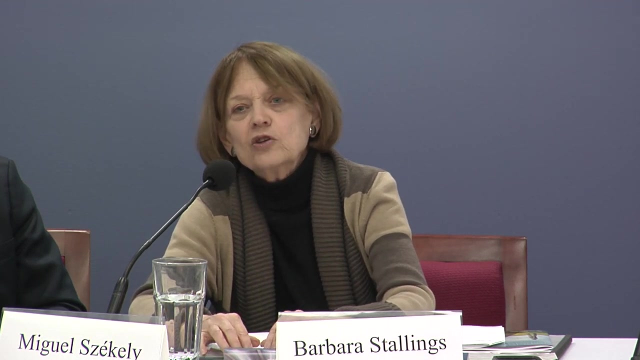 and most of the taxes are collected through the IVA, the VAT which tends to be not always, but tends to be regressive. So is a policy, a complement to the policies that you've been talking about in the book and that Miguel just mentioned. 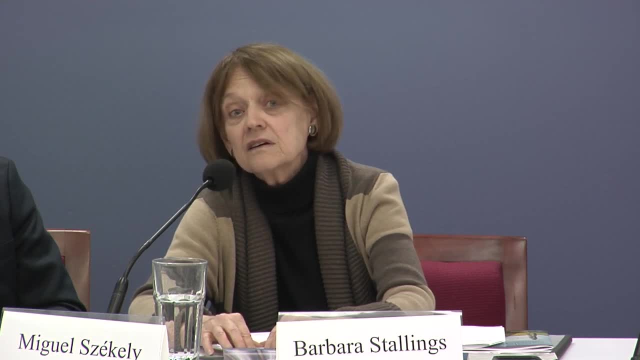 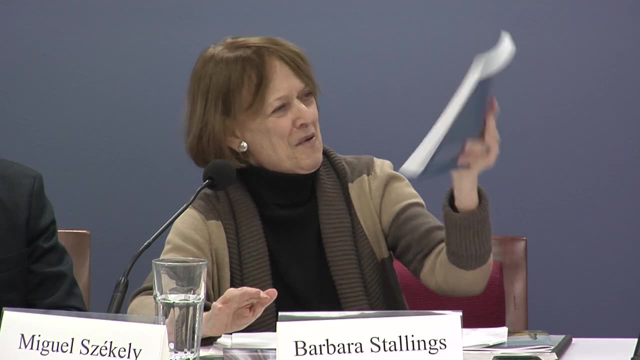 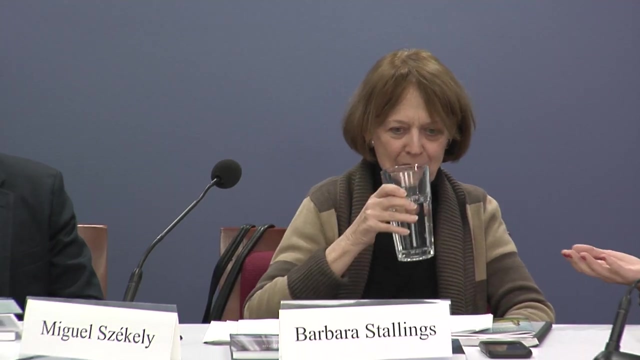 Does tax policy need to be on the table And if so, what kinds of tax policies might we think about? And does this book help us to think about some of those? Yeah, and apparently it's becoming not a taboo at all. At the last meeting of the IMF. 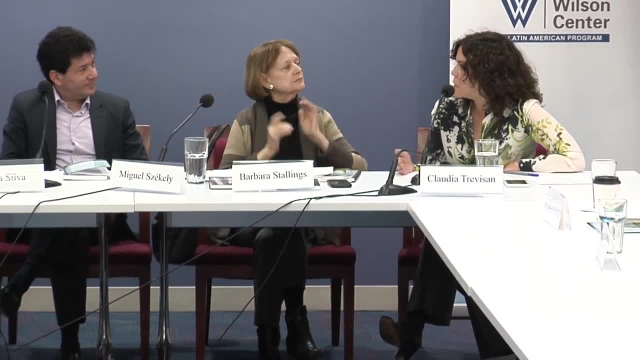 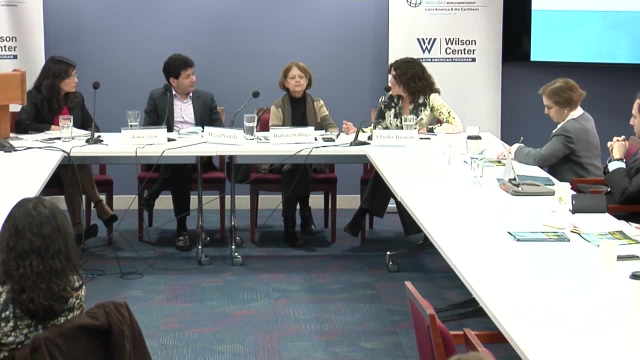 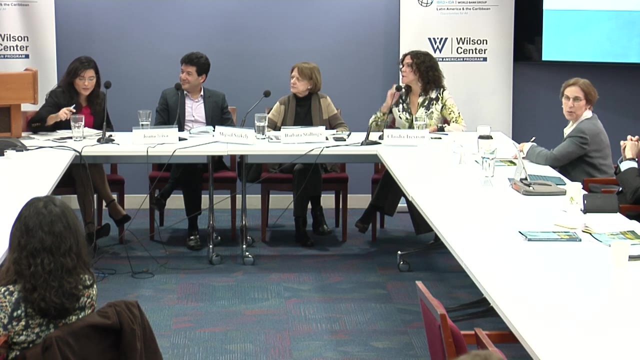 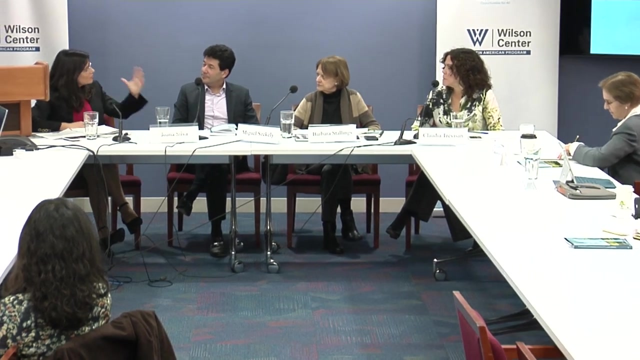 the fiscal monitor of the IMF focused a lot on education, and the proposal that they brought was exactly to increase taxation on the rich. So is that an efficient tool? So thank you very much. I'm really excited about this discussion. Just a bit rounding now. 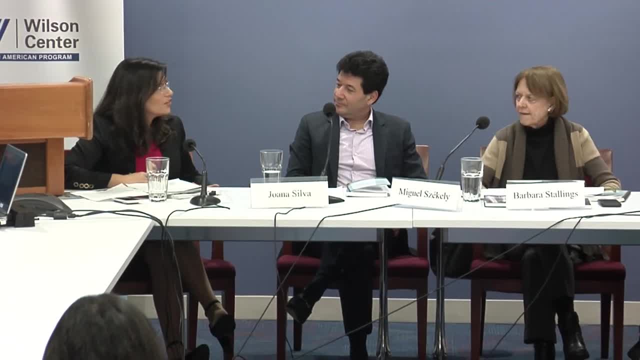 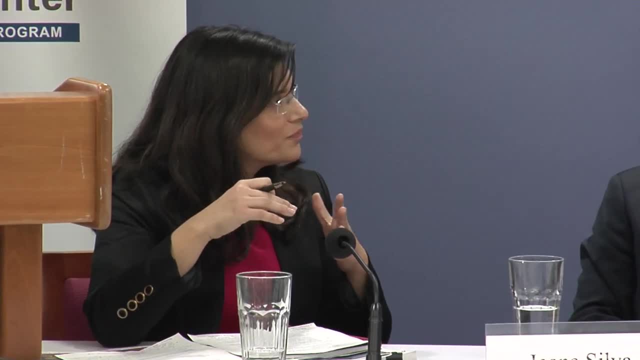 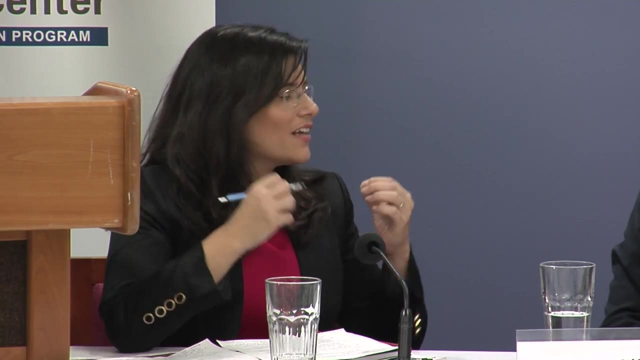 some aspects that you were mentioning. This big expansion of education was really something important because it has long-lasting effects and is likely to continue, But it was also accompanied by economic growth. But let me pause for a moment and celebrate a bit again. So, in terms of thesis scores, 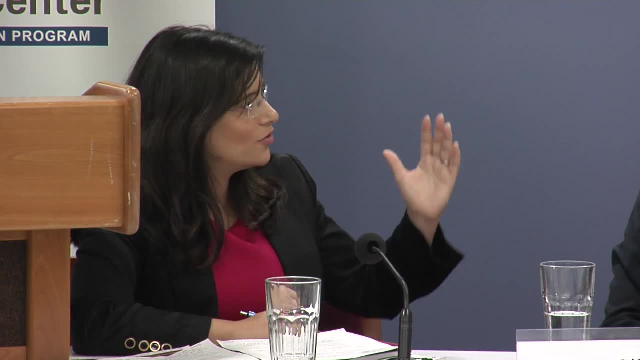 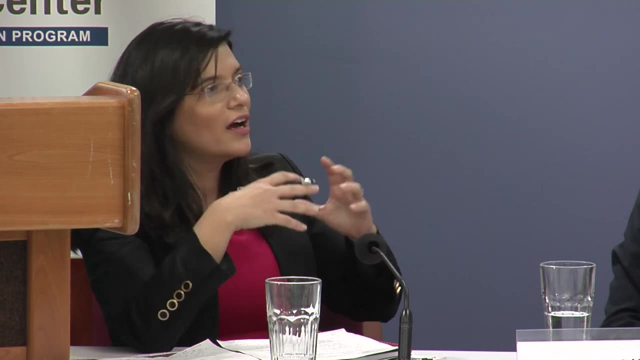 one would like to be in a higher level, but the trend, like Miguel said, was encouraging. As you expand a lot education and you have a higher level and a broader set of students in education systems, you expect the thesis scores to go down. 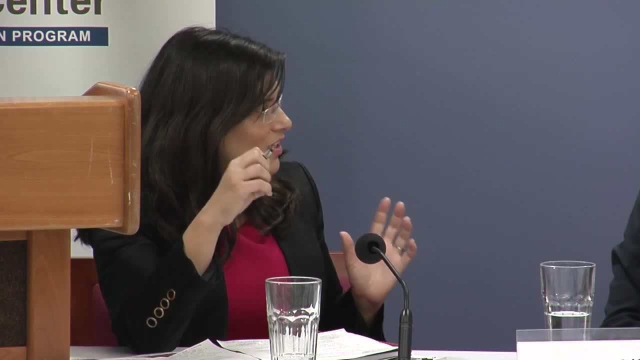 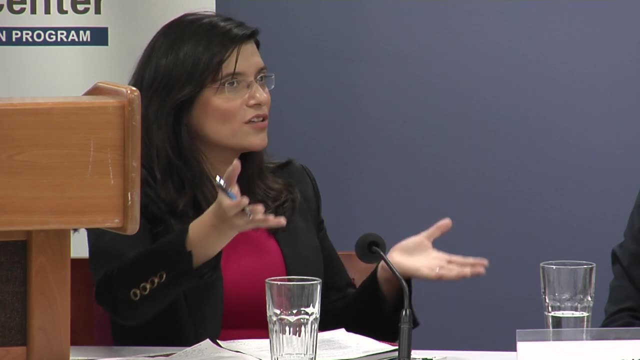 And in fact in the region they remain stable or even increasing. So this is something to celebrate And it did contribute to increase to the fall on wage inequality, which was accompanied by increase of wages at the bottom. that improved life of many. 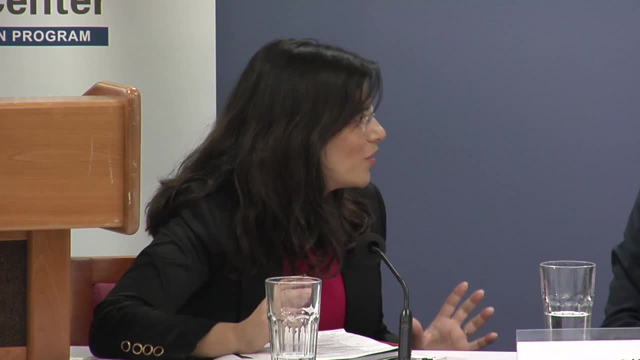 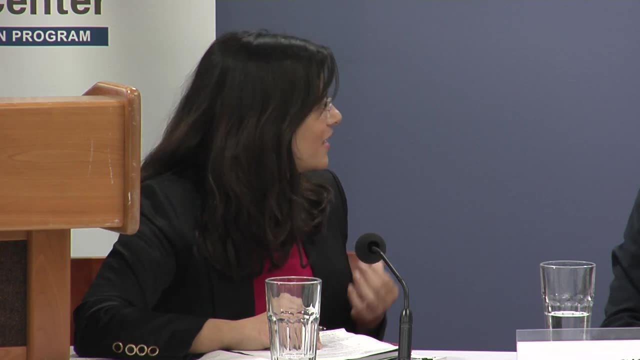 So let's, But we are definitely not where we want to be. And now we stand at the crossroads, like a study we have on higher education. Now it's time to look at quality issues, So people create skills that translate into higher labour market productivity. 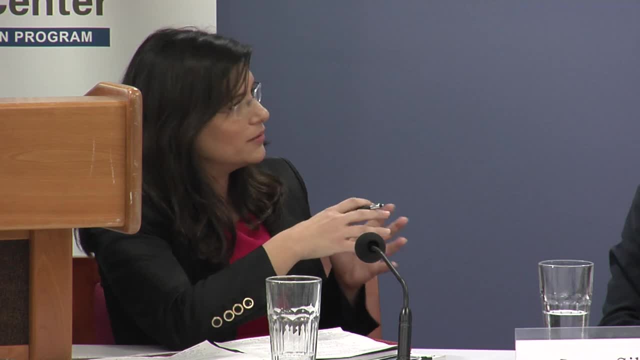 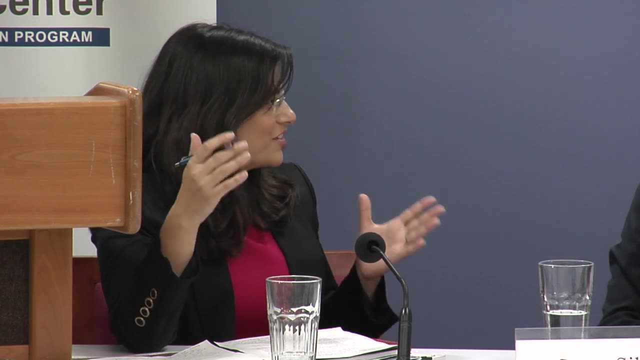 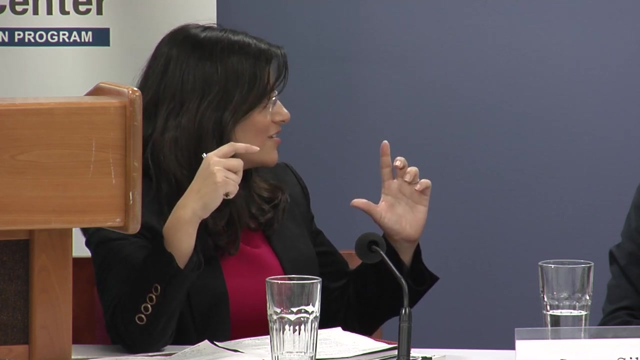 So now on the issue of sustainability, The slower growth and its different pattern are definitely likely to affect wage inequality. through this different, through the fact that now we are in a context of real exchange rate depreciation, And this affects exporting firms and makes wages insufficient. 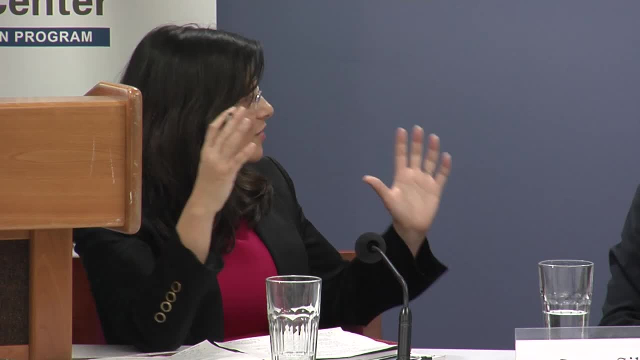 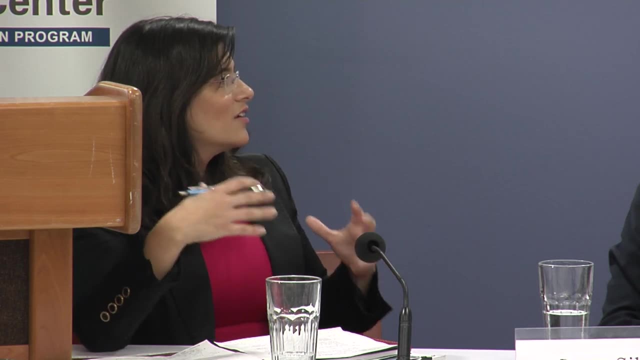 So we need to make the tradeable sector more equal across firms and expand the tradeable sector that is more heterogeneous, And this is a fact. So what we say is that, given this fact, you need to work extra hard. It's not enough to do what you were doing. 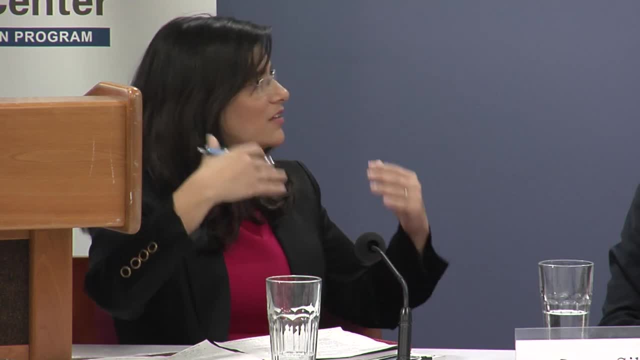 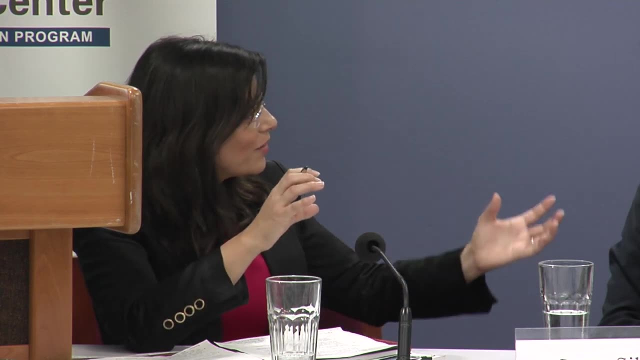 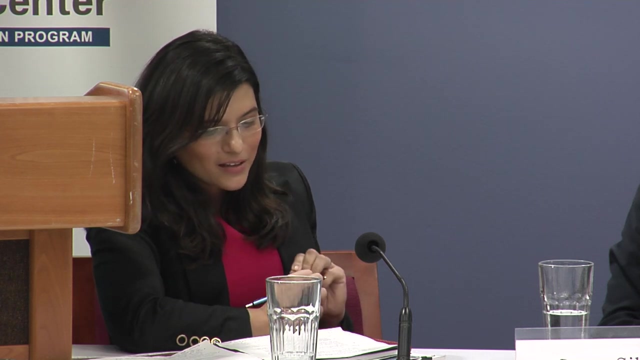 And even if you do what you were doing extra hard, you might not reach exactly the same levels because you don't have this complementary key factor. like Barbara was saying, that is necessary also for the pattern that we observe Now, just on the issue of the data. 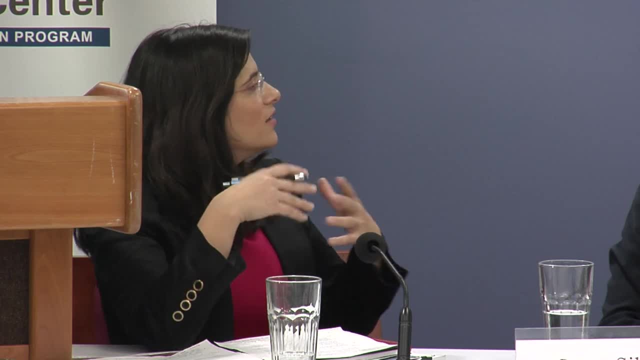 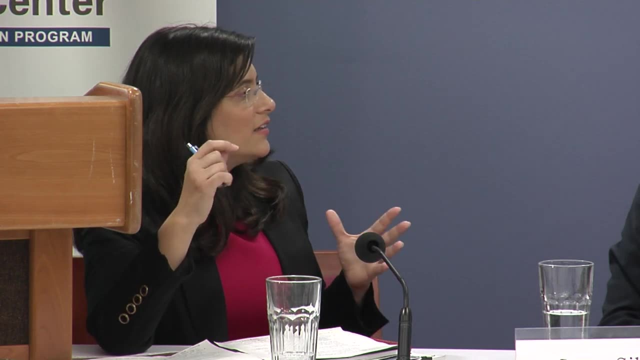 So we use here household survey data because that's the data that is available for a larger period of time and for more countries. But it's a fact, like Barbara is saying, that it doesn't cover well the top 1% of the society. 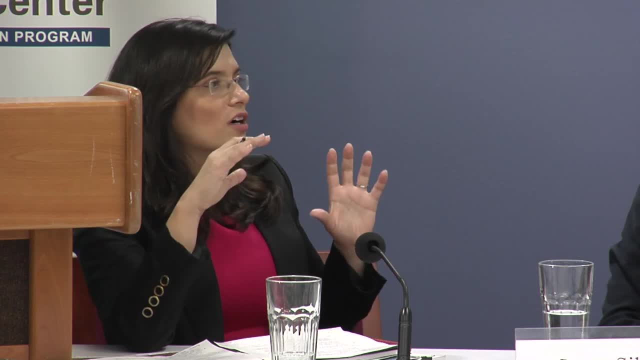 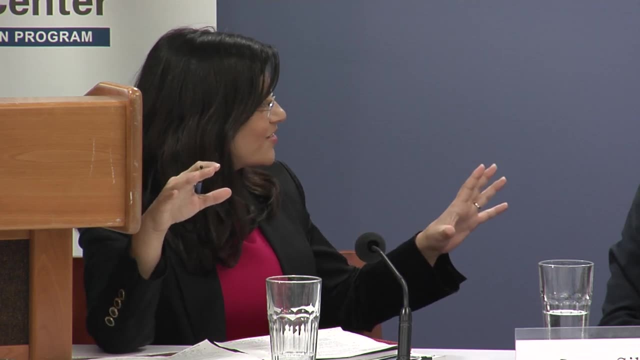 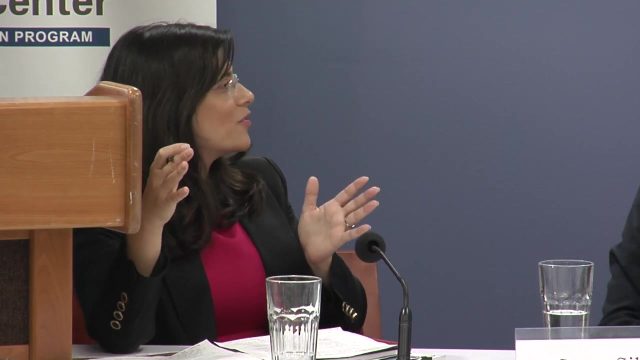 And it doesn't cover well gains of capital or rent. Here, because we are focused on wage inequality, we have somehow less of a problem because wages tend to be more dispersed in the society, So we are likely to be capturing well the remaining 99% of the economy. 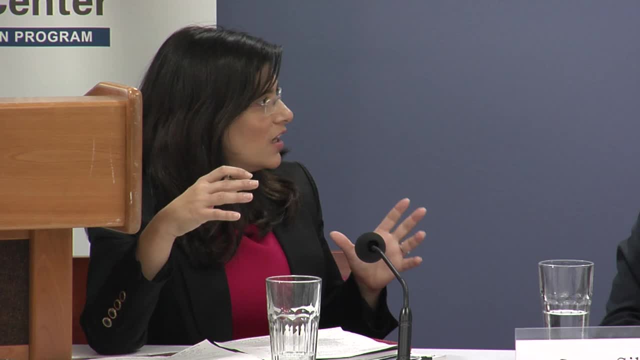 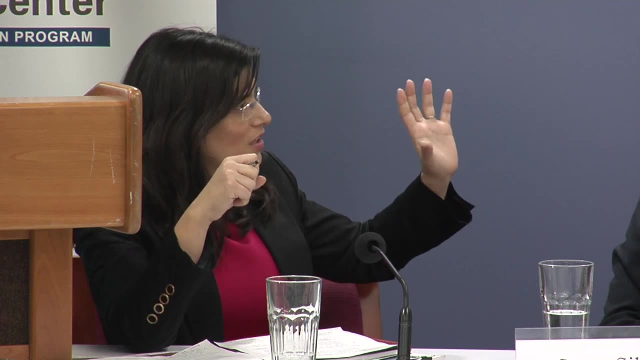 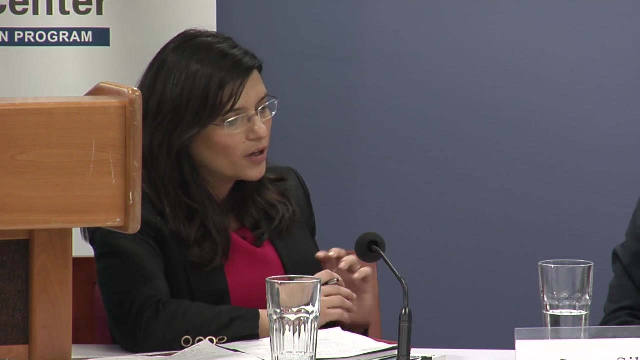 And we are using a measure that is Gini coefficient, And this measure is different from Piketty's that uses the level of concentration of income in the top of the earnings distribution. So this is why we have different results on inequality, And what you were saying, Barbara, is true. 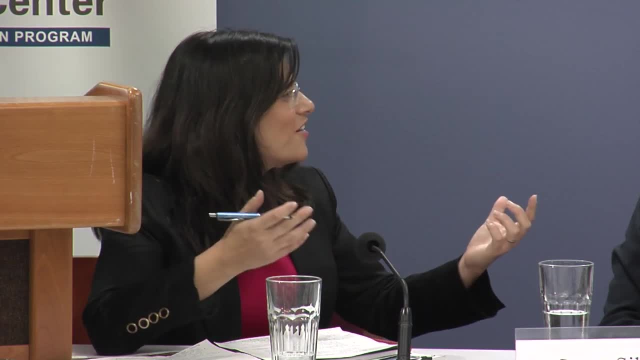 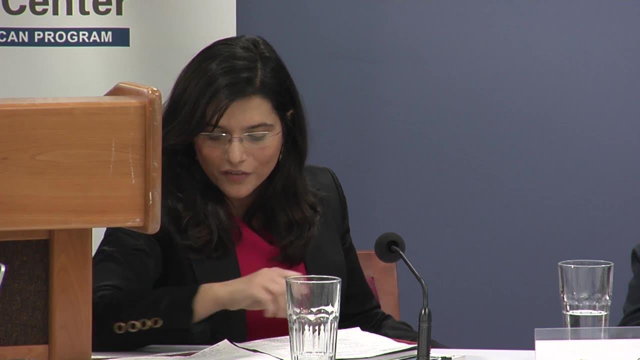 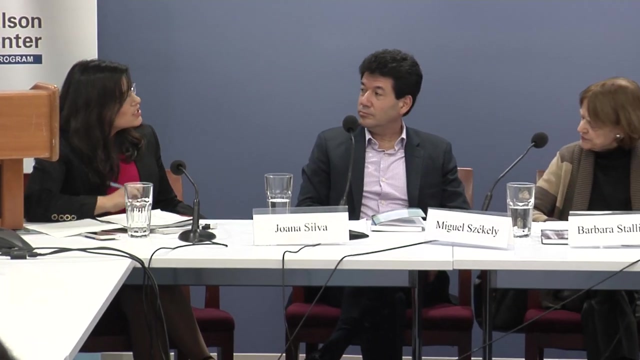 No instrument is perfect. Ideally, we would like to complement the household surveys with tax records, et cetera, to get a better understanding of the top of the distribution. Is there any trend toward more tax information availability in Latin America? Did you know that? 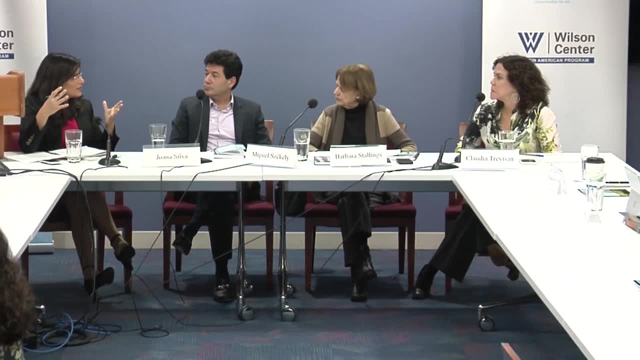 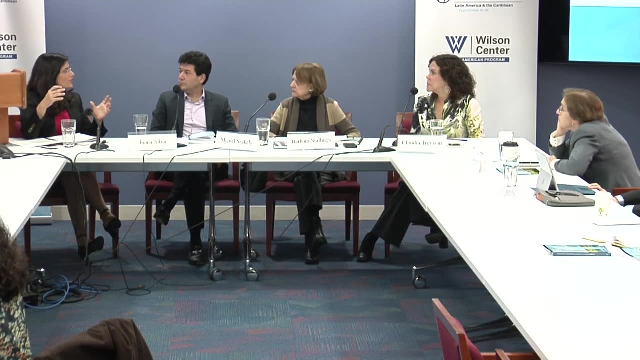 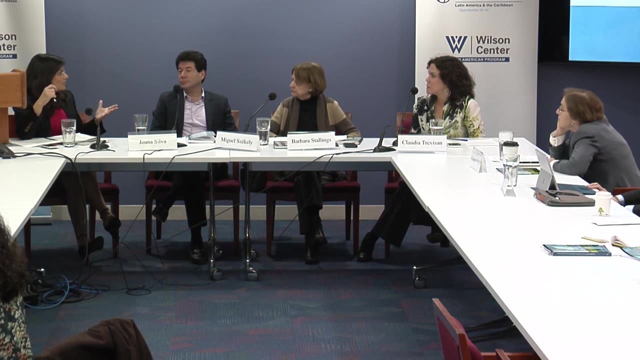 So tax records are available in many countries in Latin America, but they are not publicly available as often. They are more available now than they used to be And we had a study where we had more information on Colombia about the top 1% In theory by increasing the tax rate. 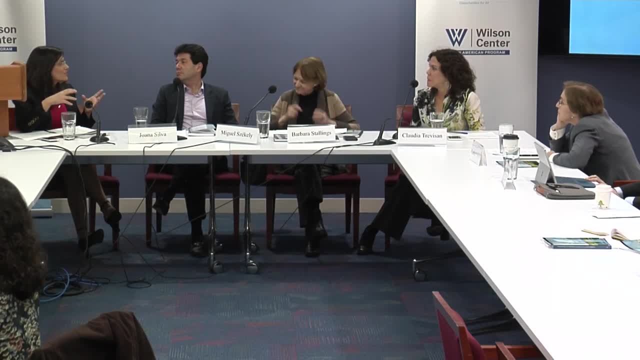 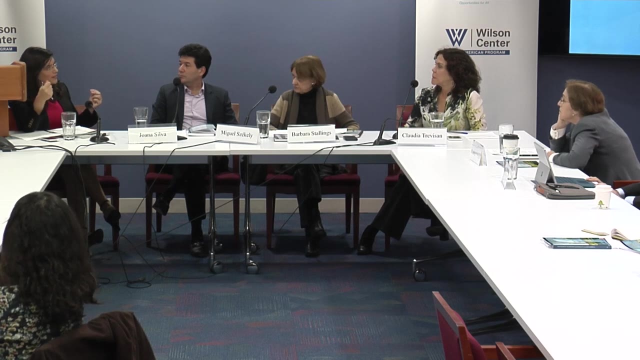 you would increase tax collection, But given the high levels of informality in Latin America, this is not guaranteed And some think that maybe we should operate in the tax rate that maximizes revenue and then use the spending to work on inequality. So these are very interesting topics. 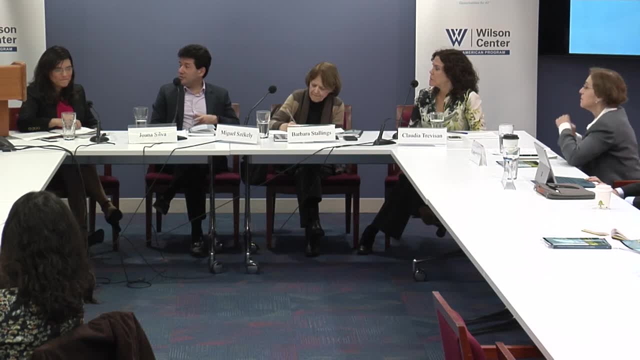 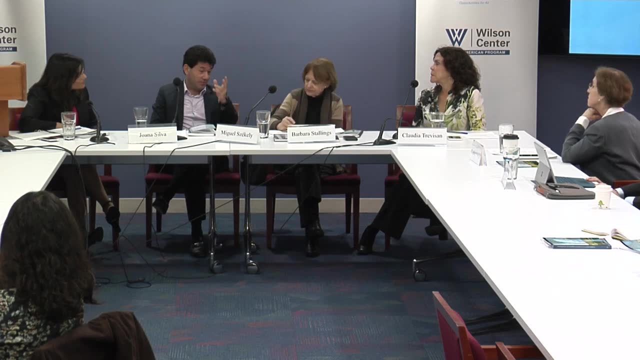 but difficult ones, no. And actually the tax records, since they cover the formal sector. the problem is that they leave out a big part of the economy, And part of it is at the very top. Yes, And considering the fact that, as Miguel mentioned, 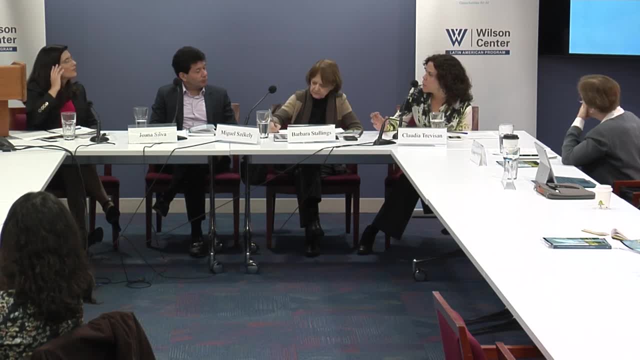 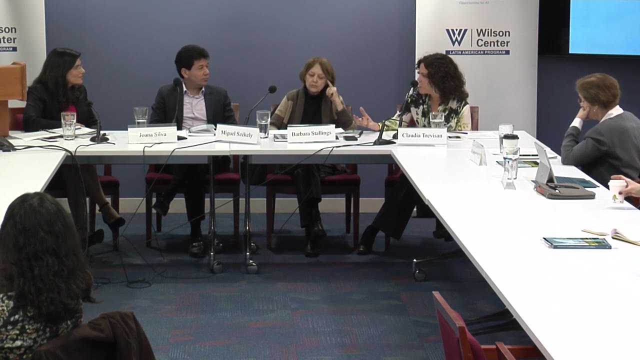 some of the key elements were related to the commodity bonds: the exchange rate, the increase in domestic demand. can this be replicated in countries that don't have, don't experience a commodity bond, have a different situation from Latin America? Is it possible? 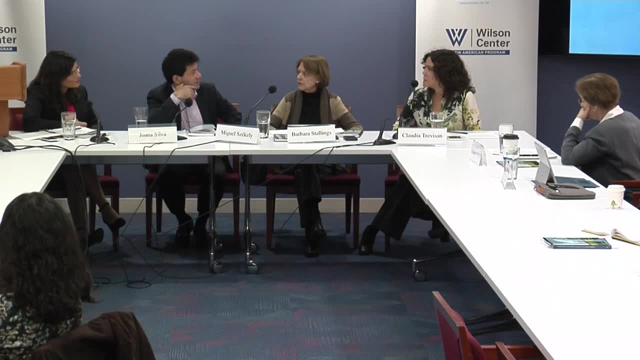 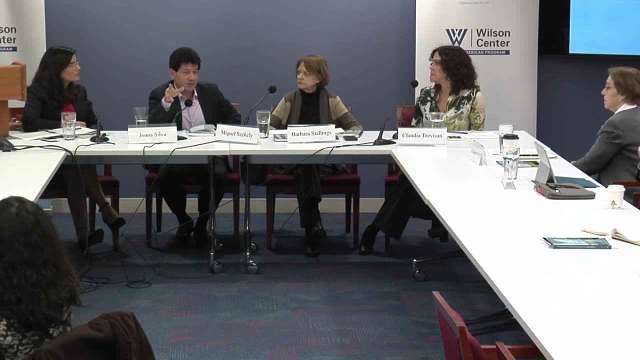 I think that that's the problem, that I don't think it is. It is more of an external factor that doesn't have to do with what the country does as policy In several Central American countries, for example. I think it is very illustrative. 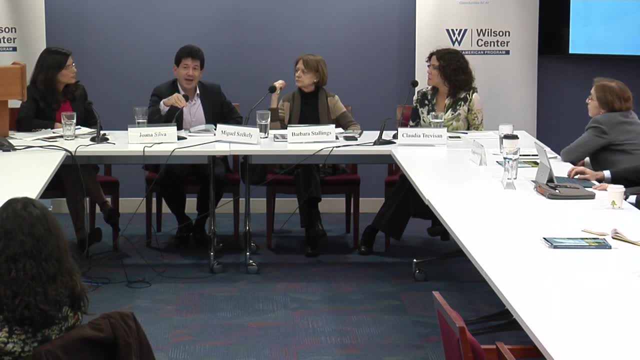 you have a certain stock of education and distribution of education, and then you have the prices paid for performing certain activities, the returns to education, And what happened, I think, and that explains a big part of that story, is that the prices changed very dramatically. 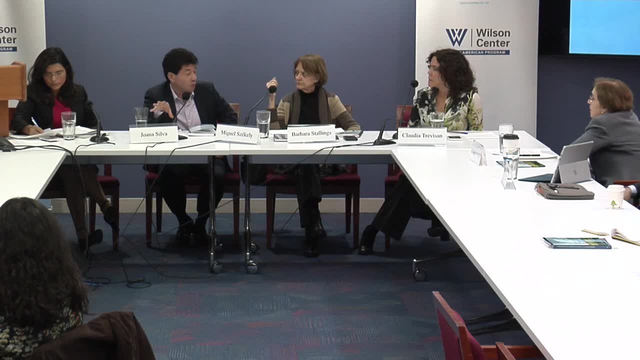 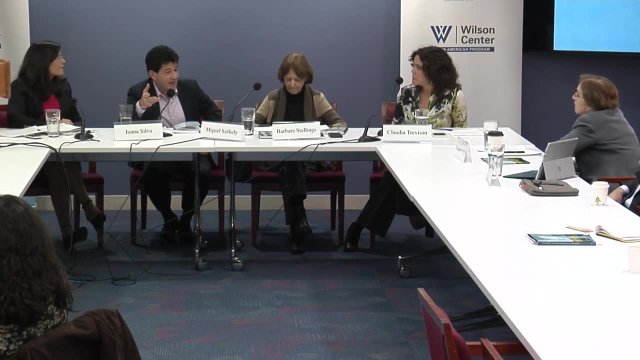 because there was a huge demand suddenly for goods produced with low-skilled labor, Exactly as Barbara was mentioning. this is totally opposite to the expectation. that was that inequality would decline because you would increase the stock of education, of human capital. Here what happened is the stock remained fairly stable. 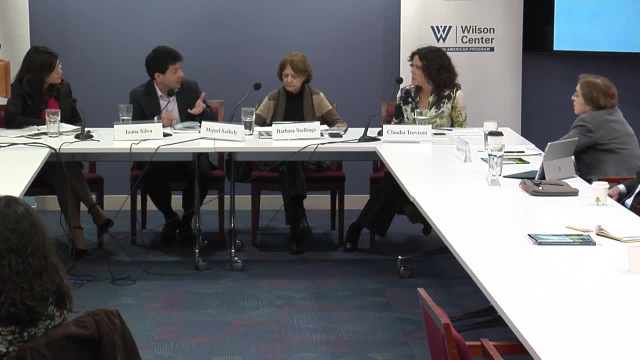 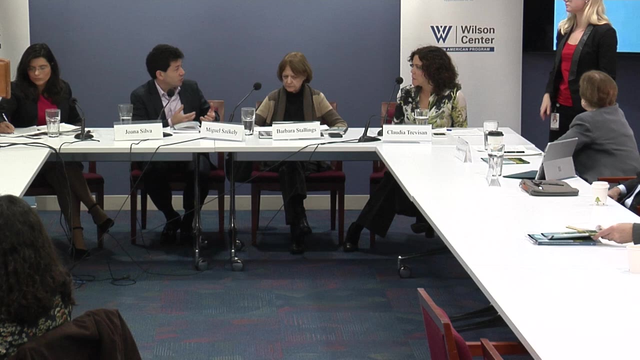 but suddenly the rewards to the lowest skills increased due to this external factor Suddenly. if the factor fades away, well, you will stop seeing that trend And if you did not invest the extra resources to improve your education, to really change the structure, 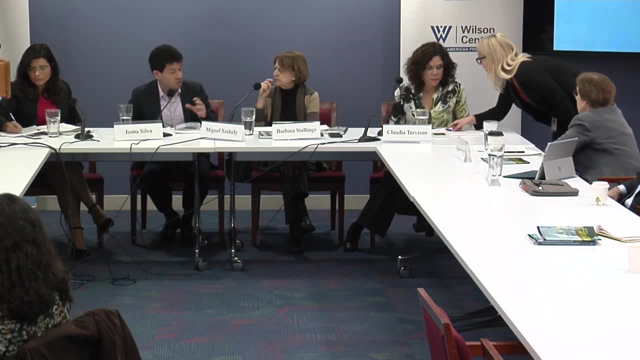 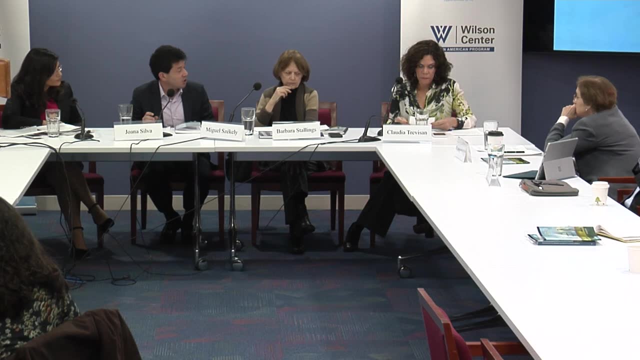 of the production capabilities, then you would be left perhaps in the same situation as before, or with that shock- positive shock. But I think this is not where we would like Latin American countries to go. It would be much better if there was a structural change. 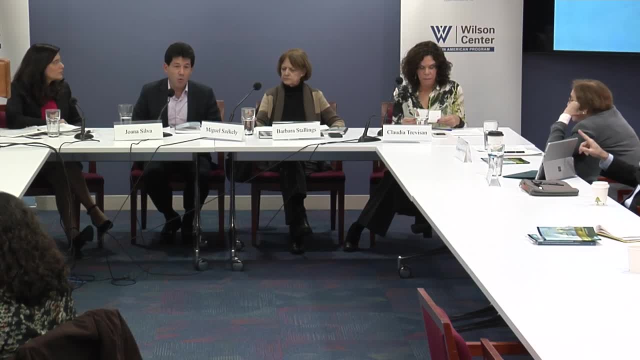 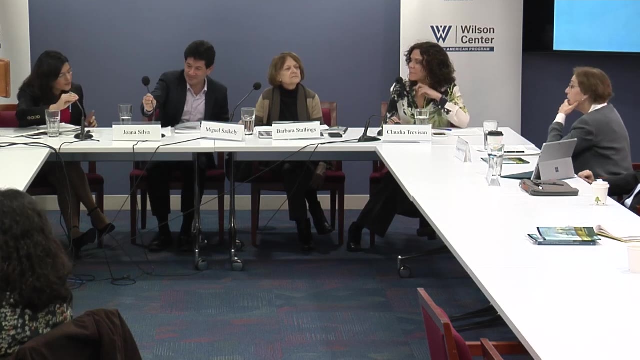 that really led to a different scheme where, more broadly, more people got educated and that education was appropriately rewarded in the labor market. That's for me, Let me just add to Miguel. So I think it depends on the country where you are. 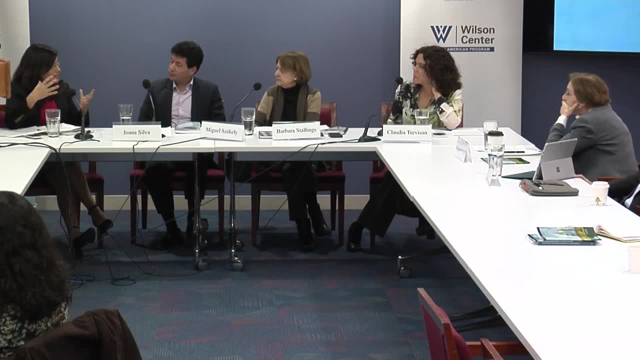 So in countries with very low levels of education, where access there are still important bottlenecks in access, education can have this positive effect of reducing wage inequality. This happens in low-income countries, for example, and there, if this is an issue, 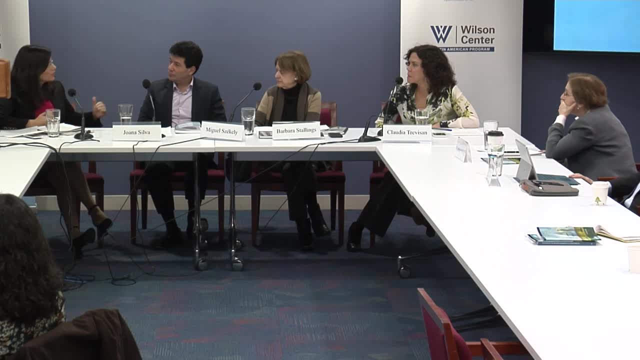 removing these bottlenecks can have a positive effect through the effect on returns to education. In high-income countries, though, this step was already made and progress now is through quality, So the extent to which it's replicable depends a lot on the level of development of the country. 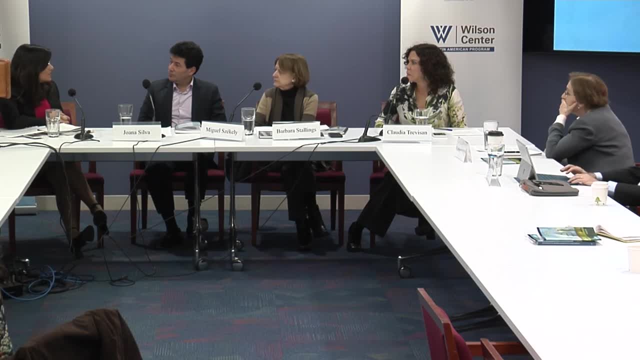 in this part of education, And I think this is something that is important to notice, And also this point that a lot of the effects occur through more equal wages across firms and the driving force, the real exchange rate appreciations. this is also something that can occur in other contexts. 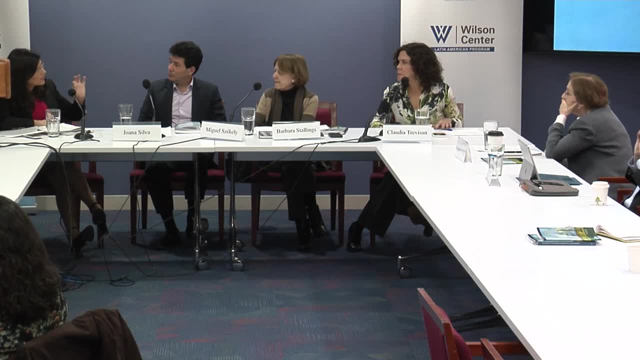 and can have similar effects. And just a point on this. a last point: Returns on education fell in Latin America, but today a person with college education on average makes 3.4 times more than a person with primary education, So it doesn't mean that he no longer pays to go to college. 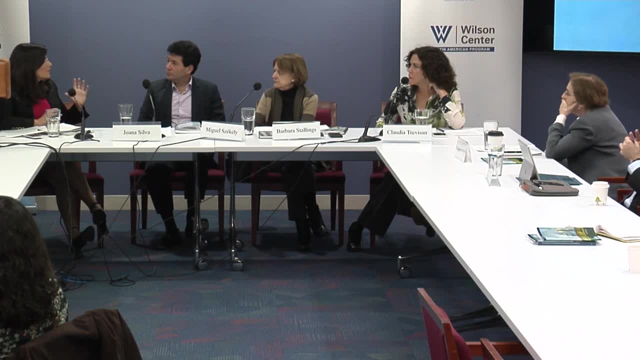 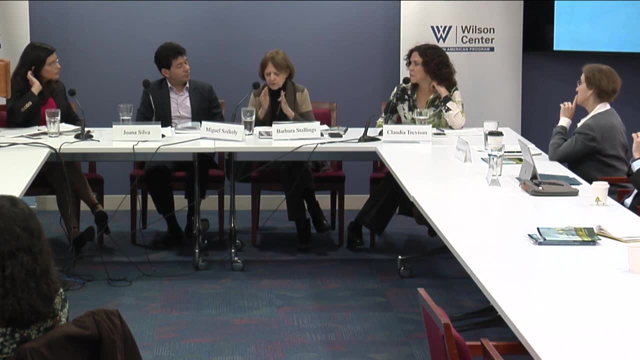 It does mean it does pay. It just pays less from a very high level, higher than any OECD country. Going back to the contrast between South America and Mexico, Central America- in the high-growth period, I really think that one could make more use. 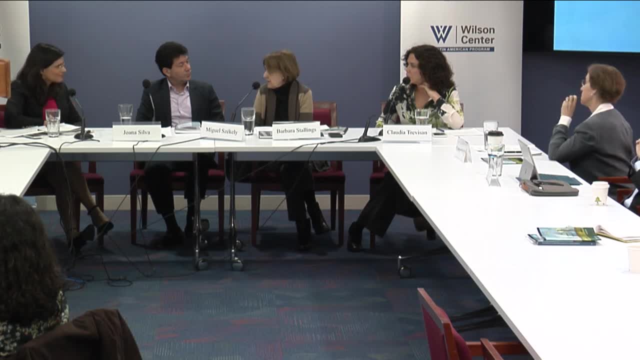 than is made in the book of this distinction. I mean, the South American case is so dramatic that we tend to concentrate on that, including myself. If we did some more work on Mexico, where you say that, yes, inequality was going down. 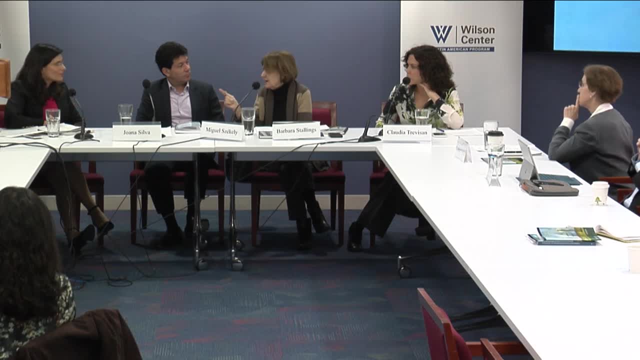 even though there was not only not a commodity boom, Mexico and Central America were hurt by China, were hurt by China. They were not helped. Therefore, if we spent some more time trying to tease out what was going on in Mexico- we used to call it in when I was at ECLAC- 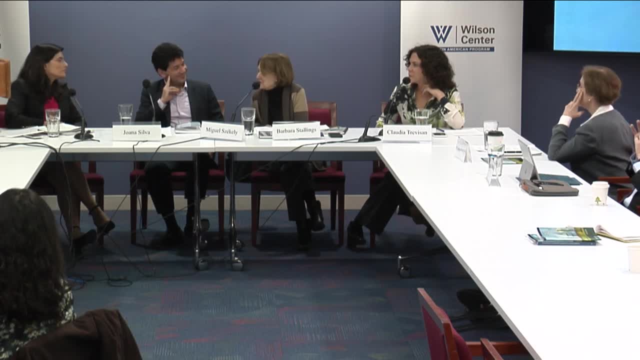 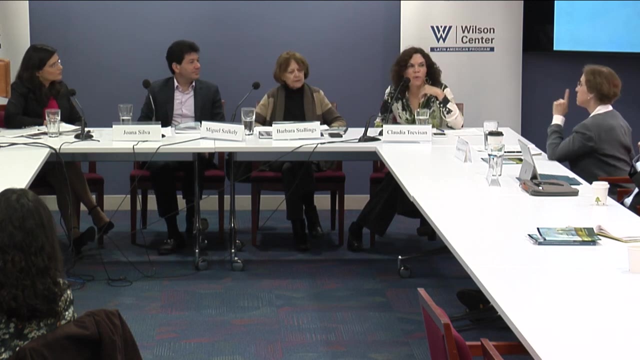 North of Panama and South of Panama, trying to figure out what was going on north of Panama during this decade. maybe that would give us some clues as to how to keep this positive trend going without a commodity boom. Well, let's open to questions. 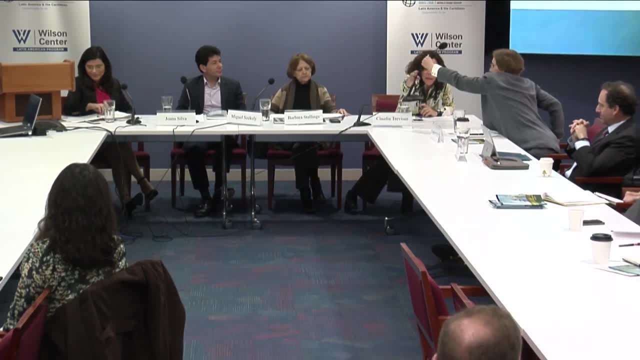 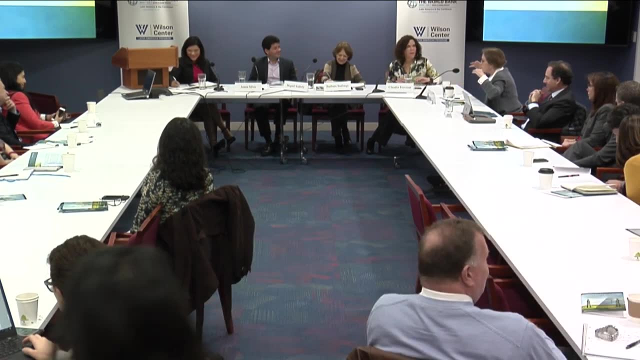 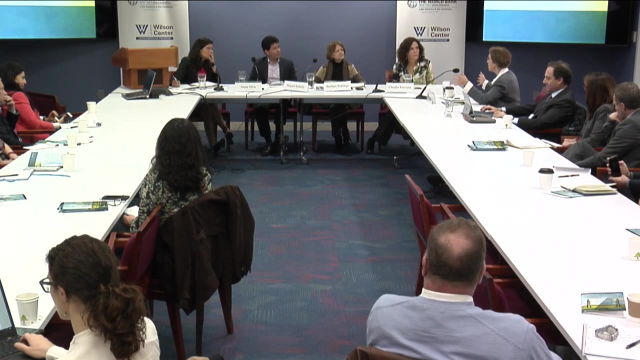 and Cynthia has one here. Thank you to all of you. I have a really burning question, until I'm just sort of jumping out of my skin to ask. What's really remarkable to me is: we've heard these wonderful presentations. Not one person has mentioned conditional cash transfers. 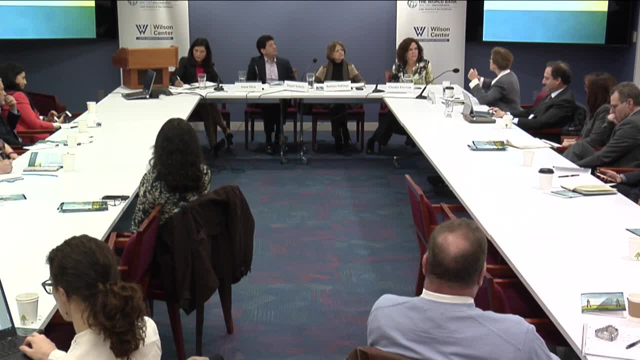 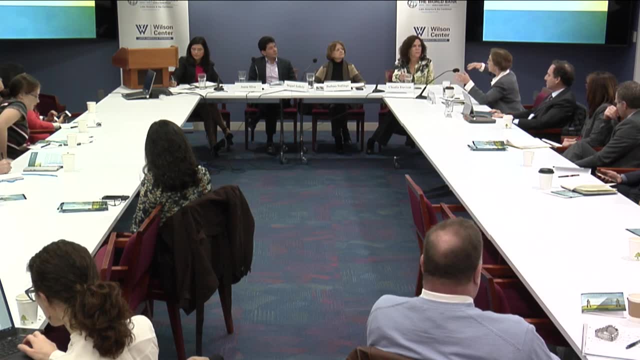 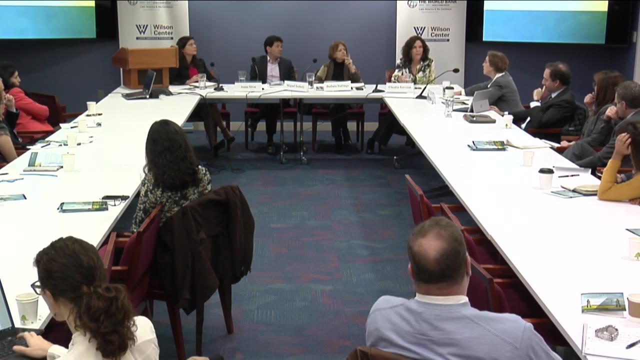 Not one, And maybe the reason for that is that the transfers were intended to increase access to education, so that you're sort of skipping over the conditional cash transfers and looking at the effect, which was, you know, greater participation in the education system. 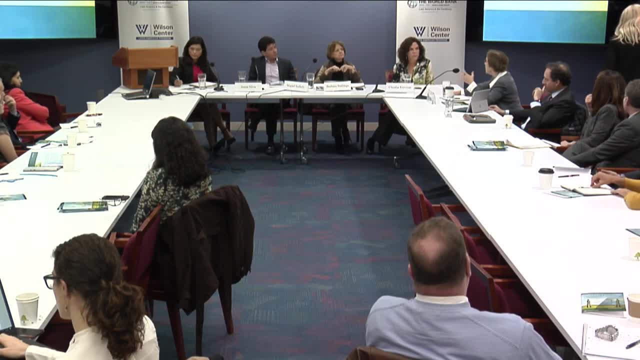 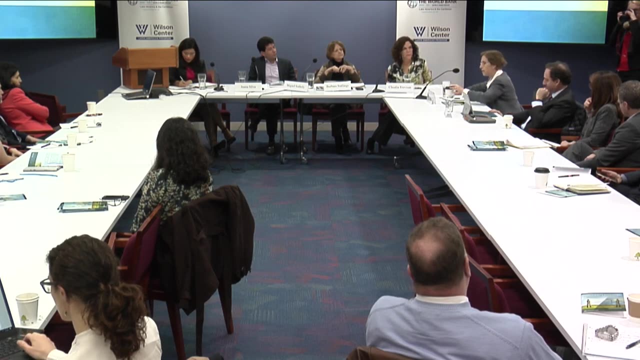 But I remember several years ago that one of the main explanations for the decline in inequality was not only the growth rates but the state policies that put money in the hands of poor people. So that's one question. Another question Danielle and I were sort of chatting about. 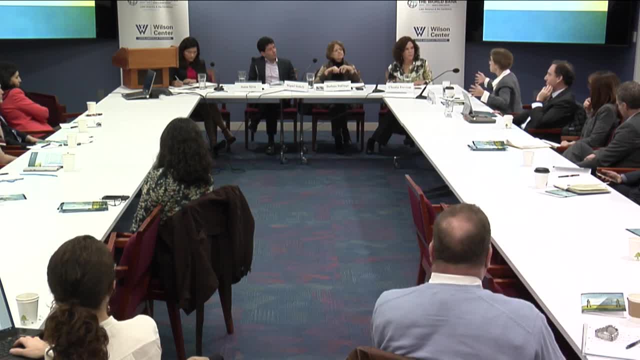 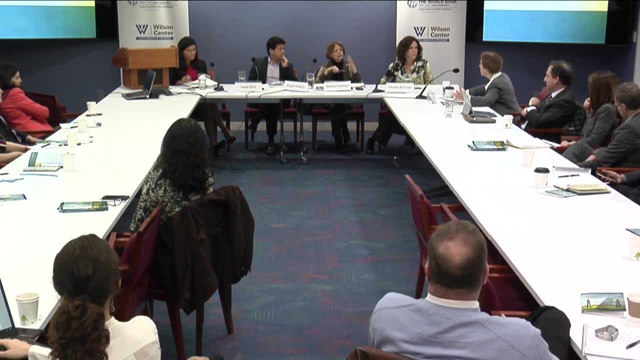 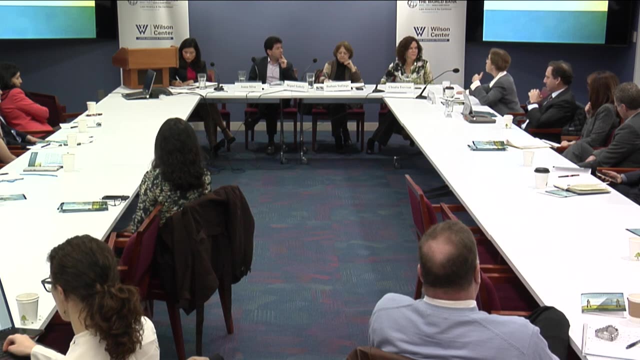 the difference between the debate now in the United States over tax reform and levels of inequality and the debate in Latin America. Why do we care about inequality? What is the issue, aside from the moral issue? I mean, this is sort of a devil's advocate question. 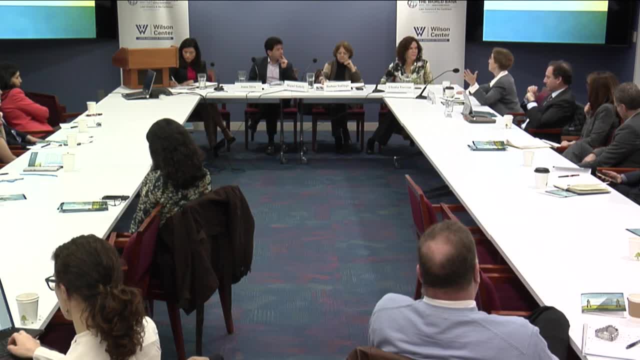 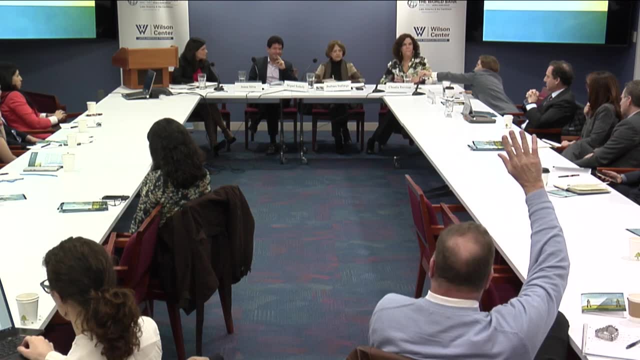 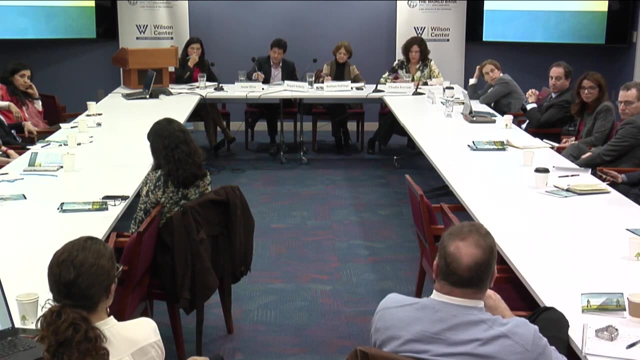 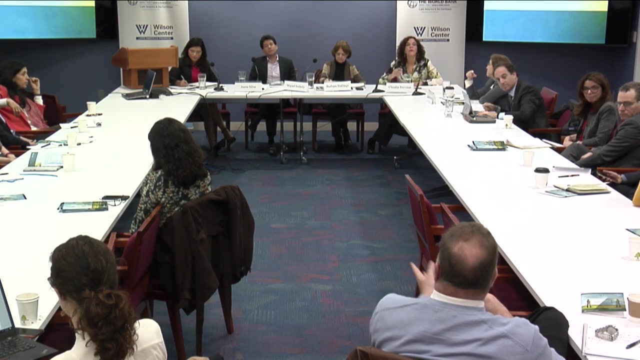 Why do we care that societies are unequal? Do you want to collect some questions? and then There's a microphone there. Thank you, Very interesting discussion, But I've got a real concern about: Can you identify yourself please? Oh yes. 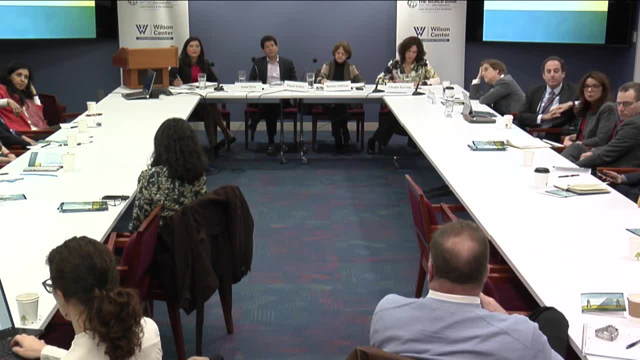 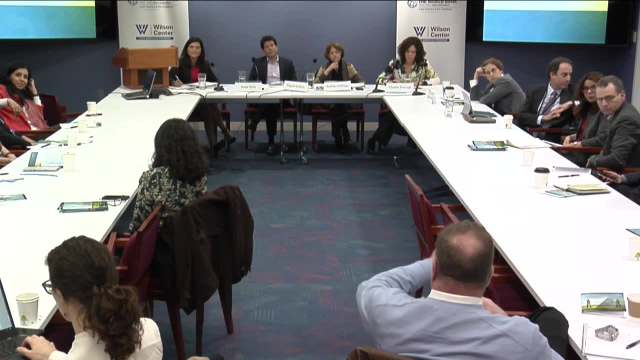 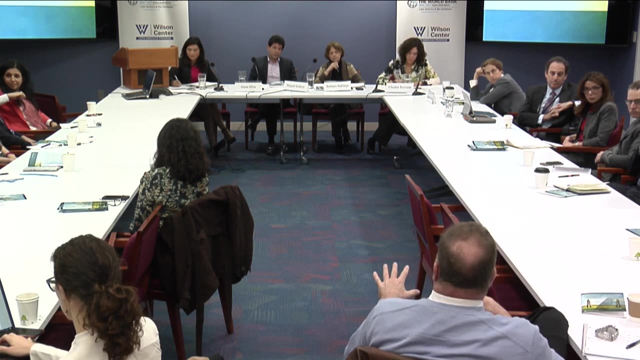 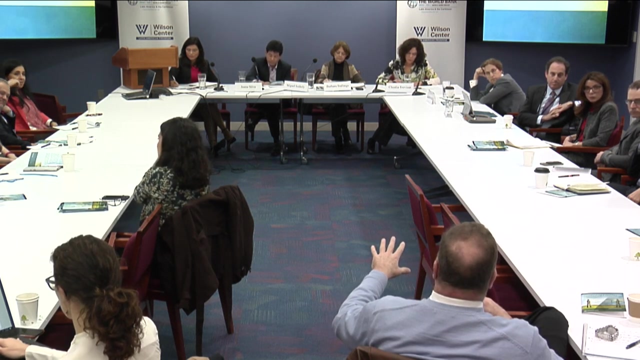 I'm Chris Gruy, Department of Treasury. There's another stylistic fact that you did not mention as you were laying out the context, which is the lack of growth and productivity And, during this boom period with the commodities productivity in Latin America. 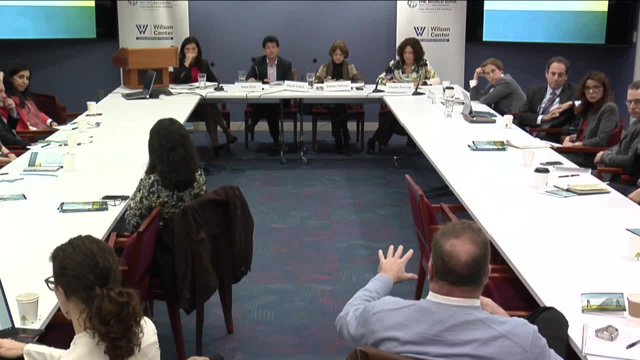 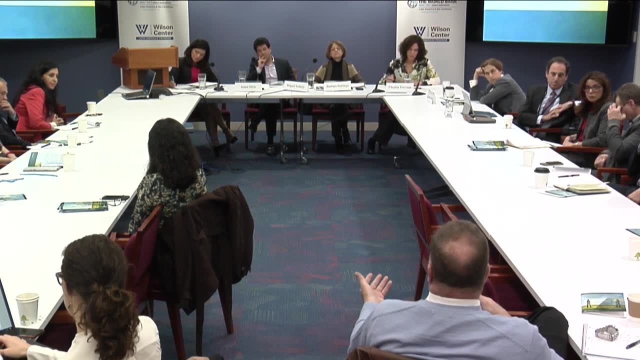 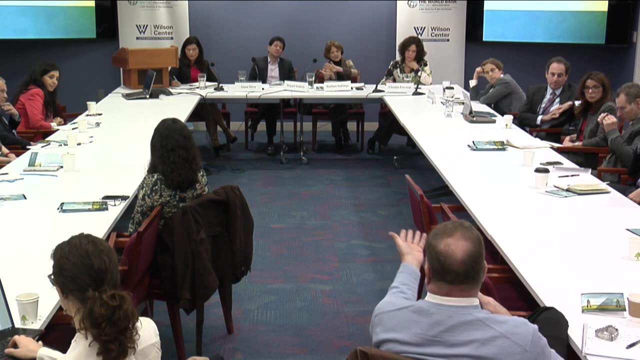 as I've seen it in the statistics, was essentially flat. It barely grew at all, which raises the question then: was the increase in low-skill wages during this period just a redistribution, or was it- And this goes to Cynthia's question- 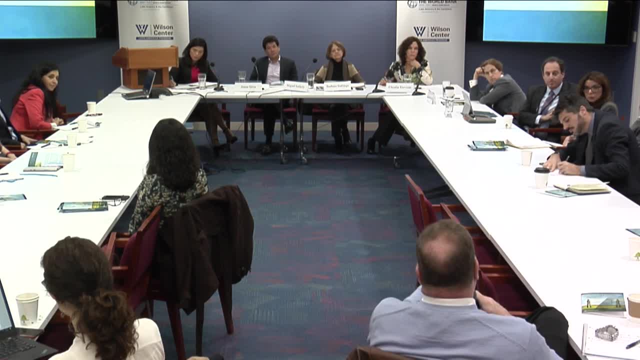 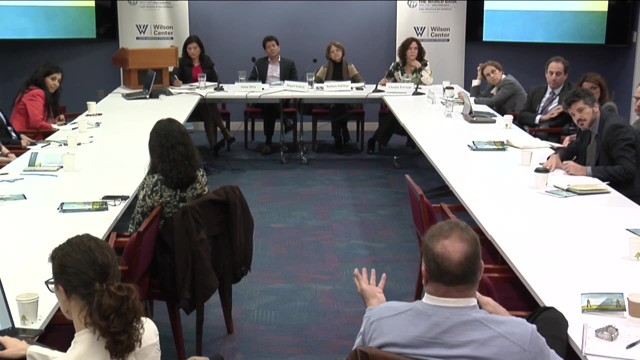 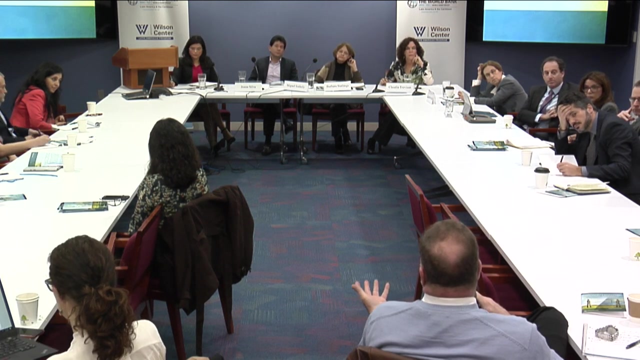 about conditional cash transfers, because I've also seen that same research ascribing the decrease in the Gini coefficient to essentially redistributional policies that governments followed, rather than In the normal labor economics. you get higher wages when you get higher productivity. Better education should lead to. 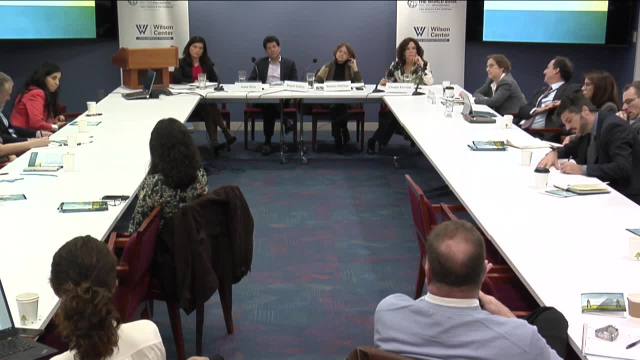 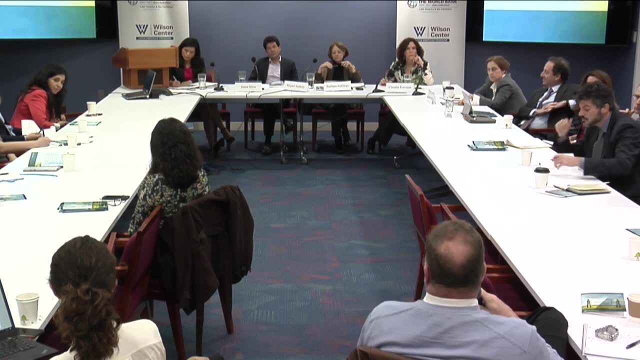 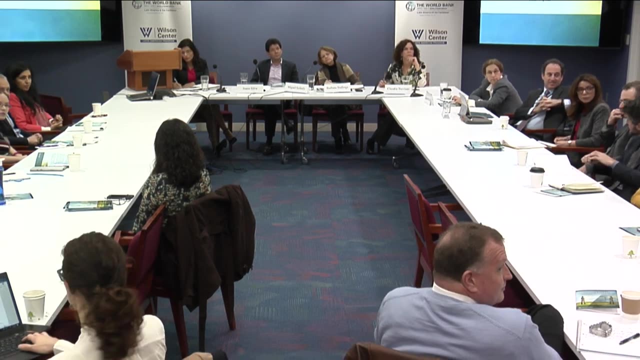 then greater productivity, which leads to higher jobs, Higher wages, But we've got two different stylistic facts that seem to be conflicting with each other. Let's One more question. There is one there. Hi, Good morning. My name is Nicolas Saldeas. 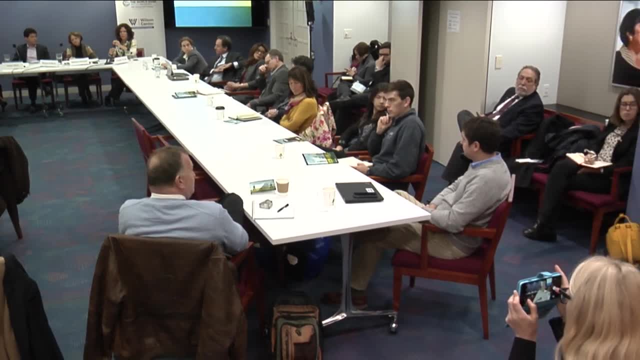 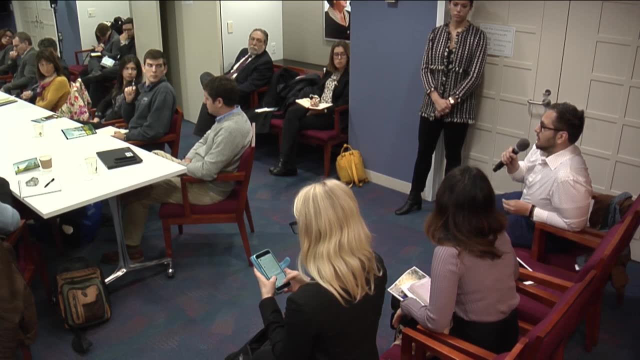 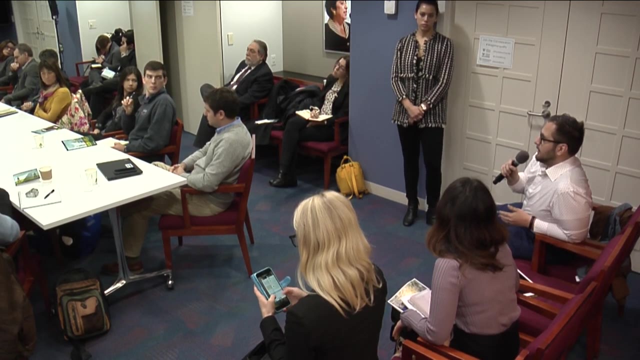 And I have a question regarding labor institutions as well. So you talk about, in South America, a general decline, But if you look at countries like Argentina or Uruguay, one thing you see is that they restarted sector-level collective bargaining, And that would you know. 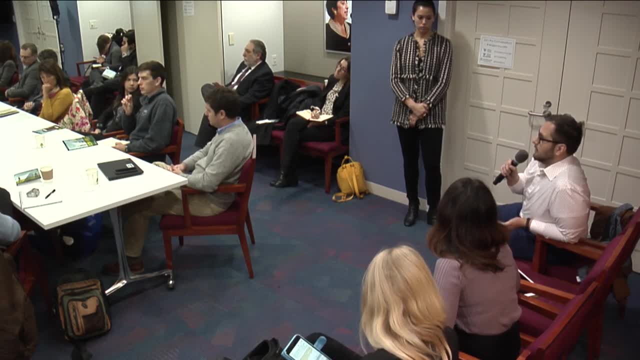 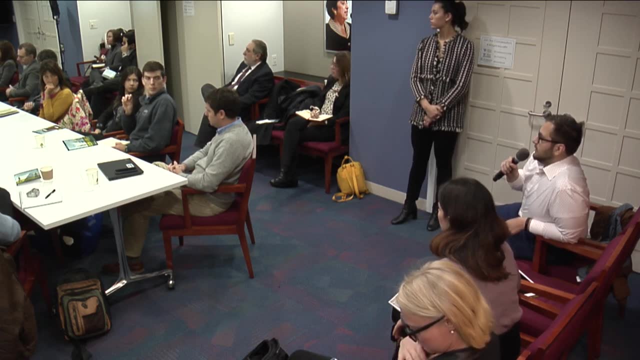 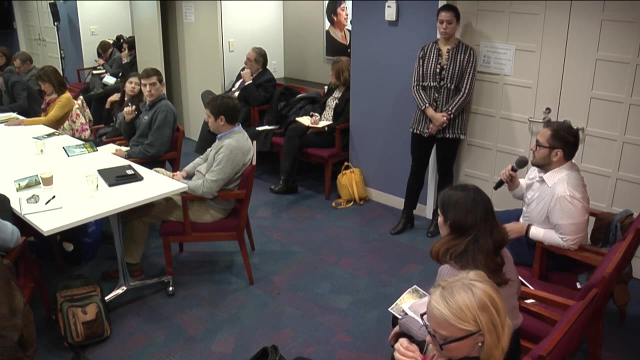 be very Have a very strong influence on one of the variables you discussed, which is the decline in intra-firm inequality in wages. So I'm wondering if you have any data or you have any way of determining the impact of this particular labor institution. 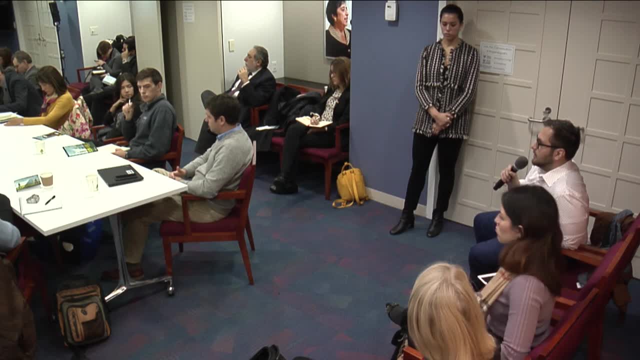 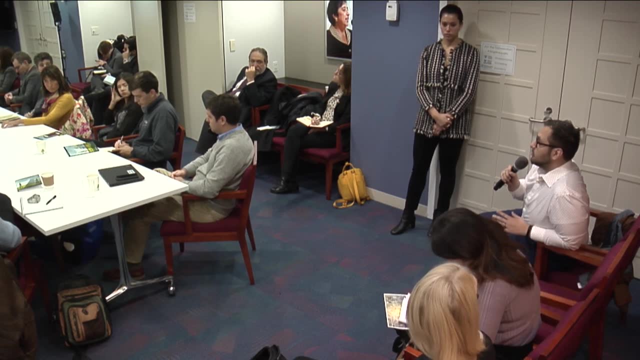 on inequality in these two countries, which are the only ones in the region that have nationwide, nationwide, sector-level collective bargaining, compared to other countries in the region, in South America in particular, that don't That do not have this institution. Well, we have four main topics here. 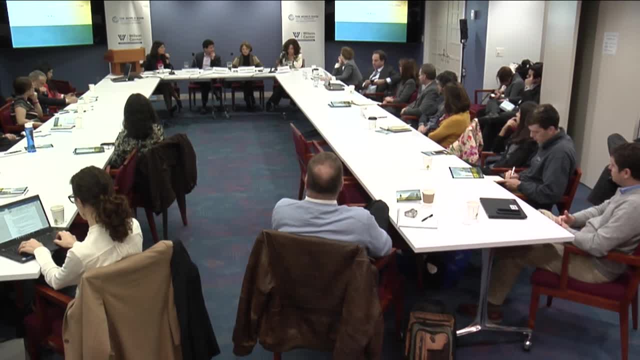 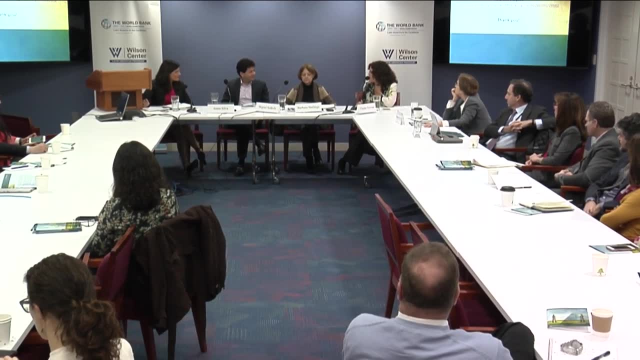 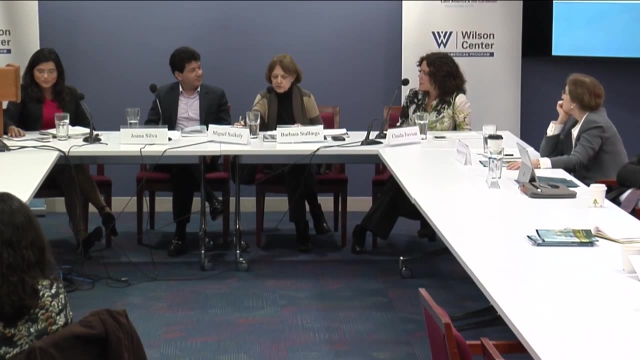 Social transfer. why reducing inequality is important. lack of growth in productivity and labor institutions. Who wants to take the first And which topic, Barbara? Well, I'm far from an expert on conditional cash transfer. I think they work rather differently. 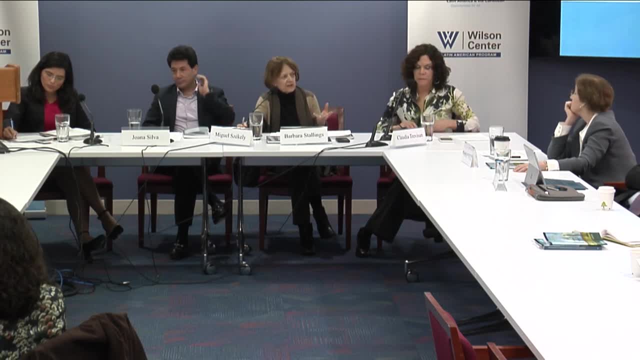 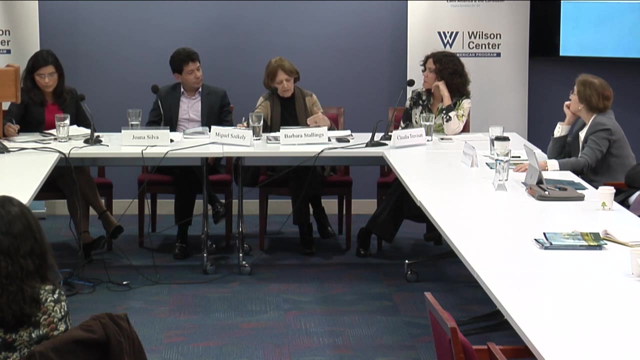 in different countries. Brazil, as I understand, doesn't do conditional at all. They're just cash transfers, but perhaps I'm misinformed on that. But my view was that conditional cash transfers are more useful in terms of reducing poverty than in terms of reducing inequality. 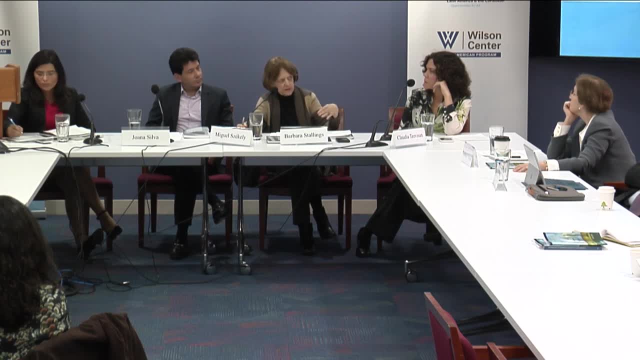 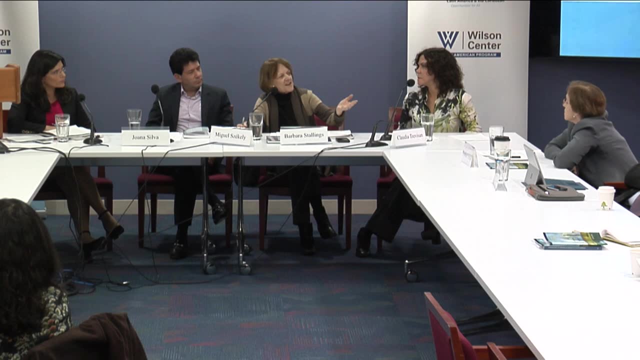 via an education channel, It could be. Again, you wouldn't get. They're talking about ways to reduce inequality. They're talking about wage inequality, So you're not going to get. You're not going to get that in. If you're talking about household inequality, 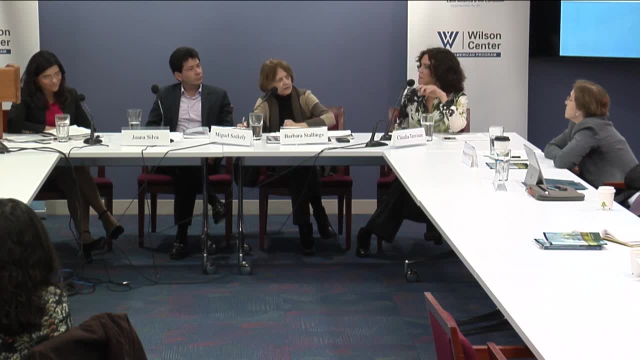 then that could be a factor in helping to reduce household inequality. The education aspect is so much in the future. These are small children. Good for small children to begin to be educated and for their families to realize the importance, but it's a really long-term process. 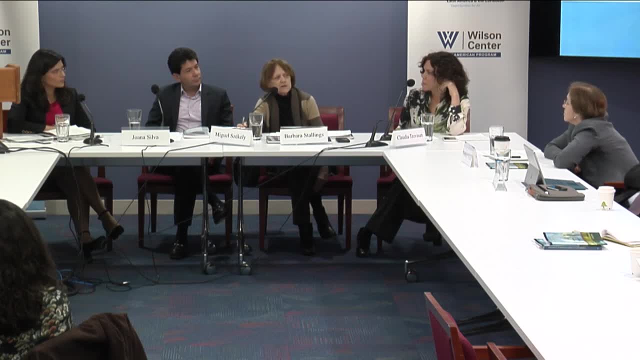 So I don't think that that's likely to have any impact on wage inequality in the particular period that we're talking about. Let me just say something about your other question and then we can take turns answering different questions. Why do we care about inequality? 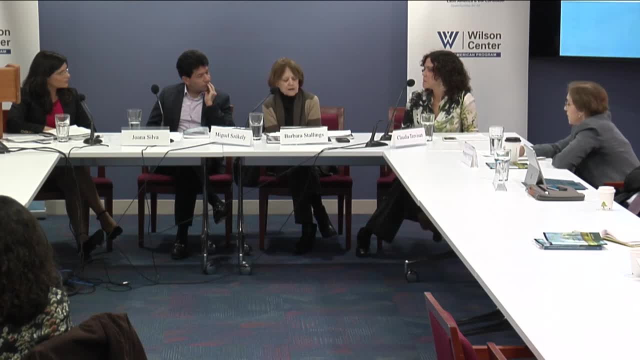 I frankly think we care more about poverty. One of the questions which we had on the list but didn't get it- not surprisingly, we had a long list of questions- has to do with political impact of inequality. There are, by my count, 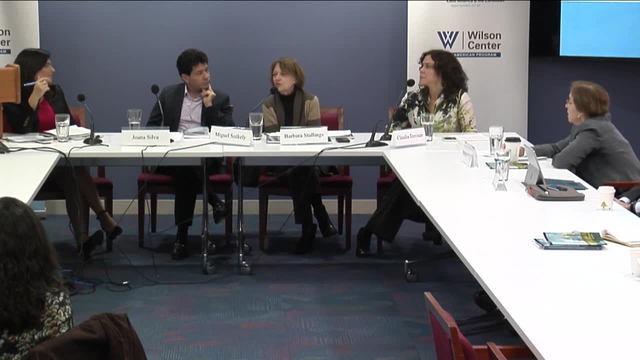 thanks to the Internet, at least seven elections in the next year in Latin America presidential elections. Does inequality have anything to do with politics? in addition to being a moral issue? I think it depends a lot on whether you have the kind of political system. 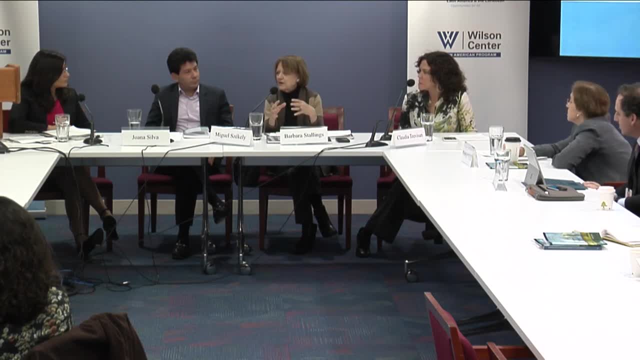 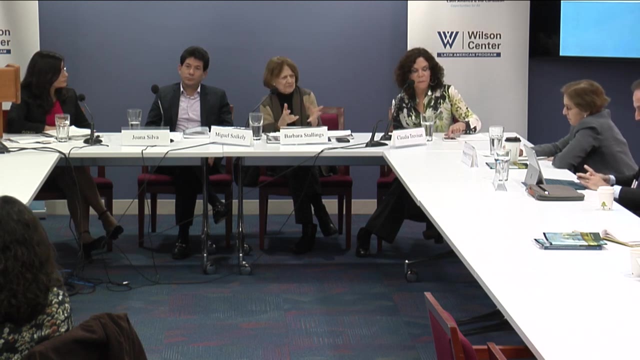 where you have populists on the scene ready to take advantage of anything, including inequality. And in some important countries in the region there are such people and they can make use of inequality, But they can make use of it regardless. I don't know how much, if ever. 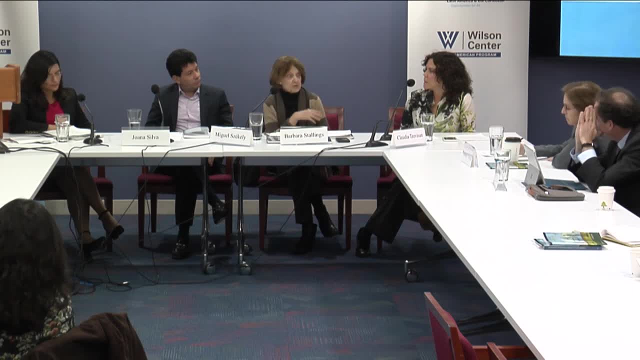 Mr Trump, for example, mentioned inequality. He was certainly talking about poverty and some people being passed over. I don't know if he ever used the word inequality. Maybe it's too dangerous. So one of the reasons one might be, but I think we're less likely to be interested. 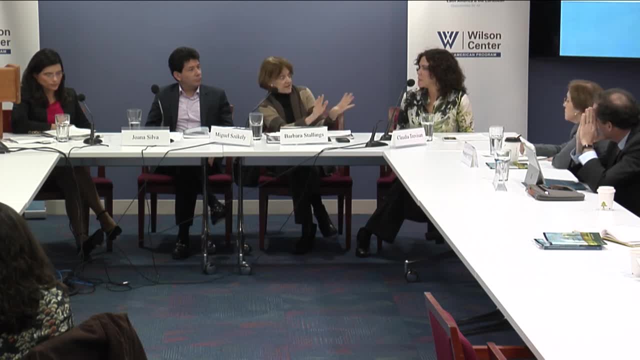 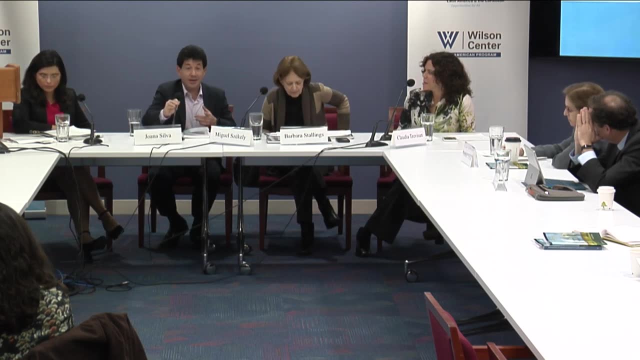 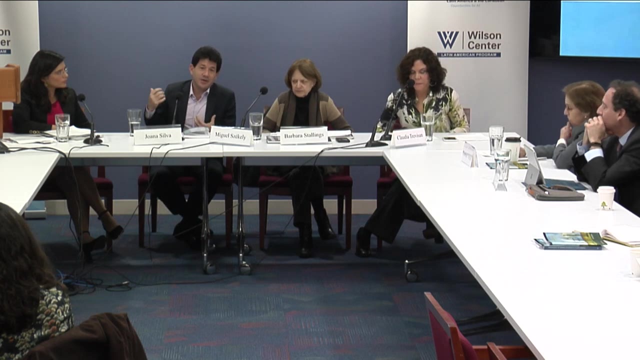 in inequality is for political reasons, But certainly we want to have that in the discussion. Thank you, I think these were very good points. Actually, I think the productivity issue is really at the heart of this discussion and precisely the difference between having these trends. 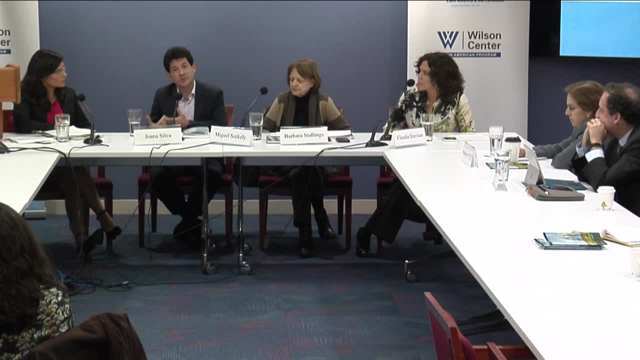 explained by greater productivity at the bottom, versus just a temporary shock on prices, is a key to step next to the policy implications of the analysis. If it's a productivity story, it would go one way and we would go the other if that was the explanation. 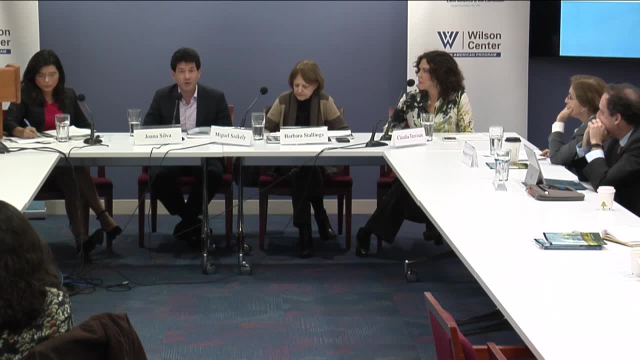 And there is a different story if it was just a temporary price shock. But I think that is a very good point because it reveals in part also the limits of the increase in education, And let me just give an extreme example. that, of course. 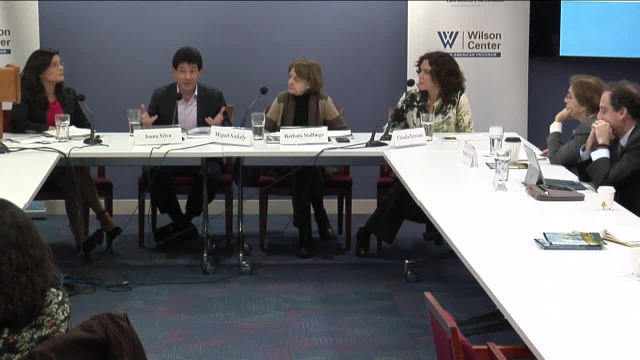 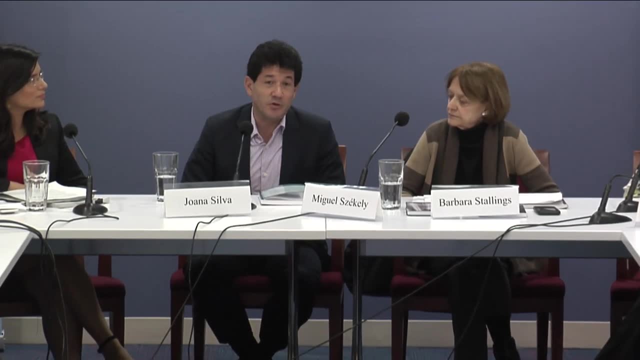 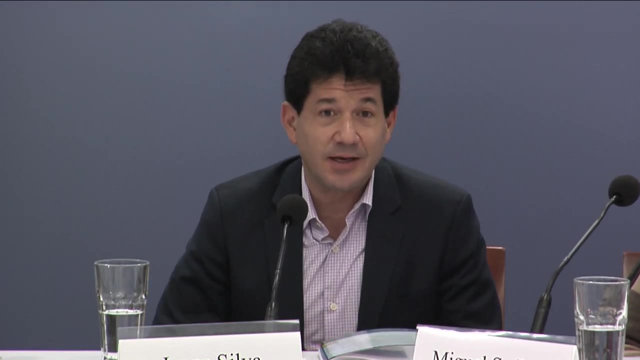 this is not a generalization, but it's just something that actually happens. If you have a PhD, somebody with a university degree driving a taxi versus somebody with high school driving a taxi, perhaps it won't make much difference And you have that actually happening in Latin America. 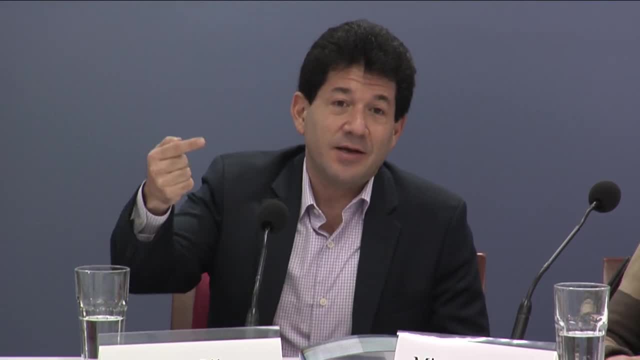 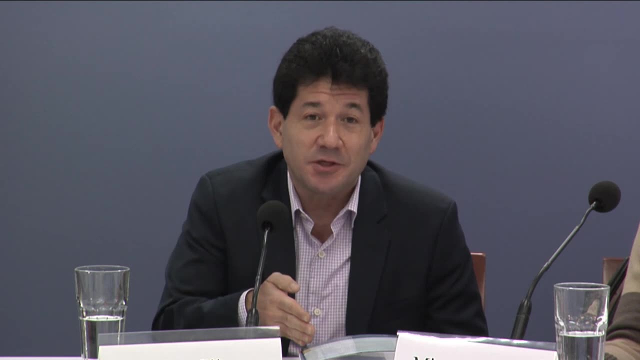 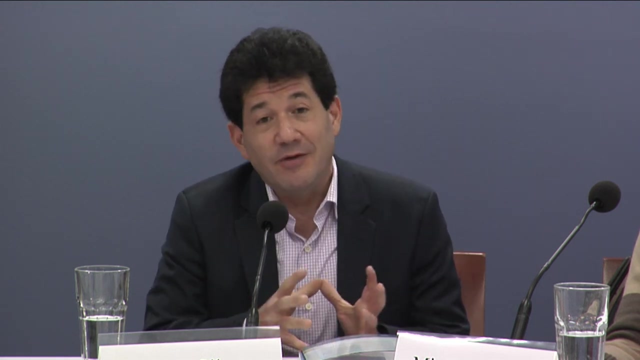 So the effect on the value added of the provision of that service, I mean education, doesn't make that much of a difference. actually, perhaps the university degree person might give a lower quality service than somebody with high school or a lower degree. So if you have an economy, 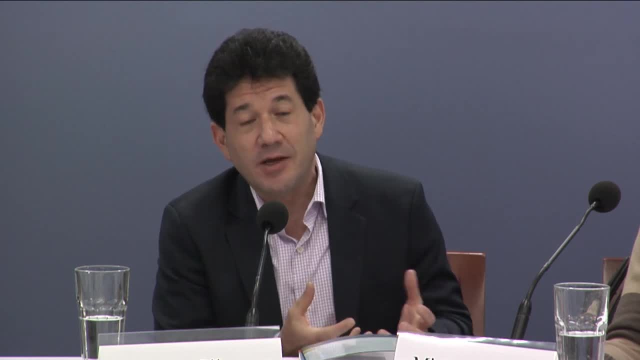 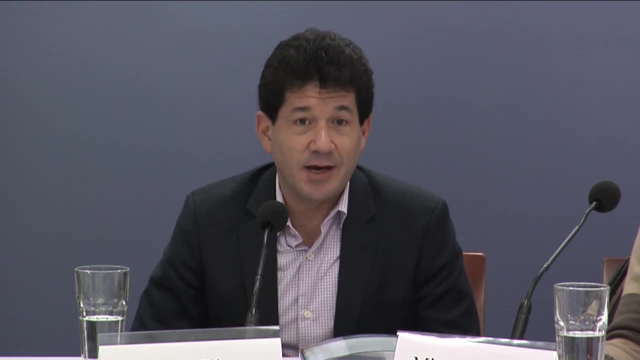 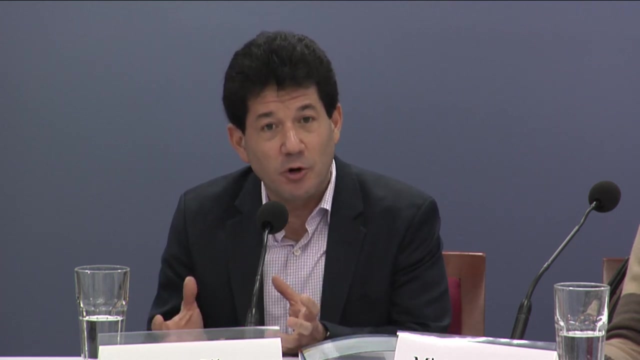 where not enough jobs or opportunities are being generated for that education to materialize in greater value added, then I think part of what you see in Latin America is exactly that It's not only increasing the human capital stock but having an economy that can absorb it. 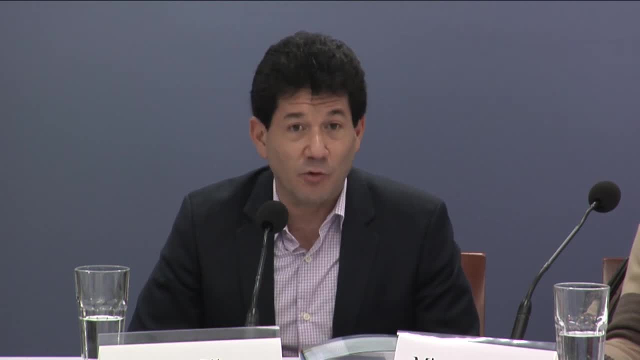 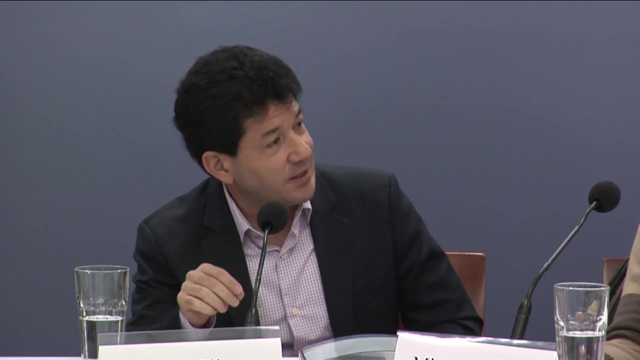 and channel it to increase growth and speed up development. And I think the CCT question is also very, very interesting because it has been a part of the story in Latin America. If you go to the household surveys, many of which already identify who has these kinds of programs. 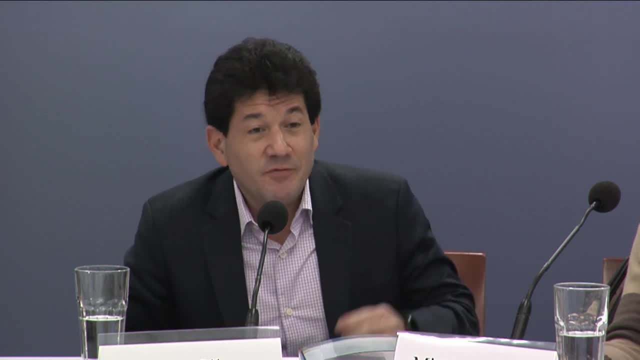 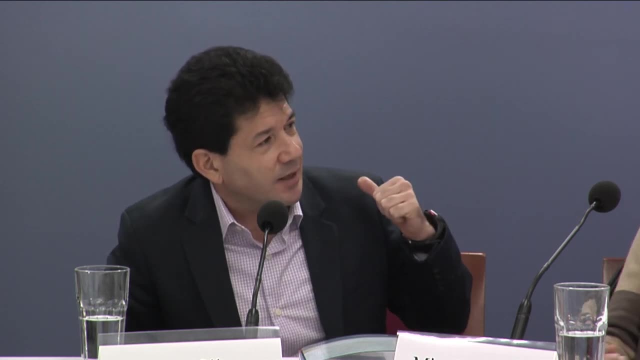 which have proliferated in the region. incredibly, if you calculate how much of the income comes from that, it does make a difference, but it's not huge. It doesn't explain the whole story. Let's say, if you go to these surveys and you take out the income from cash transfers, 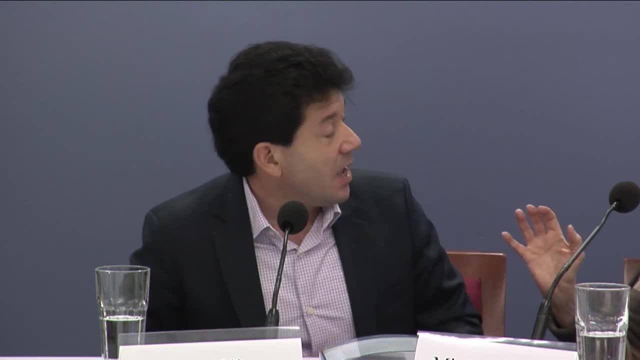 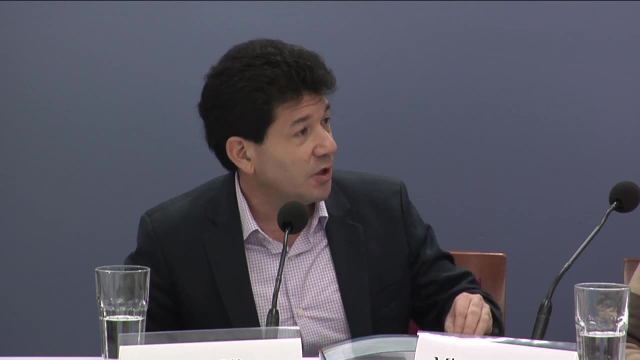 you still see the inequality decline. It's household inequality, But it also is related to wage inequality through the human capital investment, because the logic of at least the conditional, which were the ones that started, was that this was a way of investing in human capital. 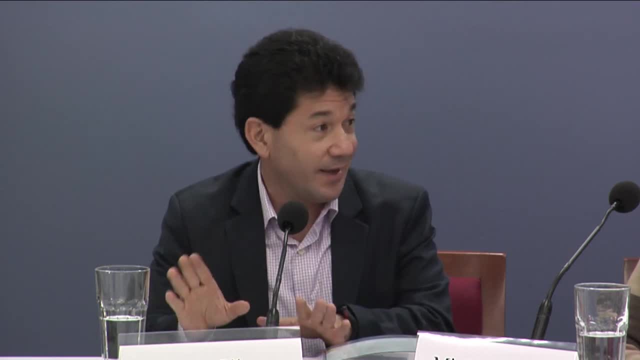 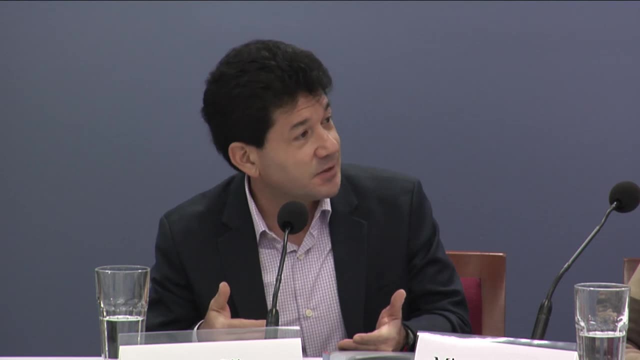 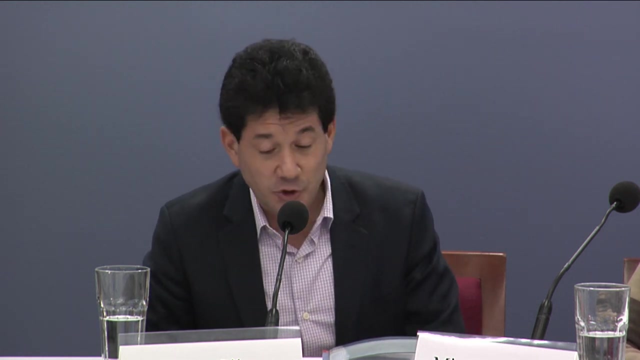 and then you would have greater productivity, etc. which again hasn't really materialized. Actually, one of the big questions with the conditional cash transfers is that now we have all these highly better educated people, but they're not finding jobs to put that education in action. 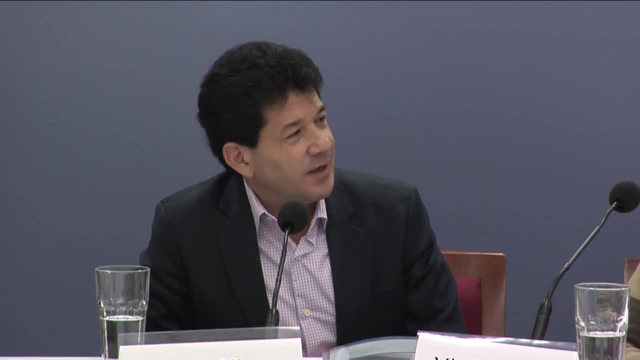 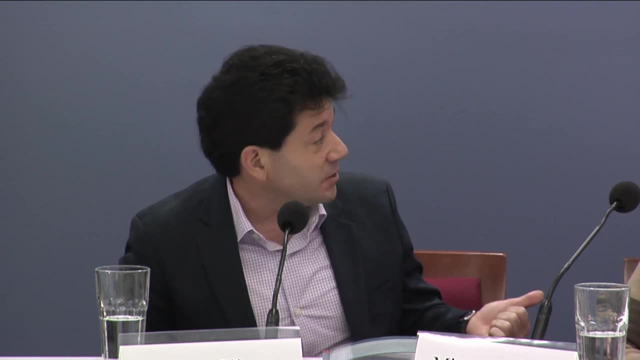 But the CCT issue, I think, is broader than only that, than accounting for how much of the income, And it has to do a lot with the changes in the political system. at least I think I'm sorry to give a not very optimistic view. 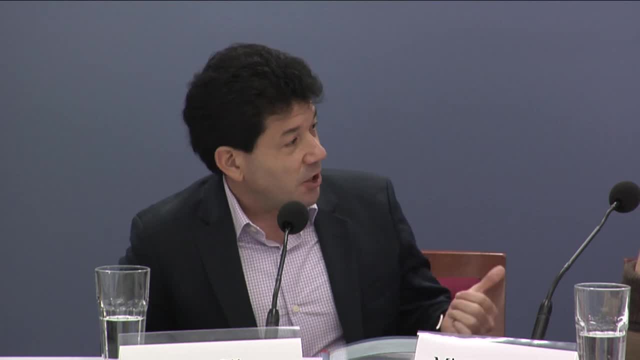 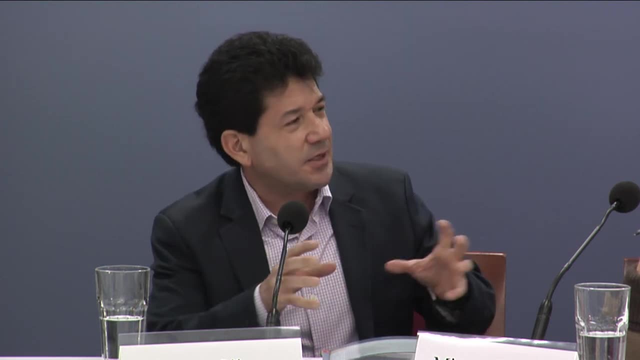 but I think what we're seeing is, on the one hand, there's very little discussion on the tax system and how that could be made more progressive, But on the other hand, there's always this argument that well, if we get some more money, we'll spend more. 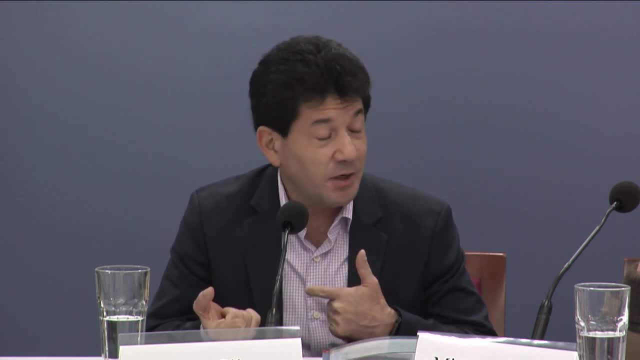 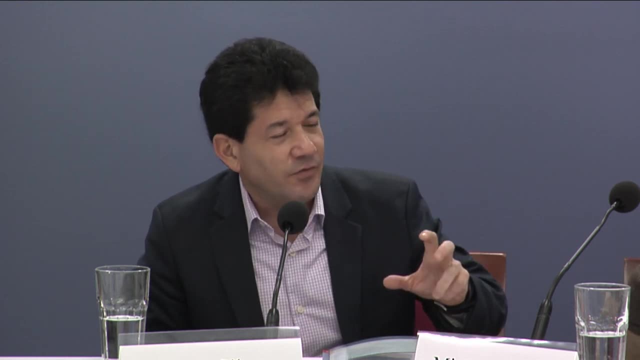 and that will take care of the problem. But the way the money is being spent actually makes a huge difference. Conditional cash transfer programs at least had this view of investing in human capital, so you would have a short-term effect, but you would also have a longer-term effect. 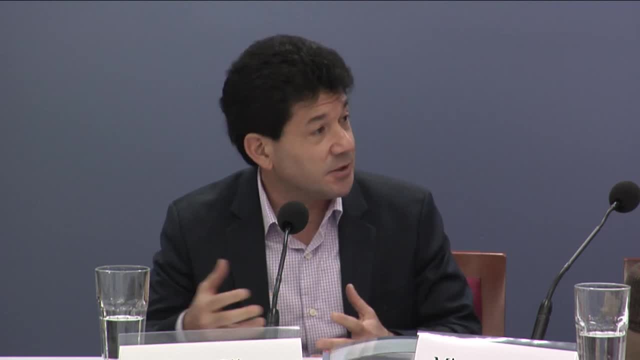 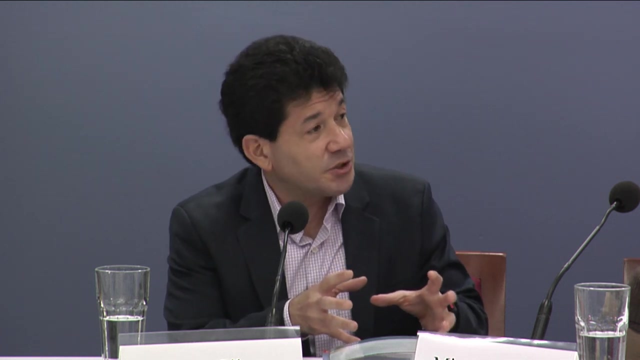 a longer-term effect on the capacities of the poor, But in combination with the political system. the way the political systems are working in the democracies in Latin America. what you have now is basically a segregated system where a minority of the workers have access. 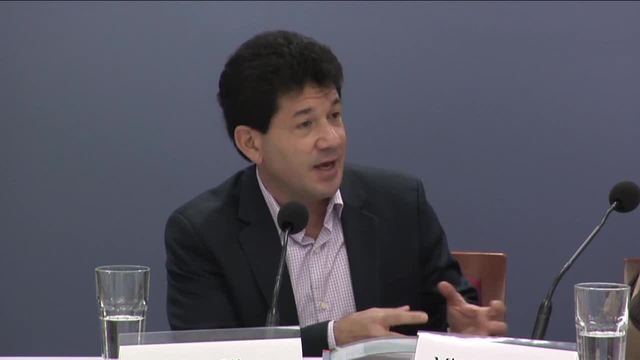 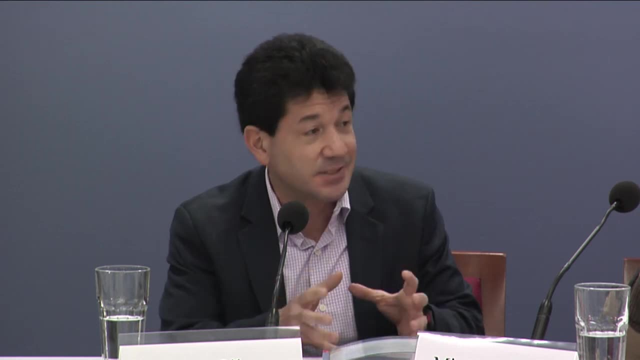 to the institutionalized social security systems- pensions, et cetera- as a right, not as a handout or as a transfer from the government, but as a right because they're working. And then you have, in many countries, a majority of the population. 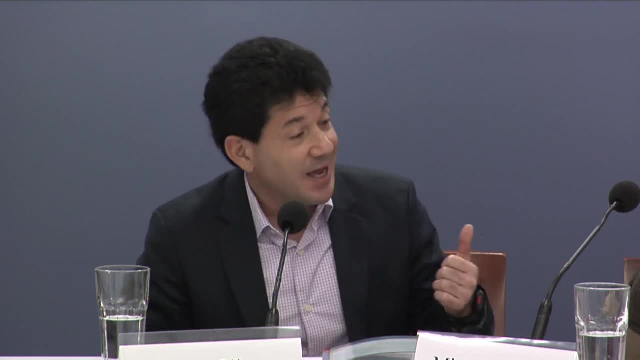 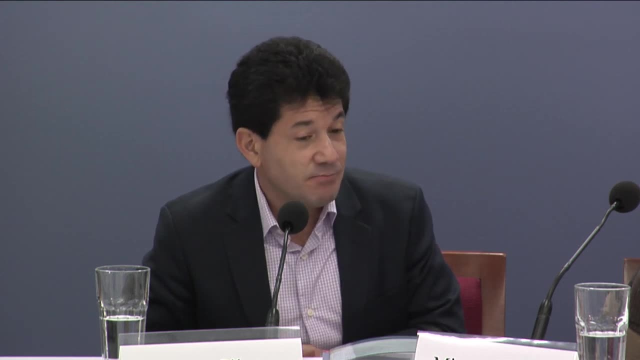 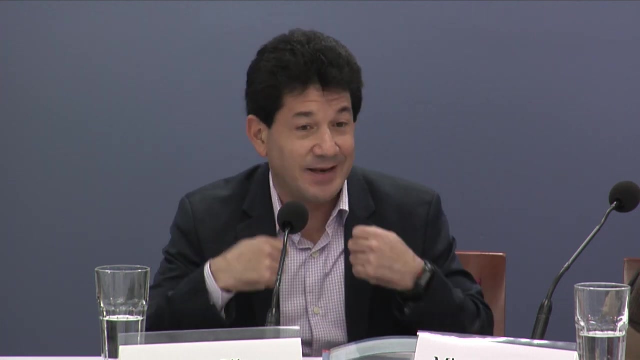 subject to whatever the government gives them through these cash transfers. And it's linked with the democratic developments, because now it is much more rewarding for a politician to go out and give now a cash transfer for the elderly, for the disabled, and they go and they have the picture. 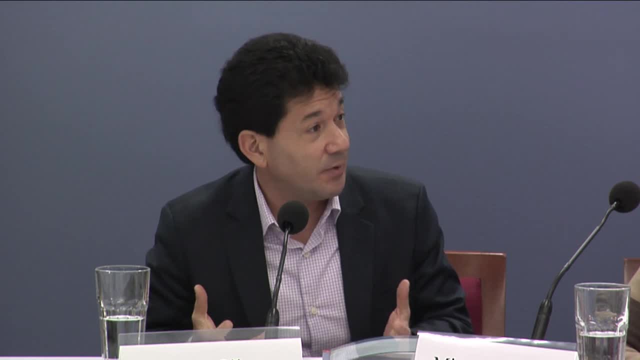 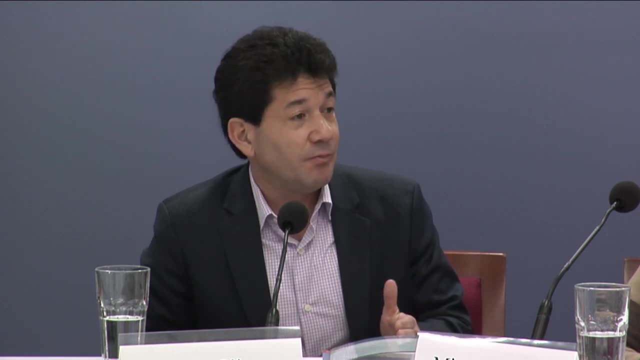 they cut the ribbon in the inauguration. It takes time. It's really been capitalized very favorably for many politicians in the region. When somebody gets a pension because they have contributed to the pension system for 30 years, you don't thank anybody. 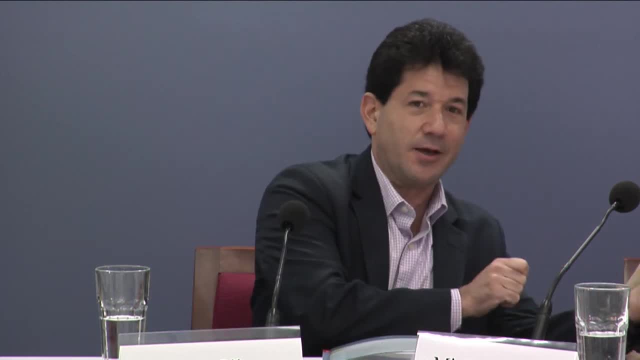 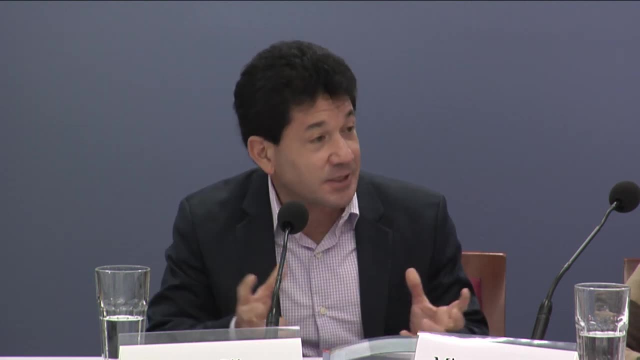 It's your right, So you don't have the politician going to you and giving you the check in TV. So that doesn't really give any leverage in the context of the democratic systems of Latin America. So I think they might have a short-term effect. 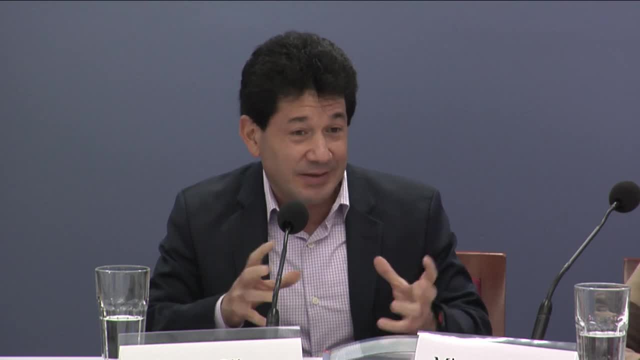 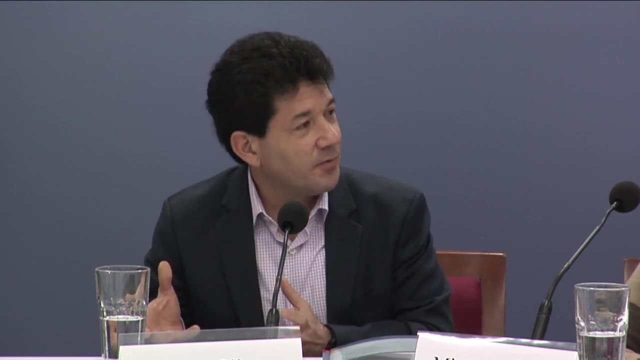 Perhaps even a longer-term effect over human capital. But I think the picture is now so distorted in that area of just saying we'll spend more and that will solve the problem. That's not really solving the problem And it actually might be creating a new time bomb. 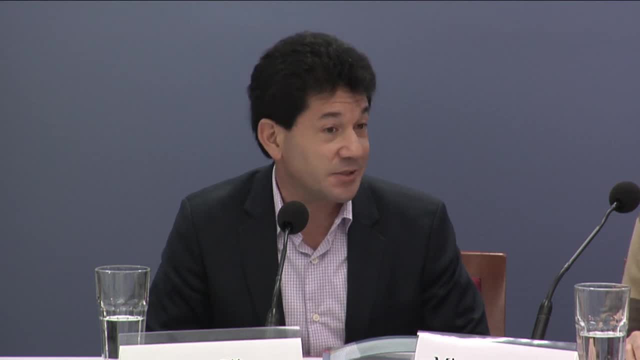 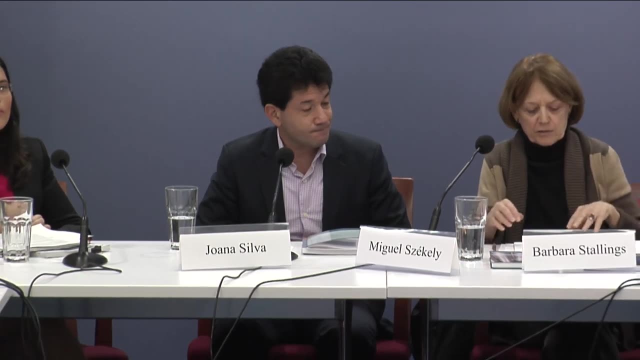 in terms of pressures over the government expenditures that perhaps will have more negative effects in the future. Let me say something about the question back here in the back: Unionization, collective bargaining, collective bargaining, et cetera, Traditionally in Latin America. 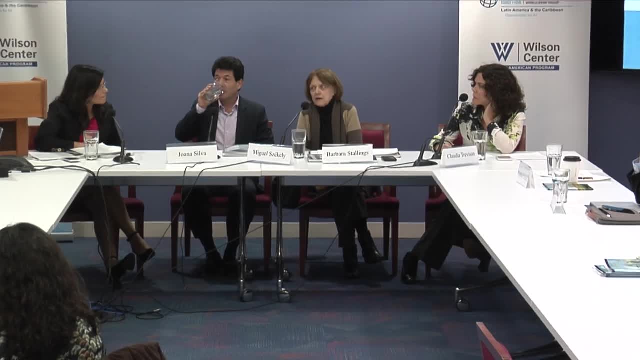 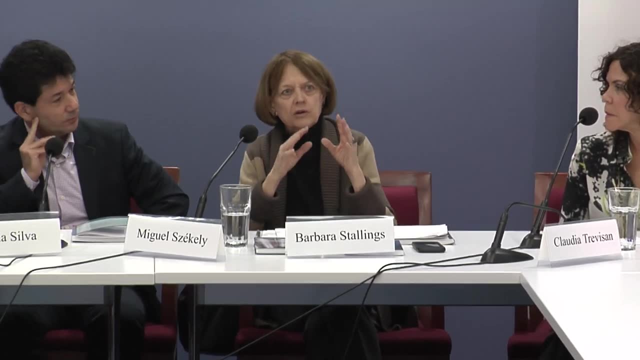 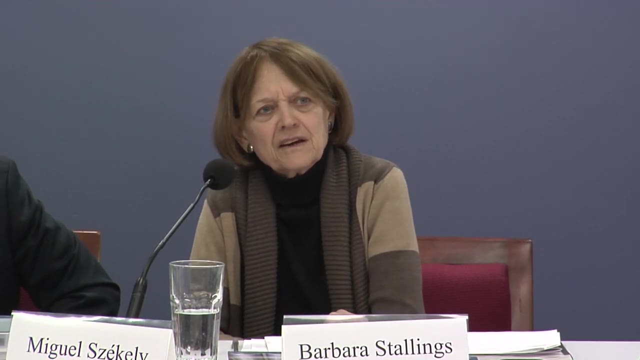 unionization has been a factor promoting inequality, That the small group of unionized workers- and this goes with the formalization as well, because in general unionized workers are formalized workers- So that's been a negative thing for the society as a whole. 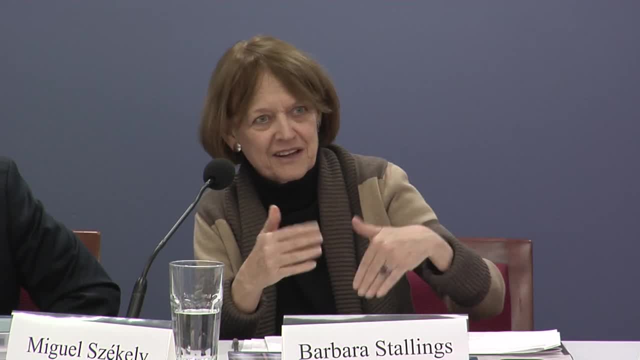 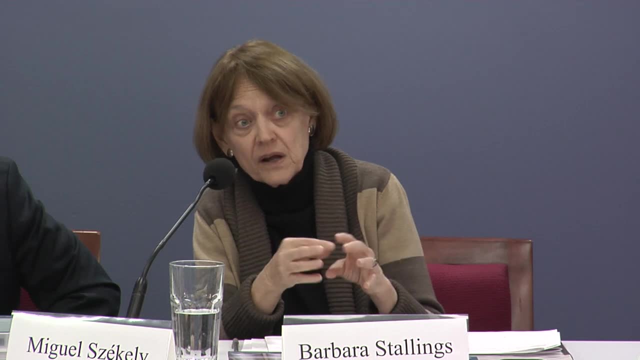 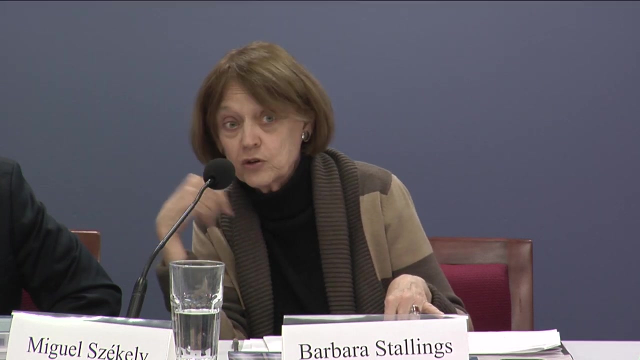 Obviously, it's a very good thing for those who are unionized and can get better wages. Now you were aiming at at a somewhat more specific question about nationwide collective bargaining, and does this reduce the inequalities across firms, which is one of the important stories that's told in this book. 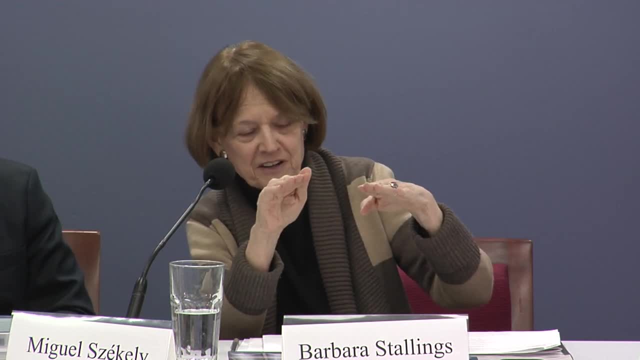 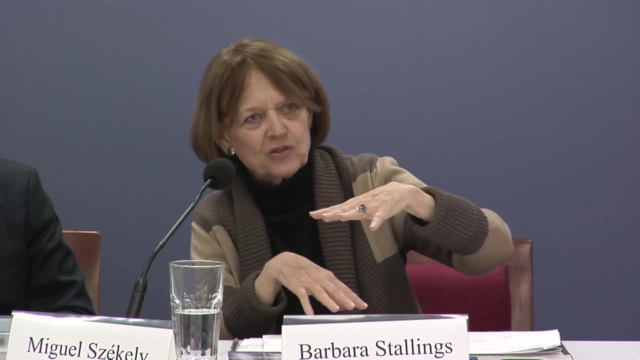 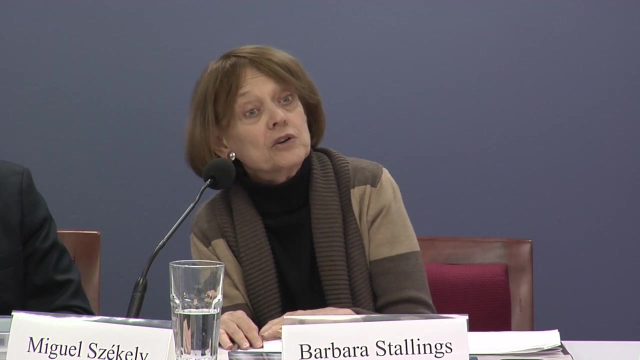 Even so, maybe it reduces that kind of inequality, but it will increase inequality between unionized and non-unionized workers. So it's hard to say. At best it's probably a wash. There's a lot of literature on Europe. Social Democrats in Europe think that national bargaining 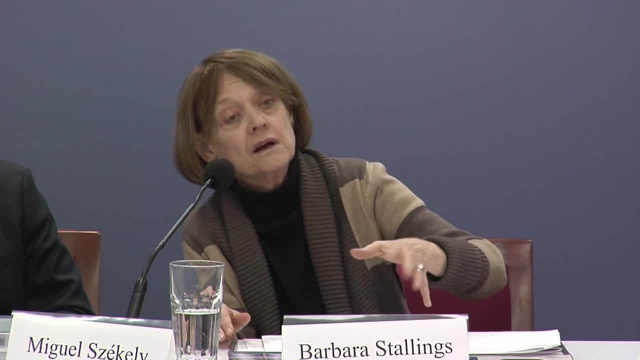 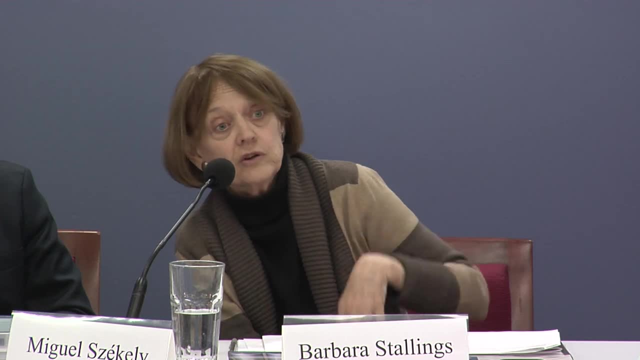 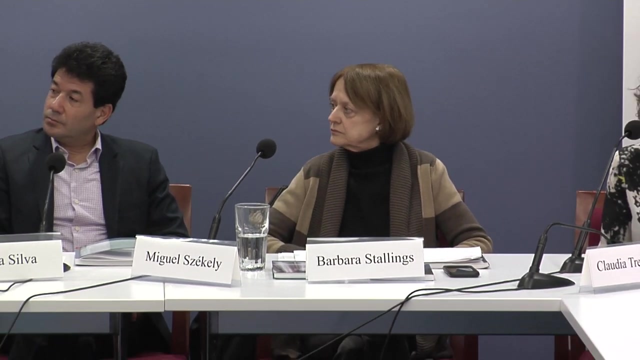 is a very important aspect of their lower level of inequality. So there's some leverage that might be gained by looking at what's going on in some of the European countries compared to the ones that you referred to here. Just a couple of points On CCTs, on the conditional cash transfers. 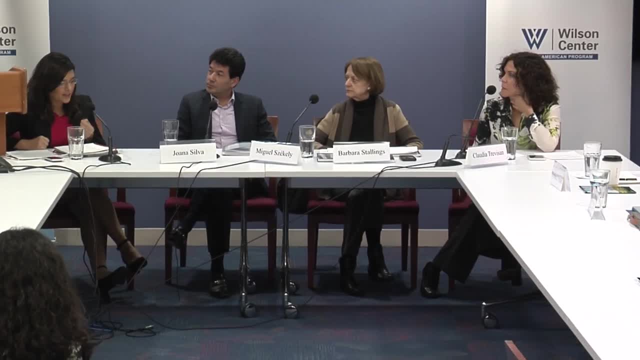 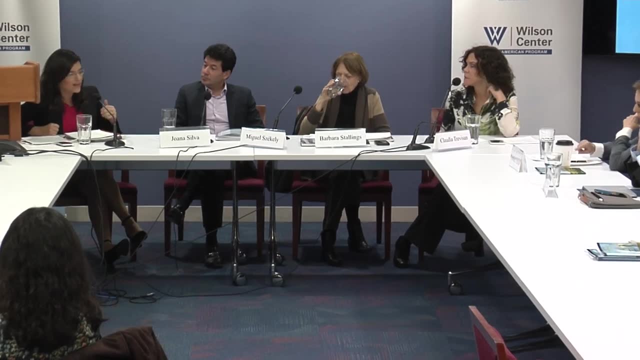 such as Bolsa Família in Brazil. they are designed to affect, affect poverty and they affect human capital formation, But mostly they are designed to affect to reduce poverty. They have also the second tier of effects by keeping children in school and improving the education levels. 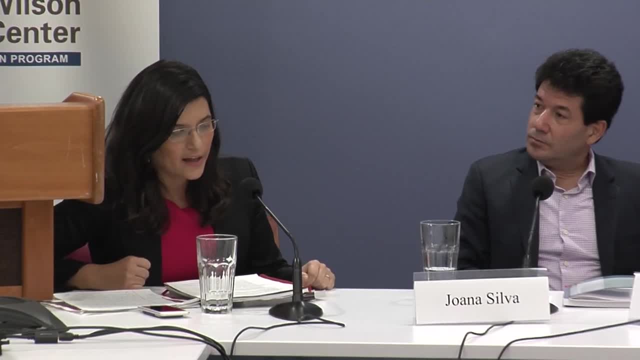 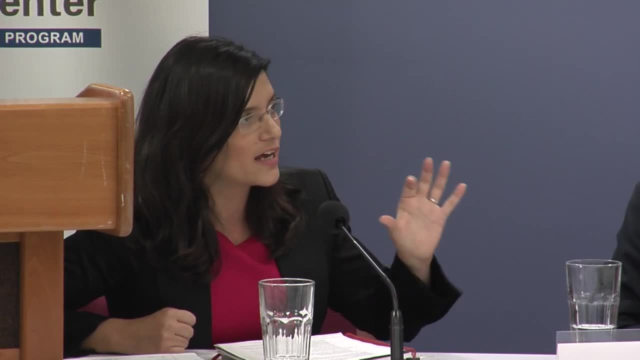 and this could have a positive effect, A long-term positive effect. They are not the biggest drivers of wage inequality because they are, in terms of income, a small size transfer. So they did not roll down this massive reduction in wage inequality, But this is not to say that they had 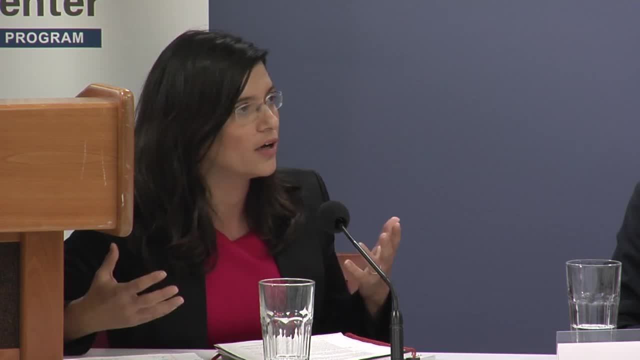 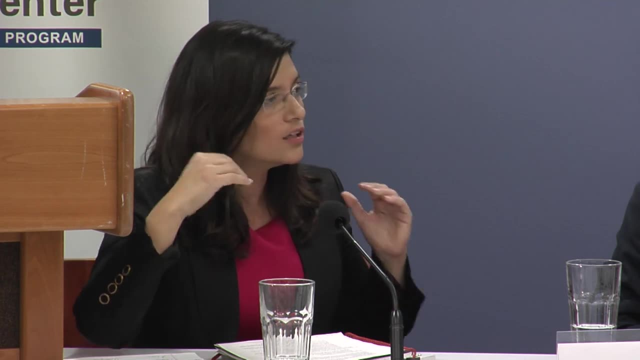 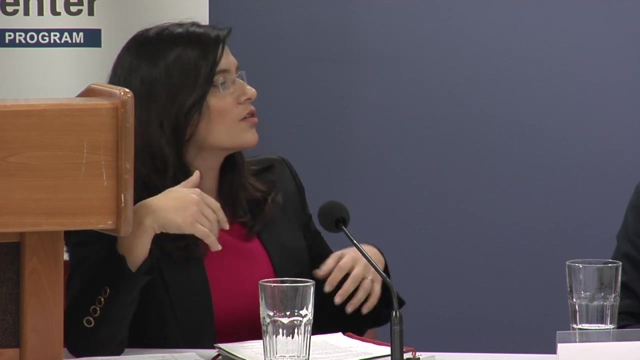 a negligible effect on income inequality. In fact they had- about they counted them- plus pensions, which have a larger impact. actually, The non-labor part accounted by more or less one-third of the reduction in income inequality, In wage inequality. 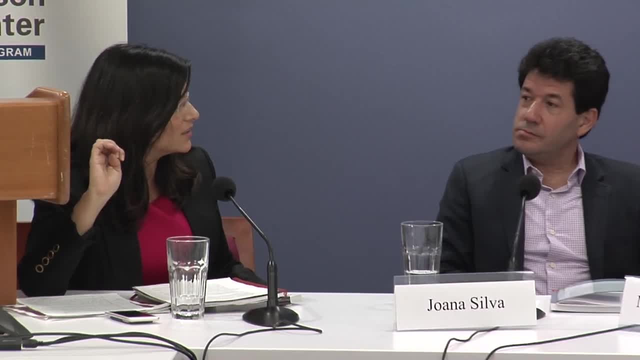 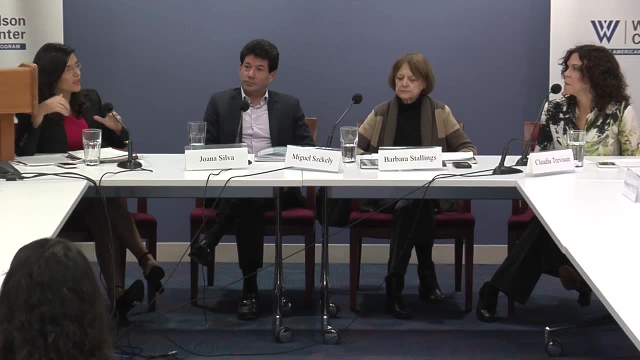 Income inequality, Household income- Exactly, exactly So one-third of the reduction of income inequality was due to non-labor, non-labor transfers. So it includes pensions, which has a bigger effect, and then a smaller effect from CCTs. 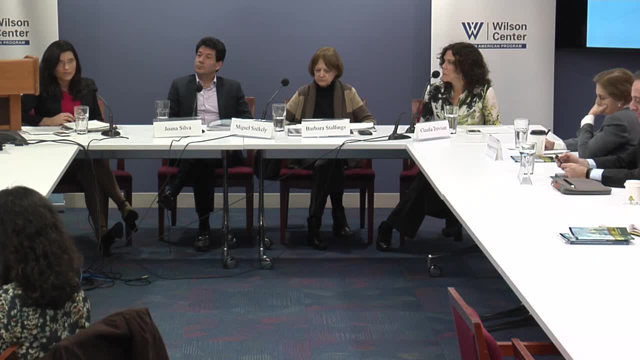 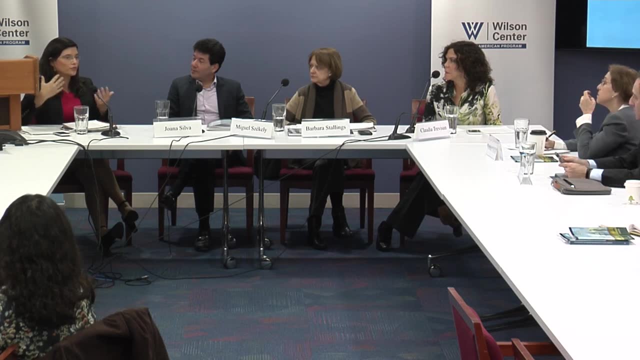 Also, why do we care about inequality? Not all inequality is bad, and we make that point in the book. Inequality that is bad is the one that doesn't allow you to fulfill your potential, that doesn't allow you to seize your opportunities. 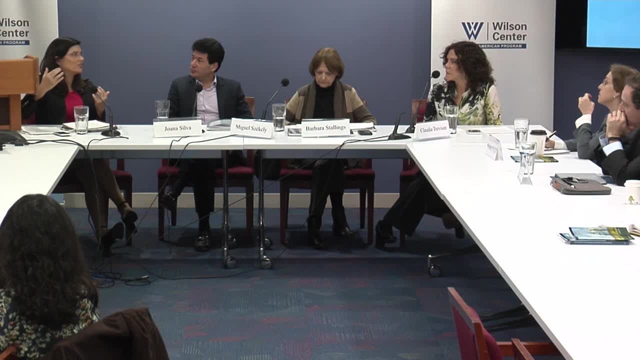 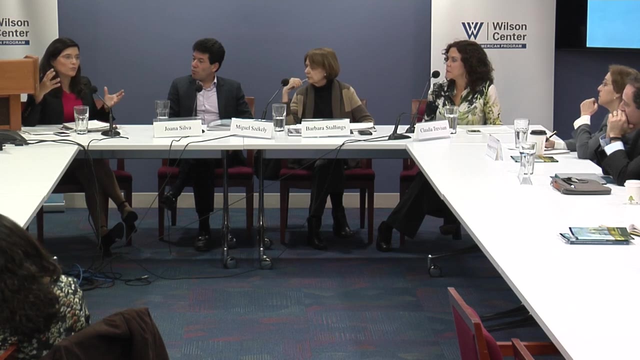 that doesn't allow it, as a poor kid, to have a quality education. So this is the type of inequality that we are concerned about And in fact, in Latin America, even in the Central American country, in Mexico, the inequality reduction came with 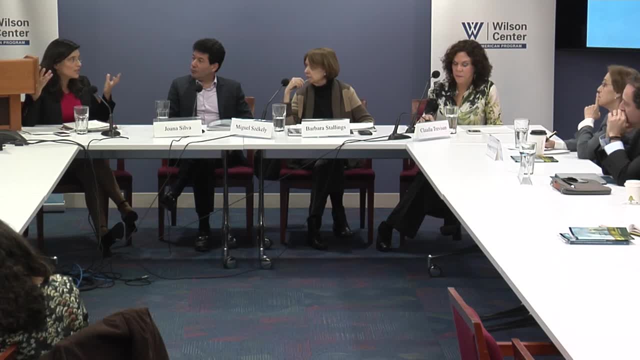 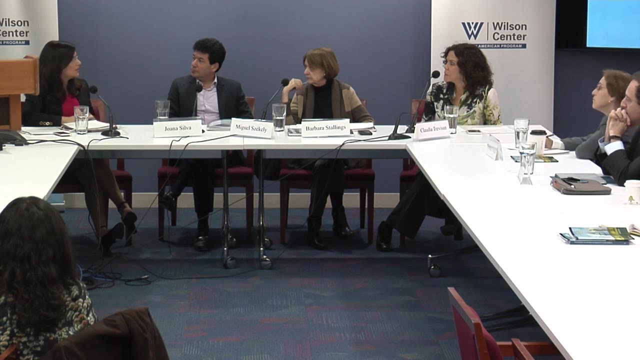 labor markets that were pro-poor Most of the action. the biggest increase was in wages of low-skilled workers. So these are developments that are important to keep in mind when one thinks why to care, because these improvements can improve the life of many. 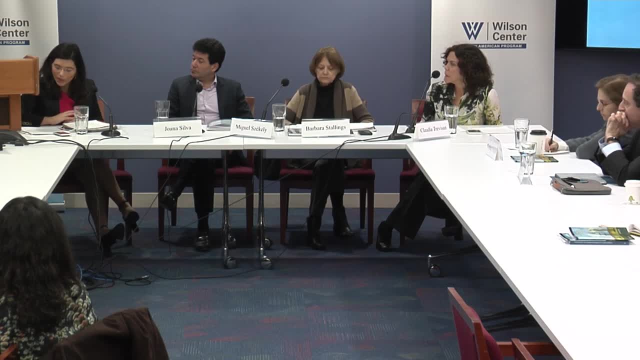 along the education expansion in the society that also raises wages. Then this idea of productivity. This is exactly why we say that there is a two-tier approach. Productivity is really important And we need to Don't go against the flow. It's important to protect productivity. 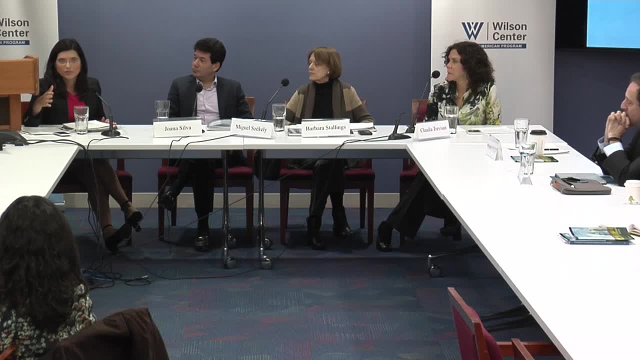 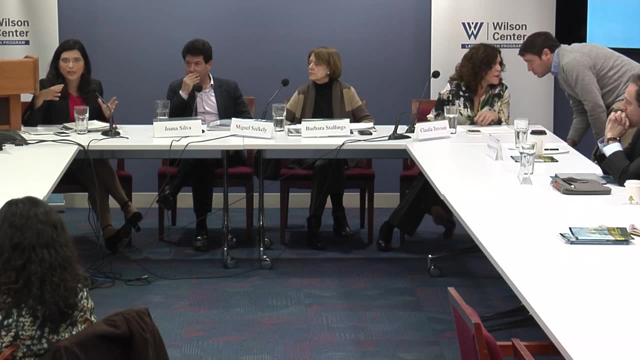 That's why we say: look at policies that are protecting efficient firms. Look at policies that don't allow productive firms to flourish. Act on those. Don't be an obstacle to technology adoption That can improve your productivity and can have long-lasting effects. 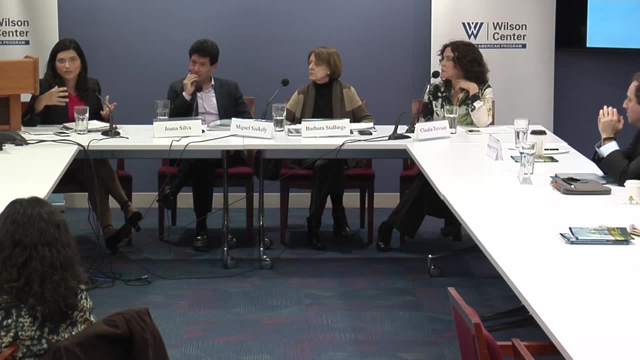 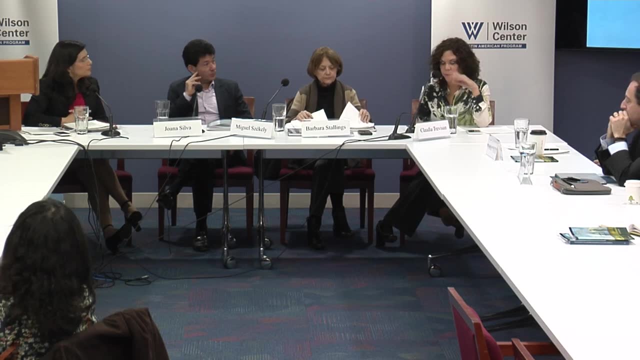 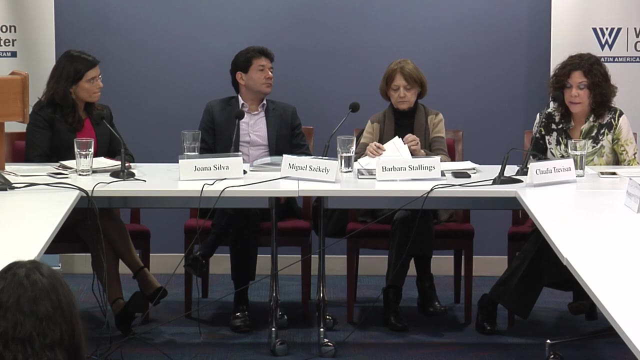 Also education. Improving the quality of education will have productivity effects and long-lasting effects, And indeed this is a very important aspect and one that the region should care a lot. We have two questions from our online audience. One about the: Has wage inequality decreased? 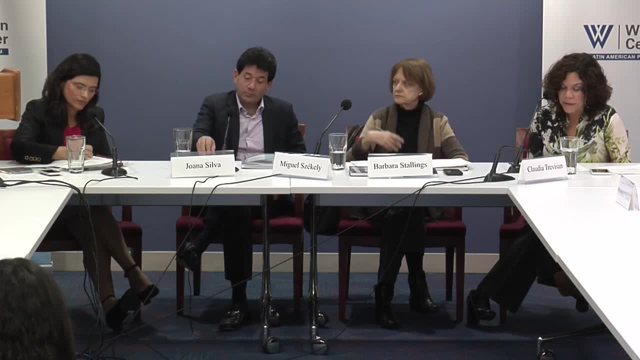 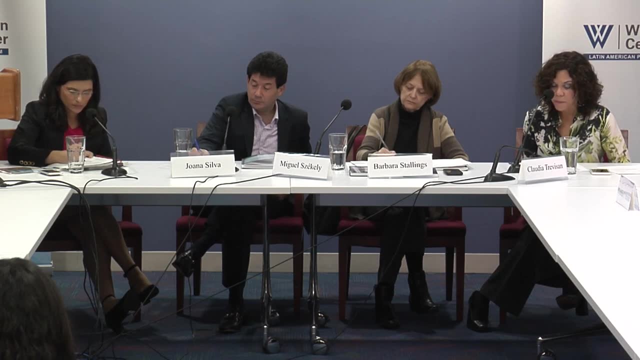 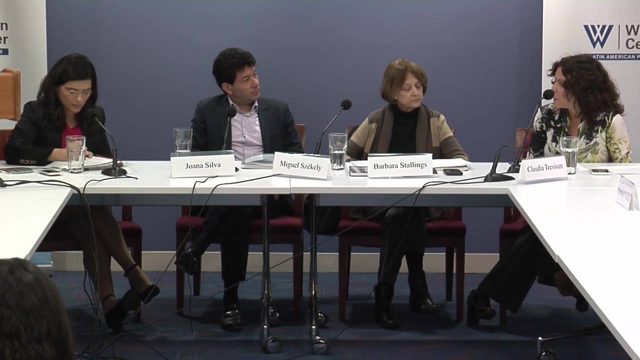 for both women and men. I don't know if you have this response in the report And another one regarding education. In Brazil today we see many people with higher education out of the labor market. Exactly what Miguel was mentioning Is a degree worth it. 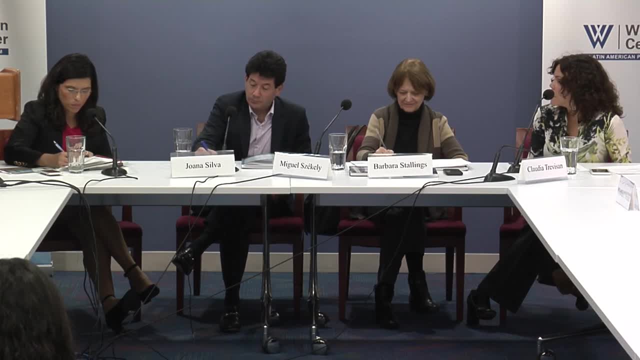 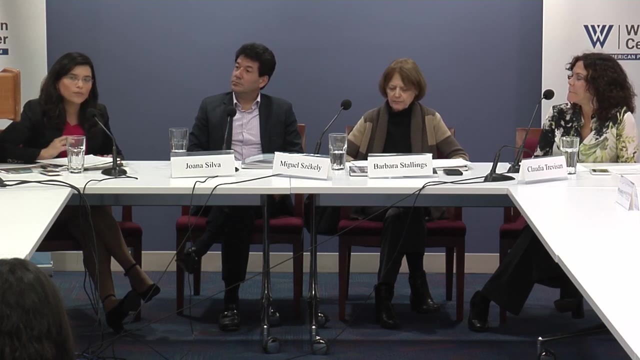 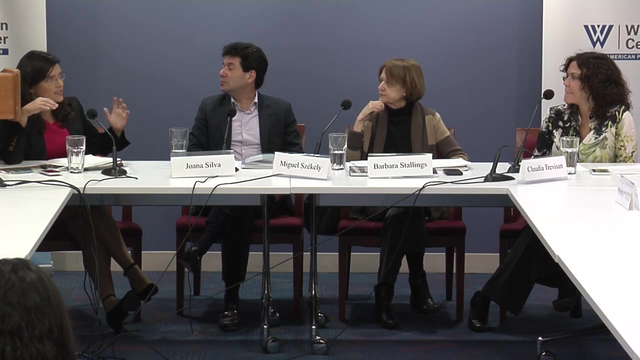 And government should invest in technical education. Who starts? So why don't you talk about the gender part if it's in the Yes? So in terms of wage inequality, we've seen reductions in many gaps, in the gap between urban and rural areas. 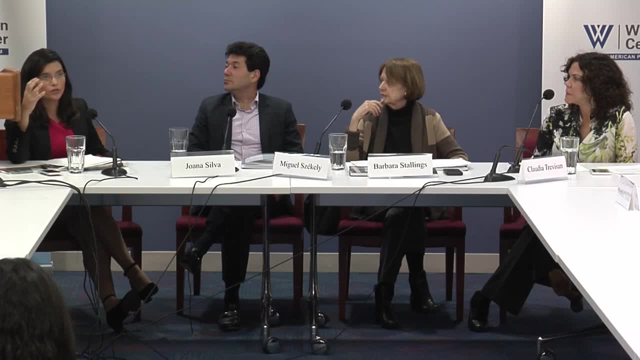 in gap between men and women, But these had a smaller contribution, although not negligible, but smaller than the massive reduction across skilled and unskilled workers or across wages in different firms. So this is an important factor. This is a gap that closed. 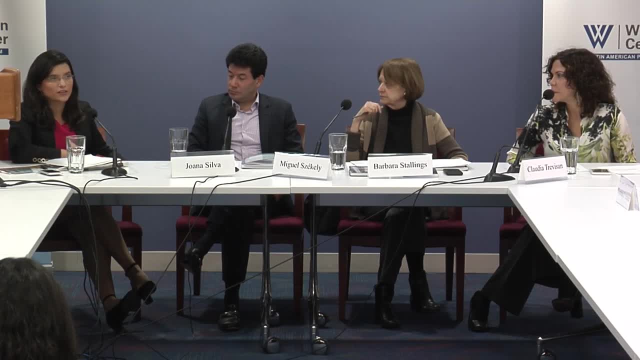 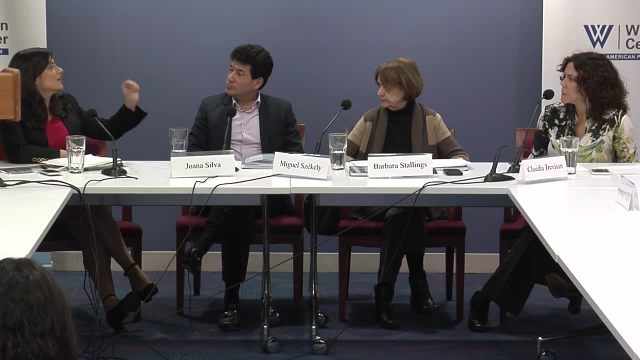 in Latin America, but not as important as other factors, but important to keep in mind In terms. How about the increase of women in the labor force? That affected income inequality? So, through these non-labor markets, So as more people. 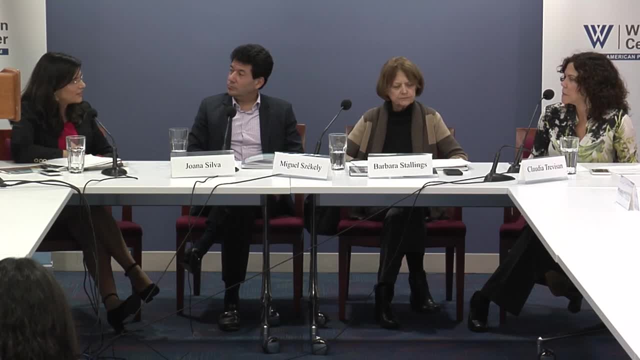 I'm calling household inequality. Okay, Exactly, Exactly. That had an important role there and was an important factor in several countries. Sure, So, is a degree still worth it? Definitely So. a college-educated person in Latin America still makes 3.4 times more. 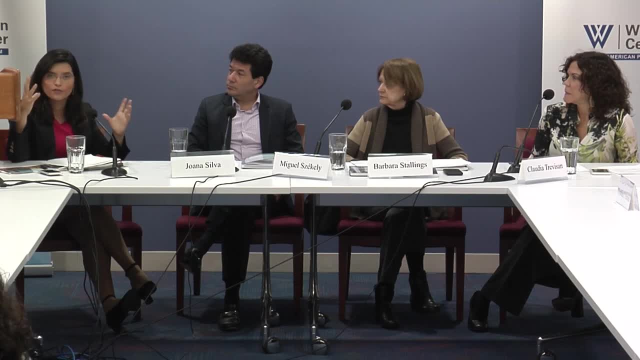 than a person with primary education. This is controlling for all their characteristics, from their gender, from where they live, et cetera. So definitely it is still worth it. Are we where we want to be in education? No, We want to be better. 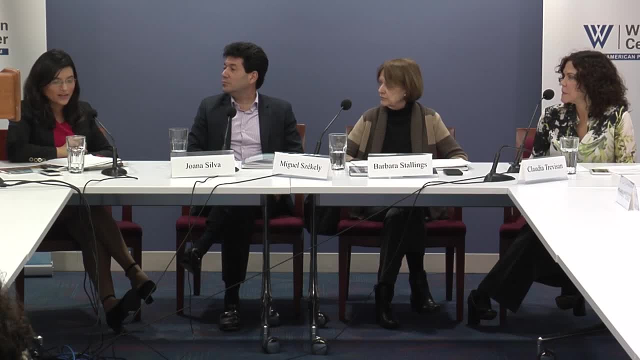 We want better quality, and this is a key thing to keep in mind. And training is a key aspect because, like you said, we don't just care about students in school that then arrive at the labor market, but we also care about those. 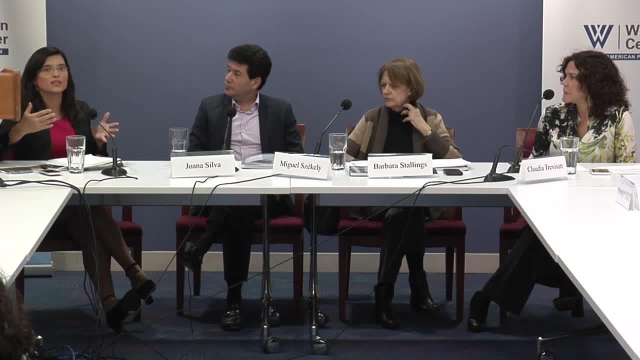 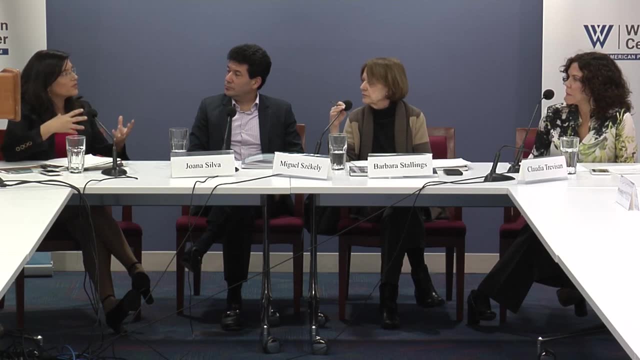 that are already in the labor market and they need to improve their skills for better wages and sustainable livelihoods. So we definitely care a lot about that. And then in the book we don't specifically exploit which type of training we should invest on. 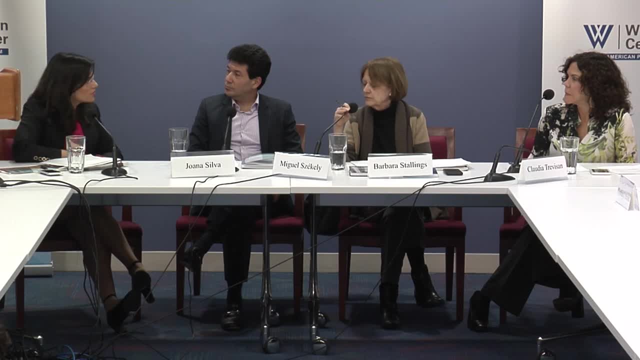 but we stress the importance of building skills for the workforce. Let me just make one little comment to add on to that. In this book that we did, that has a different chapter, not the Conley chapter, but a different chapter on education. it's interesting that. 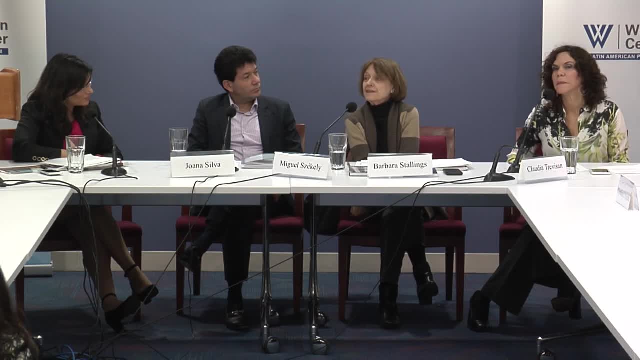 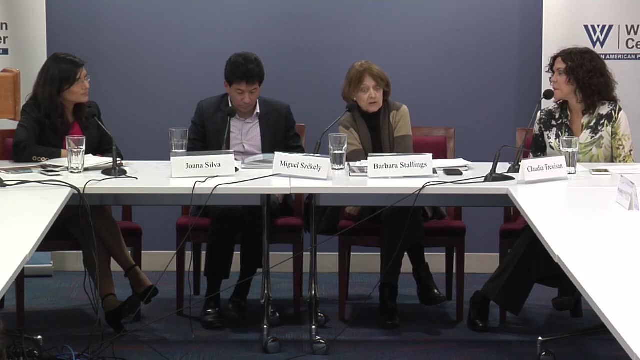 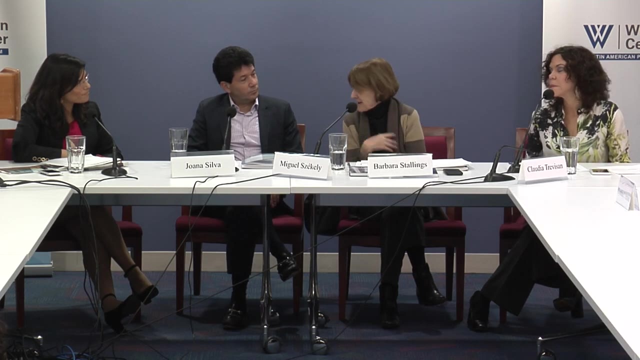 technical education, training, was in the past an extremely important aspect of the Asian story of economic growth. But here is the downside: As the country grows, as education is increased and as it's now that getting a university education is a prestige mark, people are less willing to go. 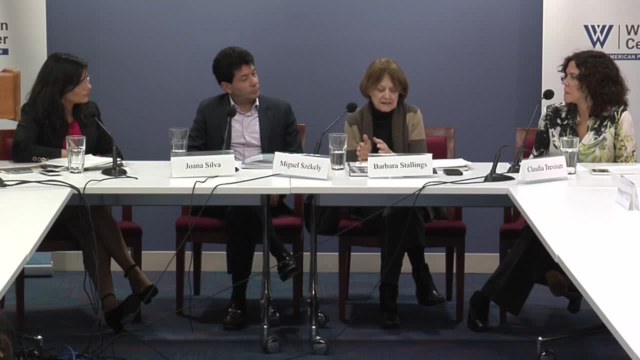 to technical schools than they used to be. So one needs to figure out how to make them attractive, And it's interesting that I guess in this country people are beginning to say the same thing: Is the college education really worth it, or should I go off to learn? 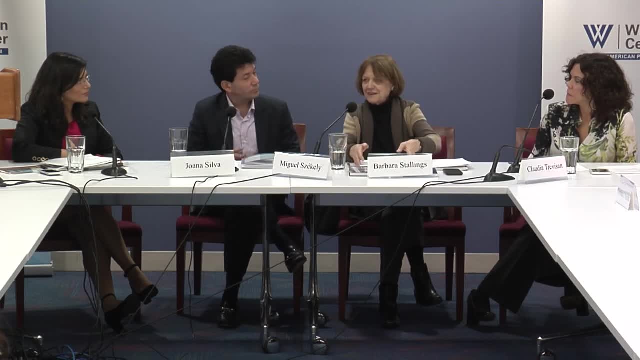 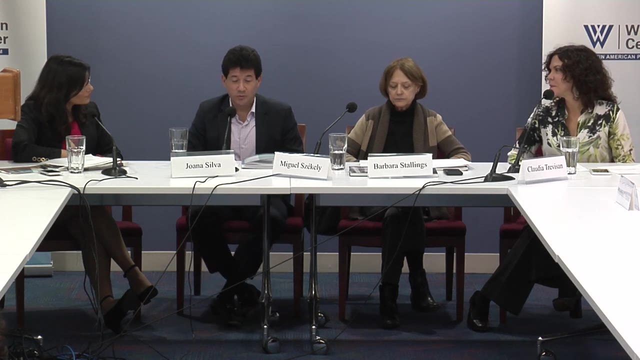 to be a computer programmer, A computer programmer, in a quick course. So maybe there are different ways of You have to think about marketing technical education if you want to bring that into our package of changes policies going forward. Yeah, I also would answer. 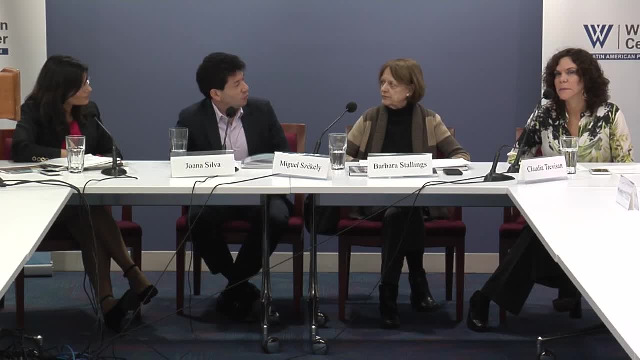 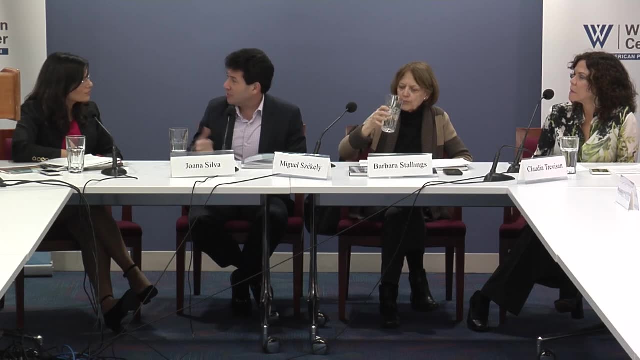 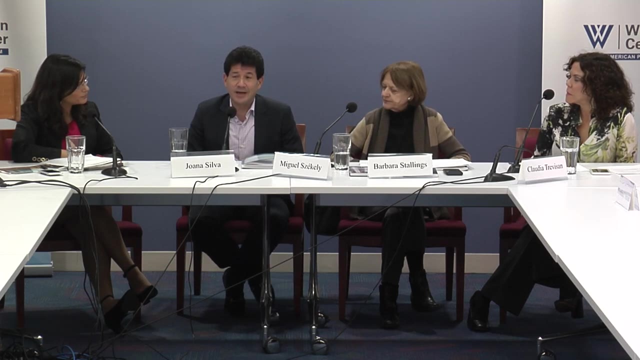 that definitely yes, but much less so that it should be, I think, having a higher education degree. Still, the differentials are very large- 3.6, you mentioned, between high school and higher education, and that is very revealing, But I think we're still missing. 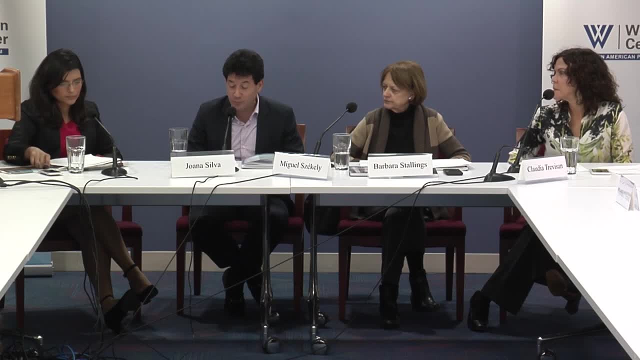 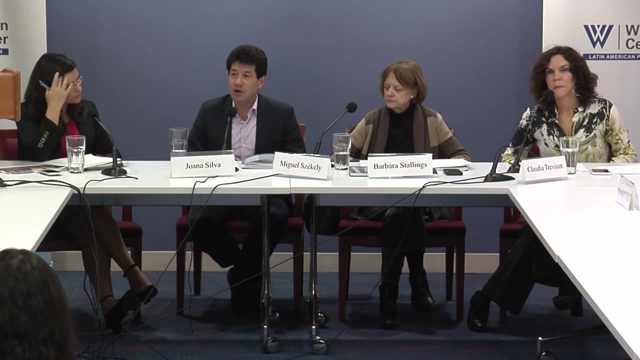 two elements in the puzzle here that should make the investment in higher education even better. One is that it is not any type of higher education. For example, in many Latin American countries we still have an excess of people starting to be lawyers, accountants, et cetera. 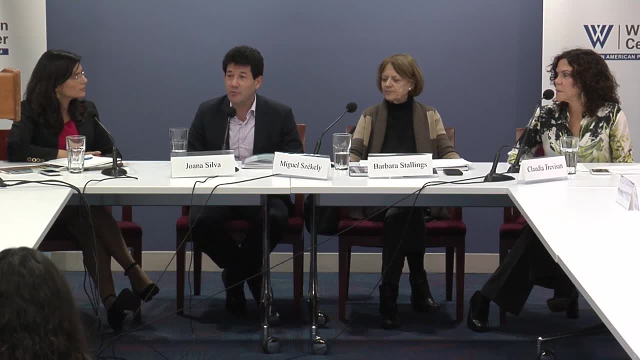 and there is a whole new area of different careers that are more linked with opportunities not only in the countries but in the world in general, And the second is that So part could be supply and the quality, but the other, which I think is, 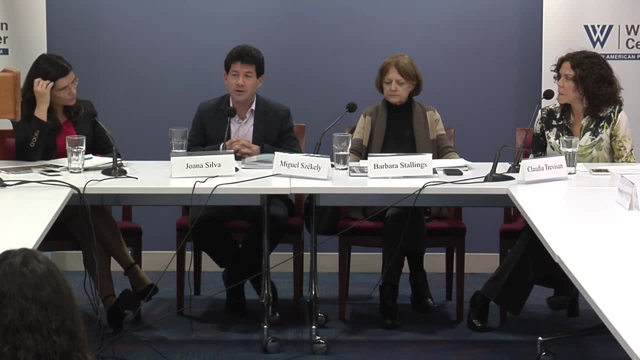 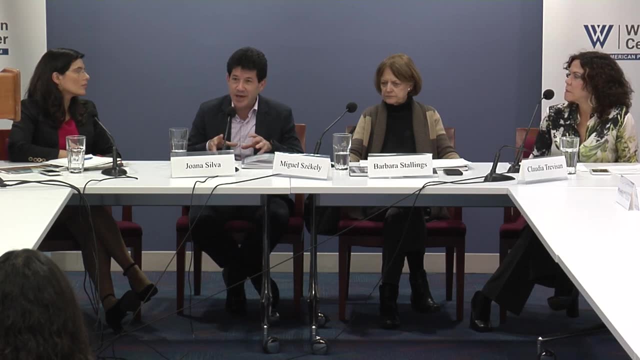 the most important one- and it refers to examples like the one Barbara was mentioning of Korea- is that I think that in Latin America we don't really have this view that education, and especially higher education, is a strategic investment. for something else, It happens more. 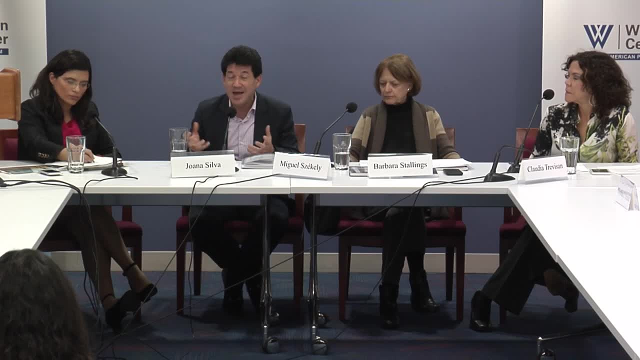 because we have, because there is supply that exists, because there is funding, but there is not really a strategic view. And many Asian countries actually made a big jump when they took this strategic view of not only investing in education in general, but in what type of education? 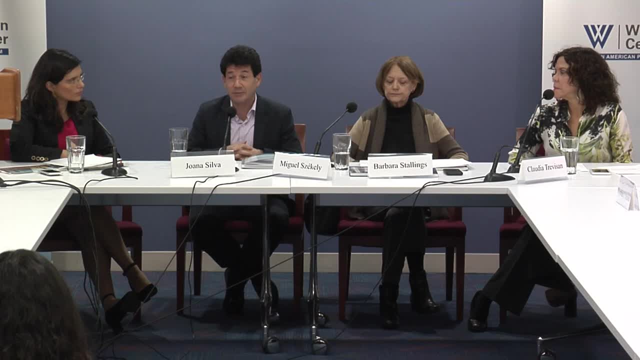 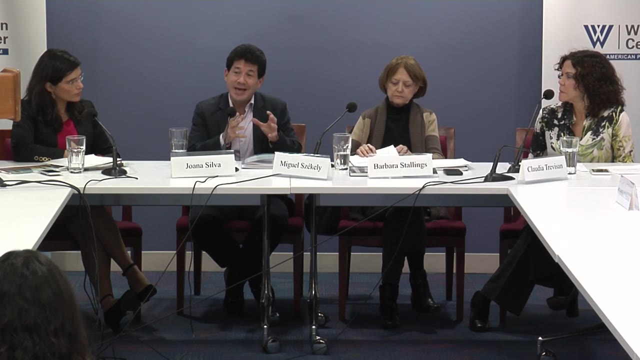 in particular- And there are many success stories- like Ireland and many other, many Asian countries, where first, what the countries did is set a target in terms of developing some sectors of the economy and then really invest as a policy, as a national policy, in developing the capacities. 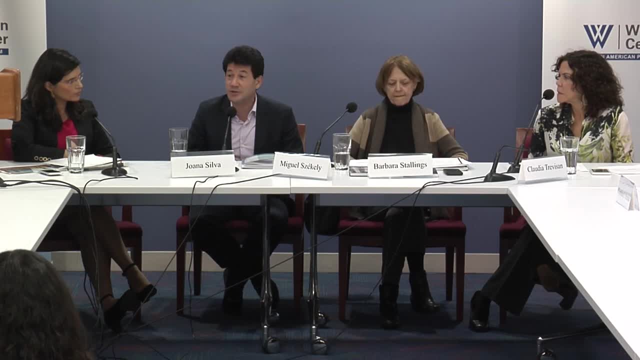 for generating the supply of higher education, exactly for those sectors where they identified that there was an opportunity. If we look at Latin America, I don't see that happening anywhere And I think that would definitely make a big difference. It would have to do. 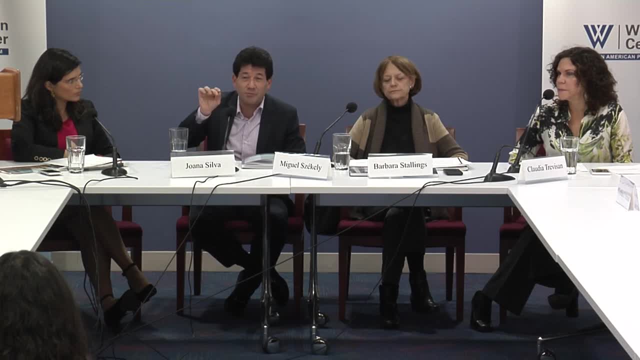 with productivity, because if you don't just invest in education, but in a certain type, that you need to trigger the potential of one sector, which would be more a strategic view, I think that would really make a bigger difference And you would perhaps see increasing returns.